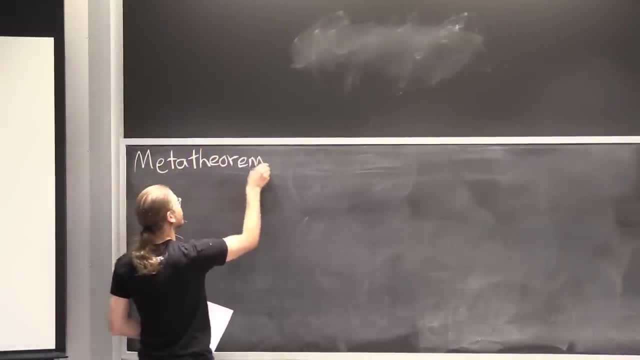 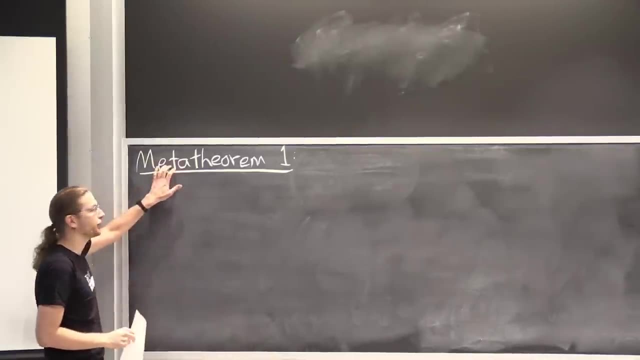 and the fun part is applying them to various games, And they apply to a lot of different games. So meta-theorem we're using here in a somewhat vague sense. This won't be a formal theorem because it's hard to state all of the assumptions. 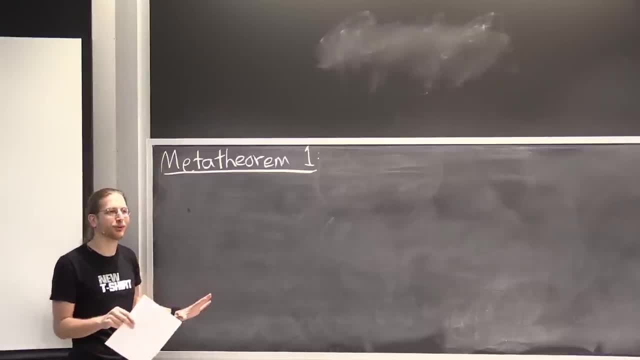 you need about your game, But it's sort of think of it as a really roughly true theorem. We're not going to state all the assumptions you need, But the general setup for meta-theorem one is that you have a player or the paper calls it an avatar. 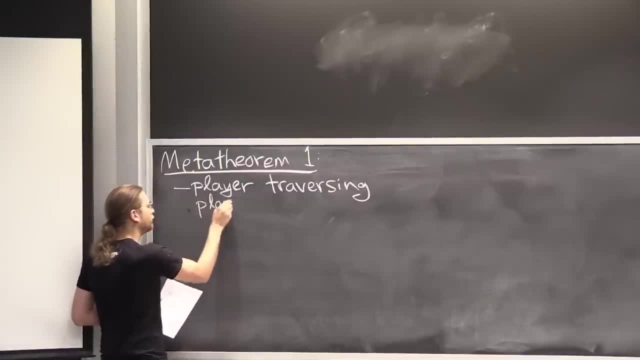 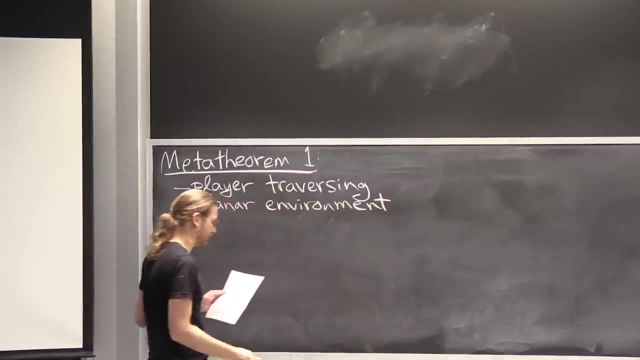 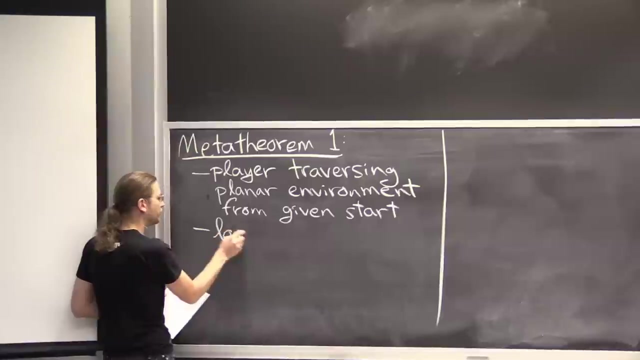 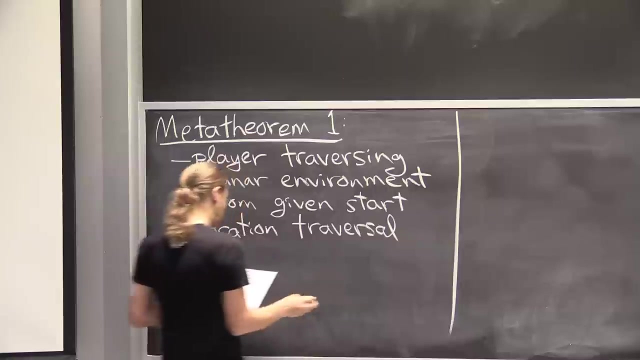 a little guy walking around. You're traversing a 2D environment, so you're not allowed to have crossovers from a given start location And, given that setup, if you have two features in your game, one is called location traversal. 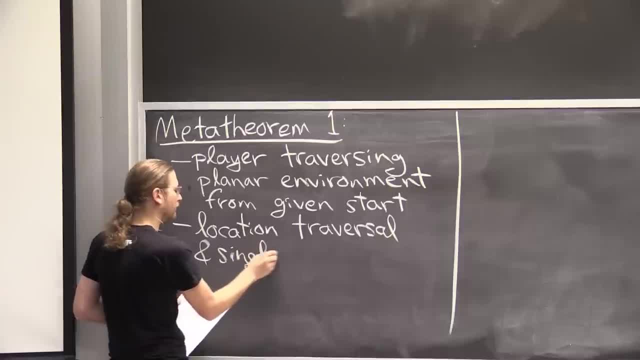 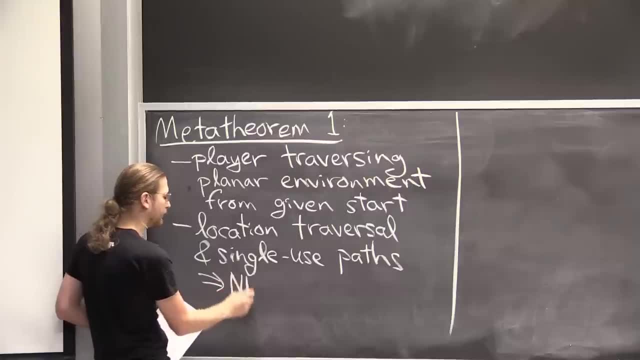 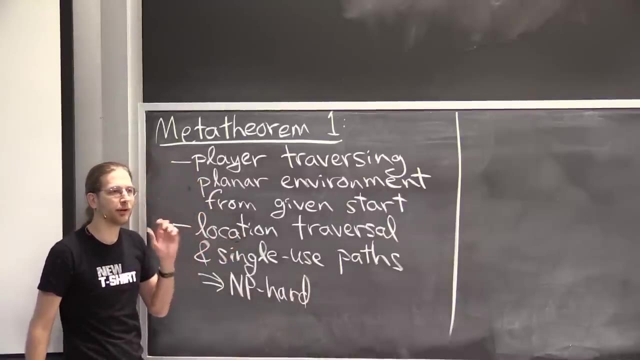 and the other is called single-use paths, then your game is NP-hard. That's the meta-theorem. So Location traversal means that there are some locations on the board that you have to visit in order to win the level, So there's no target location. 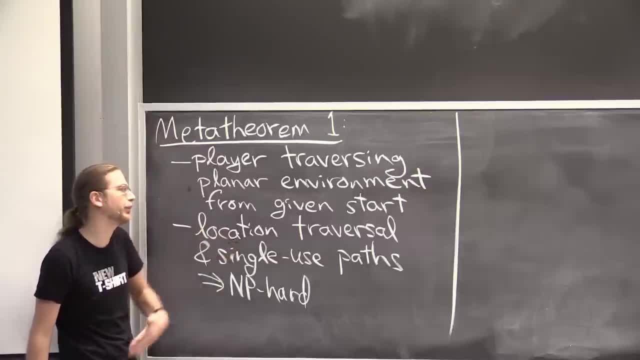 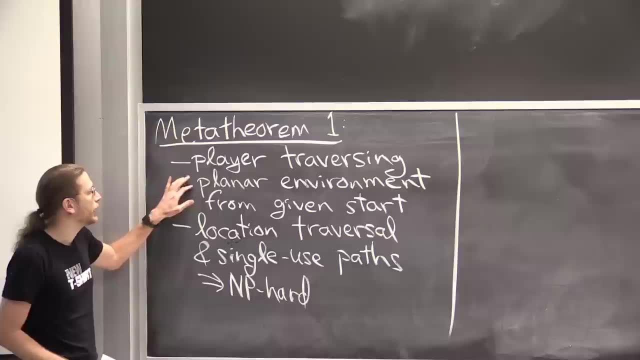 Your goal is to visit all of the locations. Once you do that, potentially you win. Or maybe there is also a target location you have to get to at the end. Question: Does planar mean you're on a plane or like a planar graph kind of environment? 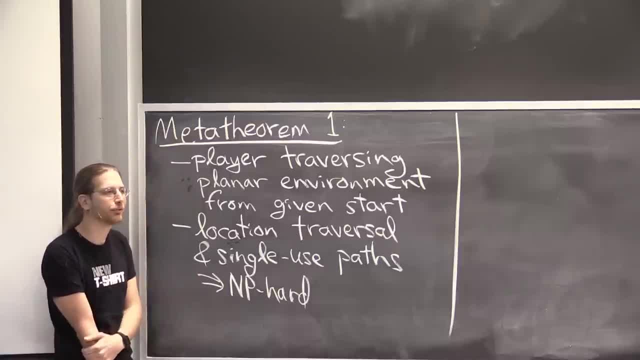 Either way, You could be sort of in a grid, You could be in a planar graph. It's vague, But the goal is two-dimensional. So the point is, we don't need, We don't need crossovers for this reduction. 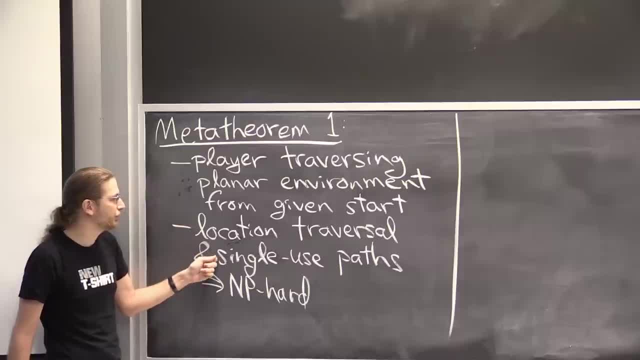 And so location traversal. you have to visit certain locations. Single-use paths: you can only use them once, So they're traversable. but once you traverse them once, they're no longer traversable. So from this you can get NP-hardness. 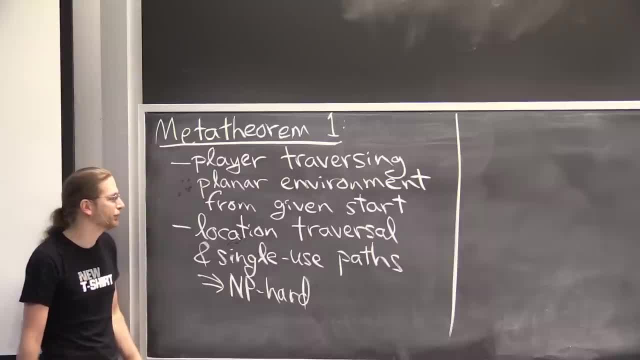 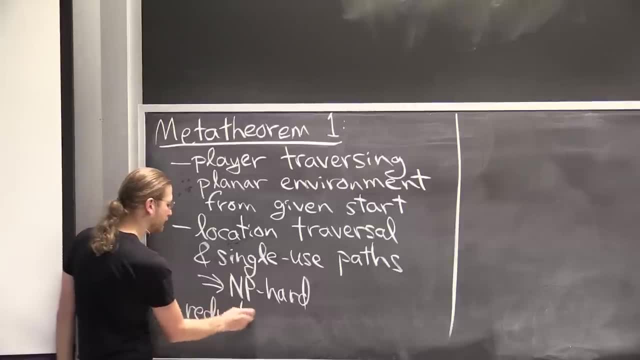 Any guesses how? What should I reduce from Hamiltonian, Hamiltonicity, Yep, All paths are single-use. No, Not all paths are single-use. although it will work here. The idea is that you've marked some paths as single-use, others. 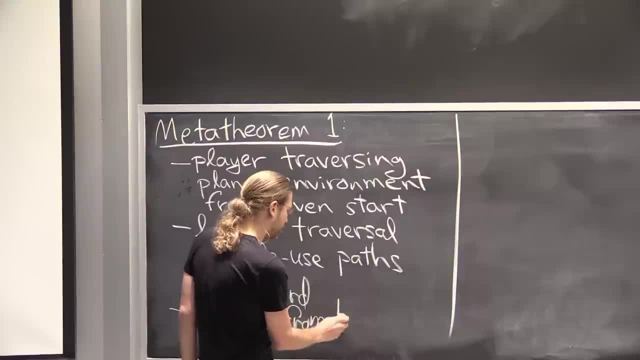 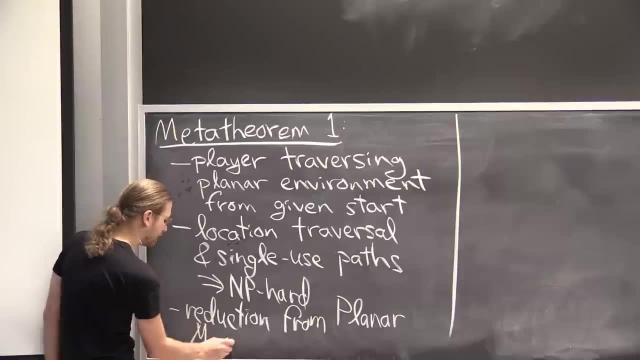 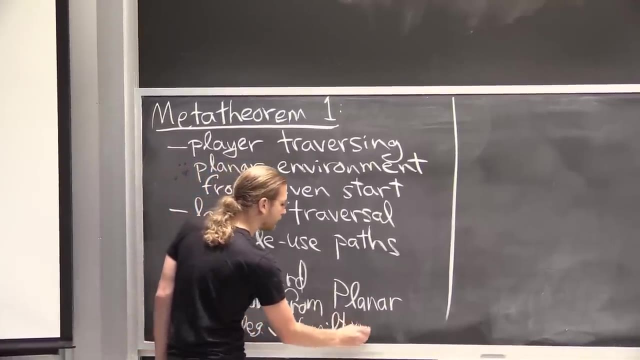 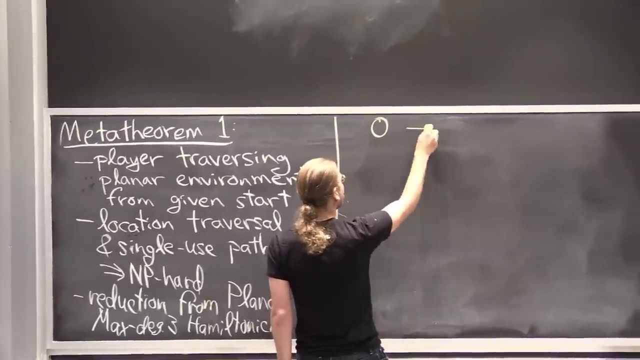 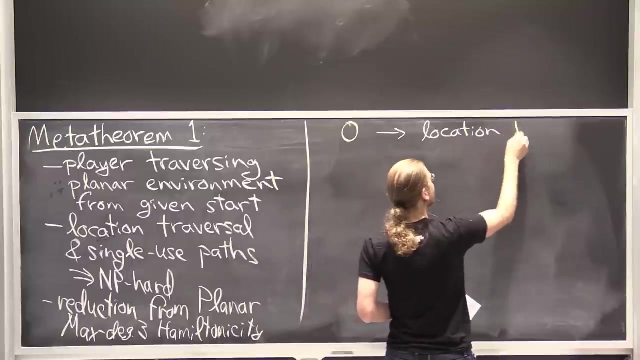 not So. reduction from planar, let's say max degree 3. Hamiltonicity. And so the idea is, whenever I have a vertex in my graph, a Hamiltonian graph, I'm going to turn that into a location that must be traversed because we 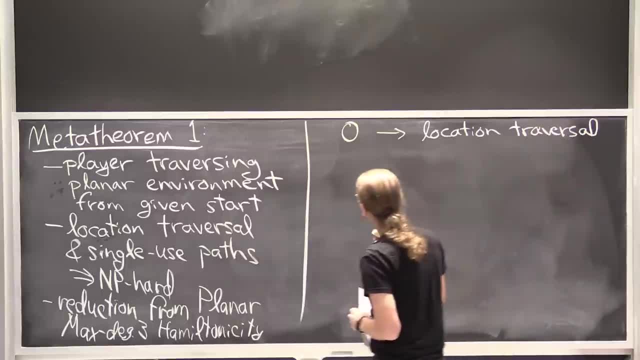 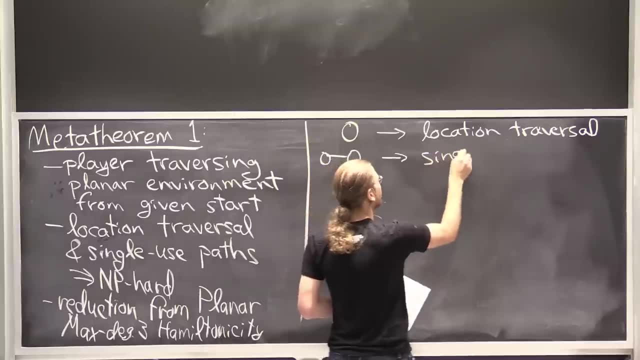 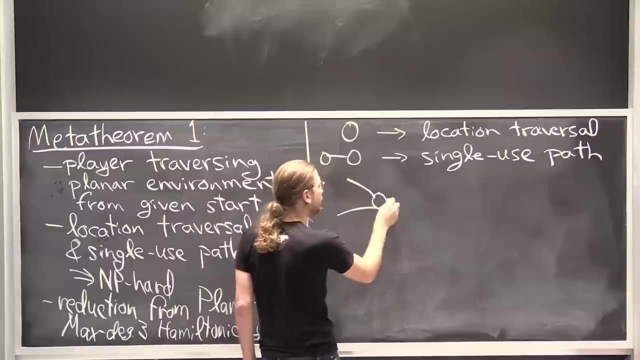 want to visit all the vertices. So there you go. That's where to put them, And whenever I have an edge, I'm going to convert that into a single-use path. And because I'm maximum degree 3, and each of these edges, 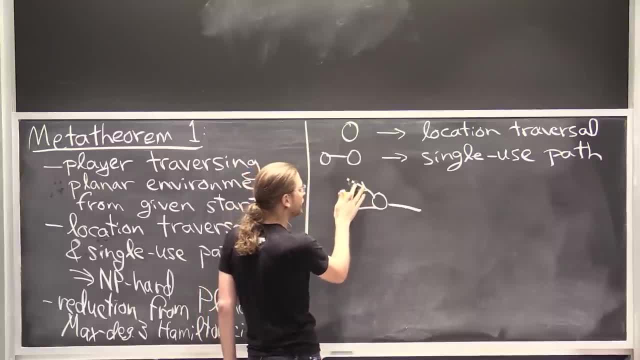 is single-use. Once I use one of the edges and it disappears, and then I use another edge and I get the treat that was in that node, And then I use another edge and that disappears. It's a really bad idea for me to use the third edge. 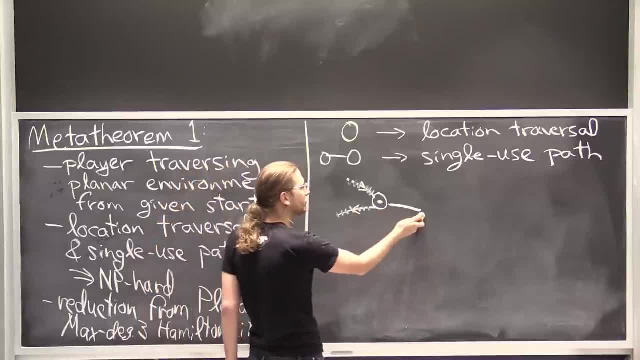 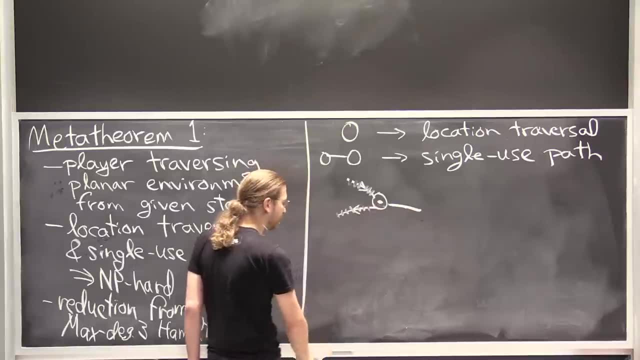 because then I'm trapped there forever. So I would have had to have already solved the puzzle. I would have had to already get all of the vertices before going here, So there was no reason to traverse that edge. Therefore, you're effectively doing a Hamiltonian path. 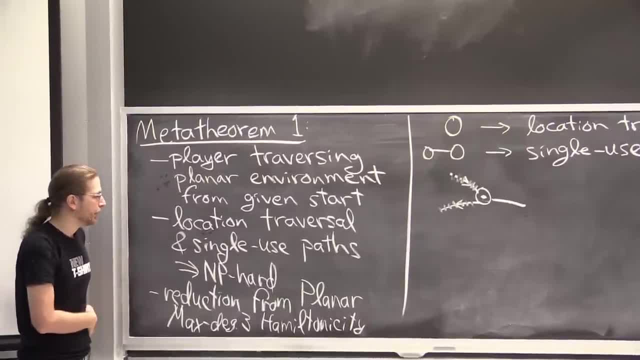 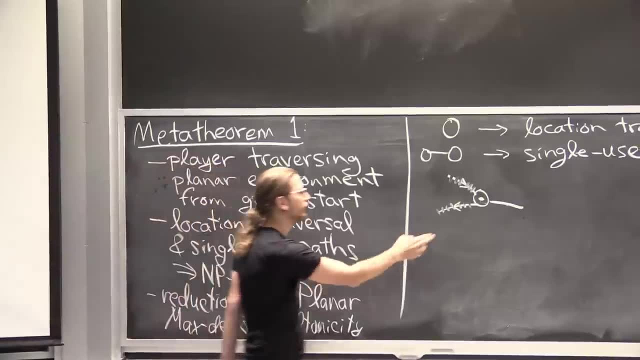 from the given start position, which we know how to reduce from Hamiltonian cycle, And because we can do planar graphs. it's a planar setup. Max degree 3 is critical for not being able to revisit a vertex. OK, we've seen a very similar proof to this. 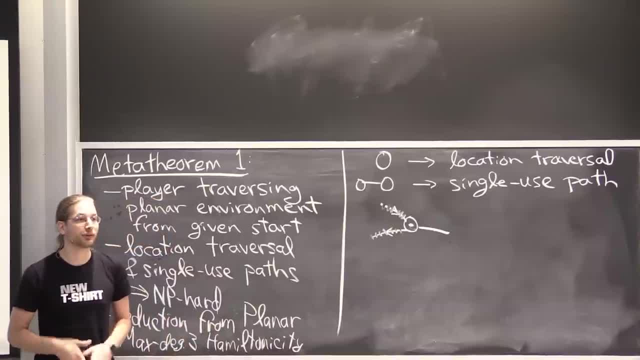 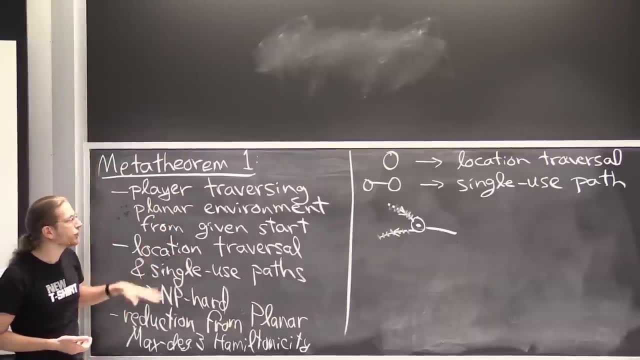 back in the Hamiltonicity lecture, But there the assumption was that there was a time limit plus collectibles, plus location traversal. This is another way to do the same kind of proof And it makes it a little easier. It's easier to be convinced that your proofs work perfectly. 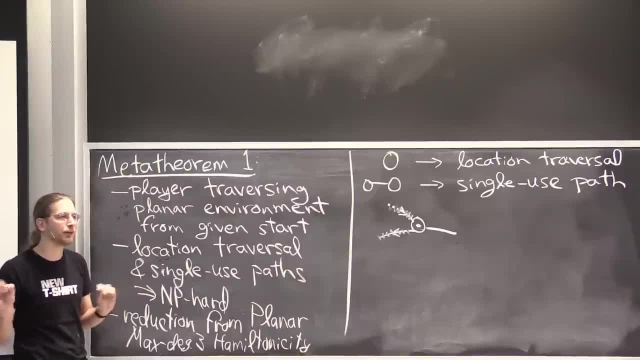 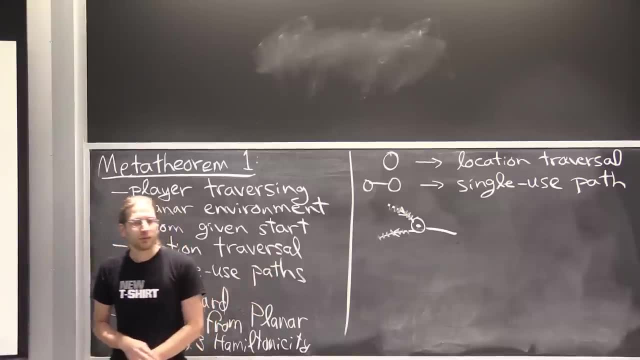 Because with time limits, you're very sensitive to timing. Every edge has to be exactly the same length. Here we're adding single use paths instead of that to force you to finish the level. The claim is also it makes the puzzles more fun. 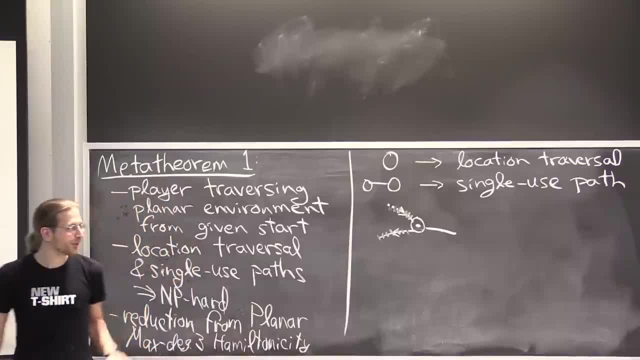 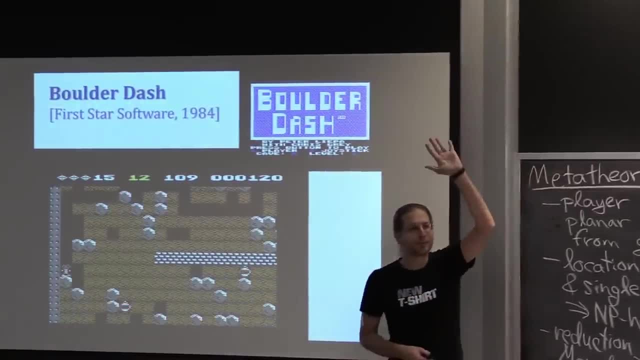 That's, of course, up to interpretation, But at the very least, using this proof, we can get a whole bunch more games that we haven't seen. So one of them is Boulder Dash. How many people have played Boulder Dash? Boulder Dash, let's say. 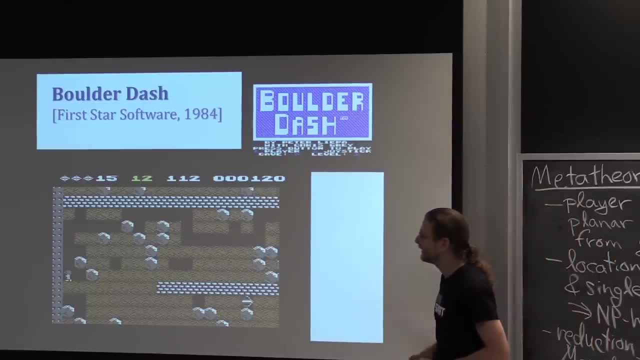 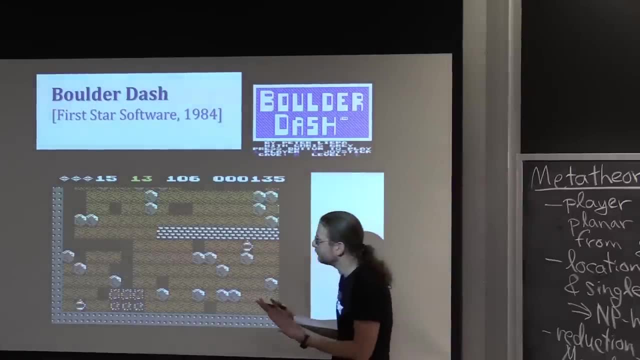 Yeah, only not very many. I used to play this in C64 days, Commodore 64.. But you are walking around these boulders. You can hold them up, But as soon as you let go they fall. And if they fall on you you die. 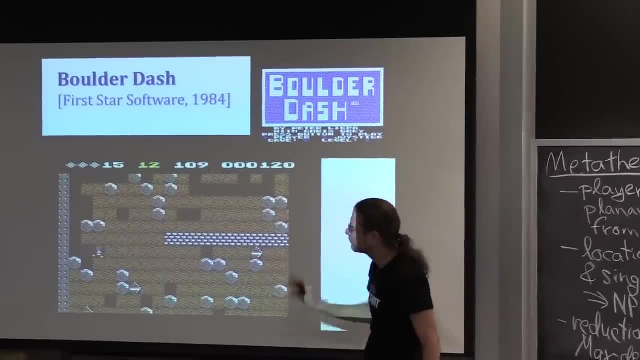 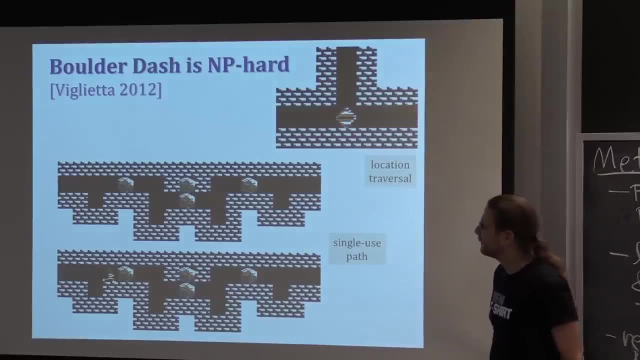 So you don't want that to happen And the goal is to collect all the diamonds roughly And then to get to a target location. There's some weird physics about how boulders fall, But basically here are the two gadgets. 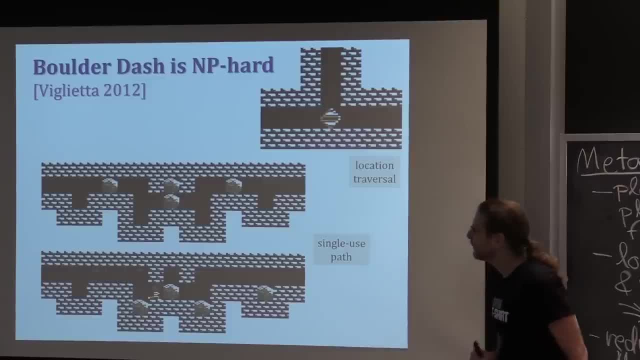 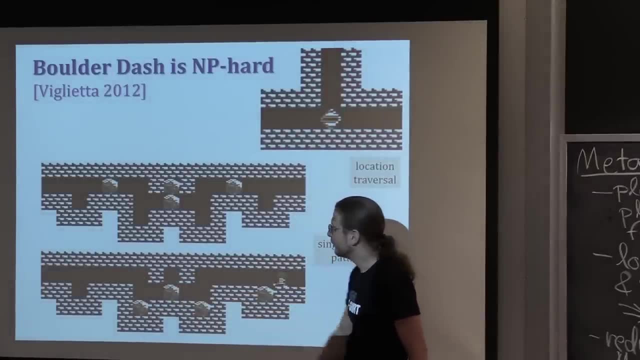 Location traversal. you just put a diamond there And then you have to get it, And then this is a single-use path. The idea is you can come from either side. push this out of the way. The boulder is then in the way. 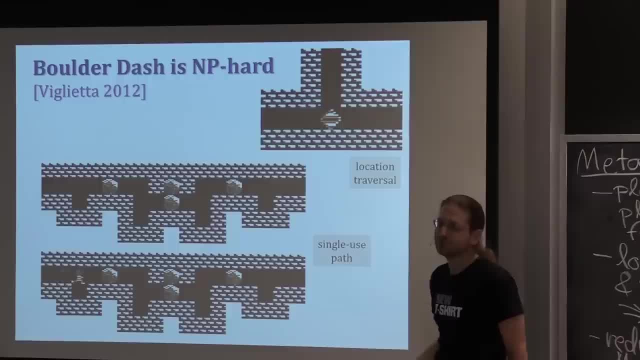 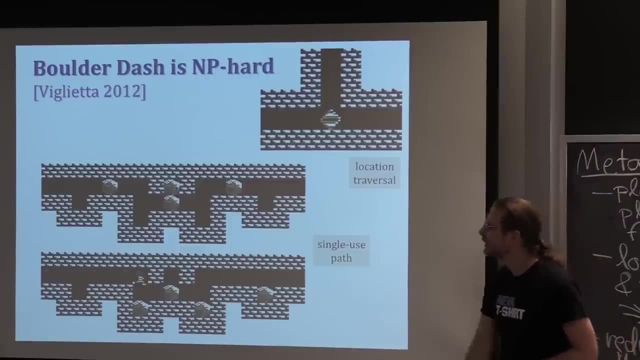 So if you then tried to traverse it, you can't turn it around the corner, So you get stuck. So once you have those two gadgets, you get an NP-hardness proof. So Boulder Dash is NP-hard. Lode Runner. How many people have played Lode Runner? 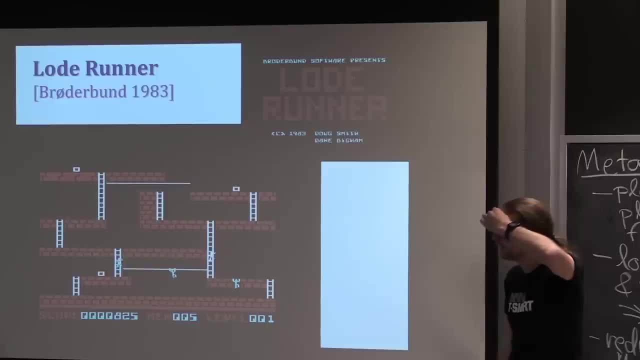 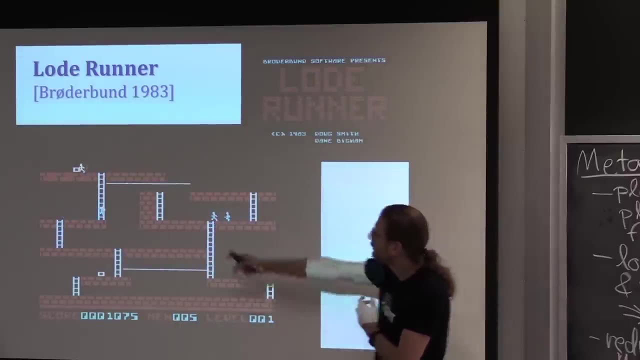 A few more. I used to play these And I don't know, It was some, I think, Apple IIe days or something, But I think, well, it was originally C64 again. So you have this guy who walks around. 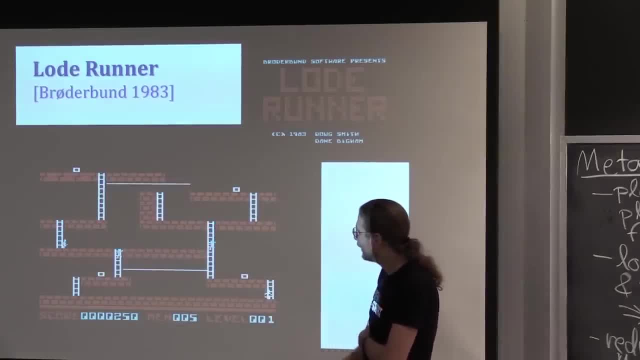 has to collect all the parts again, these things- And the fun thing about Lode Runner is you can dig a hole And then the monsters fall in. They'll drop their diamond- if they have one, And they might be able to climb back out. 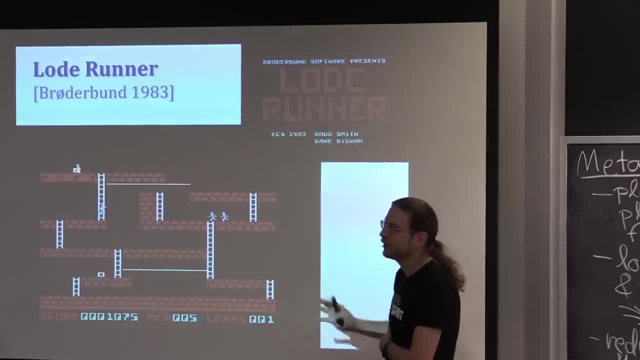 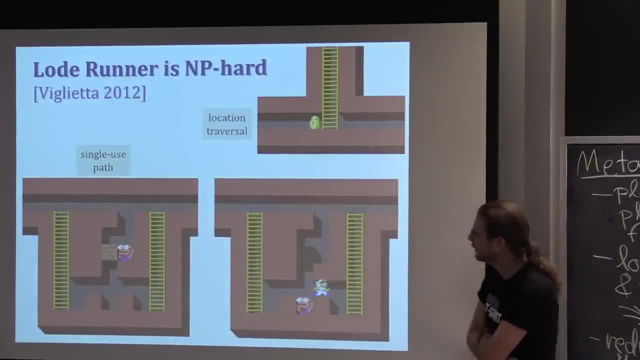 Eventually that square will refill, So it's a timed thing, And so, based on that kind of physics, we can build the two gadgets Again. You put gold wherever you want to make the thing, And this is a single traversal gadget. 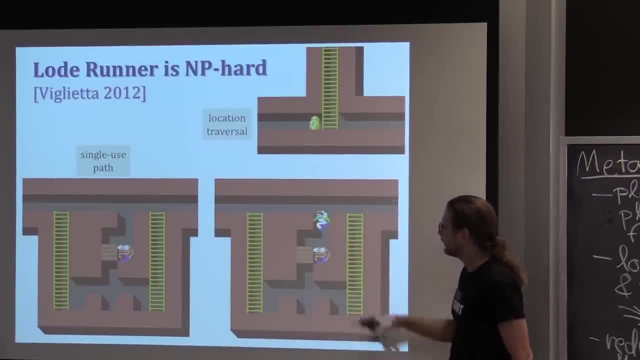 This is after it's been traversed, once You get stuck in the hole. But if there's a monster there, you can actually stand on it. dig the hole, let the guy fall. This will regenerate. This guy's stuck. But now you cannot traverse this thing. 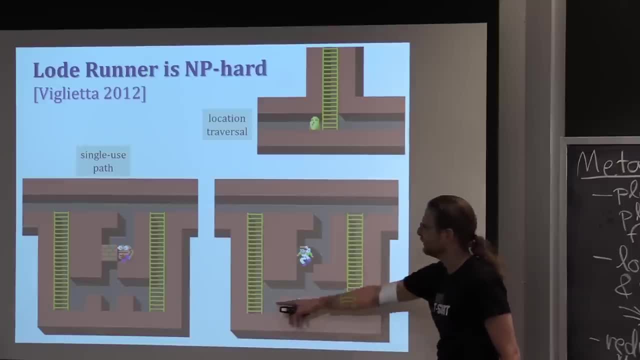 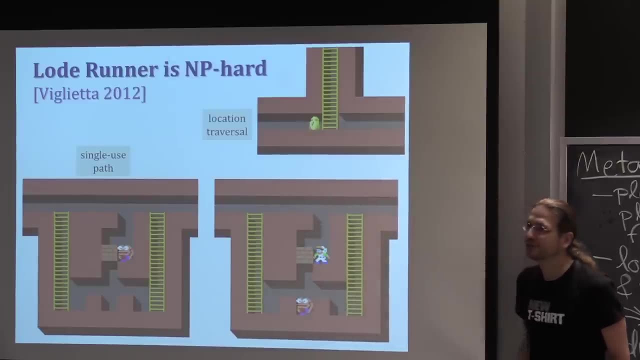 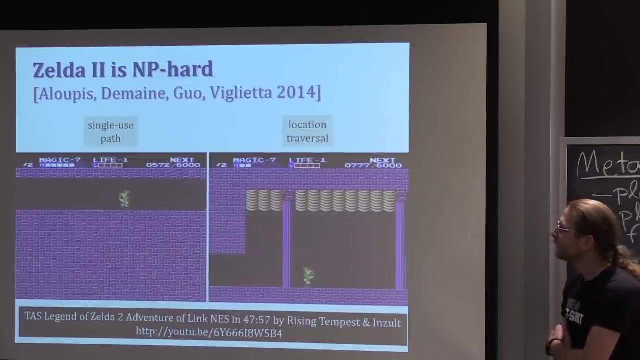 There's no jumping in this game, So you can't jump over there. You have to get to the other side by falling, And that's only possible in the initial configuration. So Load runner's NP-hard Questions Cool. Also, Legend of Zelda II- Adventures of Link is NP-hard. 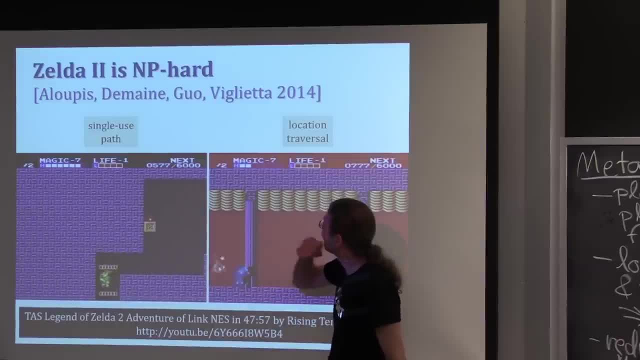 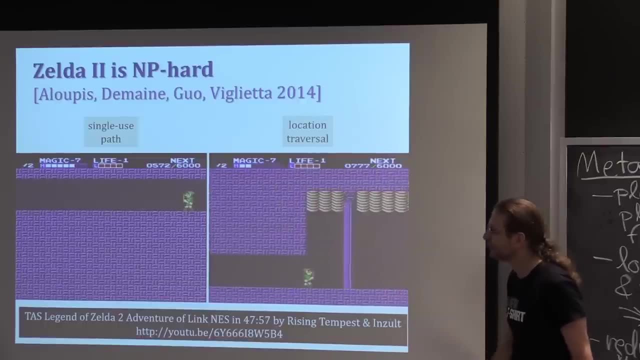 On the one hand, we have single use paths illustrated on the left, and location traversal We're going to do by keys. If you get enough keys, you can open enough doors. At the end of the puzzle, there's going to be a whole bunch of doors. 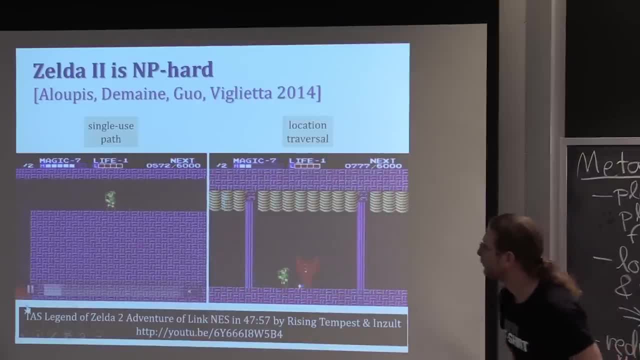 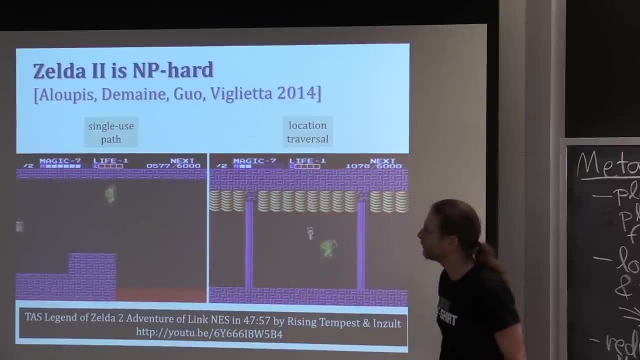 Let me get this one going again For single traversal paths. they're actually these bridges that disappear after you traverse them, So you can do some amount of jumping, But if you make it really long you will be prevented from re-traversing that path. 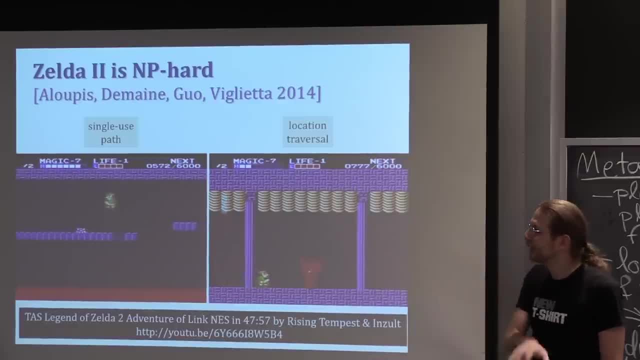 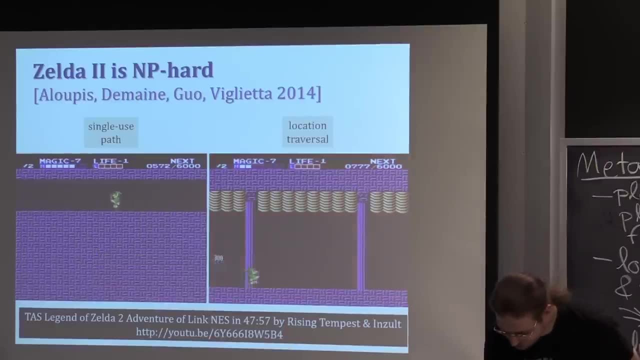 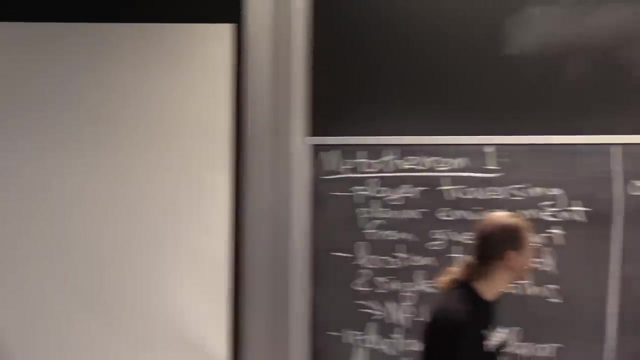 So we're going to put a key at each vertex And then at some finishing location we'll have n doors, one for each vertex, And that should do Zelda II. OK, So that is Meta Theorem 1.. OK, So I want to tell you about a slight variation. 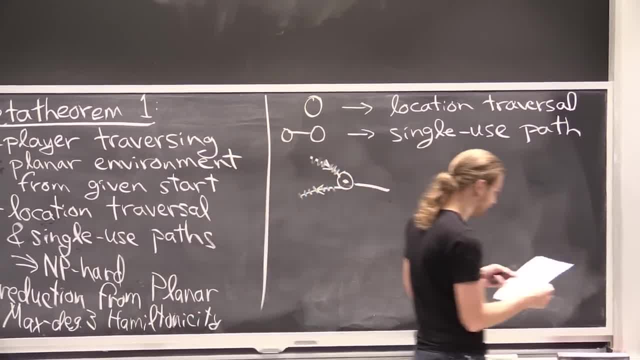 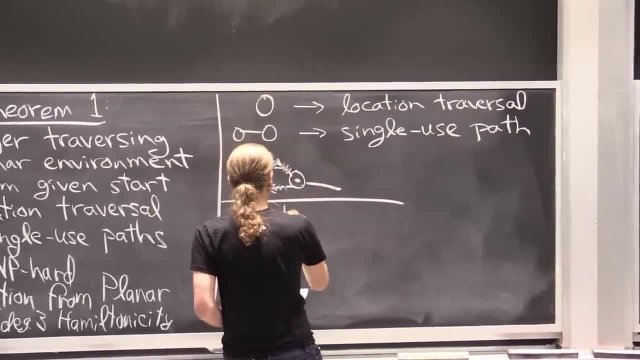 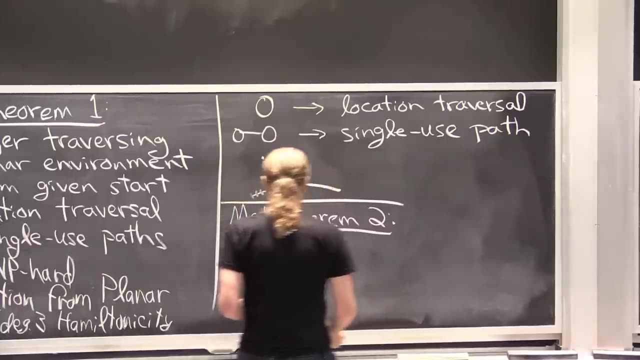 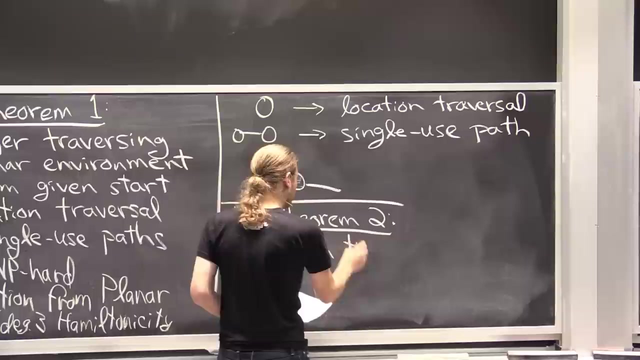 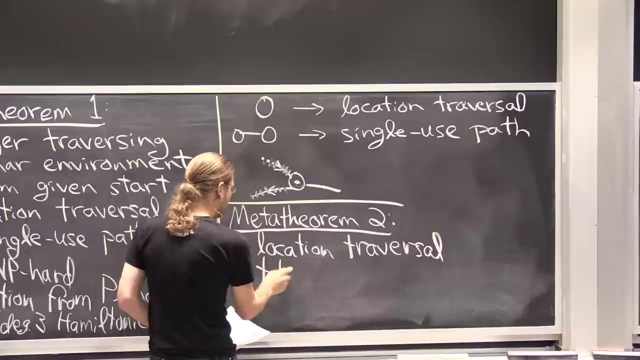 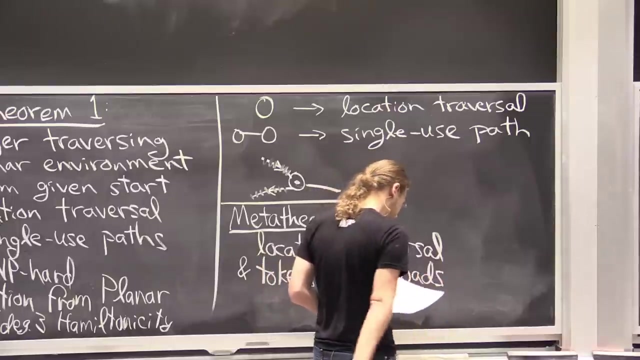 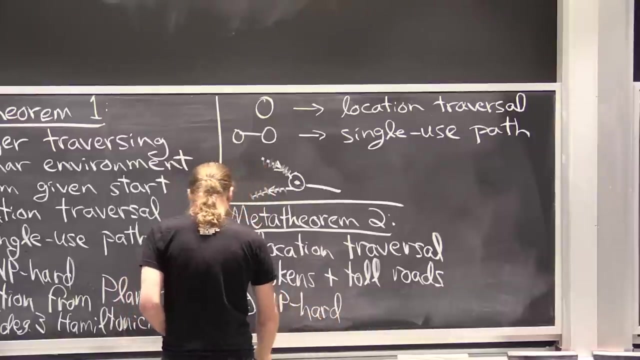 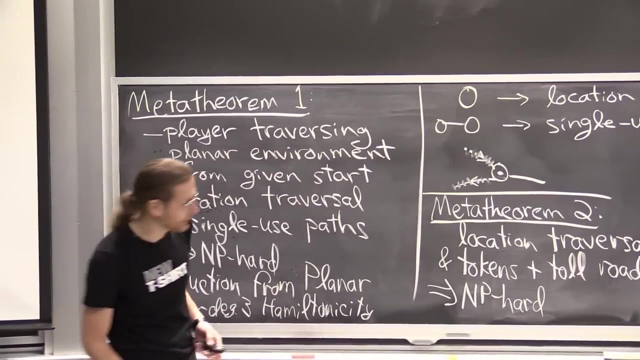 on this Meta Theorem and then another result based on it. So Meta Theorem 2 is the same kind of setup, But it's a different way to do it, So slightly different. Yeah, I'll just keep a little bit of sight. 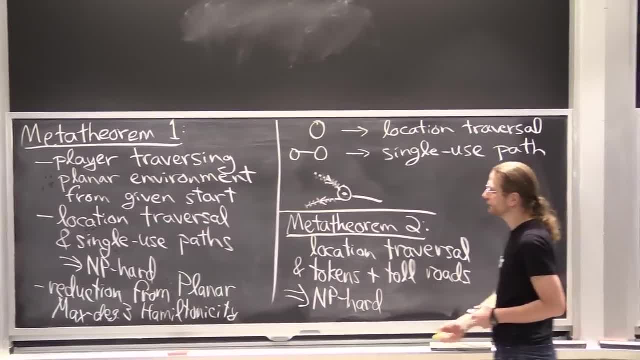 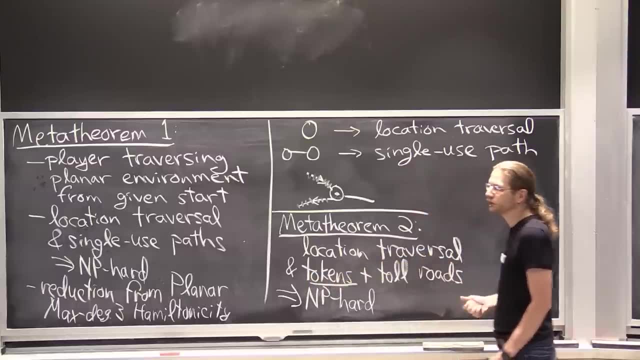 OK, Yeah, bit of suspense about why we care about this. Instead of single use paths, suppose that you could build tokens, which are things you can pick up, And for this reduction, let's say you can only pick up one at a time, though it won't matter. 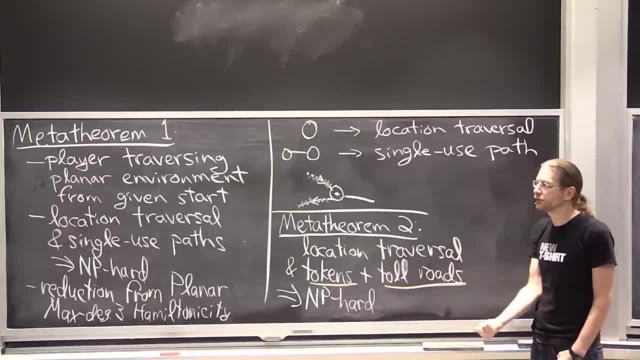 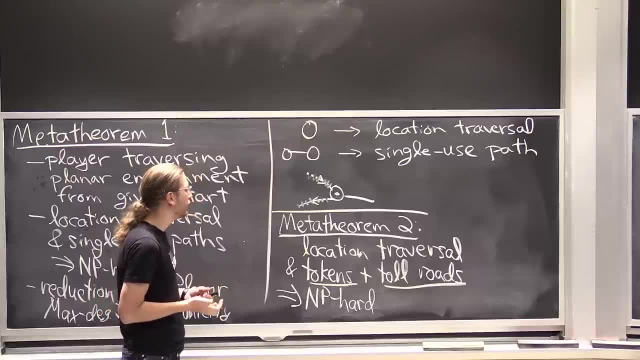 And toll roads where you have to pay with a token in order to traverse the edge. This, essentially, can be used to simulate a single use path, but it's slightly different perspective In that you can visit an edge if you. well, what we're going to imagine doing? 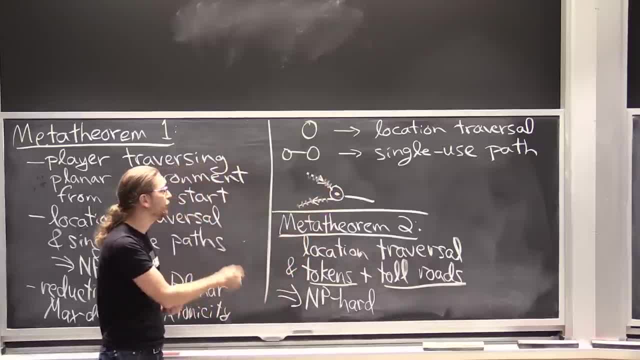 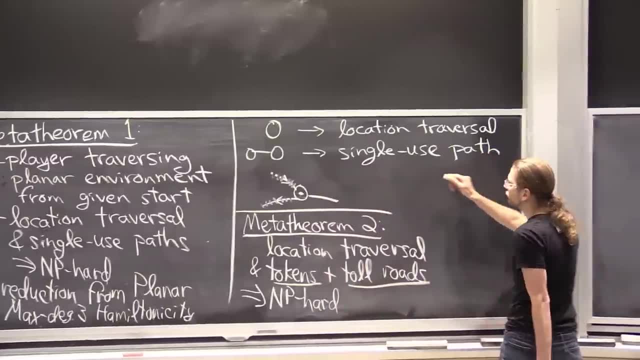 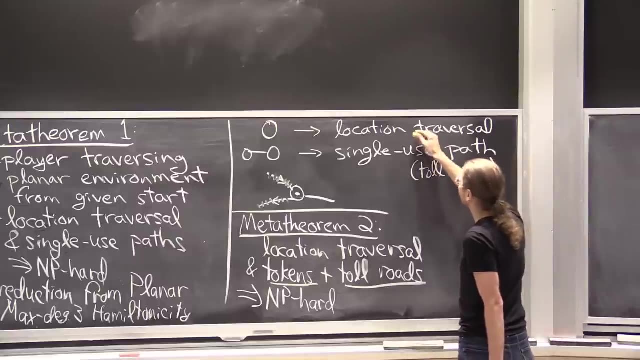 is putting tokens at the vertices, but just one at each vertex. When you pick up that token, you can then traverse one of the incident edges. So, again, every edge will become a toll road And every vertex will become a location traversal point. 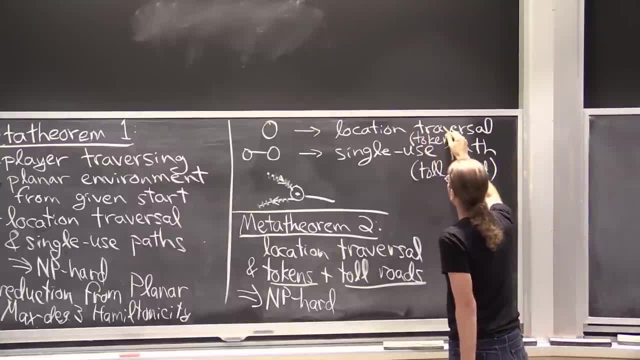 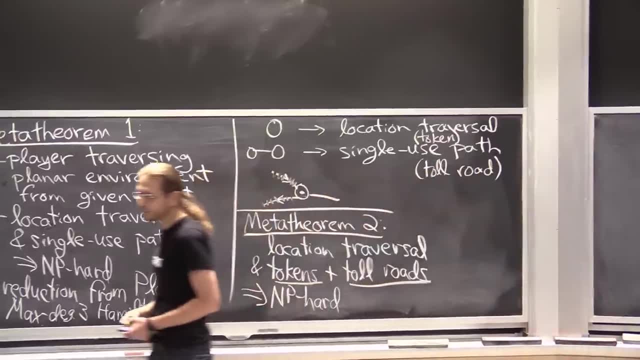 that has to be traversed And it will have one token, And so you can use the same kind of proof. It's just so, It's a different perspective on the same kind of thing, And we can use this to prove that Pac-Man is NP-hard. 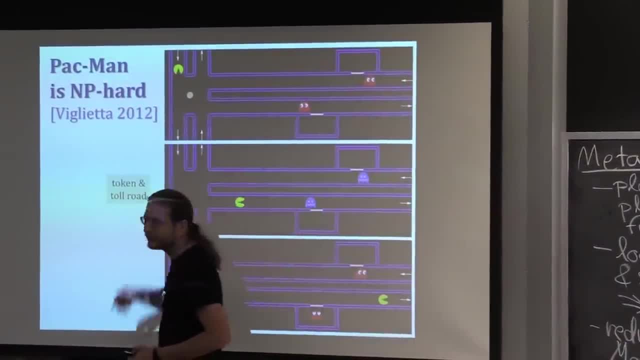 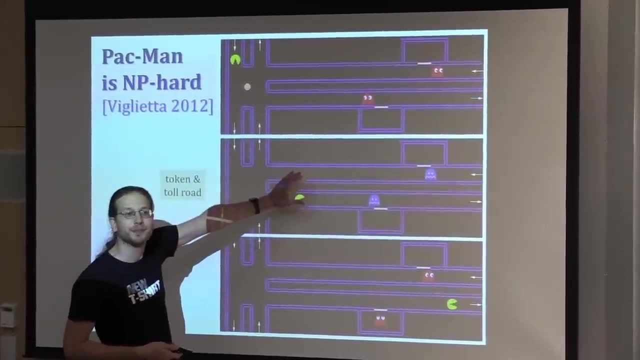 This is the motivation. So again, you have to get all the dots in Pac-Man, So you in particular have to get that one. When you get that one, this edge becomes traversable. So this is a somewhat generalized version of Tetris. 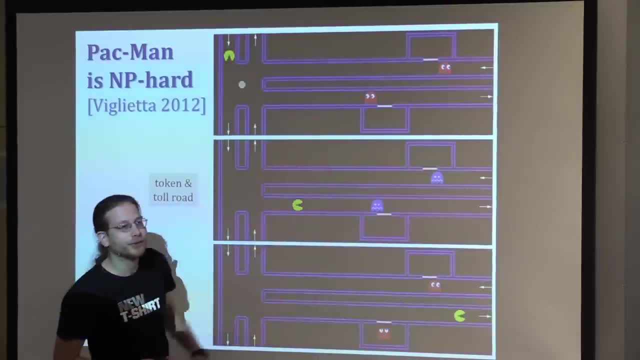 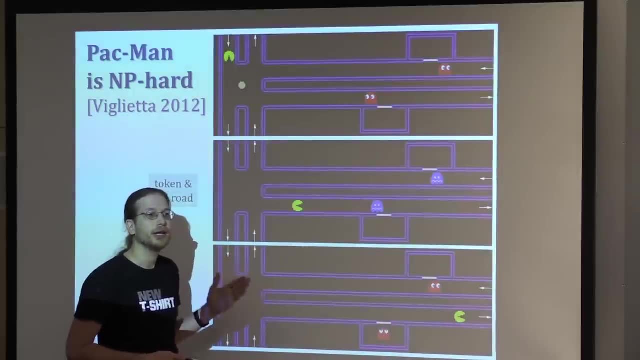 You have lots of houses for the ghosts, Lots of ghosts. obviously, The algorithms that the ghosts follow doesn't matter too much. The only constraint is that ghosts change direction if, and only if, the state changes Like you turn them into. I forget. 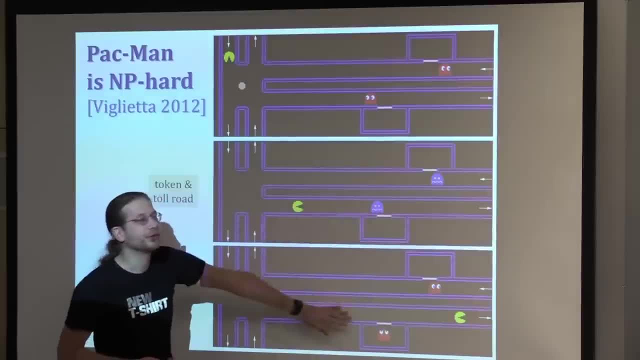 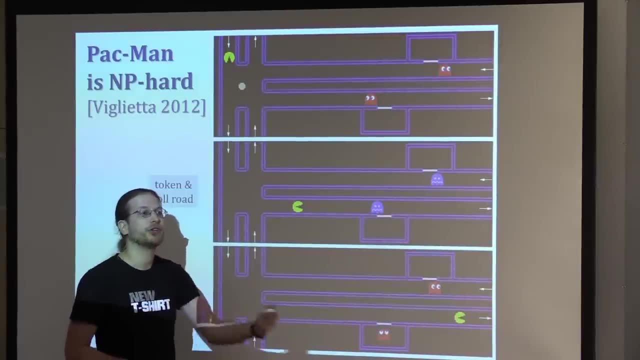 the names of all the modes, but you turn them into the blue mode or they turn back, Then they will switch direction in their tunnel And that is the only setting in which ghosts will actually change, will reverse direction, double back on themselves. 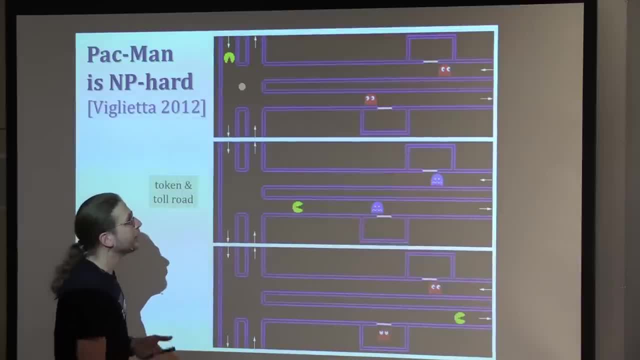 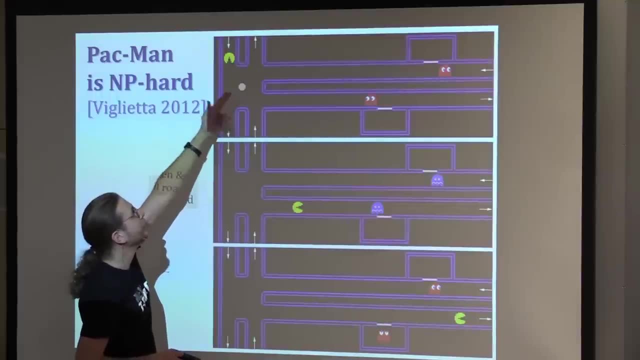 They never double back. otherwise, And given that setup, if we make these edges really long, we can make sure that the ghosts always stay within their edge, Because you're basically alternating between switching the state, turning the directions of the ghosts traversing an edge, and then doing it again and again. So the ghosts always sort of go back and forth. If you happen to capture one, it doesn't really change its location much because it just goes back to the house, But you obviously need one of these in your possession. You end up using the token right away. 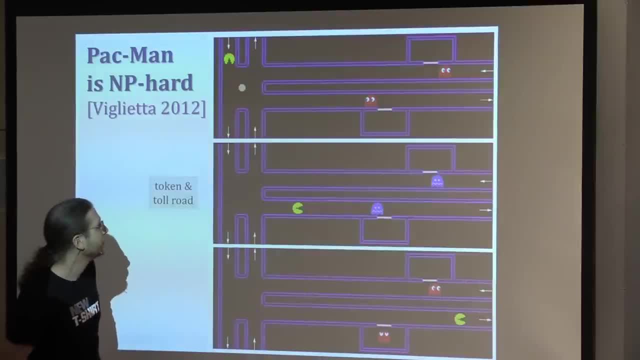 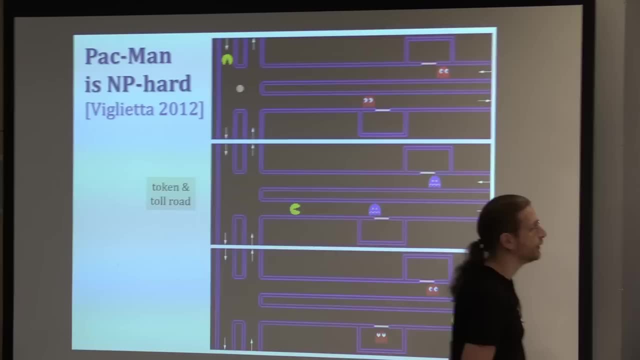 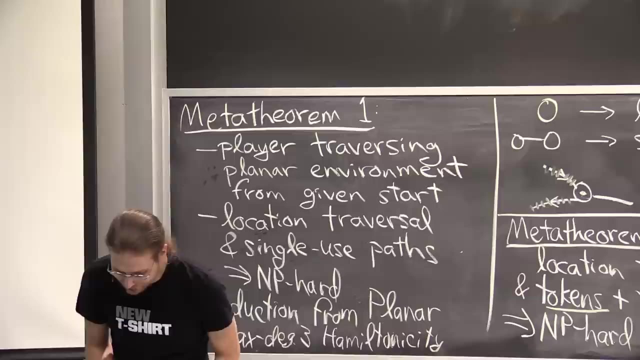 to traverse one of the incident edges so you can actually get across, But it's long enough. so by the time you cross over, the ghosts have reset. So that is metatheorem two applied to PACMEM. in case you were wondering, This is, I think, quite clever to get these things to work out. 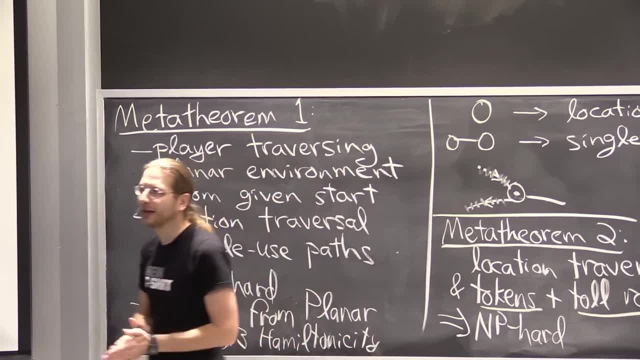 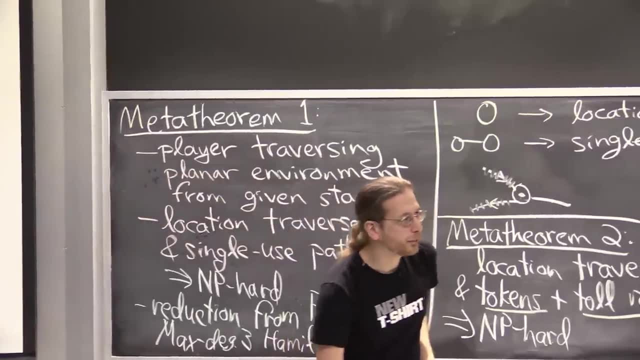 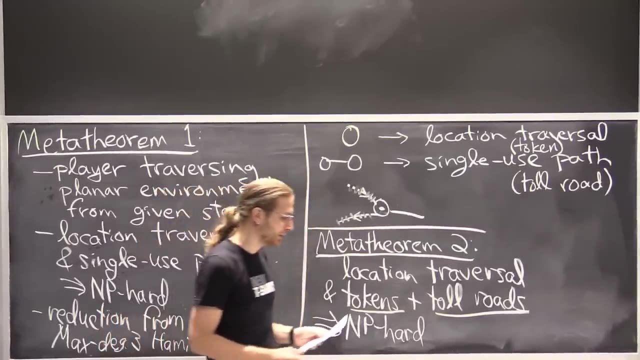 So NP-hardness, we're used to that. The next metatheorems are about PSPACE-hardness And before I get there, I need to tell you a little bit about some basic PSPACE-hard problems. like we have SAT and Hamiltonicity for everything. 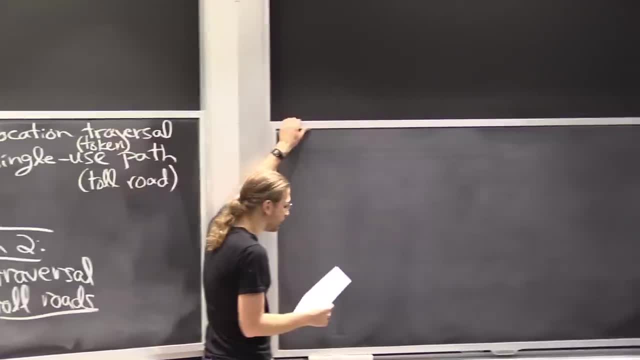 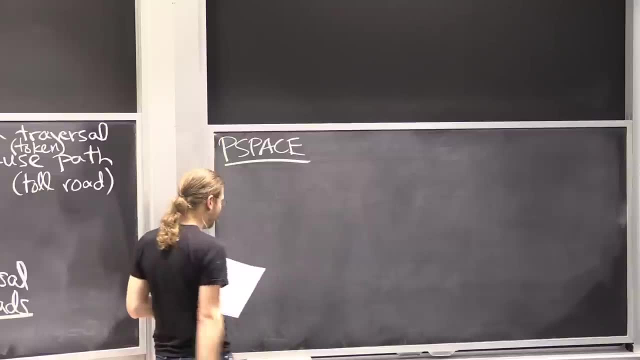 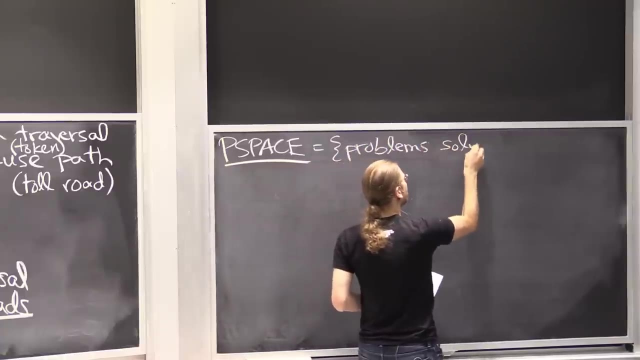 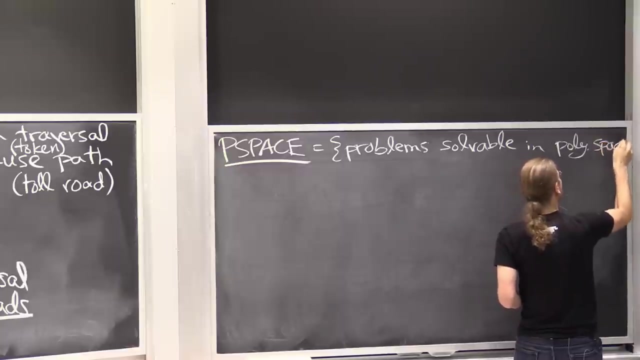 OK, So for NP-hardness, for PSPACE-hardness, there are a couple of natural problems. First, let me remind you, because it was lecture one, that I defined PSPACE. These are all problems solvable in polynomial space. So we're measuring space instead of time. 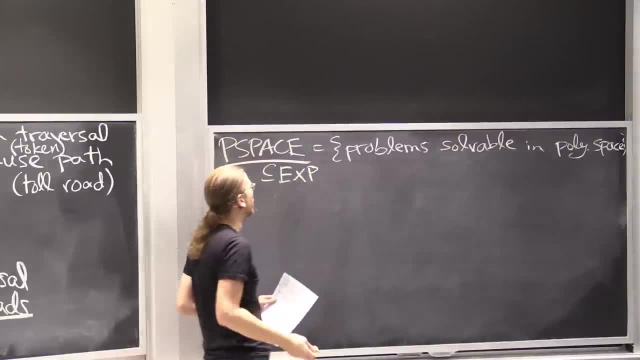 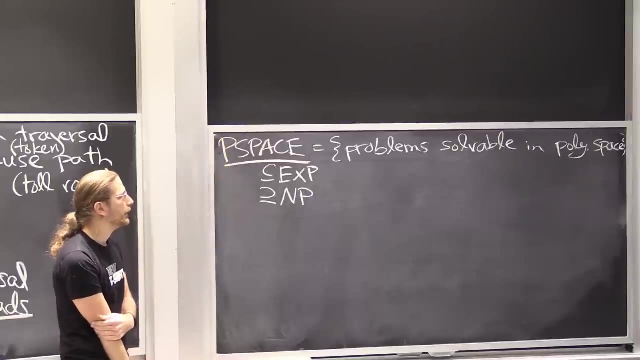 This is contained in exponential space. It's called time because there are at most exponentially many states of a polynomial space machine And it contains NP In particular. every NP problem can be simulated on a PSPACE computer just by trying all possible options for the guess. 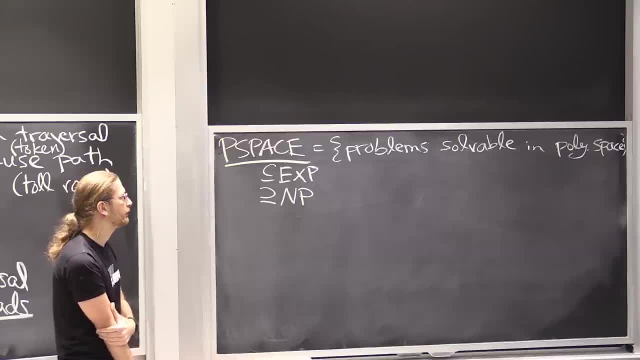 but backtracking and throwing away the information from the other guess paths and just keeping one bit of state, which is: did I find a yes solution yet? So you can turn any NP machine into a PSPACE machine. So it's somewhere in between. 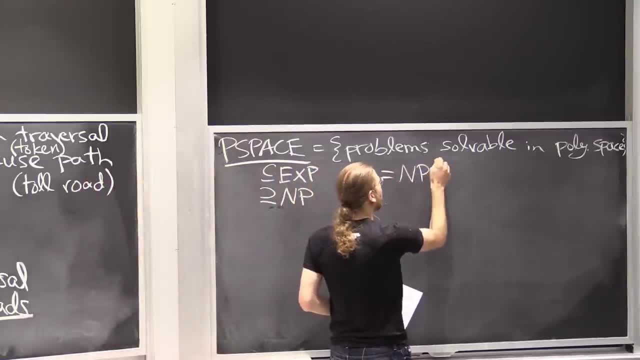 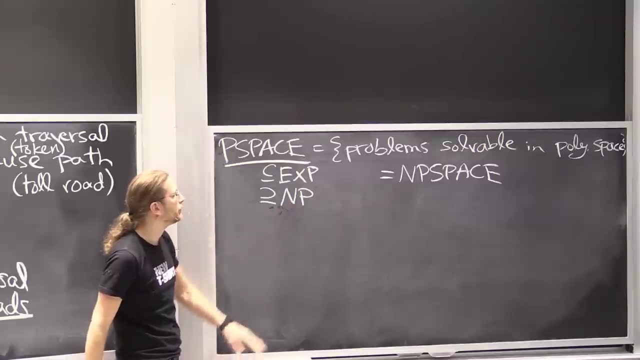 The other fun fact is that it equals non-deterministic polynomial space, so non-deterministic in the sense of NP. If you add guessing to a PSPACE machine, that doesn't help you. You can always simulate it with a deterministic machine. 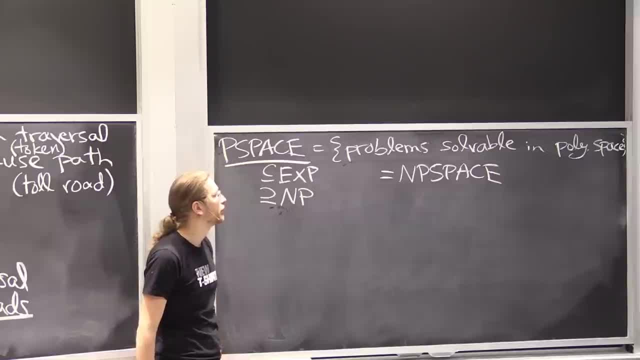 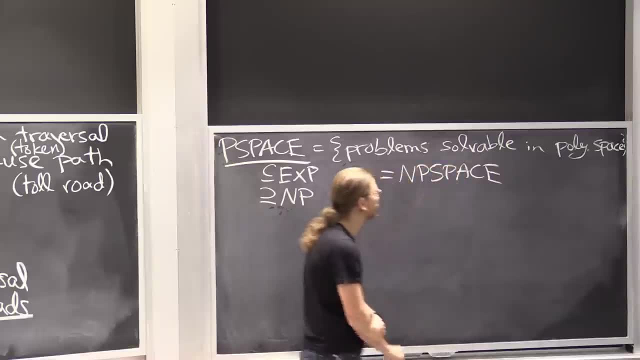 at most blowing up the space by a square. So if you had s space before, you have s squared space after, And that is closed under a polynomial space. OK, Polynomials are closed under squaring. So this is especially useful for showing that a lot of games 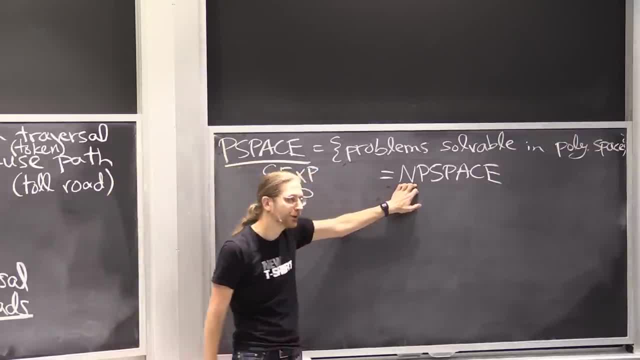 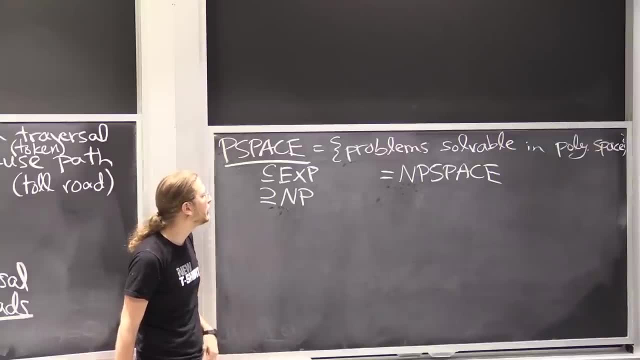 are in PSPACE, It's a lot easier usually to give a non-deterministic polynomial space algorithm. You have the freedom to guess whenever you like, just like with proving containment in NP And if you prove containment in NP space. 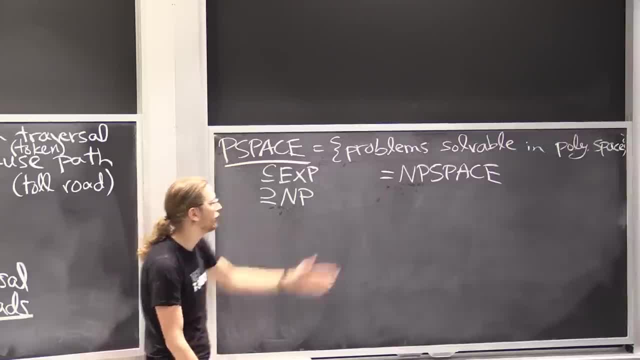 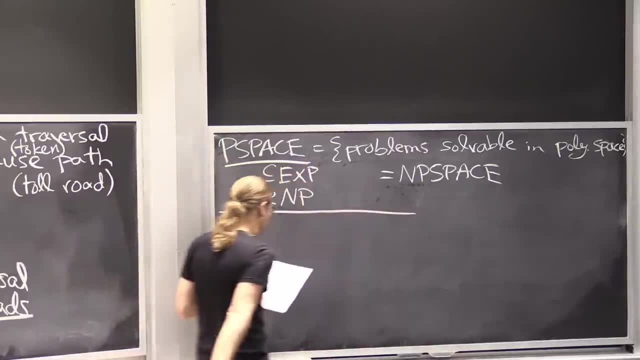 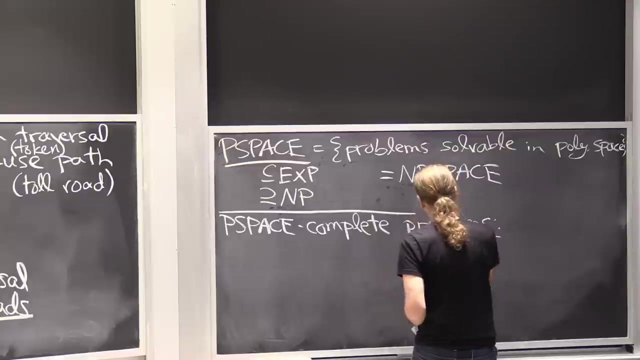 you are also proving containment in PSPACE. This is called Savage's theorem. So that was just some recall from lecture one. And now let's talk about some sort of base problems, PSPACE, complete problems that we can reduce from. I would say the most obvious one is: 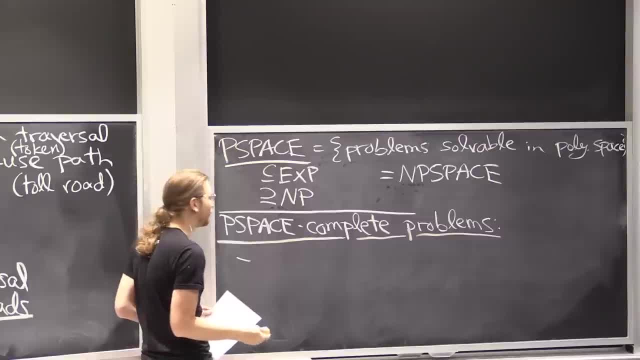 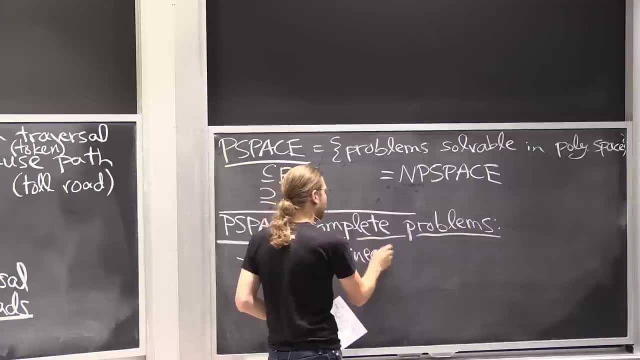 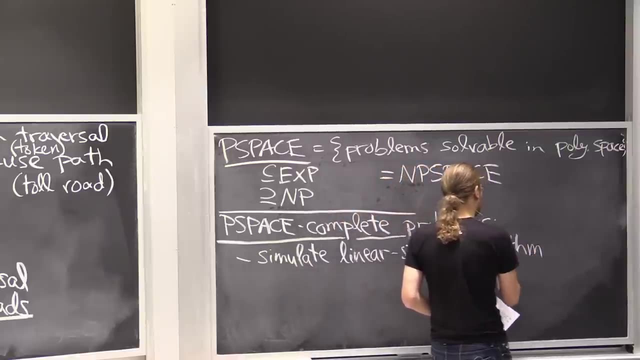 to simulate a polynomial space algorithm. You can relax it slightly. It's a little bit more complicated, But you can do it OK, All right, Slightly to say, simulate a linear space algorithm, or Turing machine if you prefer that. 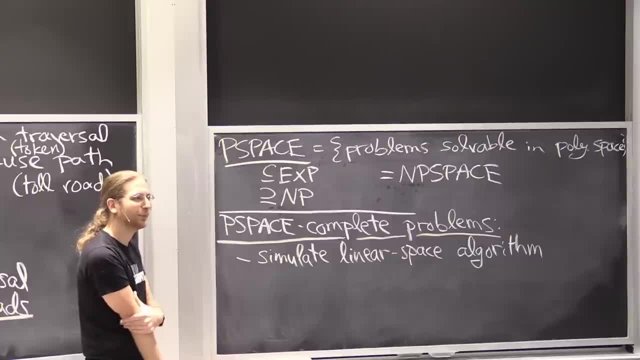 Of course, if you are PSPACE complete, if you can simulate all algorithms that run in polynomial space, And there are some proofs that work that way. Take some simple model of a computer like Turing machine, typically, like you're reading and writing. 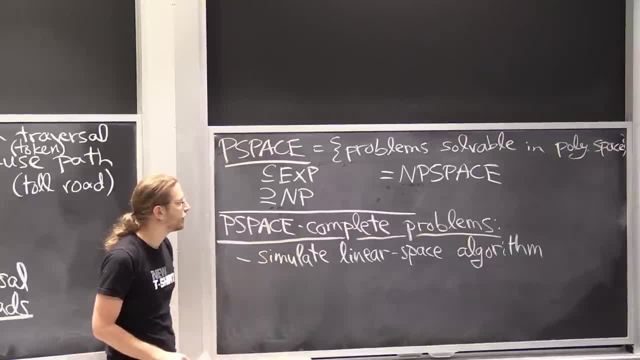 cells on a tape and you're doing whatever you can do in that linear amount of space and just simulate those transitions, one at a time, But it's usually pretty tedious to do that. I don't think we will see any proofs directly of simulating a Turing machine. 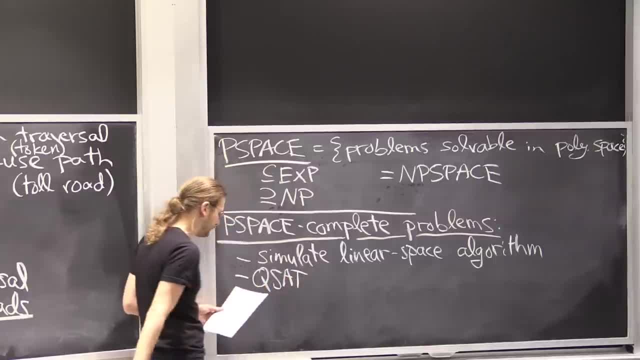 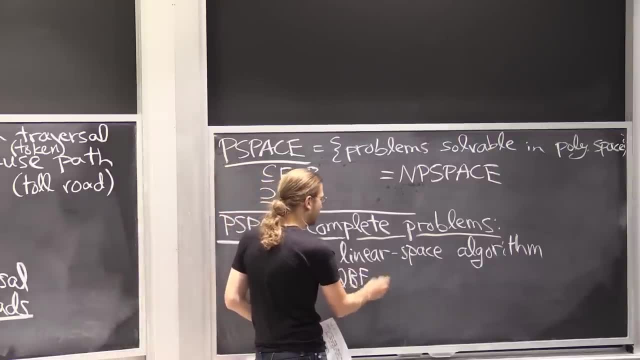 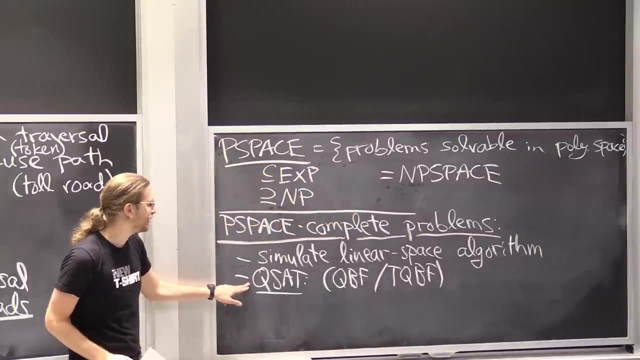 Usually a simpler way to go is a problem called QSAT. It's actually usually called QBF and sometimes called TQBF and occasionally called QSAT, But I'm growing on the name QSAT because we can specify things. It's consistent with our naming terminology. 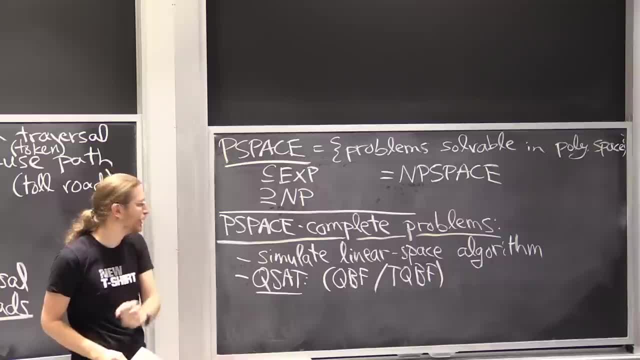 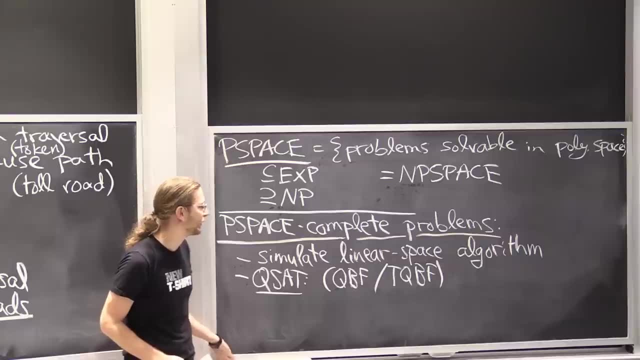 We can say Q3SAT, We can say Q1 and 3SAT, We can say planar QSAT, Whereas QBF- usually people mean Q3SAT, I guess. But this is a little more explicit what kind of SAT we want. 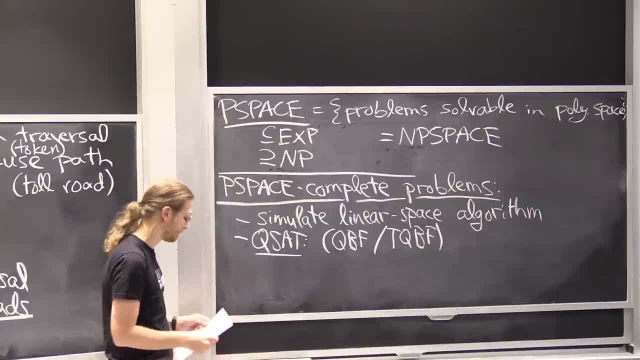 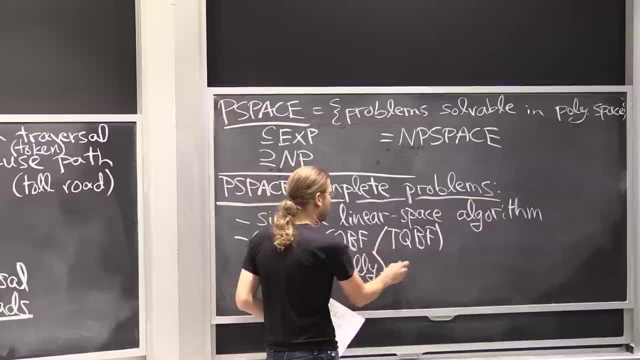 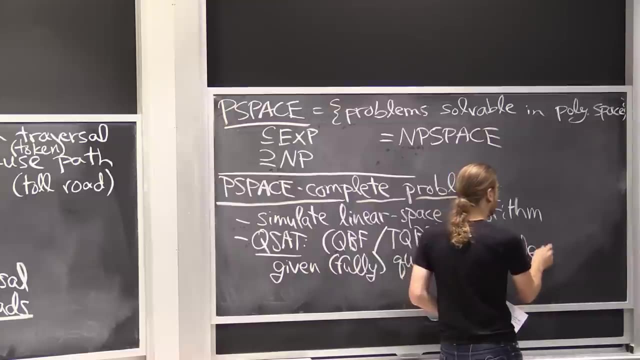 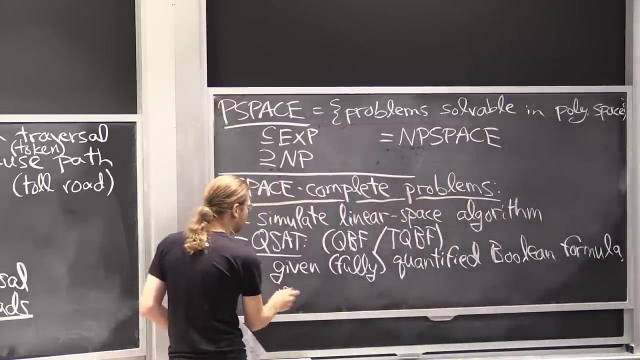 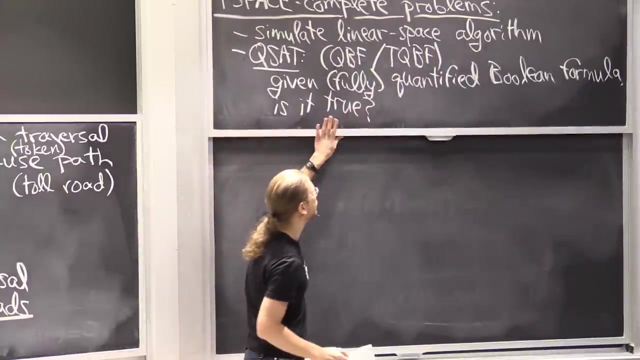 So we're adding the letter Q, which is quantified. So the general problem is: given a fully quantified Boolean formula, You want to know decide, is it true? That's the T in TQBF, if you prefer that term. 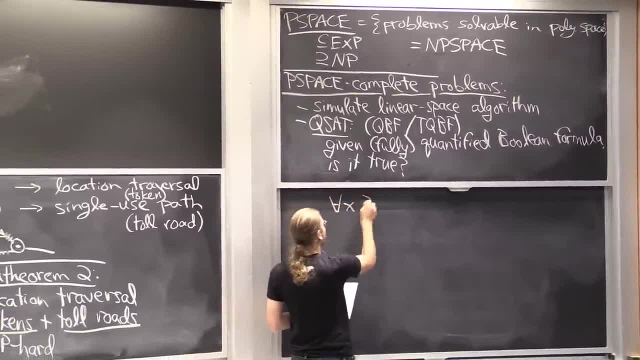 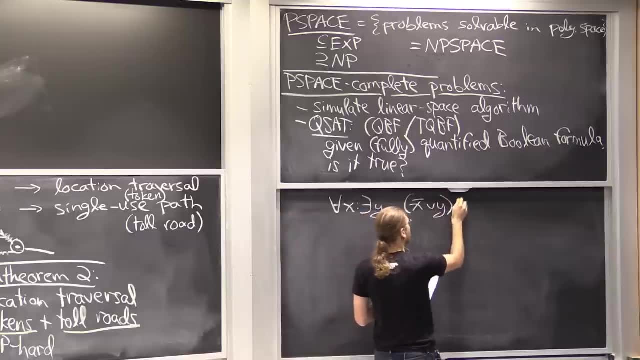 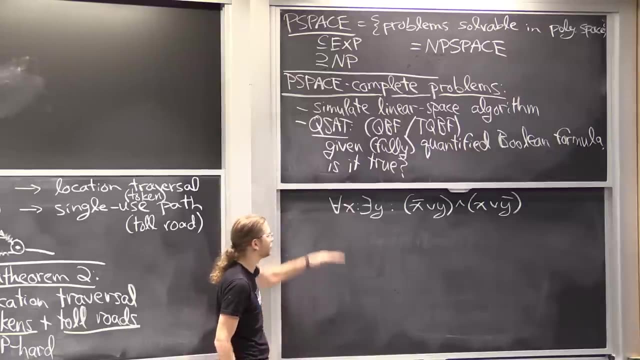 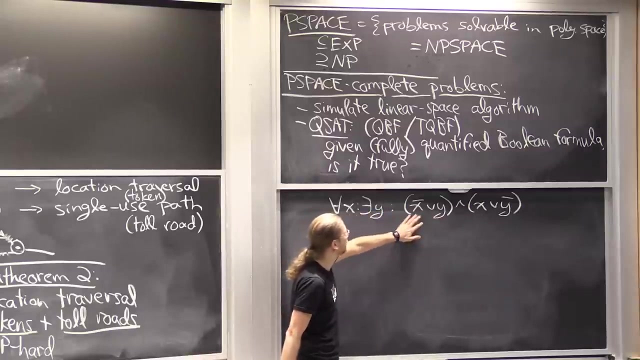 So, for example, here is a quantified formula. It took me a little thinking to come up with one that is actually true in a not quite trivial way. So this is a 2SAT formula. So in particular, you can read this as: x implies y. 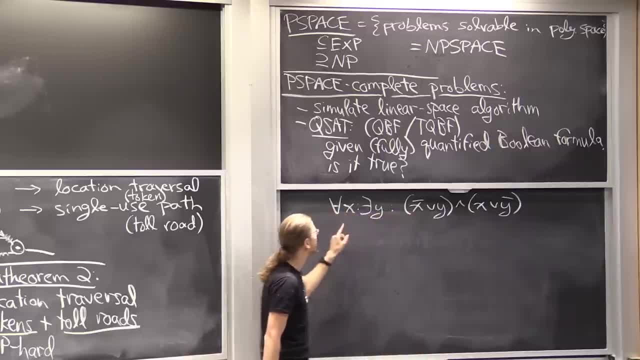 and y implies x, And we're saying for every x there is a y, such as this is satisfied And that's true. Namely, y equals x would be the correct choice, But it's not totally obvious, given that formula, that it's true. 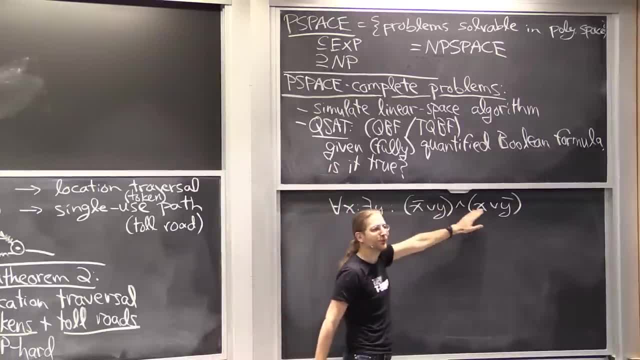 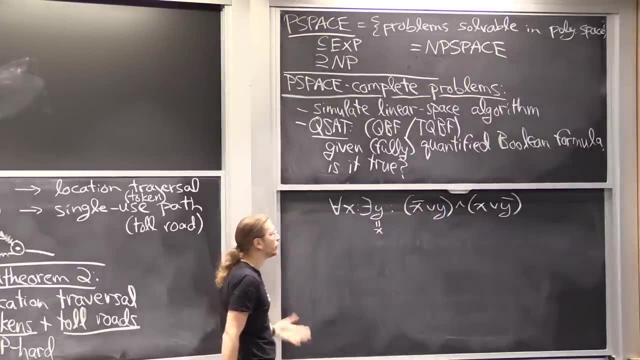 And in general, given such a formula- probably not with 2SAT in here, but with 3SAT formula- it's going to be PSPACE complete, To contrast with SAT. essentially there are a bunch of there exists at the beginning. 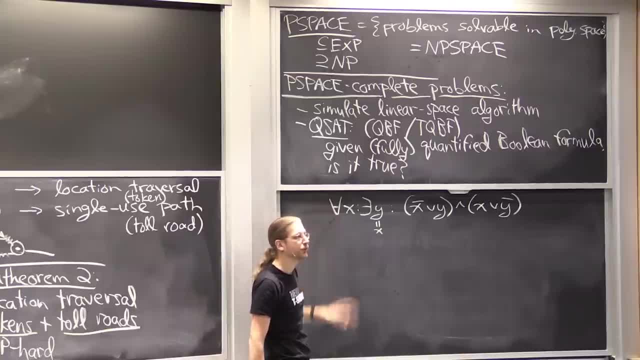 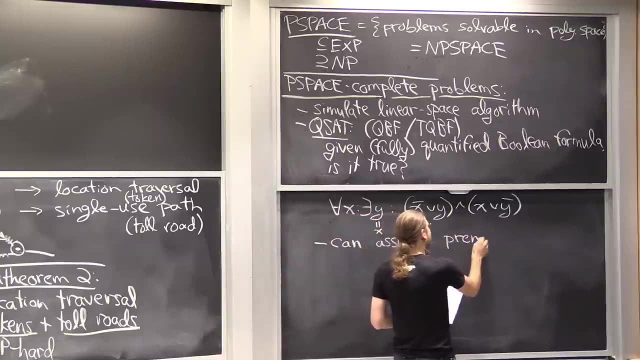 With QSAT you can have for-alls in addition to exists. That's what we're changing, And we can simplify things a little bit. We can assume pre-next form, which just means that all the quantifiers are in the beginning. 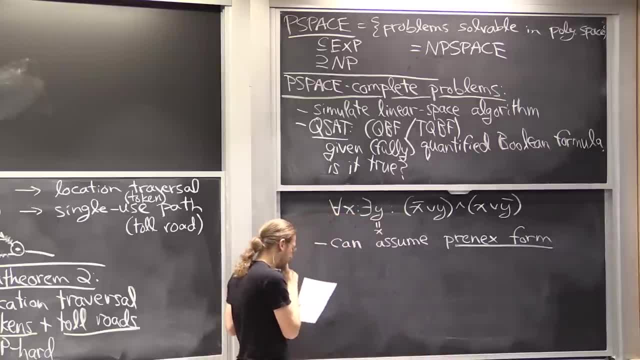 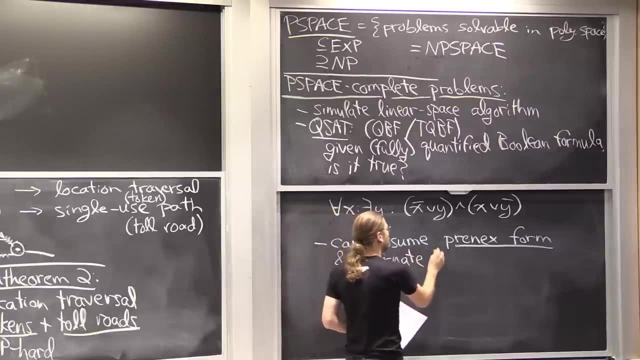 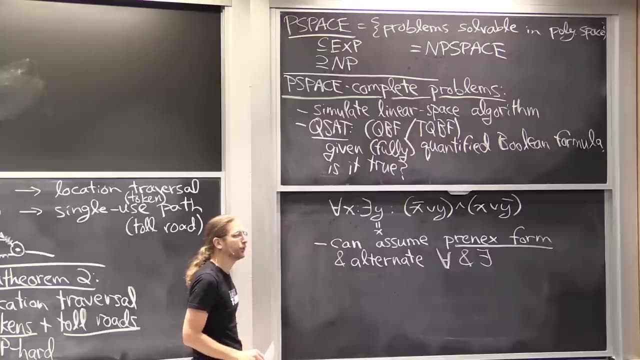 And then we have a 3SAT formula or whatever And we can assume that we alternate. The quantifiers alternate between for-all and there exists just by adding in extra dummies if we happen to use a bunch of for-alls in a row. 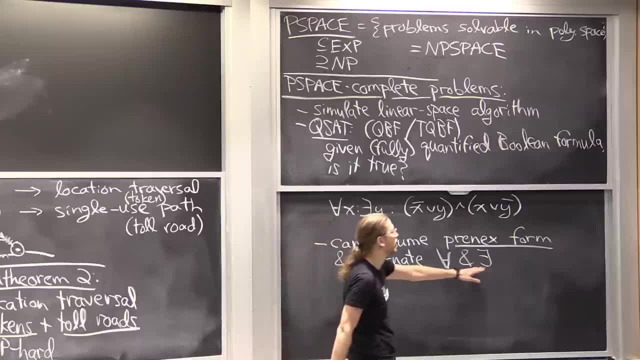 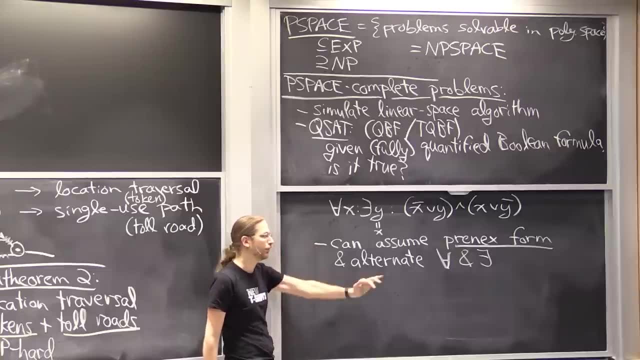 or a bunch of there exists in a row. But really the hard case This is when you have lots of both and they're interwoven. So it's not enough to look at formulas that have a bunch of for-alls and then a bunch of exists. 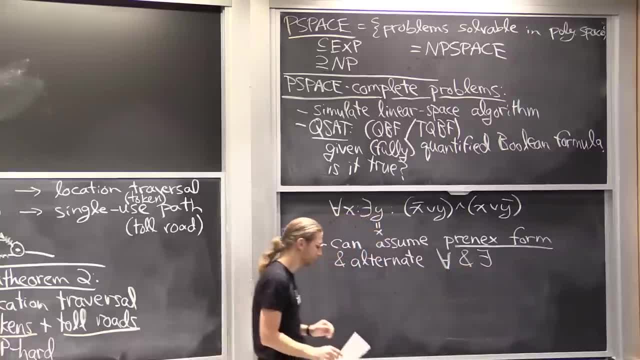 You have to think about the case where there are lots of alternations between the two. We'll talk more about that when we get to two-player games, because that relates to two-player games, But for now we're going to stick to one-player games. 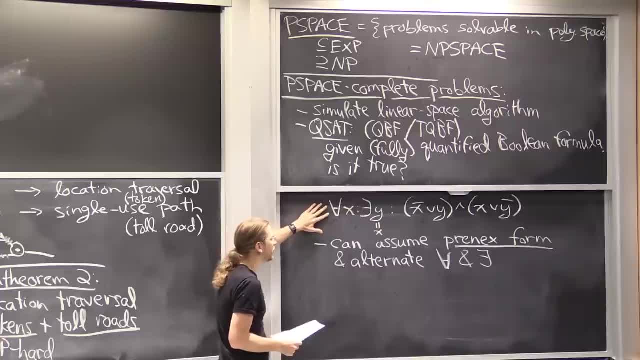 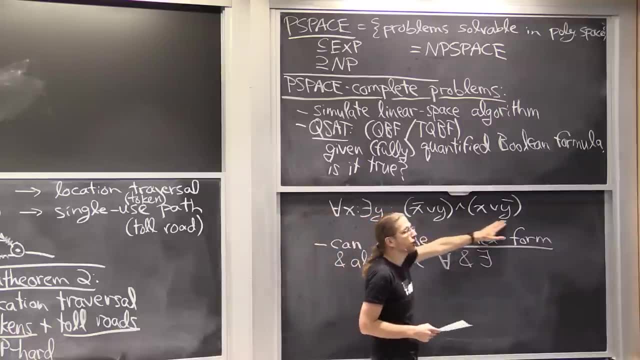 And this is just something we need to simulate by our single player. And so now the question is: what's the formula that we're going to use, And the question is, what forms can this formula take? Because we have lots of forms of SAT that we know are hard. 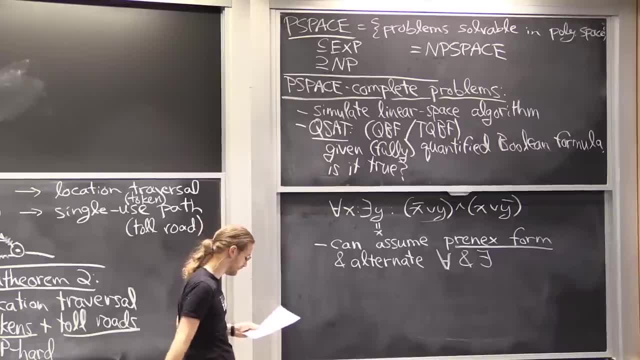 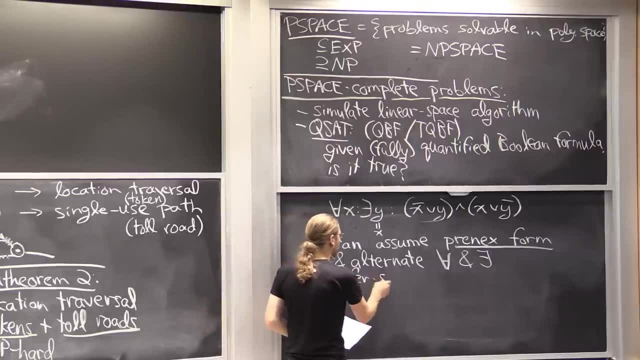 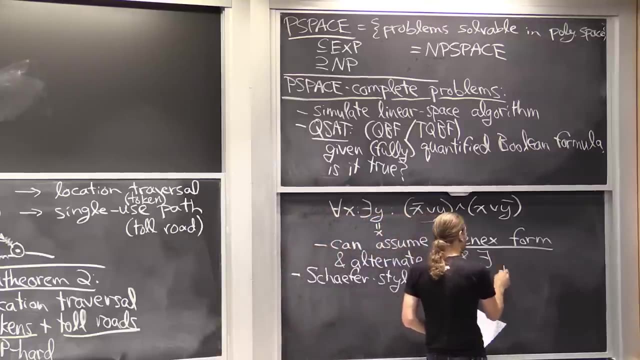 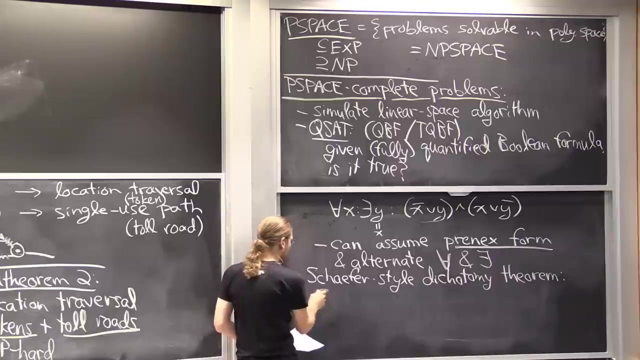 And pretty much all of them remain hard in this setting as well, when you add in the quantifiers And in fact there is a Shaffer-style dichotomy theorem, like we had with SAT and NP, And basically this quantified SAT is polynomial. 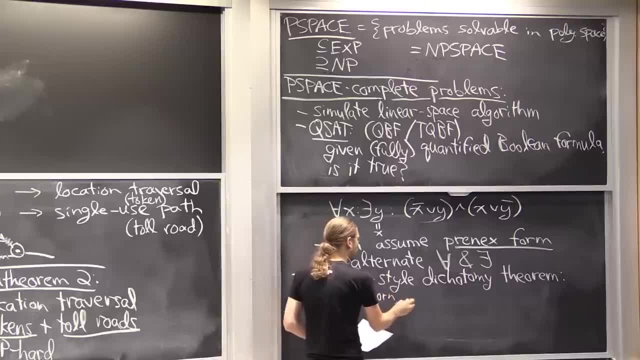 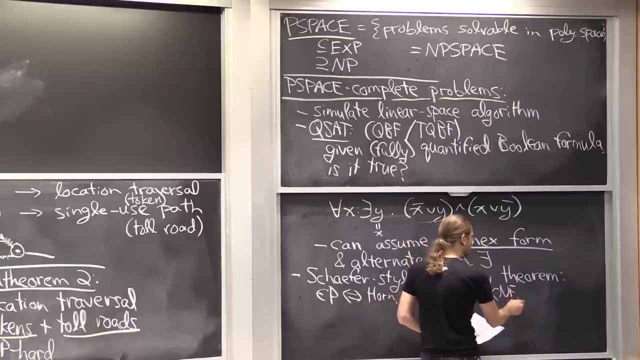 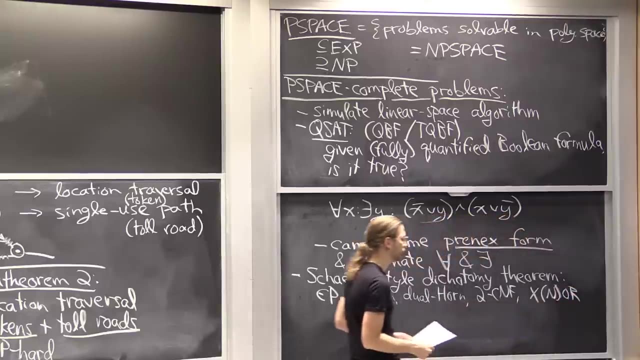 if, and only if, the types of clauses you allow are all horn clauses or all dual horn clauses, or all two SAT clauses, or a system of linear qualities, mod 2, XOR and XNOR equality constraints. Those could all be solved before they can still. 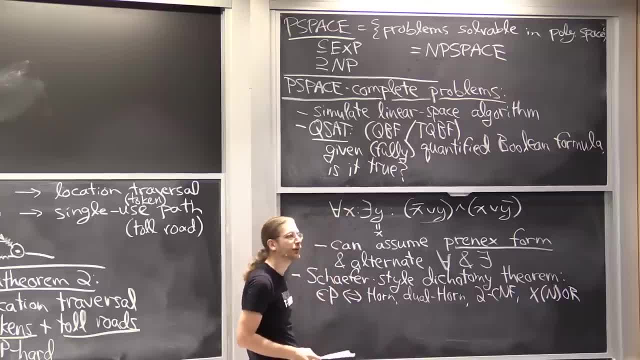 be solved In this setting in polynomial time, even with alternating quantifiers, So that's cool. However, it is no longer a polynomial time if your clauses are satisfied when you set the variables all true or all false, Because we have these for all quantifiers. 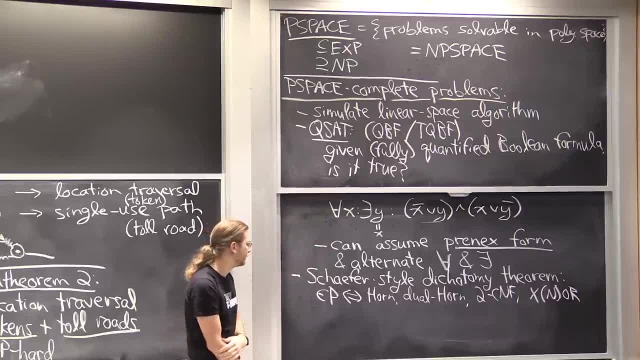 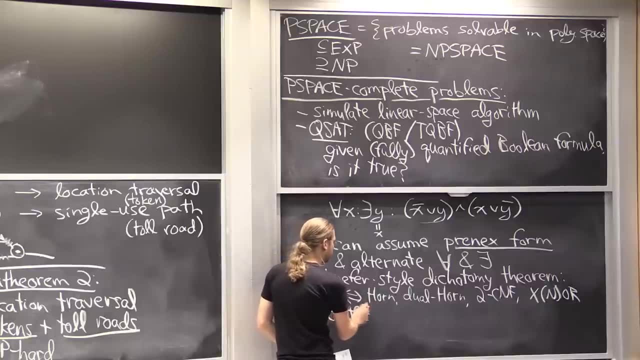 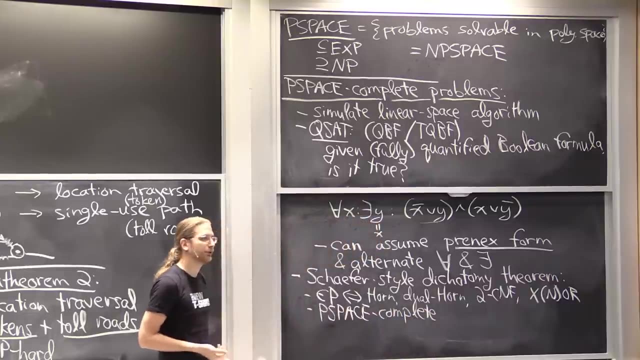 now being all true is not the panacea that it was before. So that's one case, And otherwise you are PSPACE complete. All other versions of SAT are PSPACE complete, Sorry of QSAT. So it's almost the same as the Shaffer theorem. 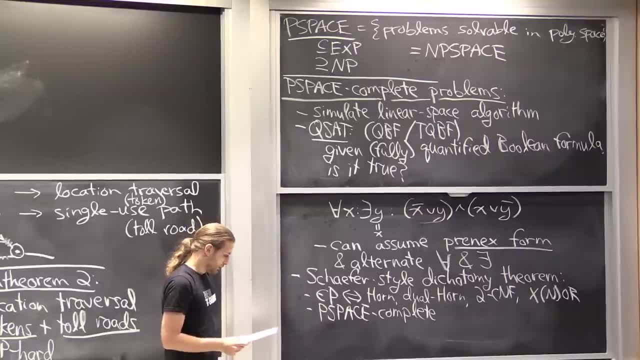 but there's one case that differs: It's hard, whereas it wasn't before. So that's cool for general from a formula perspective, But we of course typically care about planar bipartite graphs expressing those clauses and their variables. 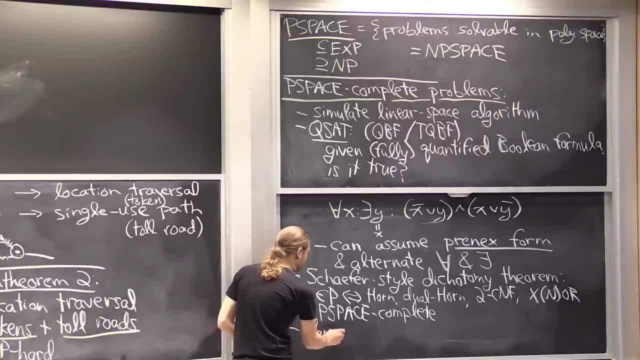 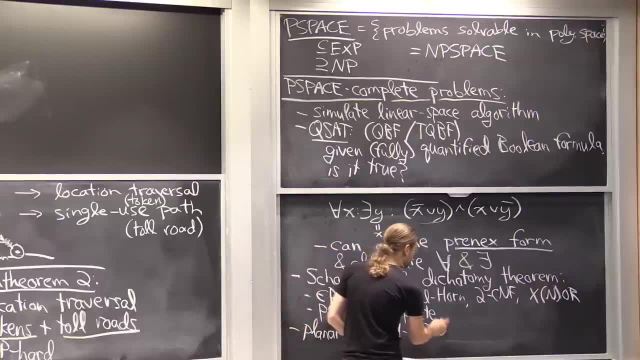 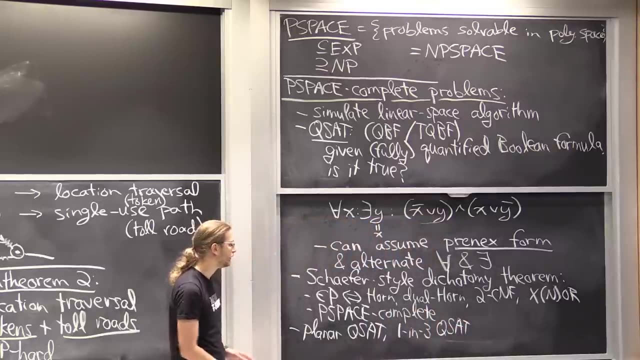 And good news is everything works as before. So planar QSAT and planar 1 and 3 QSAT are hard Planar, not all equal. QSAT is also going to be easy like it was before, But planar QSAT- we can use the usual crossover gadget. 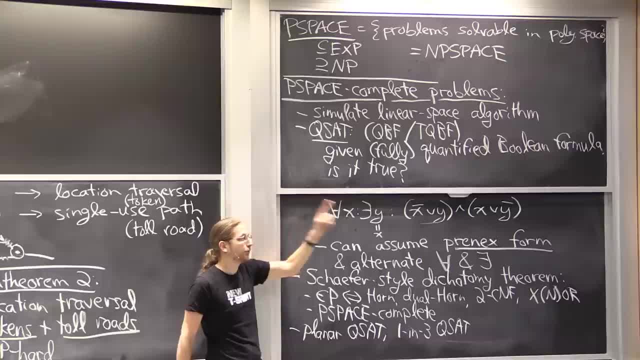 What that crossover gadget does. it forces some variables to be the same, but it also creates new variables, And those variables need to be quantified. All you need to do to simulate our old proof is put a whole bunch of existential quantifiers at the end of the quantifier list. 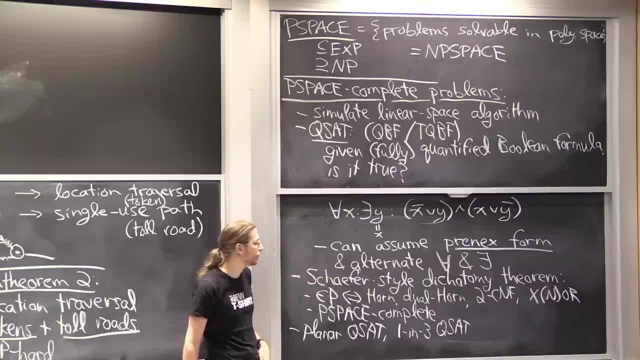 So for every new variable you create you put there exists at the end for those variables, And we know those variables are forced to be equal to other copies of variables that are given to us. And so it simulates the old planar SAT proof. 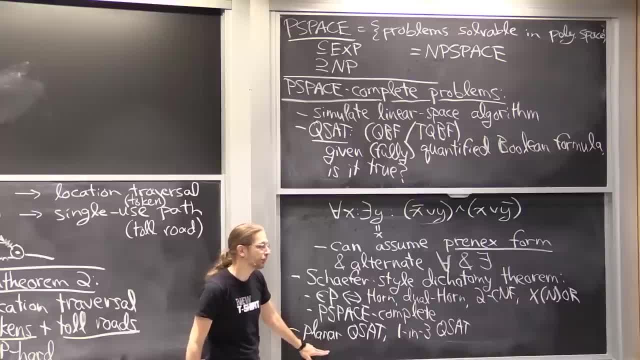 but in a quantified setting, And that was actually done by Lichtenstein in the original planar SAT paper. OK, They also talked about planar QSAT. And then, once you have this, problem is hard. the same reduction we had for 1 and 3 QSAT also just works. 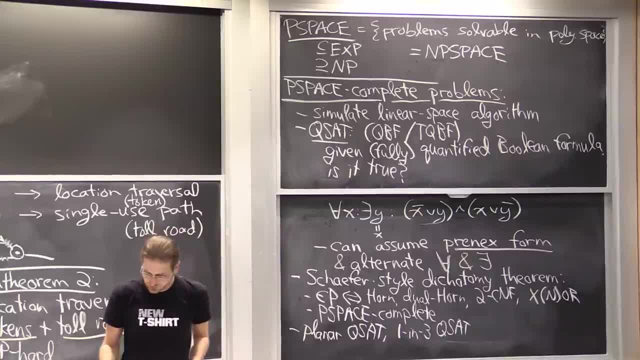 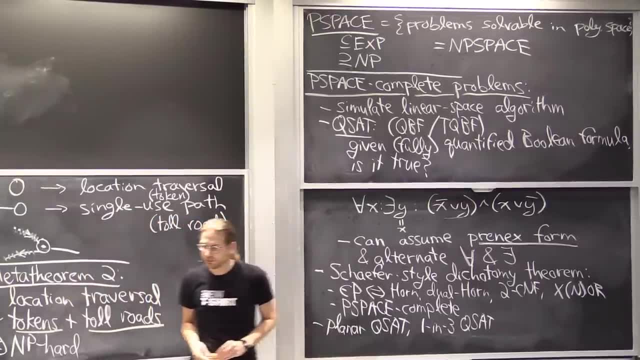 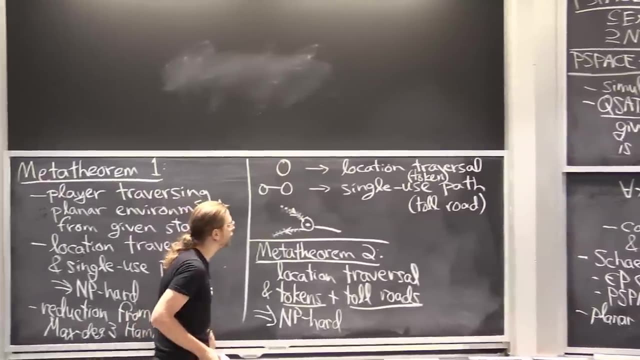 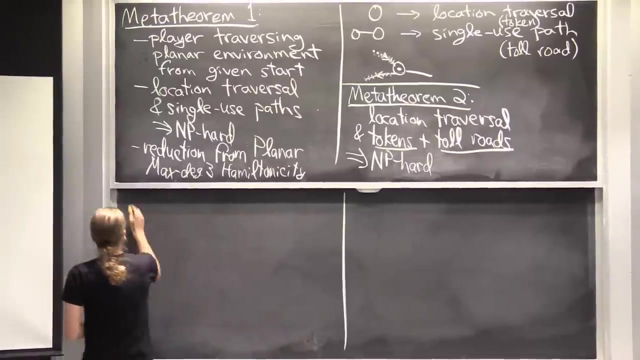 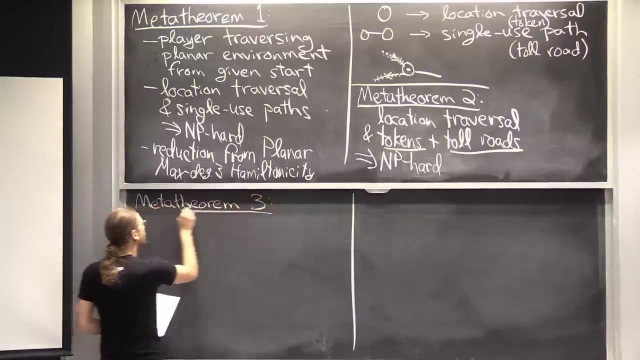 So with the same idea. So there are some base problems. Now we can do some reductions. First we'll prove a metatheorem And then we'll apply that metatheorem to a bunch of different games- One player games. So for next metatheorem we're going to have a similar setup. 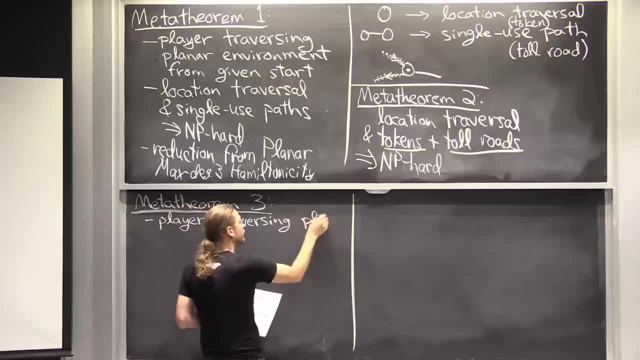 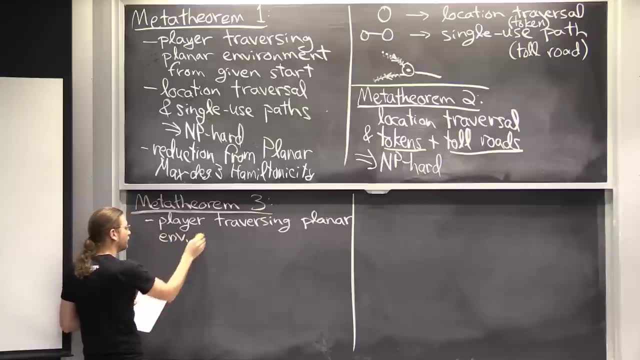 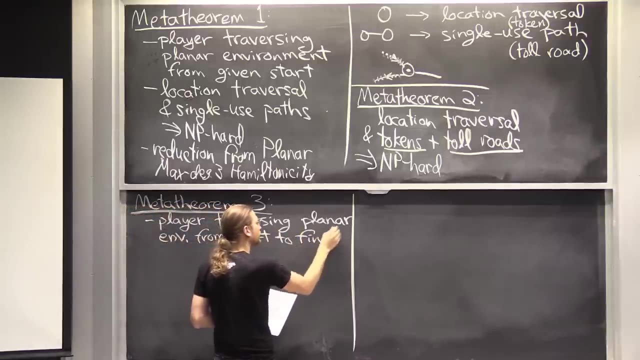 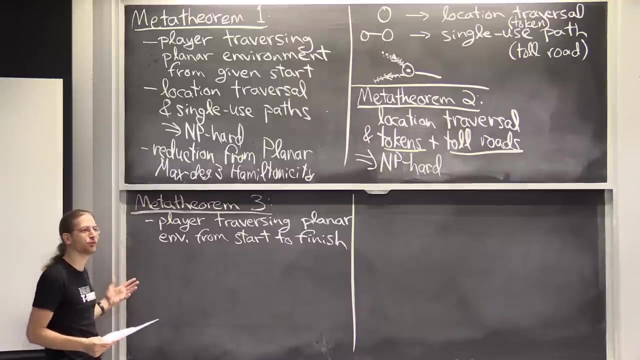 We're traversing a planar environment, but this time we are given We're going to have a start location and a destination. Because we're no longer going to have the location traversal goal, we need to add some kind of goal, Otherwise you've solved the game by starting. 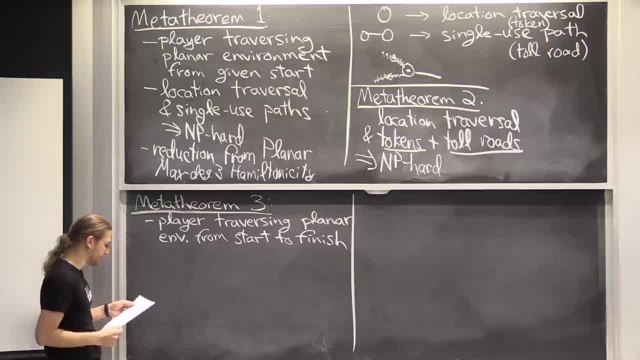 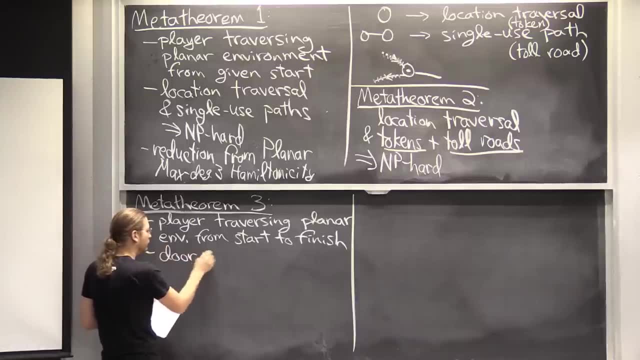 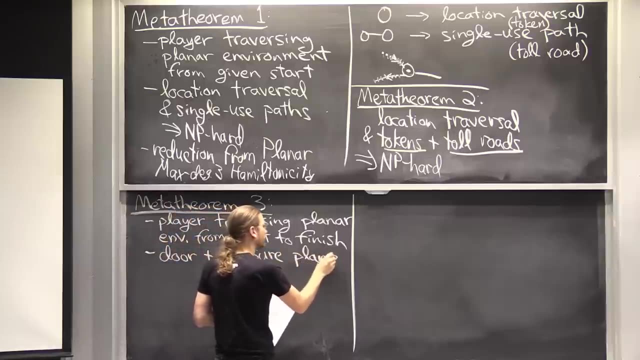 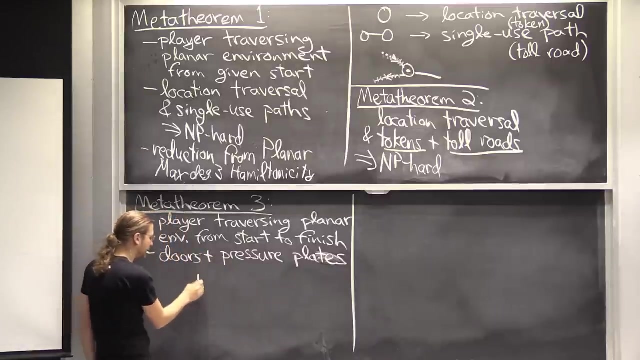 So it's a path traversal- get from A to B, And what we're going to need is a door plus a pressure plate. So the idea is that there is an obstacle, a door which is either open or closed, And there's a pressure plate where 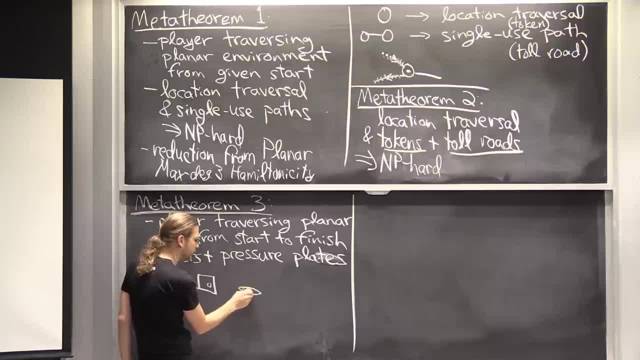 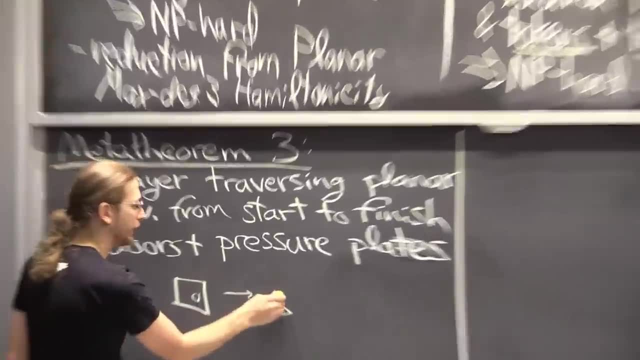 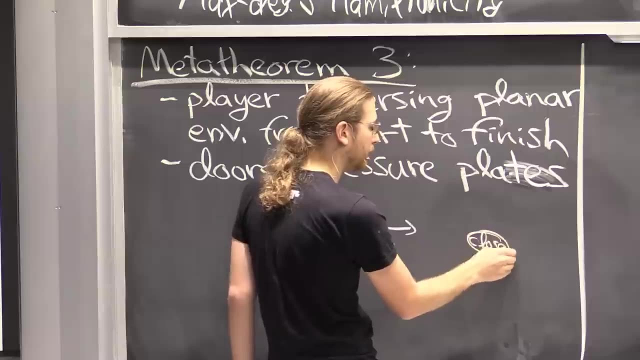 if you step on a pressure plate marked open. so you're walking along here, you step on this square, that will open this door and make it traversable. as you go across it, You're forced to open the door And there's going to be another pressure plate marked closed. 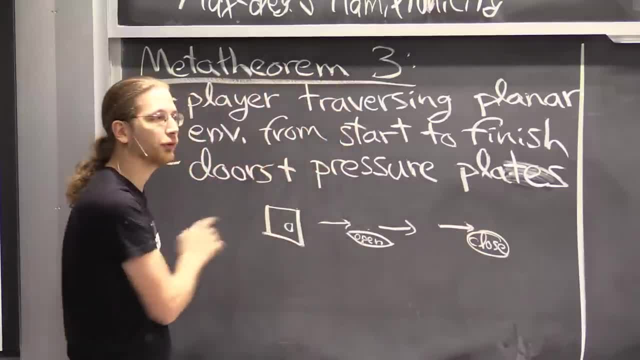 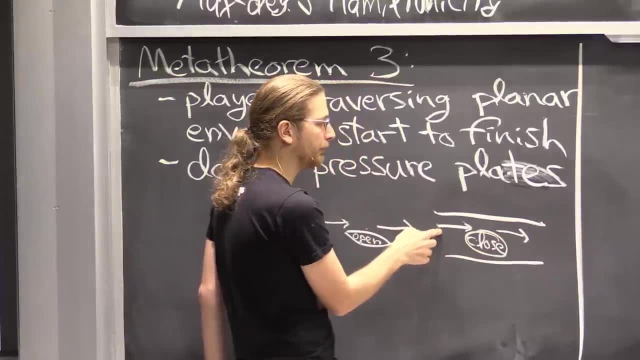 which, as you traverse it, you step on that plate. it forces the door to close. So, in order to get to the other side here- usually this is in some kind of tunnel- So in order to get from this side to this side, 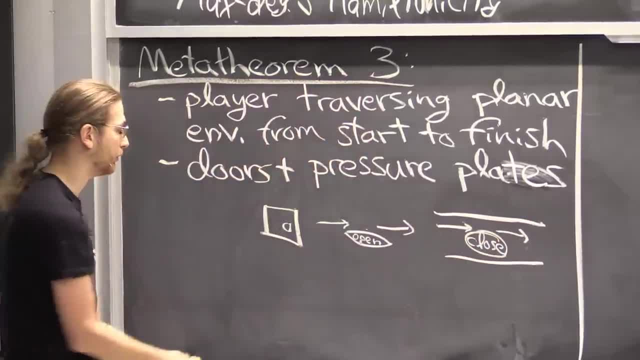 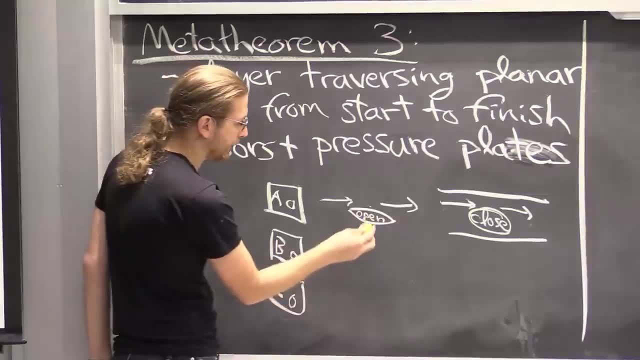 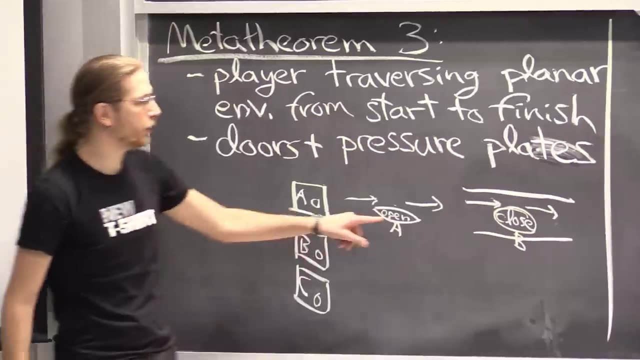 you must close this door, And we have more than one, So there are many such doors. Let's say A, B, C, And this is going to say open A, This is going to say close B, And we can furthermore assume that there's exactly one open and exactly one. 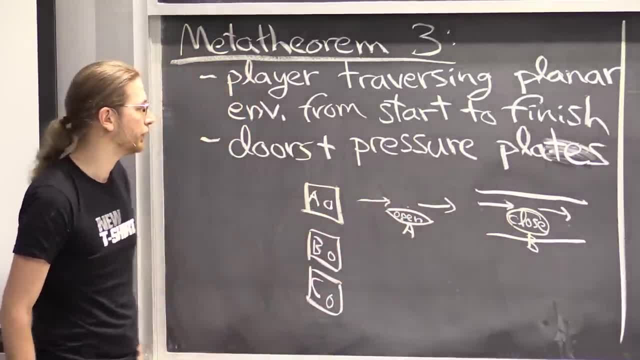 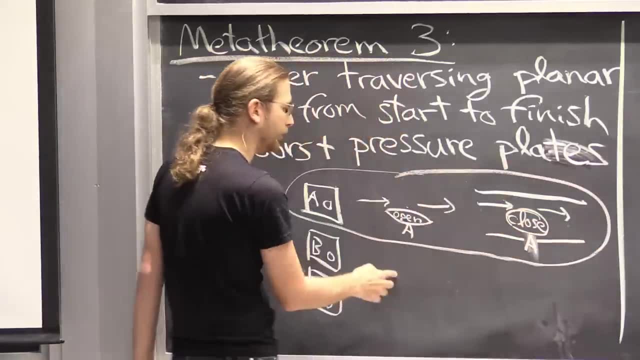 close for each door, So maybe I should have written A here. So this is the complete story for A And there's a similar open and close for B and open and close for C, And otherwise you can just walk around And your goal is to get to destination. 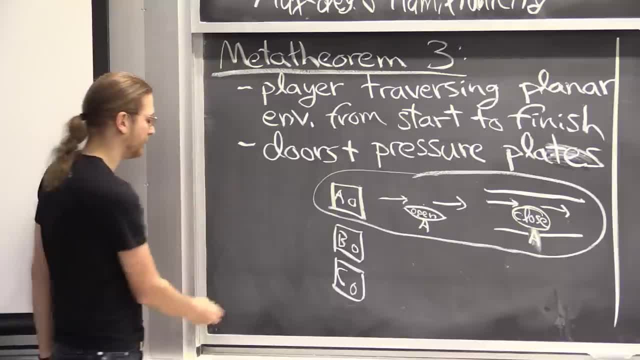 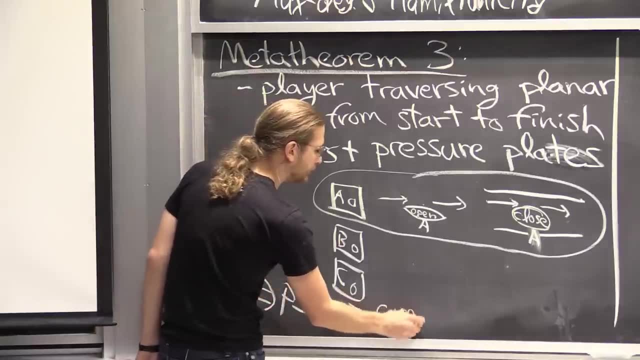 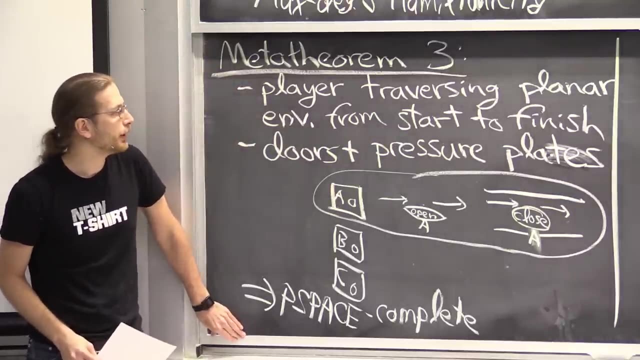 Sounds pretty simple And this is a very powerful metatheorem. This is PSPACE complete. This applies to a lot of games, But before I get to what games it applies to, let's prove that this is indeed PSPACE, complete by a reduction. 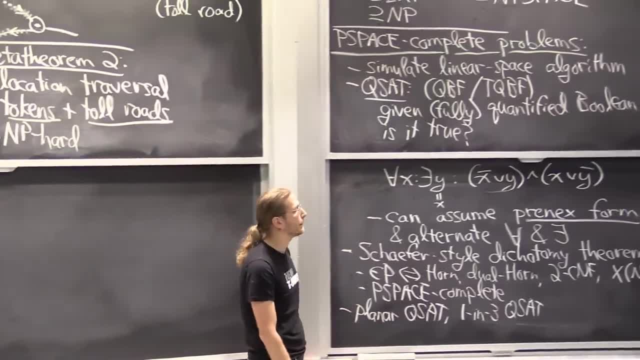 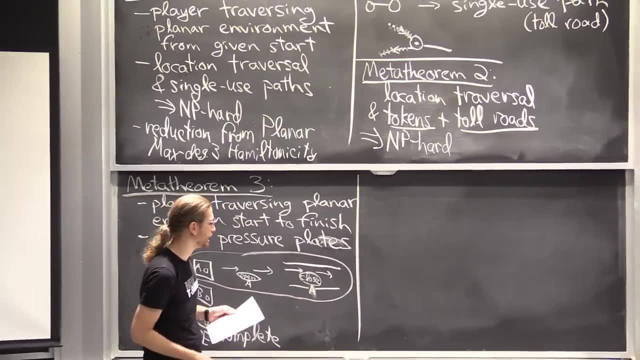 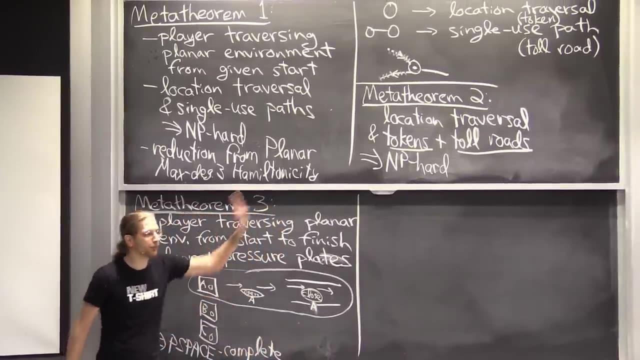 from Q3SAT. We won't even need planar here. We won't need planar because we can open doors kind of remotely. When I step on this button, which could be far, far away, I open this door So effectively. the connections between variables and clauses. 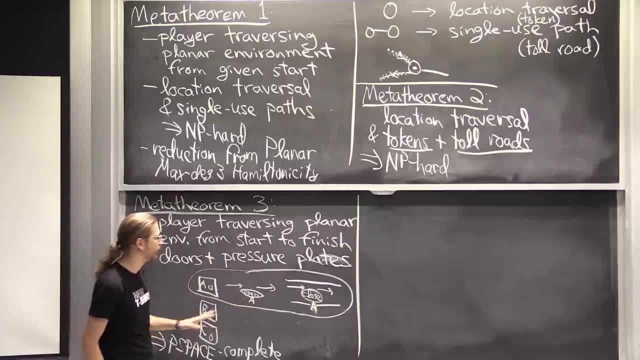 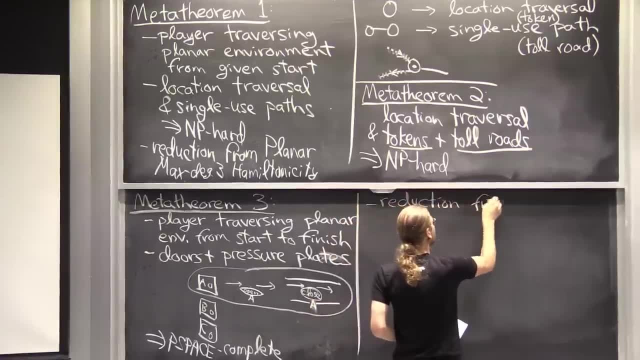 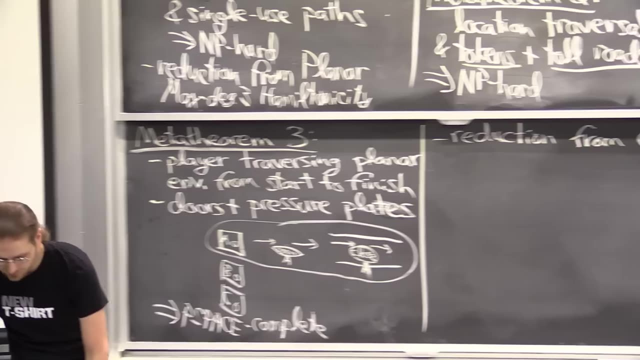 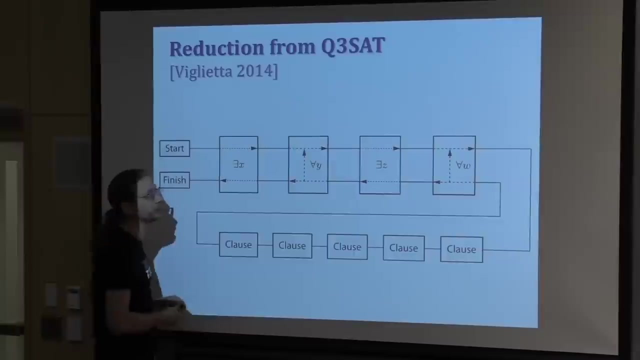 can be crossing. There's no restriction on that here. So you're going to see a few different proofs like this. We'll see others in future lectures, But this is a typical prototype for how to reduce from Q3SAT. You have your start location. 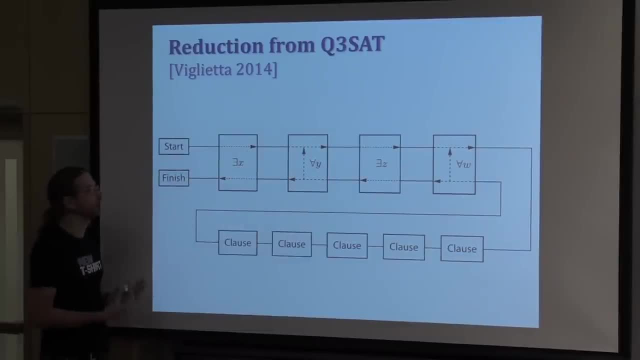 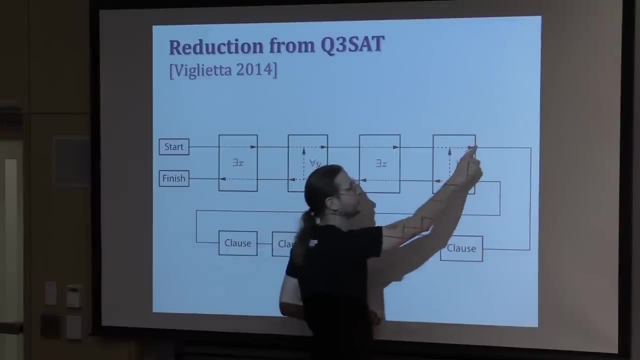 You have your finish location. Your goal is to traverse this thing, sort of like a circuit, And then you have these blocks which represent quantifiers. We'll talk about those in a moment. In the end, you exit here And you have to satisfy this formula in order. 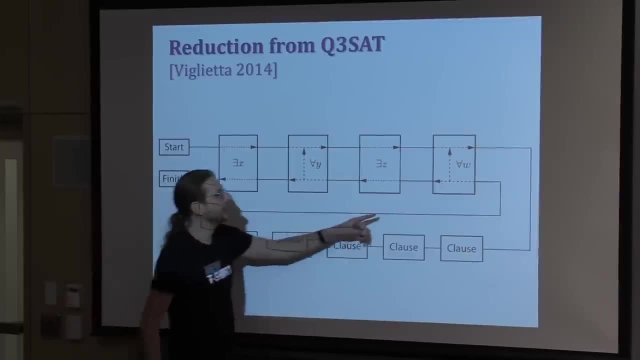 to get through. If you get through, then you are able to enter this quantifier gadget, And these are kind of in a nested structure. You can think of this quantifier gadget as calling this one. By traversing this path, you're recursively. 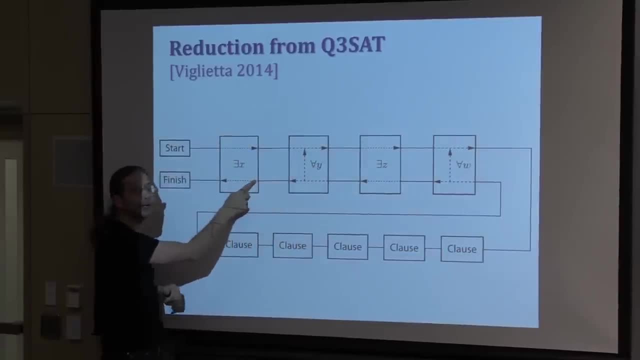 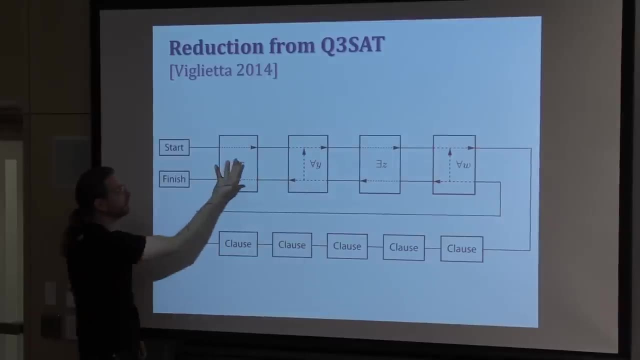 calling the rest of the formula, And then this is sort of the return value. Yes, I did it, I succeeded, I got a yes, And when you do that, so for the existential quantifier, what this is essentially doing is say: 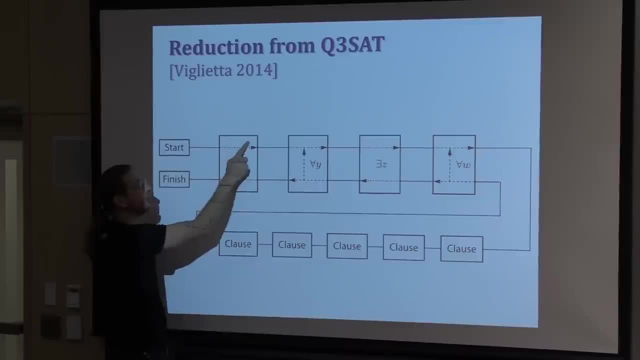 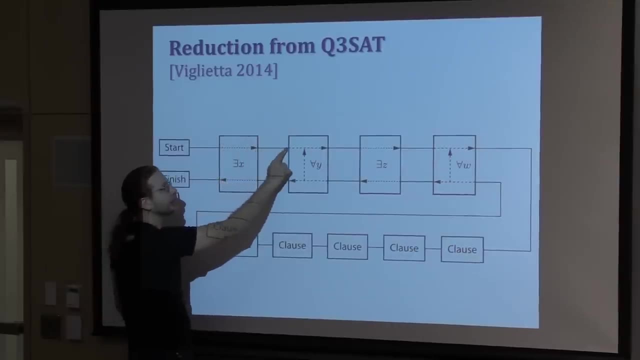 OK, I don't know what x is going to be. I'm going to let the player decide between two different paths: set x to true or set x to false. So there will be two ways to go here, And then you'll exit along the same path. 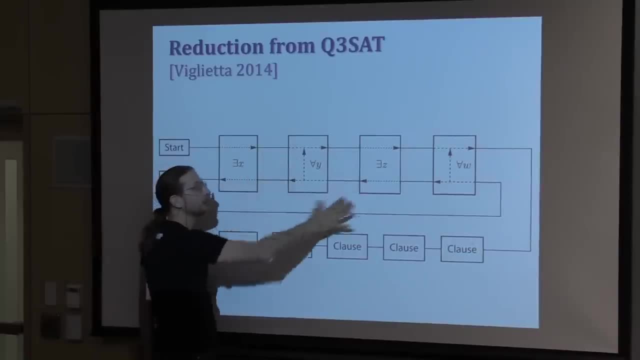 But x will be set one way or the other, Recursively. you want that formula to be true. If that happens, then the player will be able to come back here. And if you successfully set the rest of the things true, if you set the rest of the formula to be true, 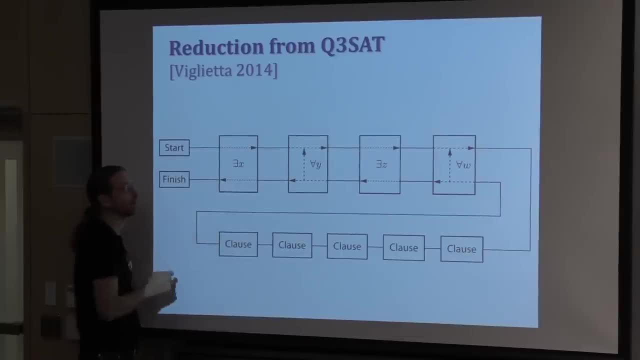 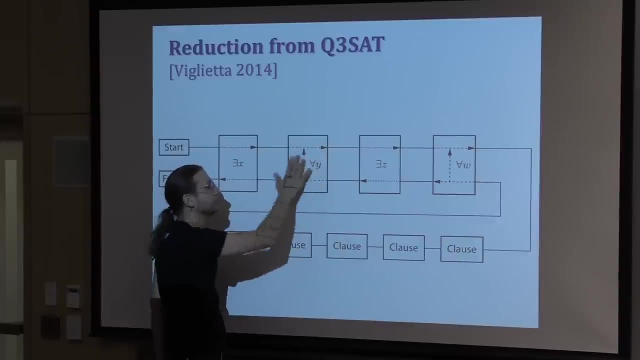 then it means the overall formula is true, because you just wanted to check that there was at least one setting for x That made it true, And so this is just a direct connection. On the other hand, for the universal quantifier this is a little bit trickier. 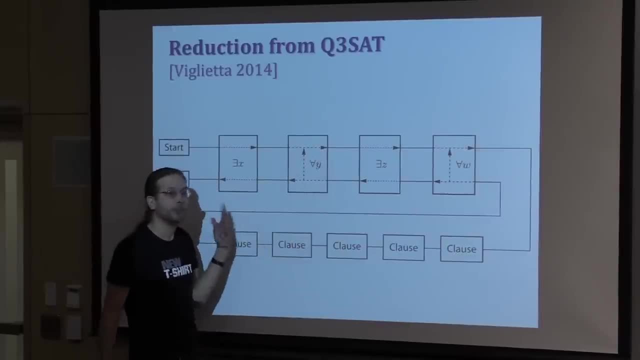 And it's drawn at a very high level. here You need to check both settings of y. So what you're going to end up doing is, if you enter this gadget, you're first going to set y to true and exit out here, And then recursively the rest better be true. 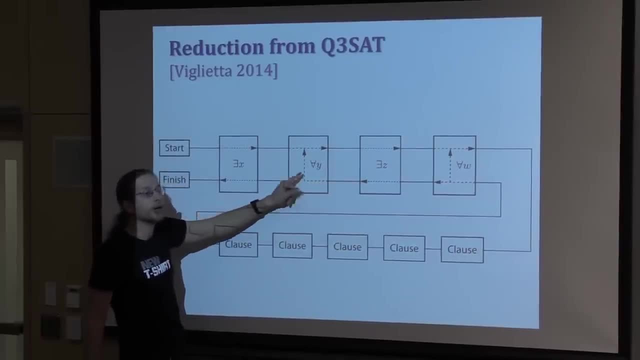 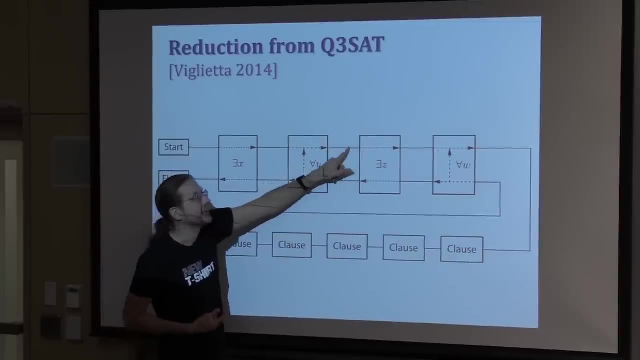 If it is, you come back here. When you come back here, you mark the fact that you got one setting correct. Then you set y to false or the other setting, And then you go out here again And if the formula is again true, 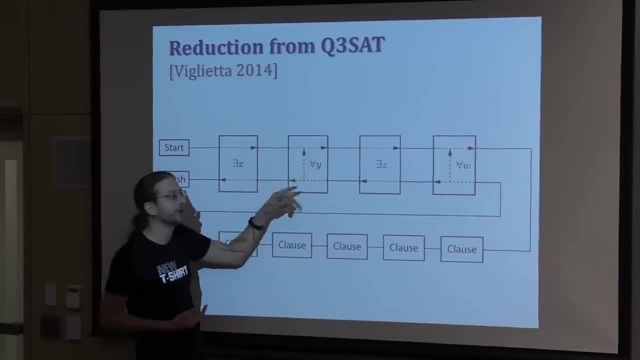 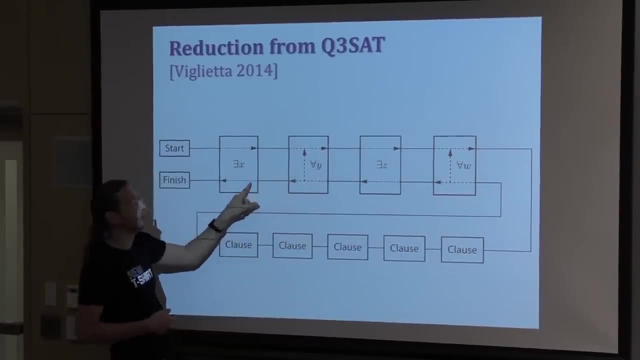 you'll be able to come back And if you've accumulated two correct answers internal to this gadget, you know that the overall formula is true with a universal quantifier here, And then you'll be able to return out to the caller. So that's the recursive algorithm view. 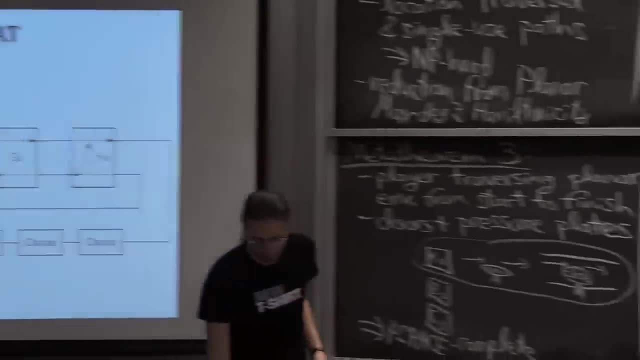 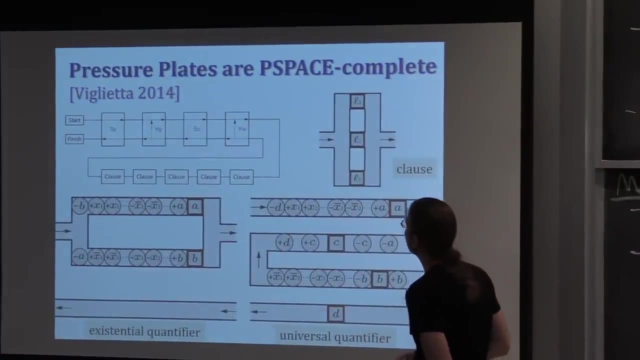 of what's going on here. Let's do that with pressure plates, So it looks a little bit messy, but the idea is very simple. It's implementing exactly what I said First. these clause gadgets, these are three set clauses, And what we're going to do is just have three doors. 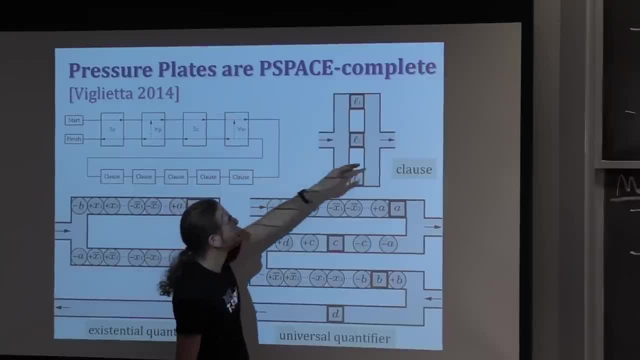 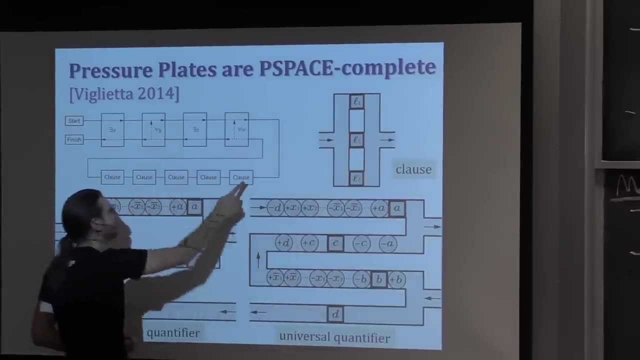 And this is drawn in the reverse order of what it should be. It's going right to left usually, but it also works in the other direction. If any of these doors is open, you can get to the other side And, in order to get through all of them, 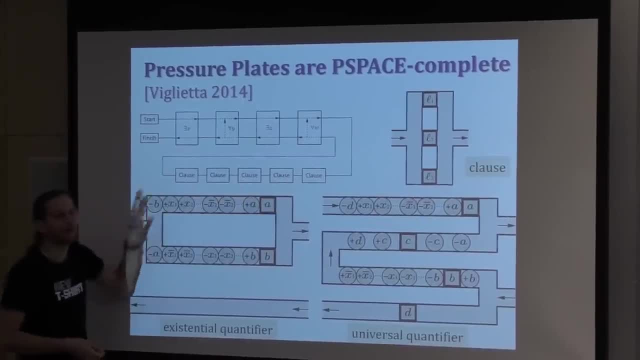 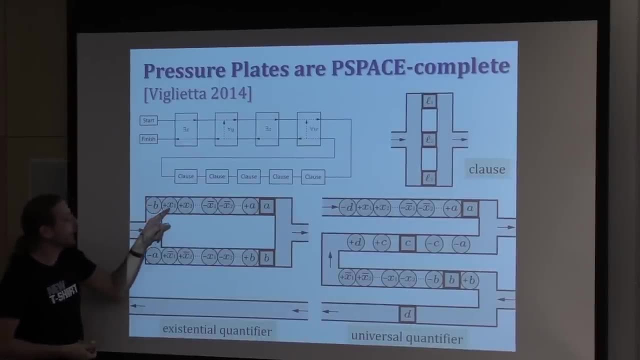 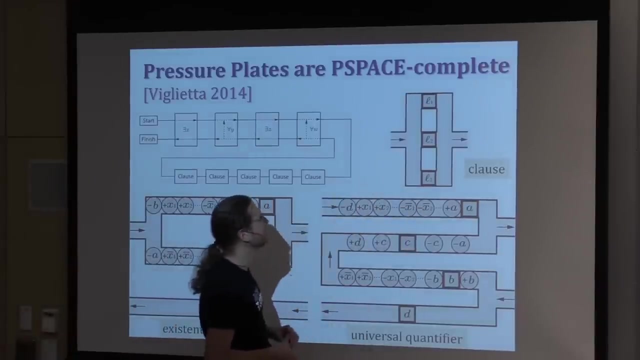 all the clauses must be satisfied. So that's the idea. Three set part. Really easy in this setting, Where door open means that the variable is set true. In fact we will have both an xi and an xi bar door, And so you use the corresponding literals there. 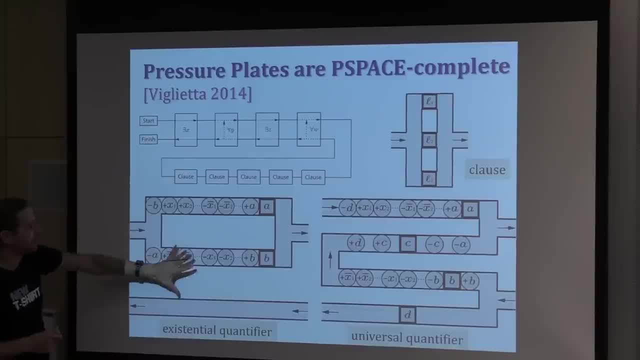 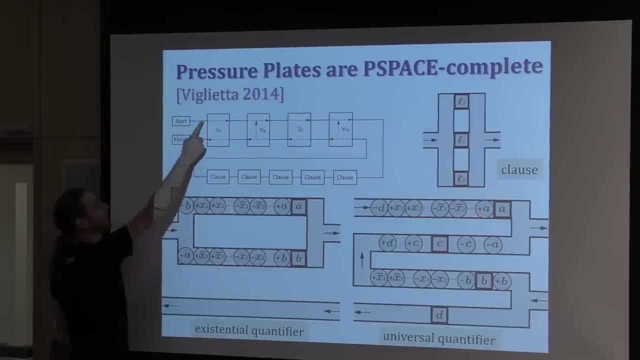 Cool. So now this is an existential quantifier, easier case to think about. So let's say we come in from the left, as in here, that's coming into this part of the gadget, And we have to give the player a choice. 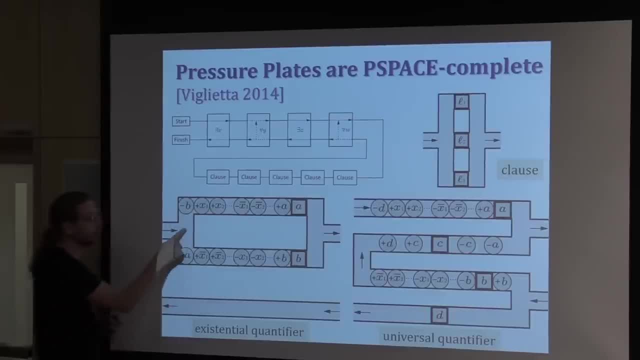 They can either take the top path or the bottom path. Now there's a worry that maybe you go a little bit this way and then double back. But that's not going to be possible. We need to argue that. So negative means close. 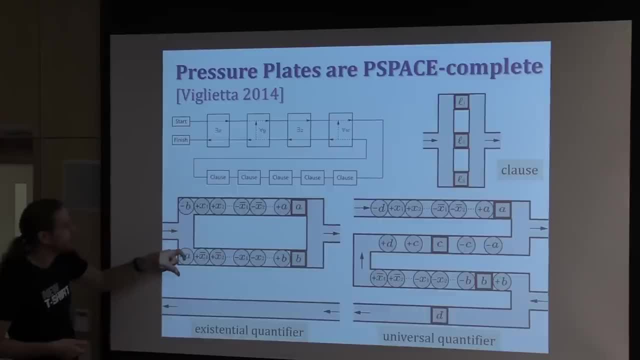 And positive means open. So if I come in here, the first thing I do is close the a door That's going to prevent me from later coming back through. this way. I can only have one door for each, But I want a variable, a literal. 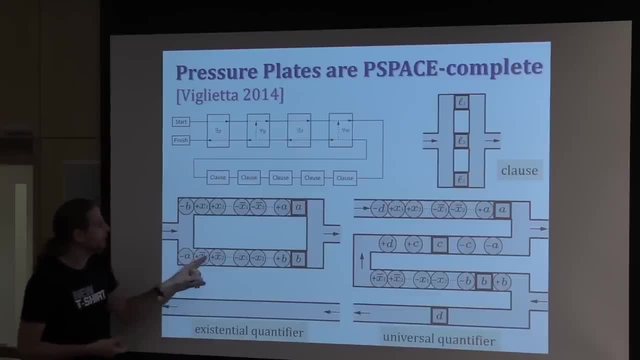 to be able to appear in many clauses. So in fact I'm going to have several copies of x here. So this is the first occurrence of x1 bar, the first occurrence of x2 bar, and so on. I want to open all of those doors. 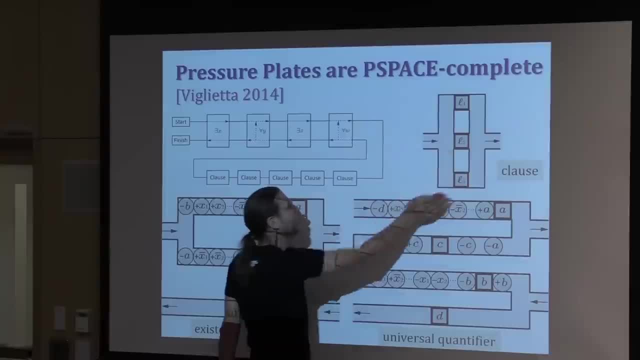 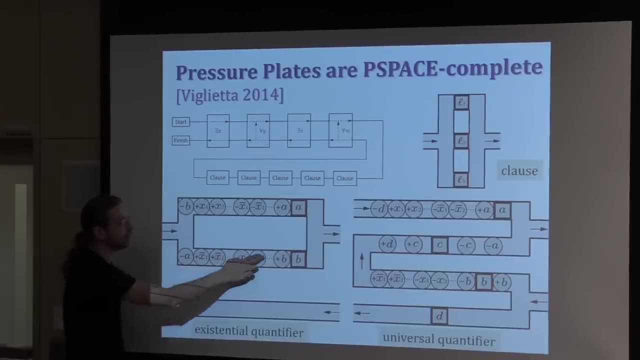 so I can use individual copies of the variable up there. And then I'm going to close all of the positive versions of x. This corresponds to setting x to false. And then, at the very end, I open the b door, which lets me go. 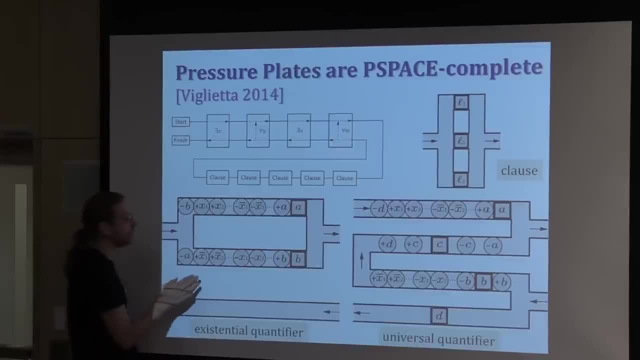 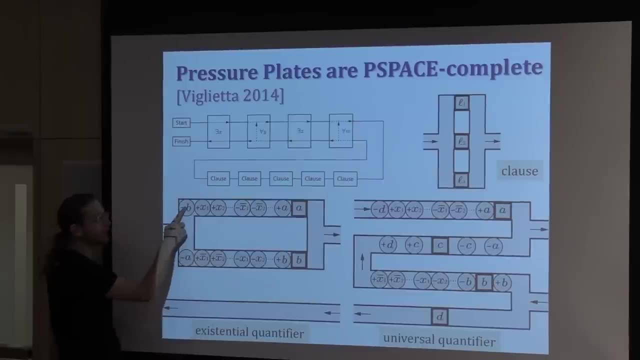 through here. And since the reason you can't mess up this gadget is, if I went part way and then doubled back, I would immediately close the b door, which means I can't really exit this way, which means I'm going to have to go all the way through here. 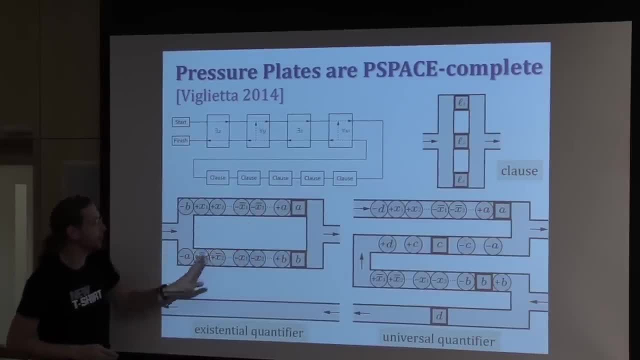 and reset all of the variables, And this is exactly the complement of this, And so exactly one of these will be fully traversed, The other one will be nullified, And then that corresponds to existential quantifier Question. The doors start in a closed state. 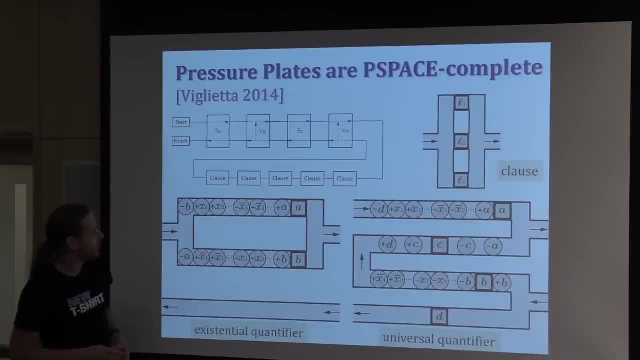 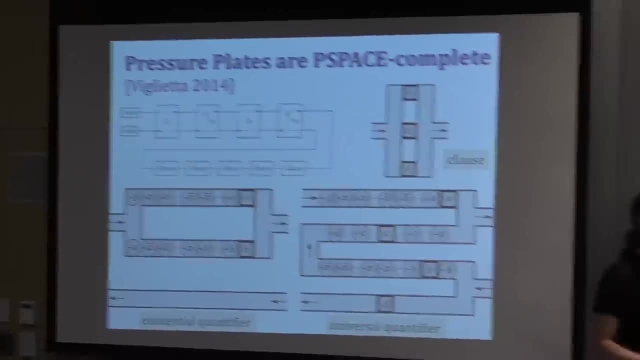 Let's say, all the doors start in the closed state, although I don't think Can you close things more than once. Yeah, Sorry. One important thing is: if you click on Open when it's already open, nothing happens. If you click on Close when it's already closed, nothing happens. 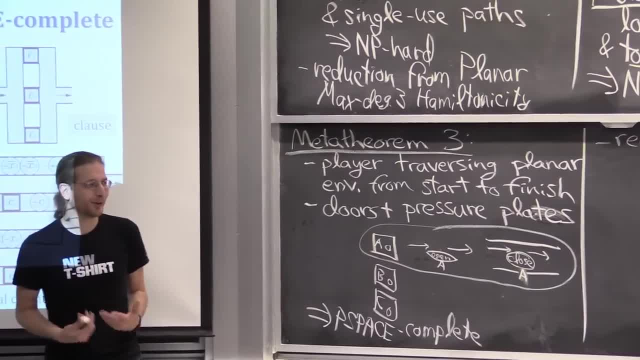 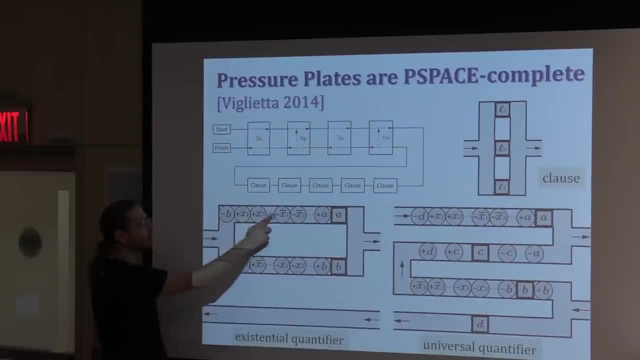 So you can close multiple times. It doesn't make it more closed, It's just closed. Stepping on the close and then going back and opening b seems to work. So you could do some of this and then double back. You're right. 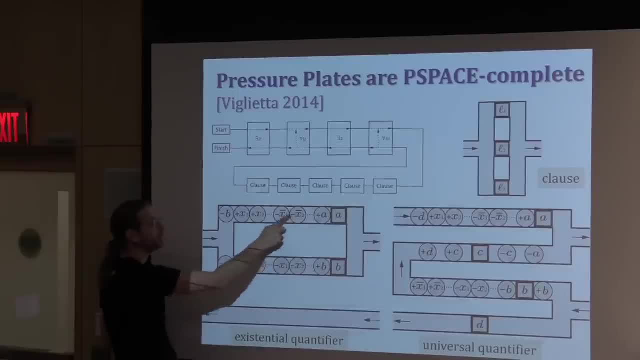 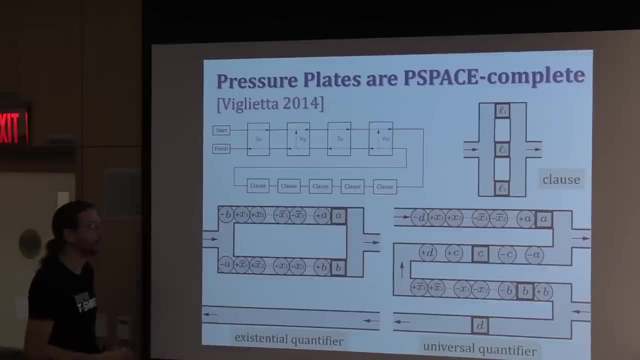 You will open up again, But by traversing all of these, you undo all of the things you did up there, because these are complementary, So you fully traverse one as the last thing you did. That's going to be the one that sticks. 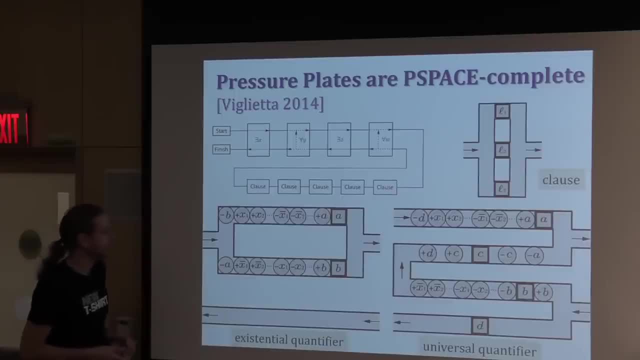 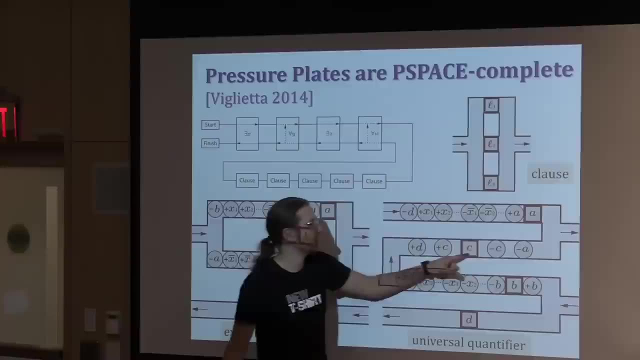 Yeah, So that's pretty nice. And on the other hand, here is a universal quantifier, Not that much harder, But this is essentially. there's one door inside here which is keeping track of. am I going through this for the second time? 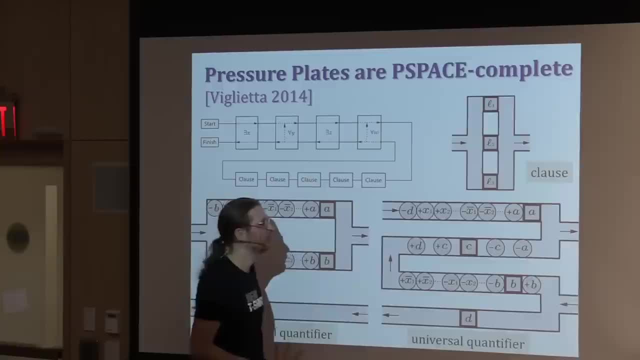 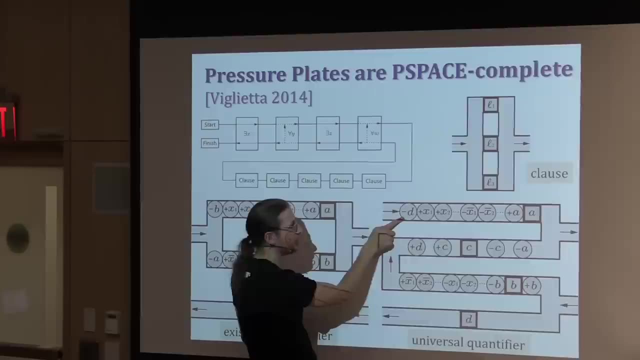 So in this case There's no choice. We just have to try both settings. The first thing we do is set x to be true. That's the setting, And we also open door. Sorry, we close door. d All right. 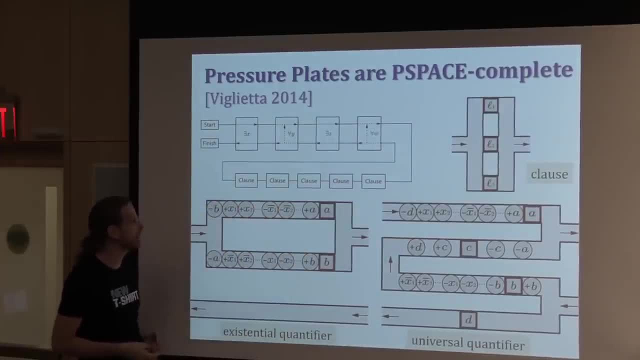 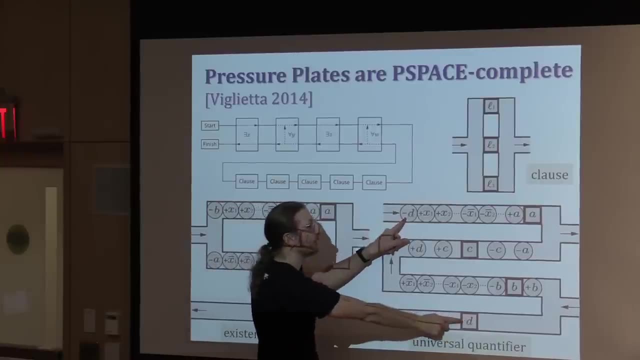 Sorry. Your other question is: do the doors start open or closed? I don't think it matters, Because we have these closed things in the beginning. essentially, everything gets closed at the beginning. So here we're going to close d, which is our final exit. 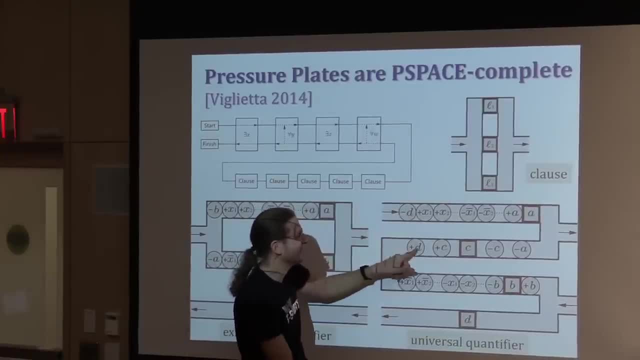 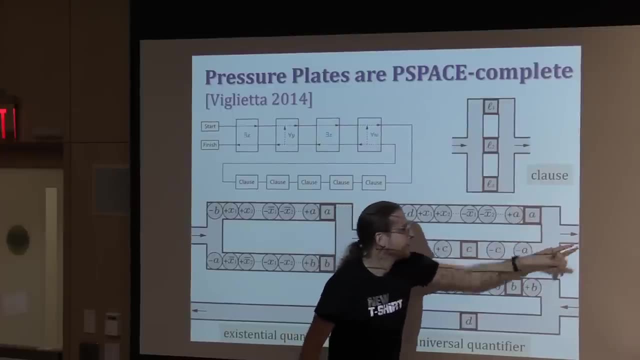 That's where we want to get. So that's going to be hard. We have to get to the open d spot, Then we set x to our setting, Then we open a And now we're allowed to go here. You could try to go this way, but it's. 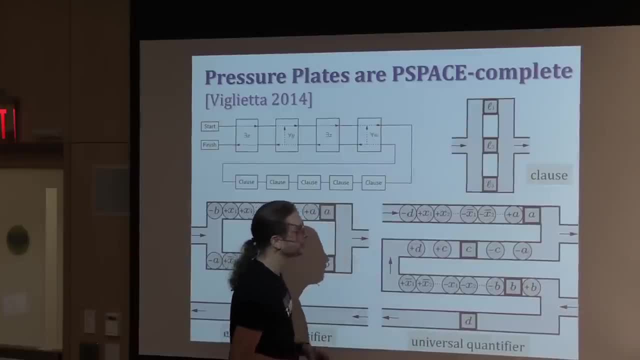 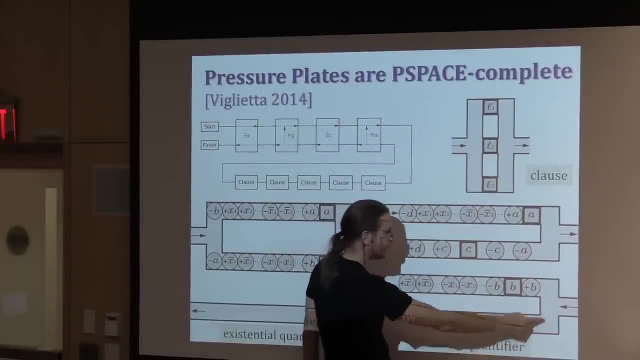 just going to close a couple doors, So it doesn't really help you. So we recursively call the thing with x true If it comes back with the thing being satisfied. we can't go through here because d is closed, So we're going to have to go through here. 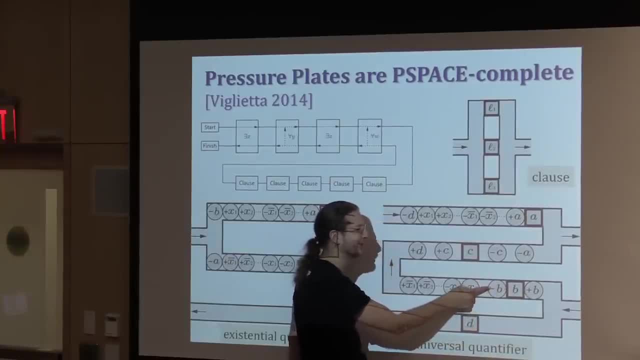 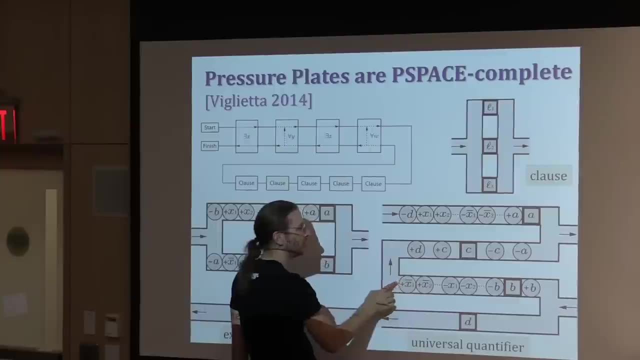 We open b, We immediately go through b, We immediately close b. So that's a one-way gadget, OK, OK. OK, OK, Now we set x to false the opposite of this thing, And we can't go backwards because b is closed. 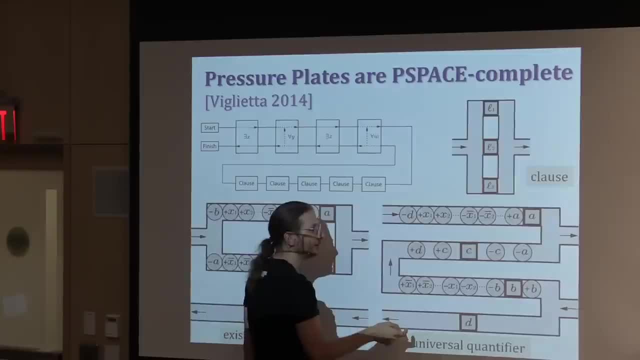 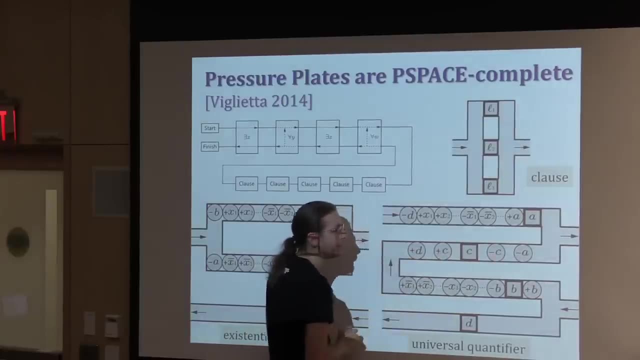 Now we open d, So if we can get through again we'll be able to exit. We can't immediately turn back because again b is closed. We open c, visit c, close c, So another one-way gadget, And we also close a to prevent other weird things. 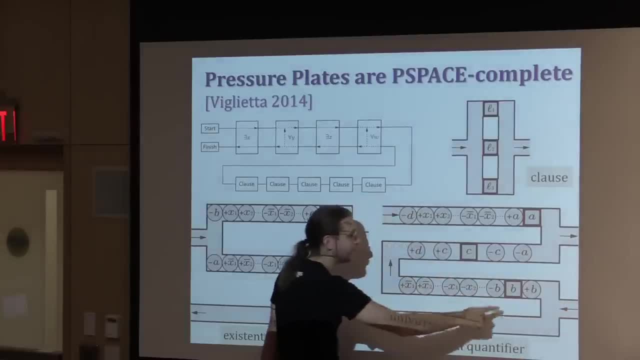 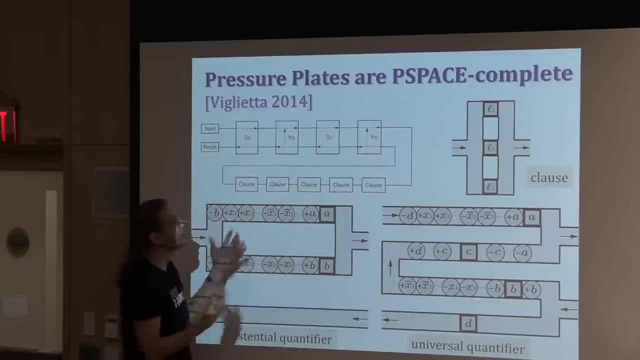 from happening. So now we go through again. If we get back with d open, then we can return and we're happy. OK, So we're back in the actual construction. Keep in mind: what's happening here is we are making an exponential length puzzle. 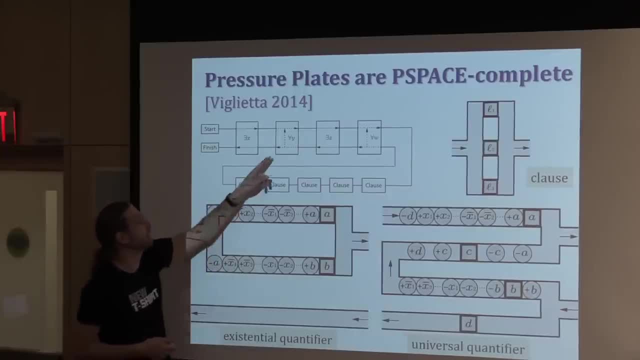 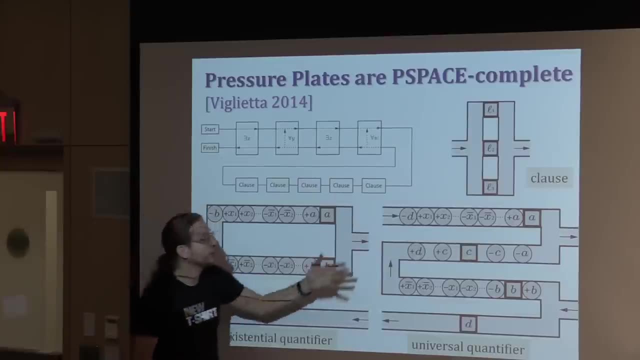 The length of the solution is going to be exponential because you have to try both settings of all the universal quantifiers. So any gadget is going to be visited many, many, many times, But each time we're completely resetting x, resetting x again. 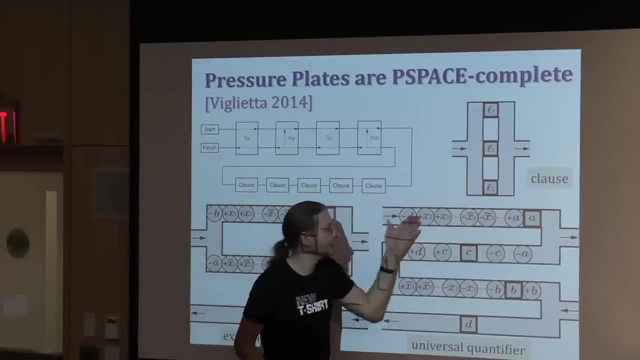 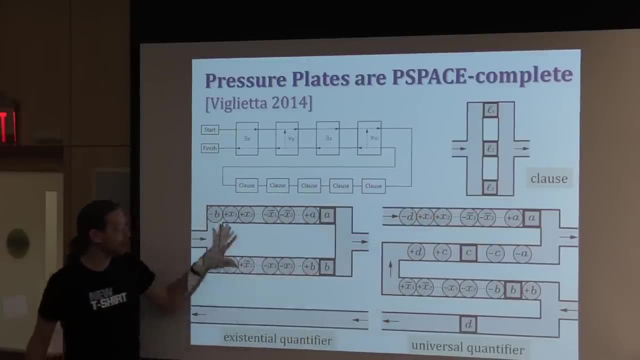 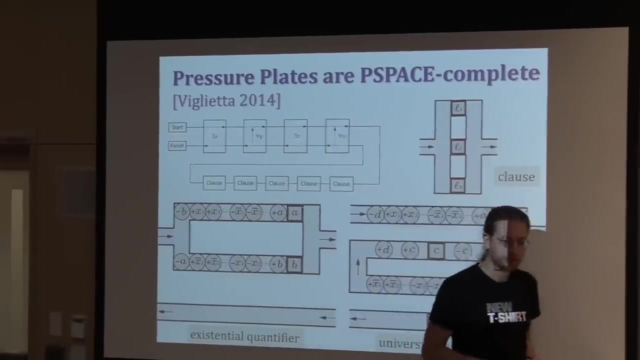 and then returning. So we'll revisit, We'll reset x to true and then later to false and so on. But we are checking all the possible assignments for here And we're letting the player nondeterministically guess. an assignment for the existential quantifiers. 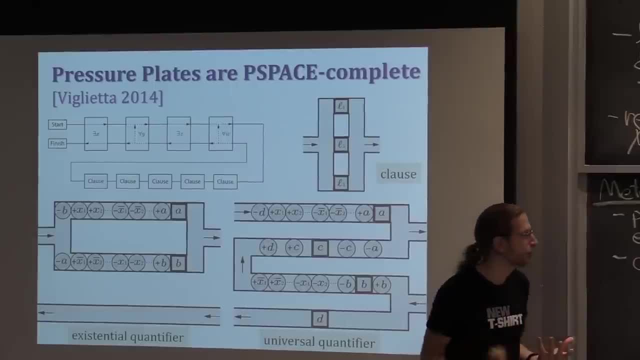 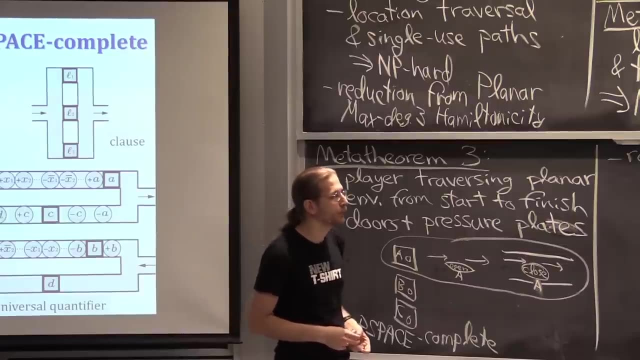 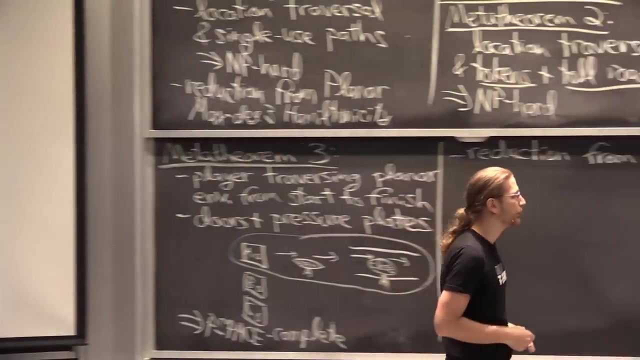 So that is pressure plates in the abstract, piece-based completeness. Sorry for another question. In our usual sense of reduction we usually think of a polynomial size thing that we make Good. Yeah, I didn't mention it, but there are different notions. 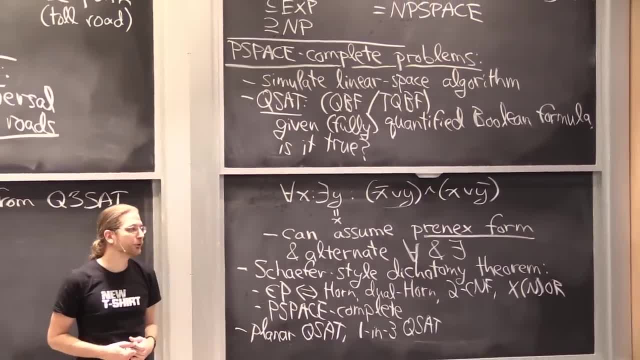 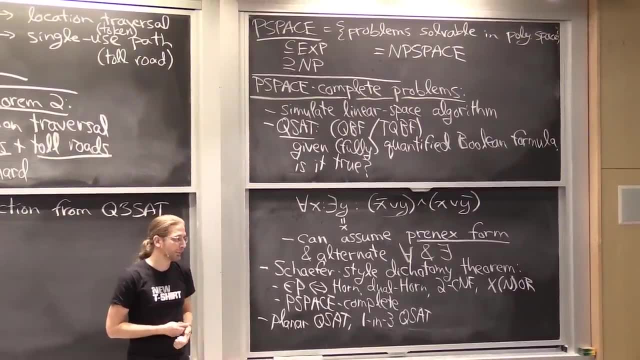 of reductions for piece-based completeness, But for the most part we will. We will just use the same notion of reduction we did before, which is the running time of the reduction should be polynomial time. So here we're given a formula which: 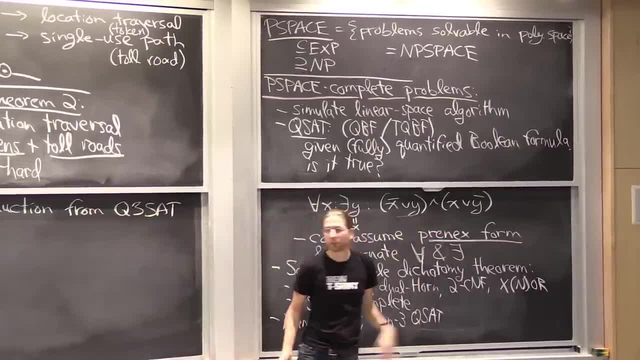 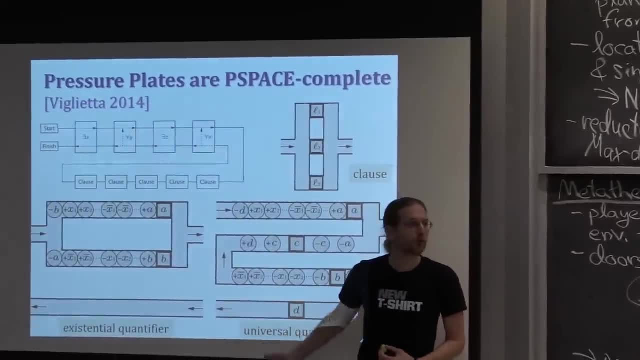 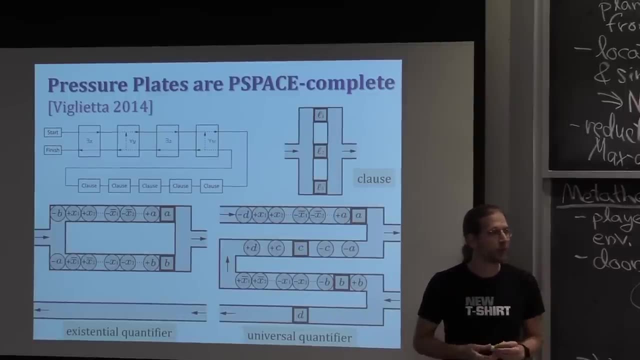 is expressed in this kind of succinct form And we're producing a level whose size is polynomial, in that Now, the actual execution of the game, the trace of what happened or the certificate that is solvable, that has exponential length, But we're not. 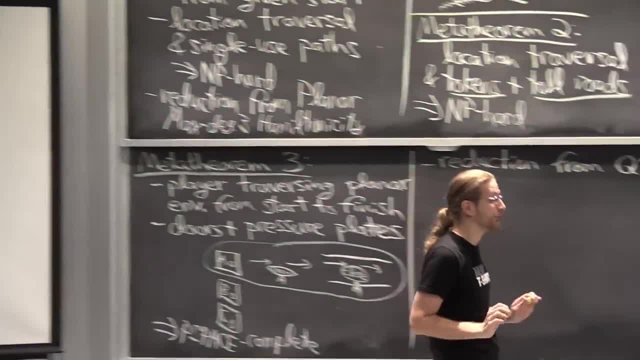 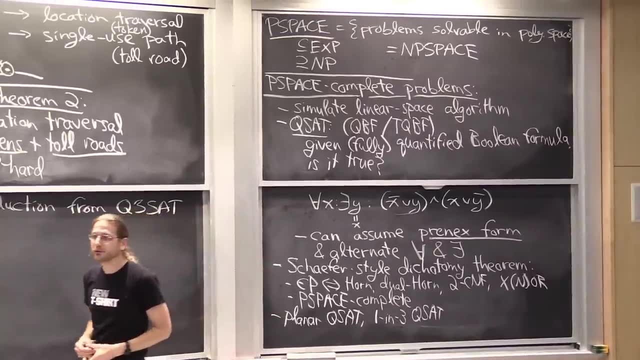 We're talking about NP here, So we don't need polynomial certificates, But the reduction itself is polynomial And again, of course, you need to preserve the yes-no answer. So that's our notion of reduction Question: Is there a way to make this reduction work? 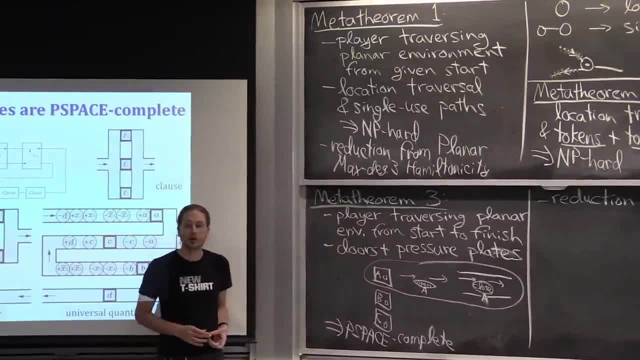 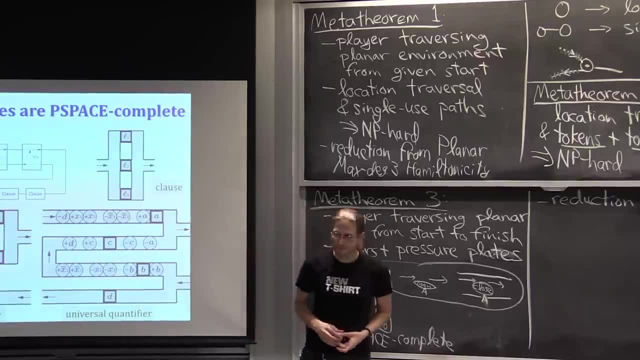 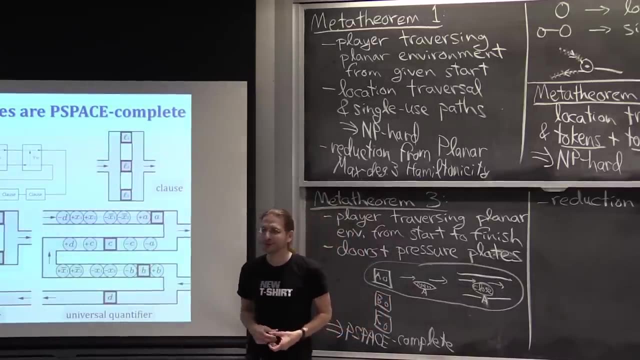 where you just have toggle plates so that they're not marked with open or closed, but just change the state of the door. I think let's come back to your question. I have a proof that does essentially that. I was wondering the same thing, but I'm not totally sure. 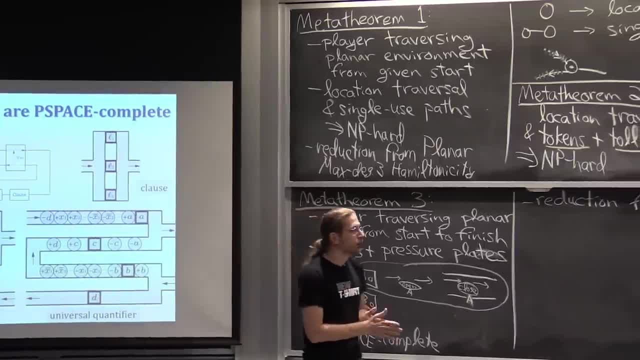 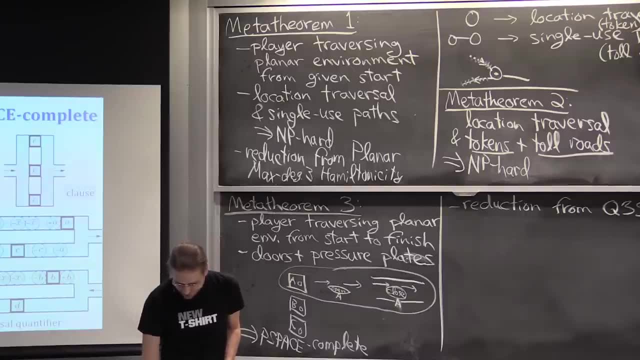 So let's come back to that and try to figure out the answer. So this applies to many, many, many games. Here is an example of an RPG: one of the earliest Eye of the Beholder, I think. it's officially D&D licensed. 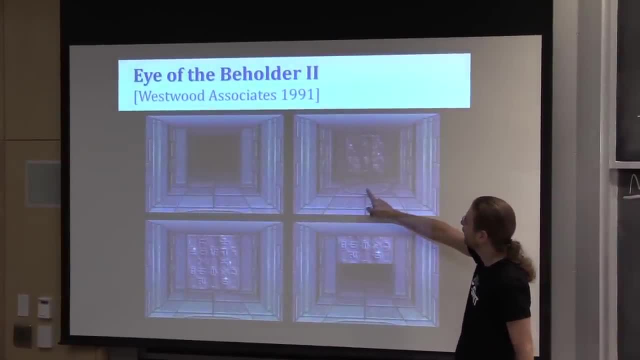 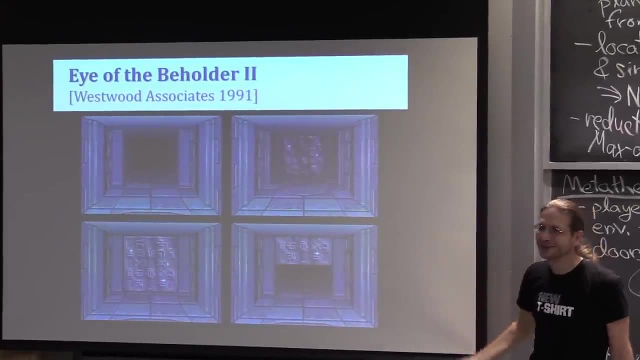 It has a small number of pressure plates. Here you are, You touch the pressure plate and this door opens. Ta-da, Not a lot of pressure plates. It's not a lot. I mean, we don't know to what extent these things exist. 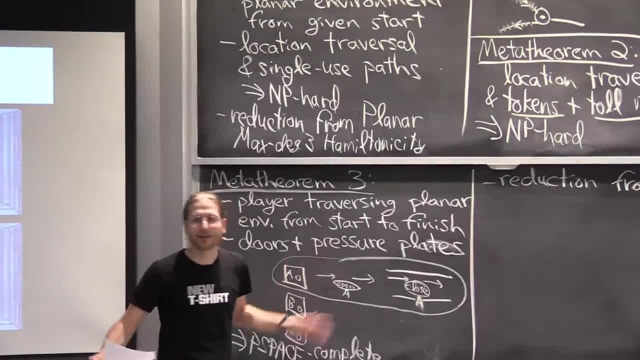 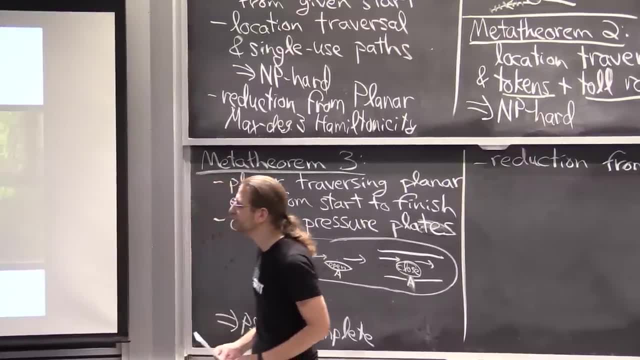 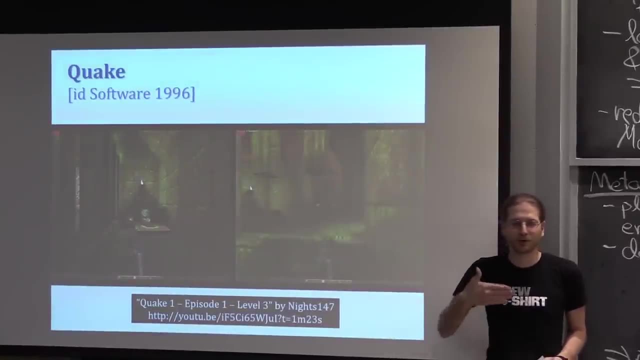 but reasonable to assume you have this kind of infrastructure and then PSPACE complete. even back in the early 90s A lot of first-person shooters have pressure plates. Doom doesn't have literal pressure plates, but it has triggers, just like walls. 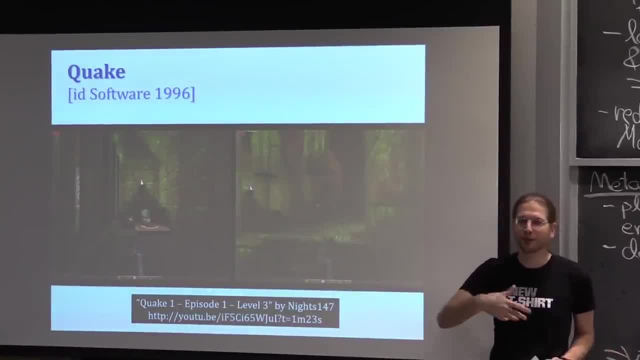 that if you walk through them, something happens: A block can appear or a monster can appear. If you make a block appear, that will essentially close the door. If you make a block disappear, which is also possible on the general script editor. 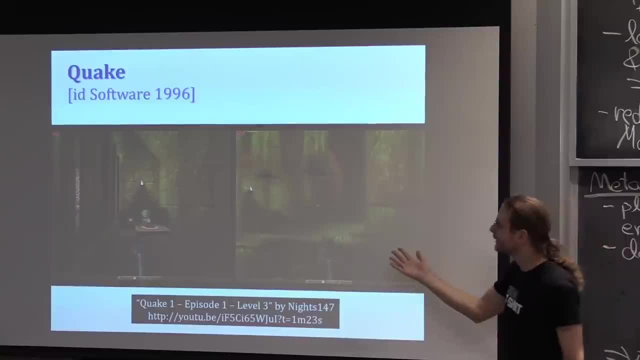 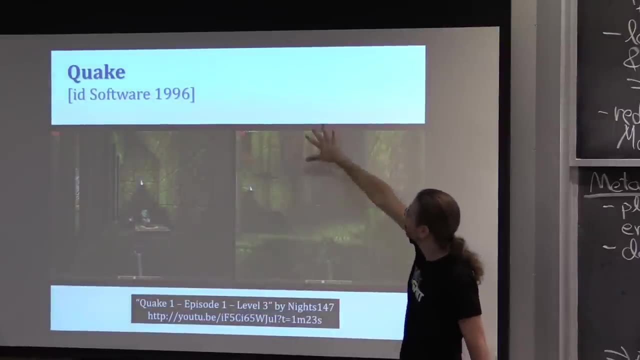 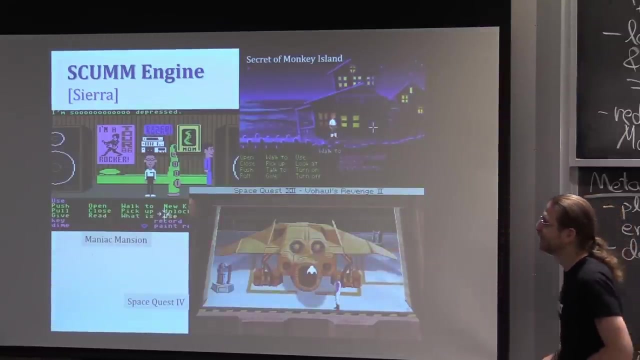 then you can do all this in. Doom Quake is the first one I know that has actual physical representations of a pressure plate. You touch this. It's a little hard to see, but this drawbridge is opening And a little more far, adventure games. 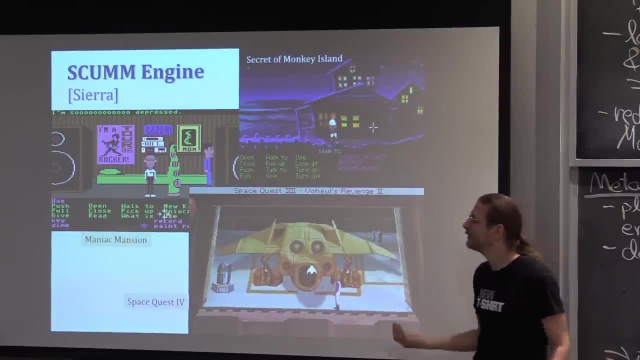 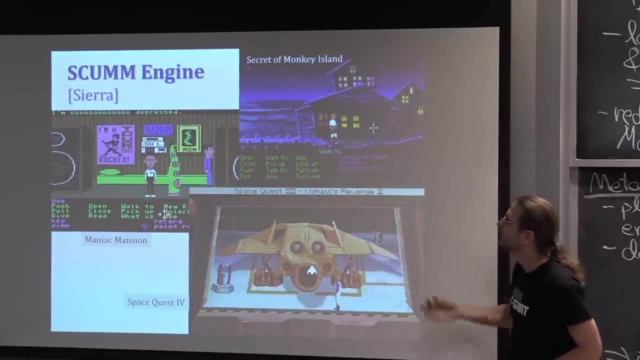 It's hard to define the generalization of an adventure game, but one definition is that there's an older engine for adventure games called SCUMM for all the old Sierra games. This, I think, stands for Maniac Mansion. That was the original game they wrote it for. 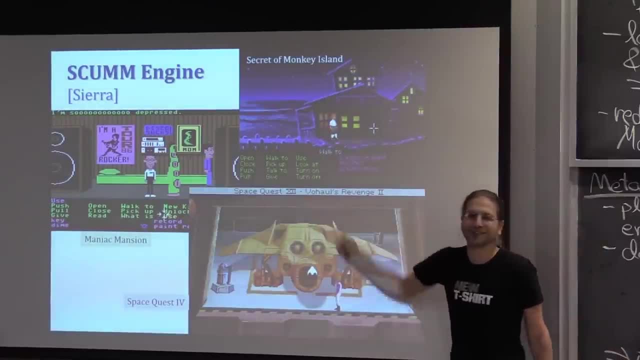 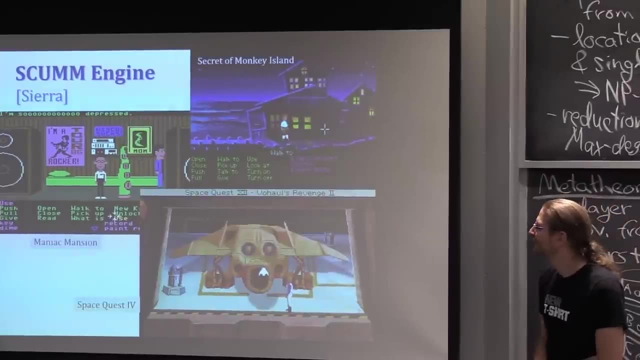 But if you've ever played Monkey Island or Space Quest 12,, which doesn't exist, but there was Space Quest 4, where they time traveled to the future and played Space Quest 12.. It's a very good game, by the way. 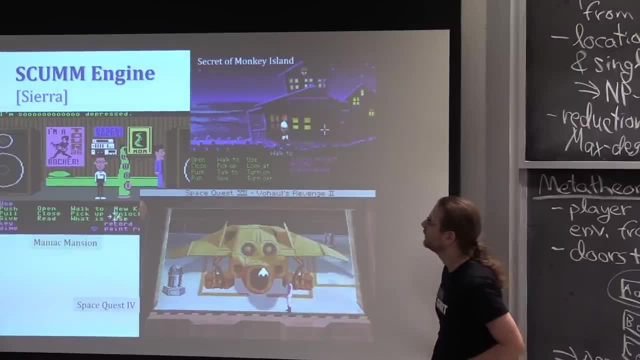 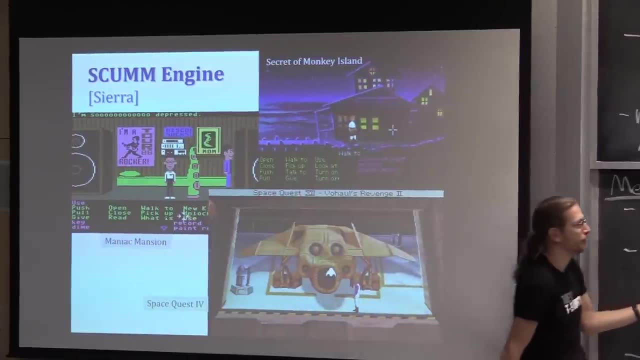 A lot of these are actually freely available now. And anyway, it's an engine. It has a very restricted set of screens, It has scripting languages And in particular it lets you do effectively the style of pressure plate things, where if you talk to someone then they. 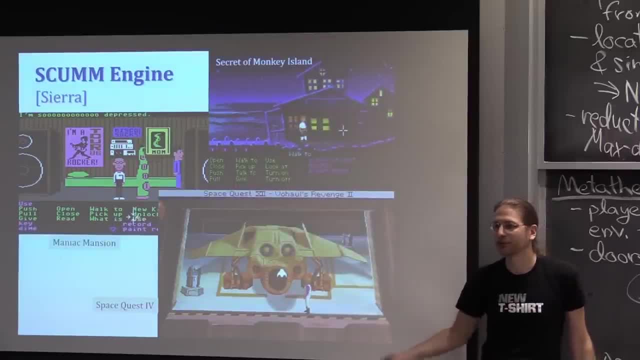 make you go to a new place and they open up some other traversal options, or vice versa. So you have to take this a little bit liberally, but you can essentially implement these kinds of things because you have rooms Here, you don't even need planarity. 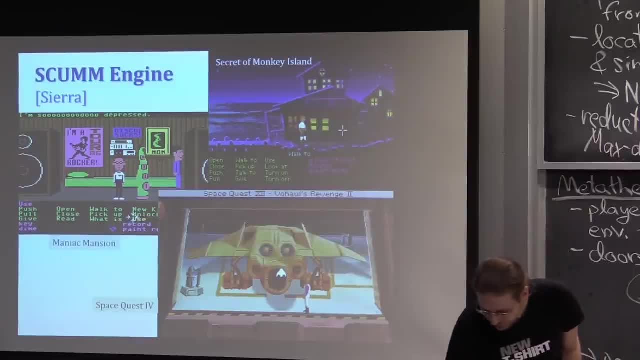 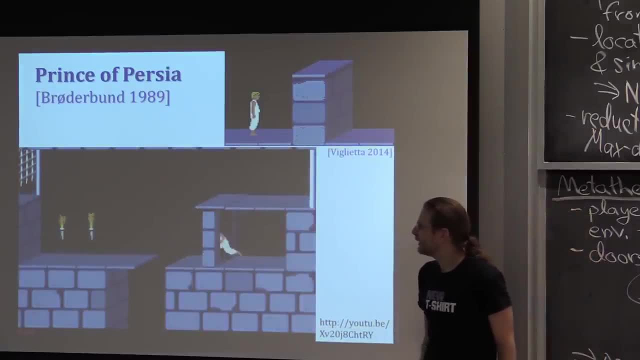 and you can implement pressure plates. So that's cool A little. more literally: pressure plates, Pressure plates, Pressure plates. Prince of Persia, one of the first platform PC video games, I guess I don't know exactly the right qualifiers. 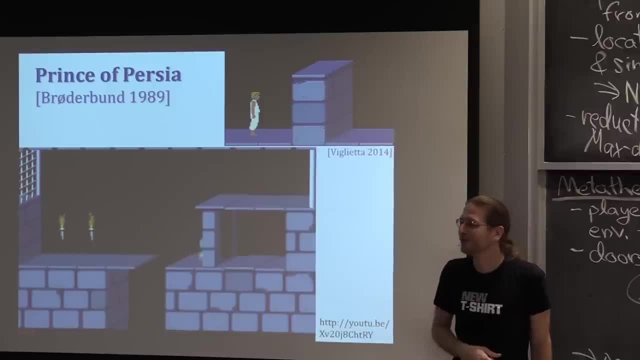 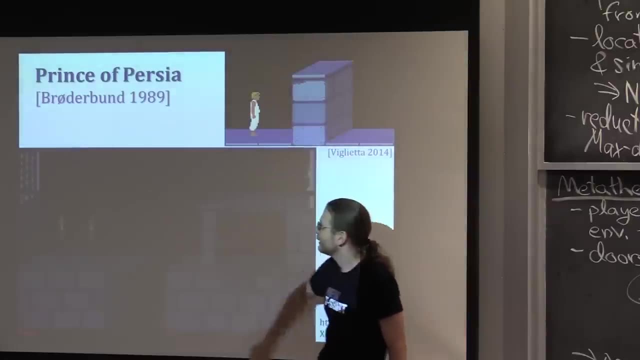 This. I think they even did motion capture. It's one of the first instances of motion capture for video games in very early days of graphics And you see, in particular, this was a pressure plate, literally that opens up that door. 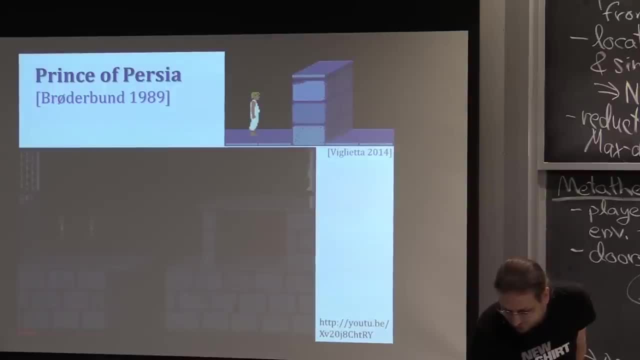 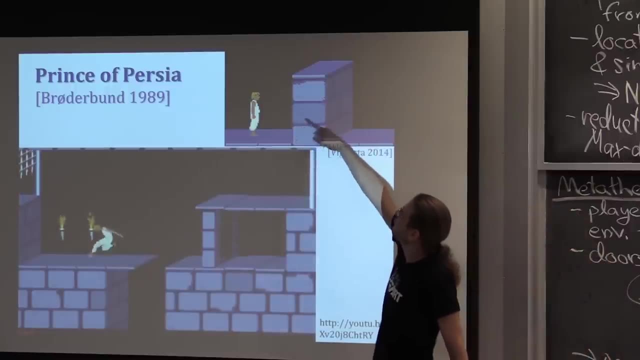 So that's pretty cool. One catch is that pressure plates in this game you can jump, So maybe you skip a pressure plate. If you put a pressure plate on the top of a ledge that you have to climb up, that will force you to touch it. 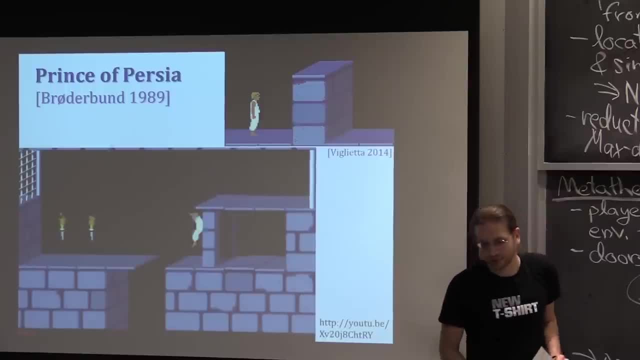 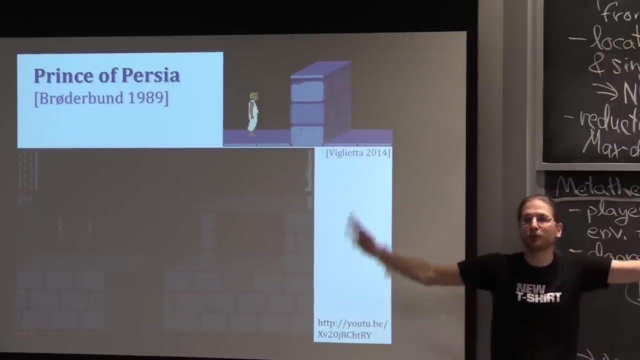 So that's Prince of Persia, PSPACE, complete. All of these games pretty much are in PSPACE, because the state of the game is some polynomial space thing which things have been pressed or opened or closed. The total space of the game is usually polynomial. 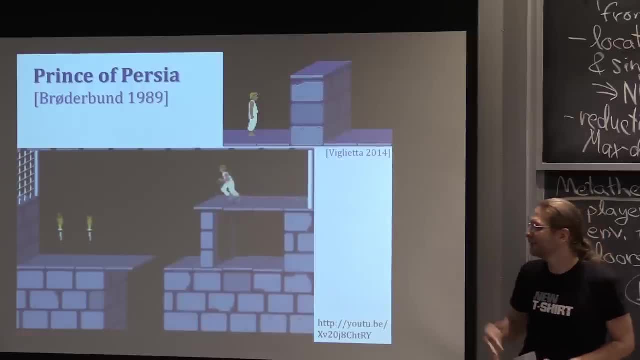 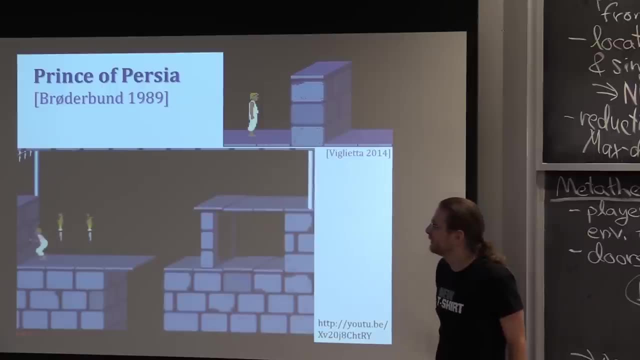 Each thing has some, at most linear, number of bits of state, So the overall thing is polynomial, Or should I say constant number of bits. That doesn't matter, I get to take a log And so you're just traversing this giant state machine. 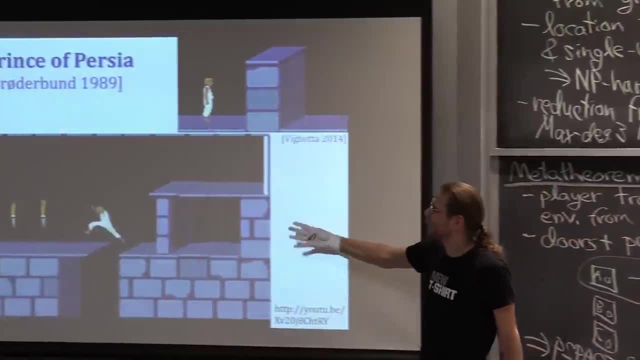 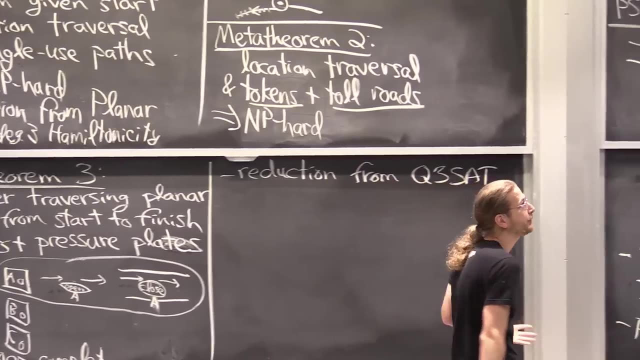 But because to store the current state of the game only requires polynomial space and at best you're making a nondeterministic choice at each step of whether I push this button or that button or wait as long as you discretize time. 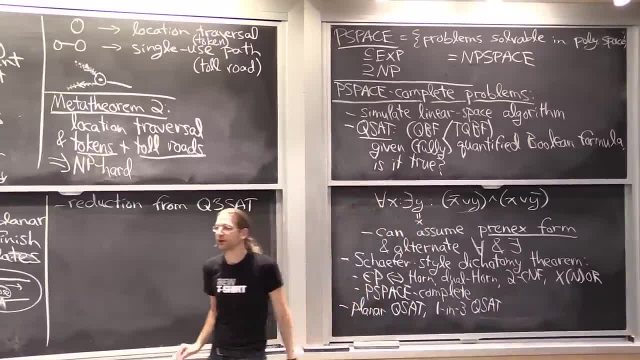 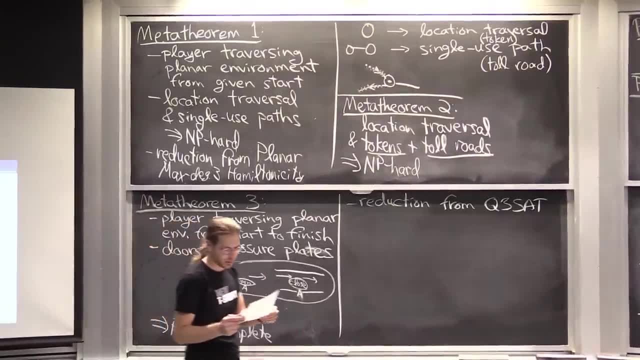 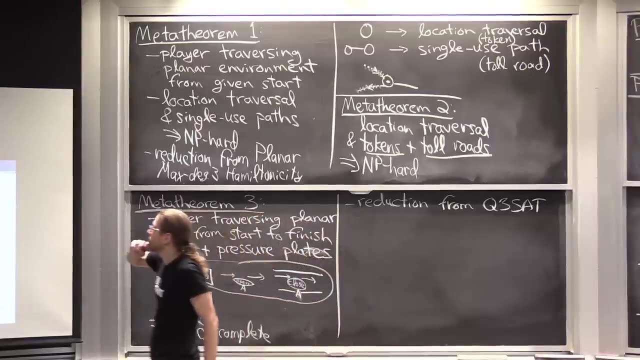 you get an easy NP space algorithm for pretty much all single player video games- Not quite all, but all the ones I've talked about. We've talked about here Cool. So that is metatheorem three. But this issue of having to force someone to pressure play. 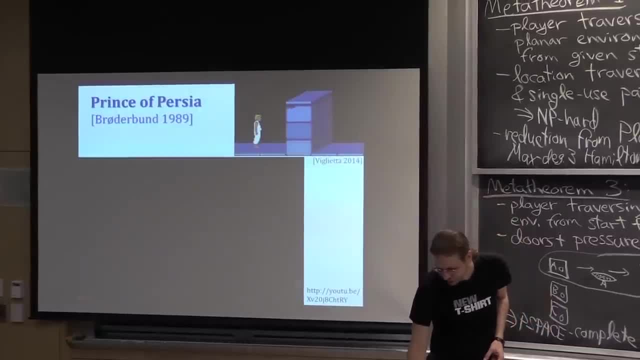 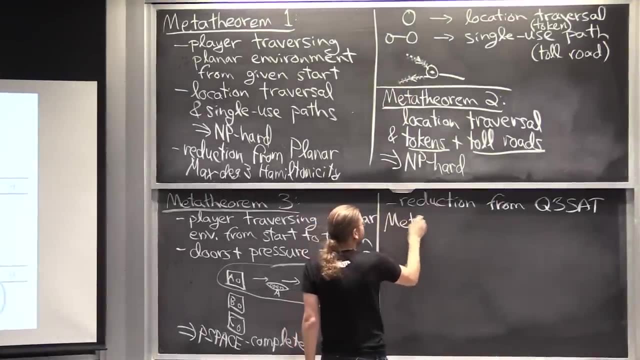 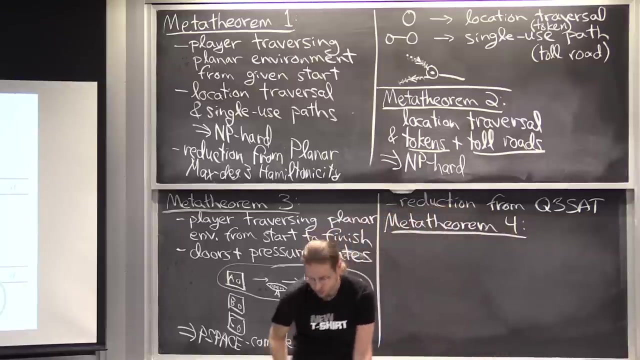 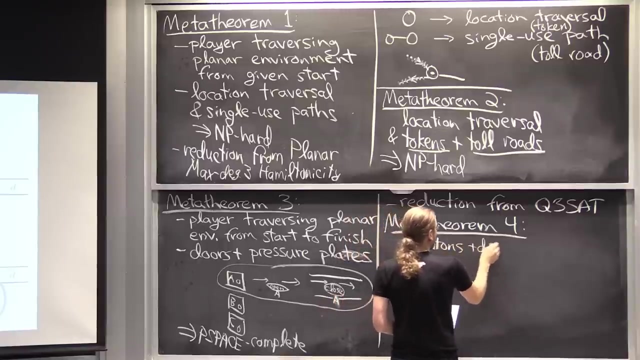 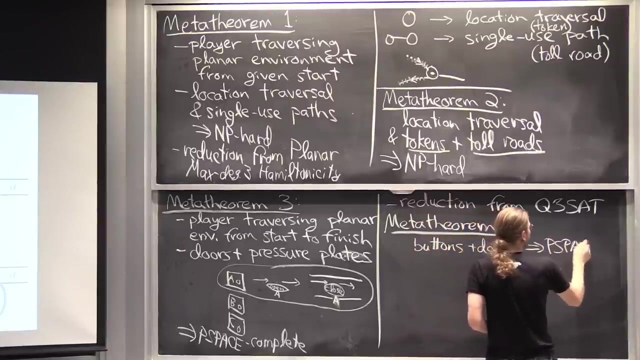 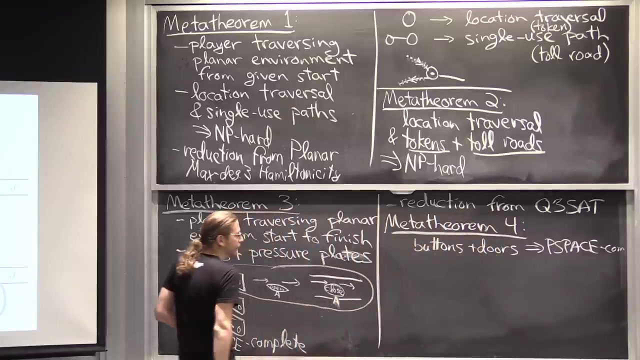 a pressure plate is a little bit restrictive And that you can definitely get rid of. And this is what Giovanni calls buttons in metatheorem four. If instead of doors and pressure plates you have doors and buttons, you get PSPACE completeness. 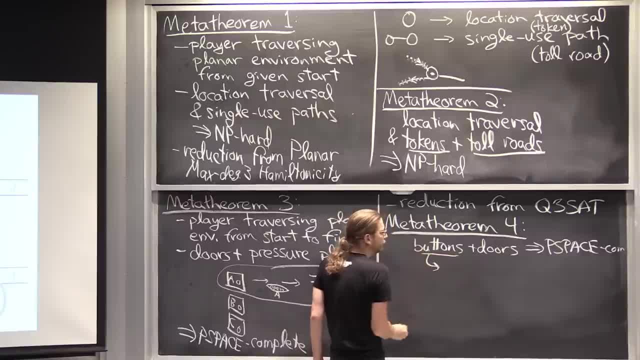 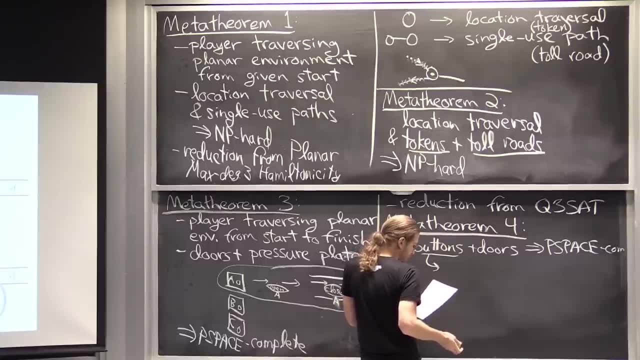 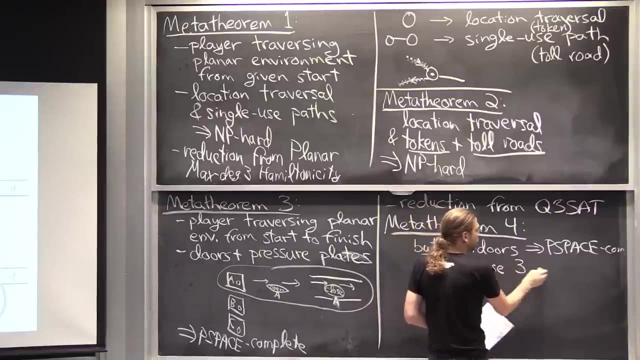 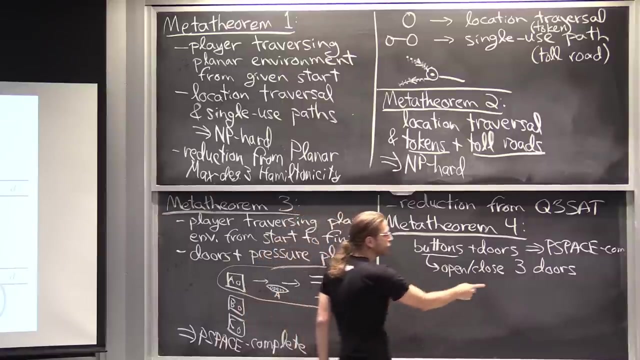 Now this is a little bit more restrictive in that we're going to allow a button to say open or close three doors. So pressing one button has a bulk effect. It affects three things at once. This has since been improved down to two, But that hasn't been published yet. 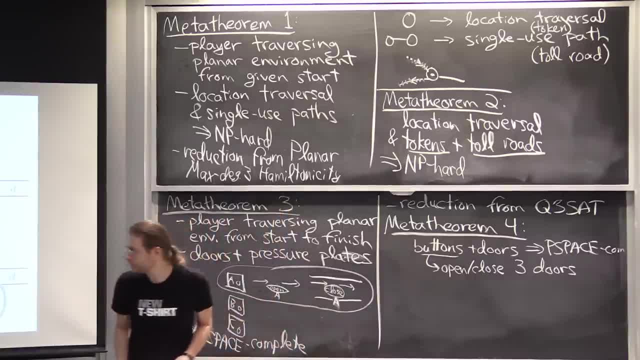 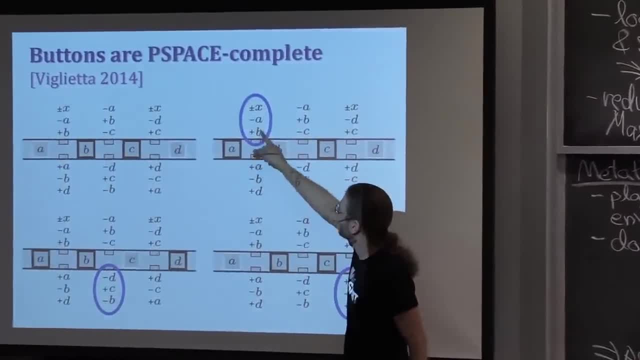 So I am going to cover the published version, which is this one Where you can see the button Where you manipulate three doors for every button that you press. And here we're drawing it with the buttons. on the sides of the walls There are many, of course, physical manifestations. 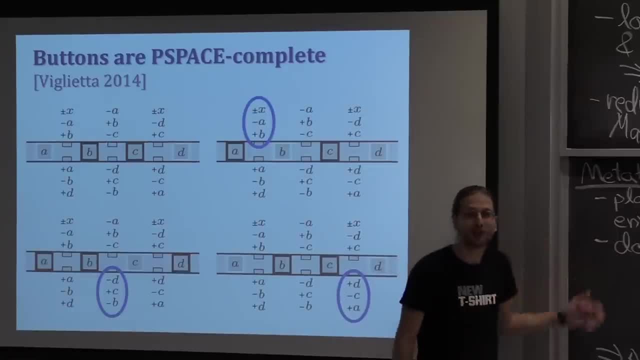 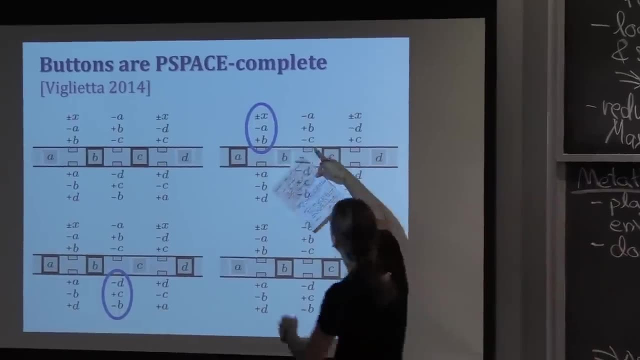 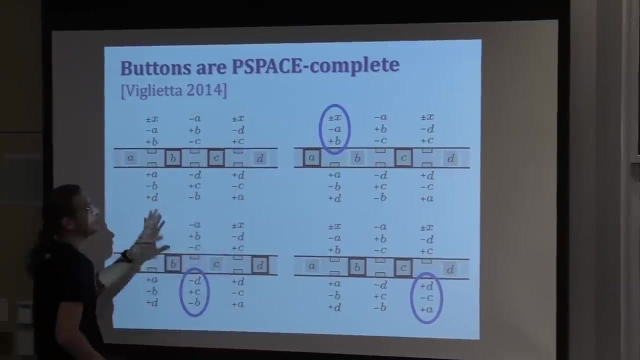 of this, And the proof is a reduction from pressure plates. Question: The buttons are allowed to close one door and open another. Yes, So you can see that here One button will close some doors, open others, And this is one gadget. 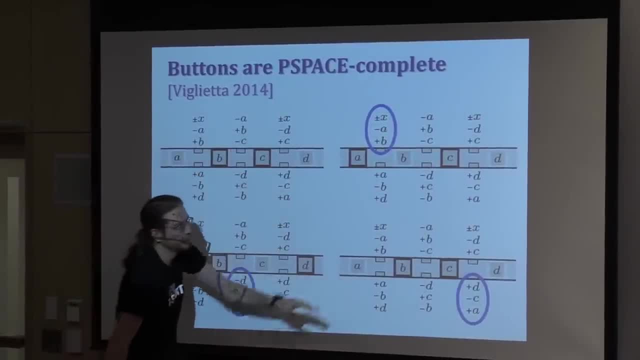 Just here's the gadget in the top left And this is a sample execution Going left to right. This simulates a pressure plate And in this case you can enter from the left and go to the right or vice versa, Although in the proof we actually 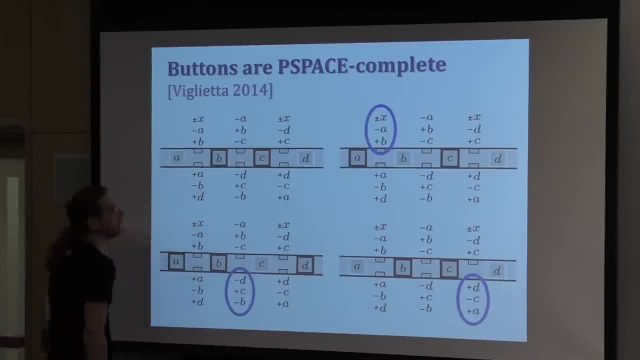 need one of those traversals So you could just stick with the top half of the gadget. So, and the white means open, The black means closed here. So the initial state is supposed to be: A is open, B is closed, C is closed. 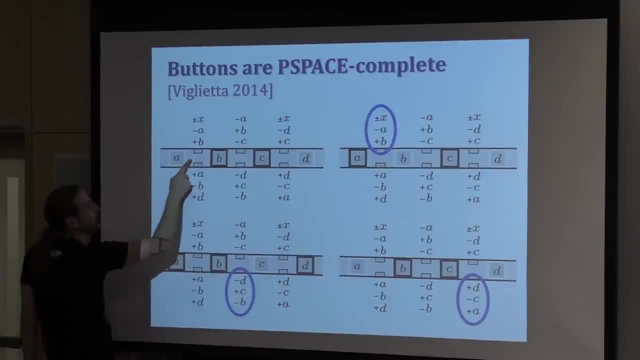 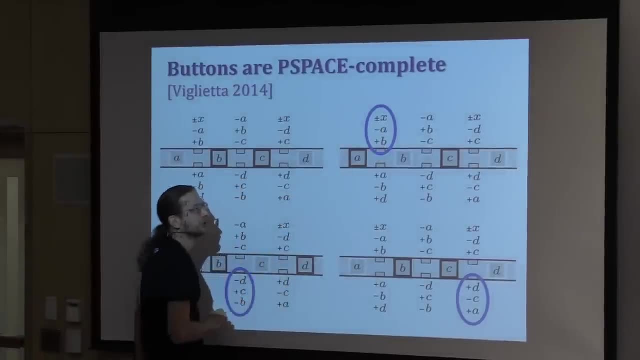 So you come in here. If you want to traverse, you have to hit one of these buttons. Let's say you hit the top one And we're going to do this plus or minus X, which is the actual thing you wanted this pressure plate to do. 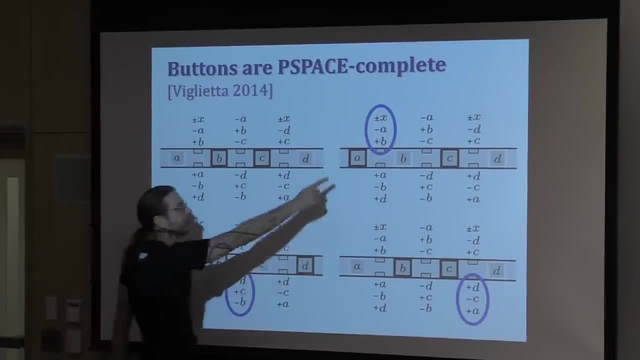 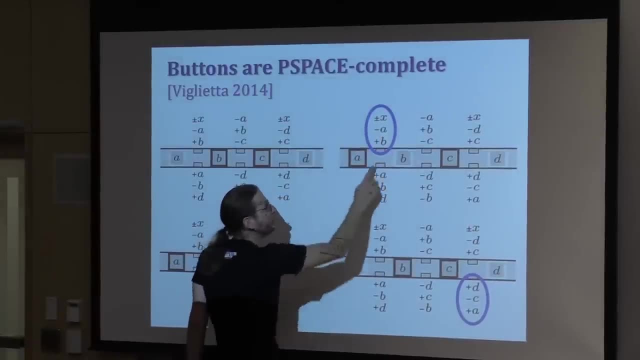 Open or close door X. If this was an open for X, there would be a plus X here, But then also we will close the door. we just came through and open the door to go to the next spot. Then you go to the next spot. 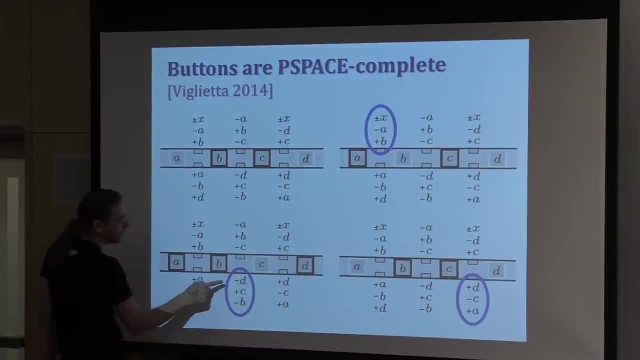 Let's say you press the bottom button And here you, because that opens C, you want to go forward. So that's the only one that opens C. This one would have closed C, But you're going to go to the next spot. 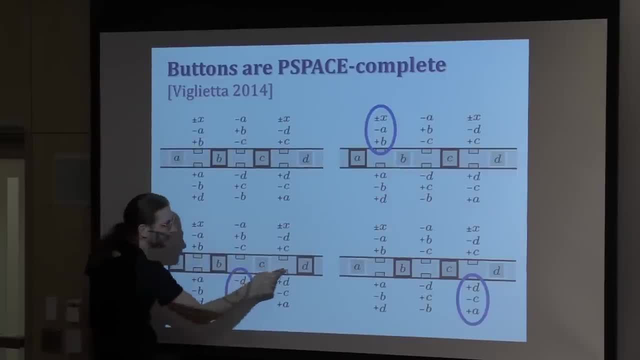 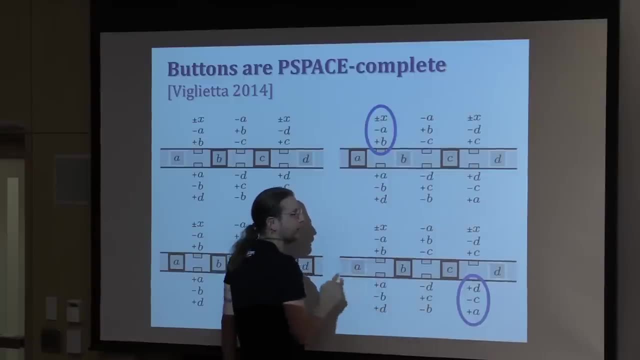 And we also close D and open B, which gets us to the next stage, And say: we press this button because this is the only one that opens D. Then we close C and open A. The point of that is to reset the gadget. 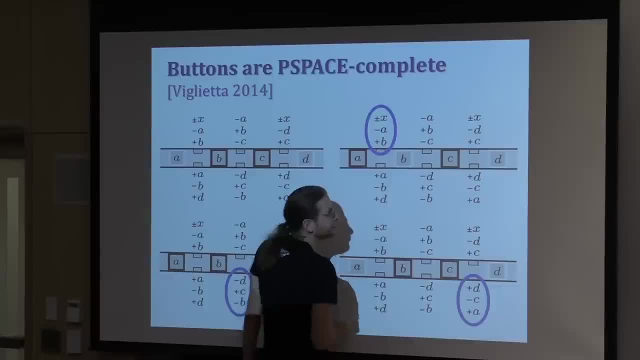 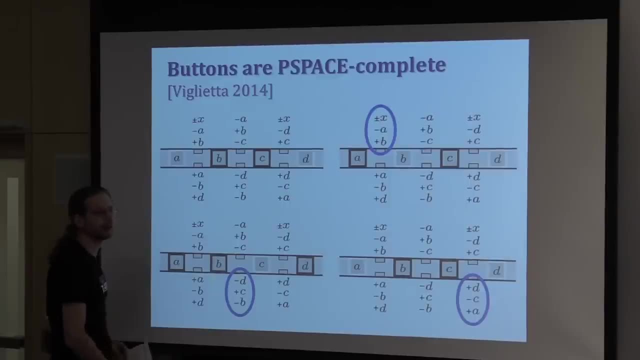 to its original state of open, close, closed, open, And then, along the way, we also activated X in the way that we wanted it to be activated. So that was pretty easy. Now we have buttons which you can press or not. 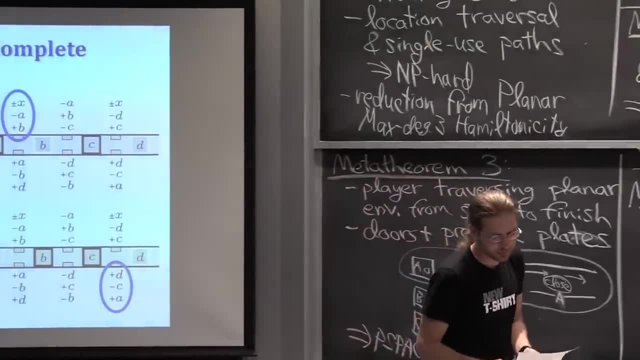 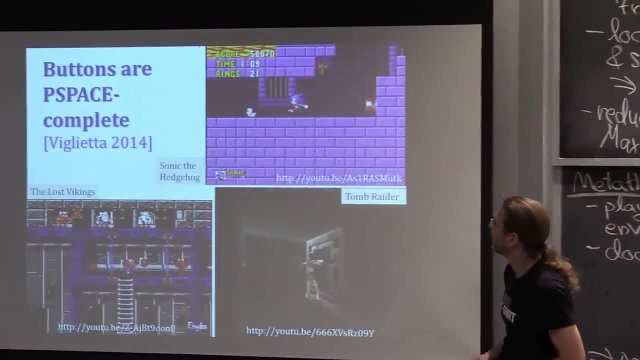 But when you press them it activates three things at once, And this also exists in many video games. Here were a few that I found. We have the original Tomb Raider And I think all the Tomb Raiders probably have some notion of Switch. 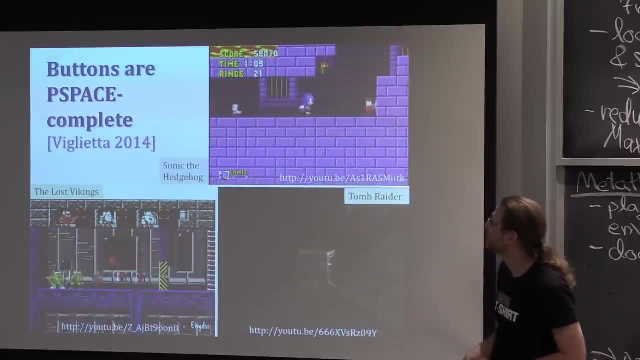 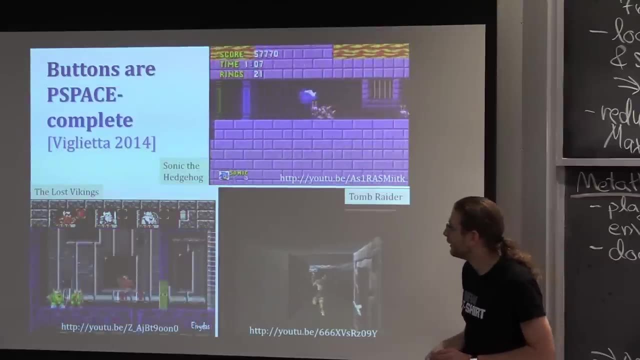 which opens in this case one door, But you can imagine generalizing to more doors. We have Sonic the Hedgehog here. When you press that button it opens that door. You can use that to simulate the same effect. And this game, Lost Vikings, which I barely remember playing. 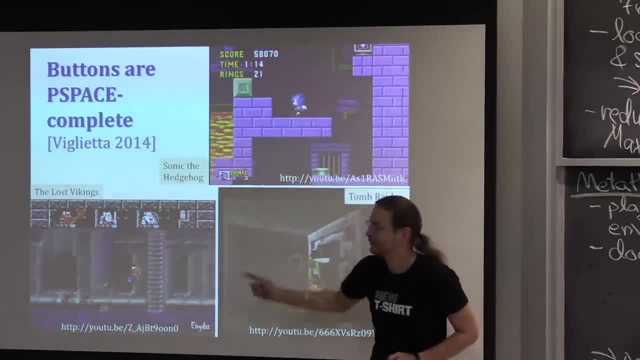 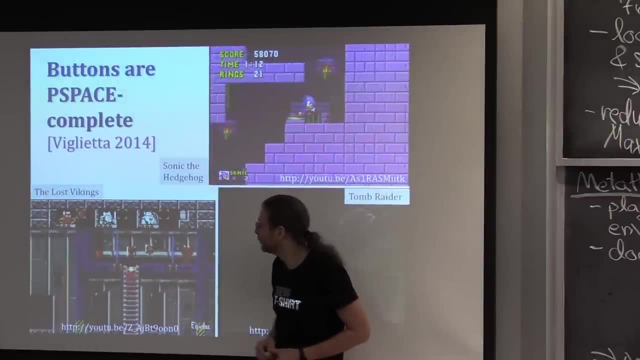 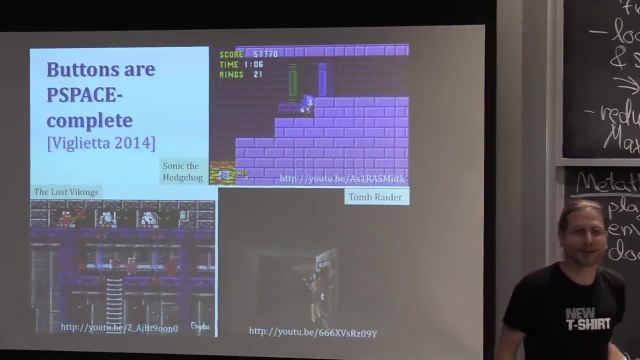 but I do remember in particular that the main character here is called Eric the Swift And you see him pressing a button which in this case actually opens two doors. So that's pretty compelling, And in general tons of video. I mean almost every video game with some puzzle element. 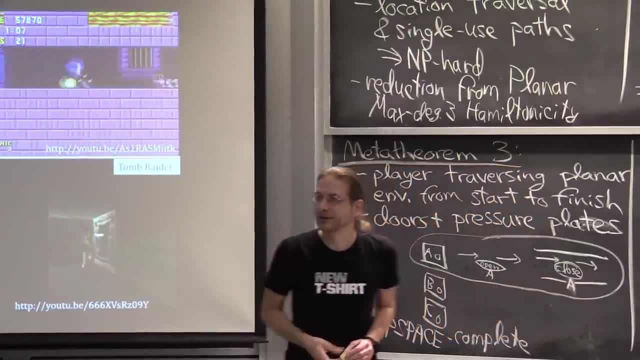 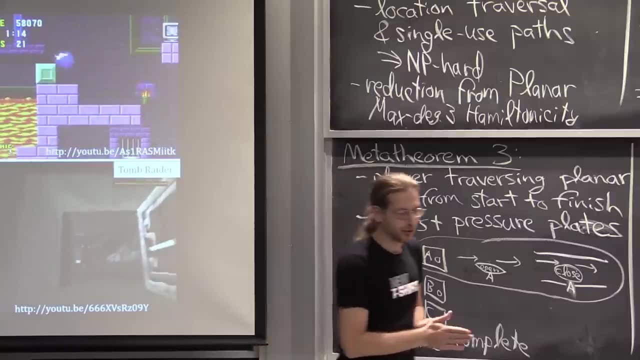 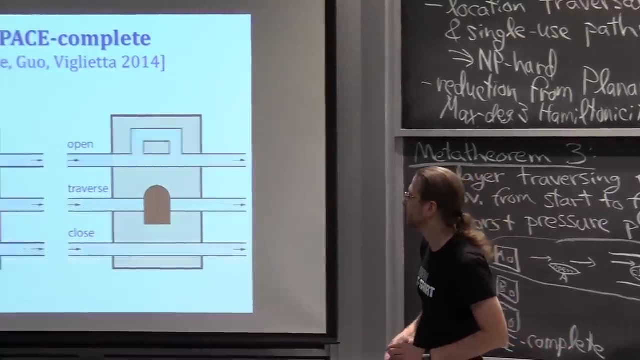 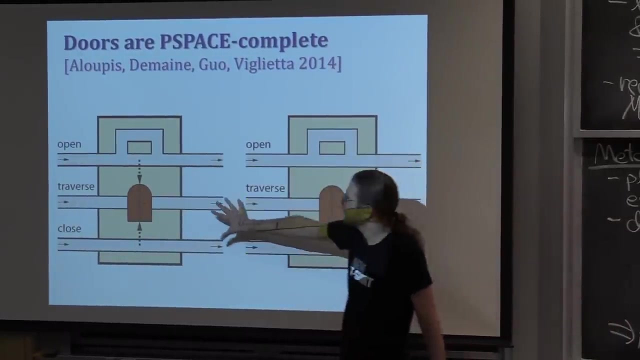 has buttons in it. So now you know a ton of video games that are PSPACE, complete Questions. All right, So the next meta-theorem is going to be a specific kind of implementation of that same construction. It's more of a physical realization of a door. 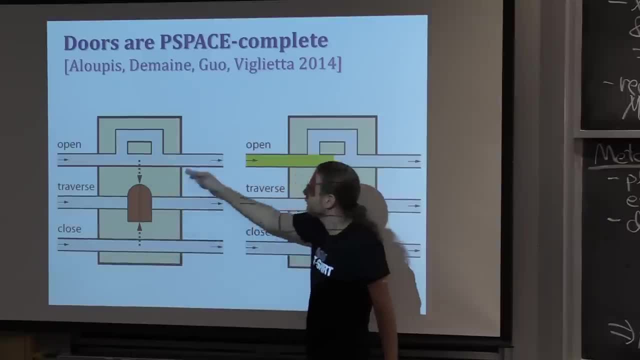 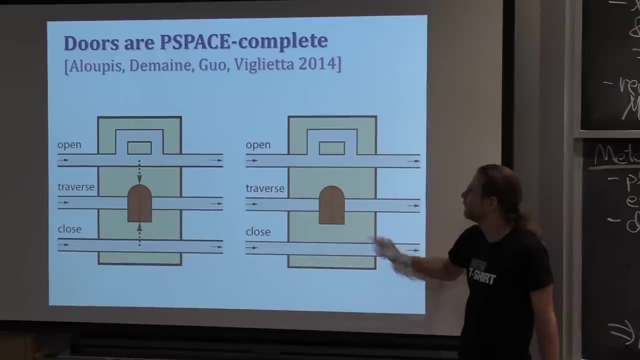 It's a door that can be open or closed, And it has various ways to interact with that door. If it's open, you can traverse through it. If you go through the clause connection, you are forced to close the door, in which case. 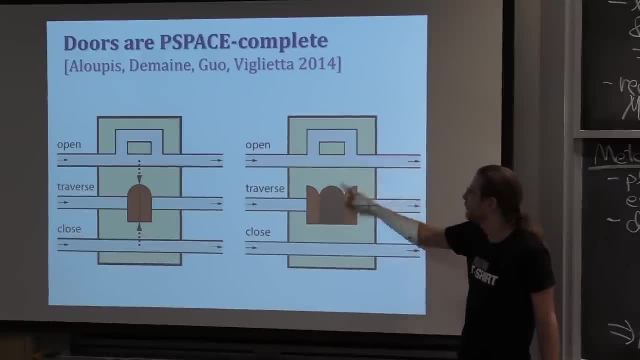 you can't traverse it. If you go through the open connection, you can either just go through or you can open the door if you want. That doesn't really. you don't need this connection, but a lot of gadgets will end up doing that. 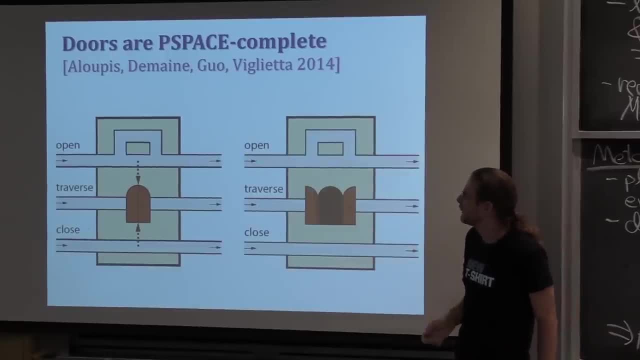 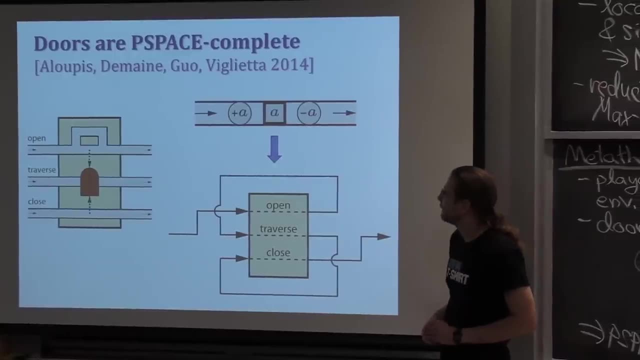 So this is just one bit of state doors- open or closed- And we can simulate this kind of thing or simulate the previous type of pressure plates. If you have a door and an open pressure plate and a closed pressure plate, we're. 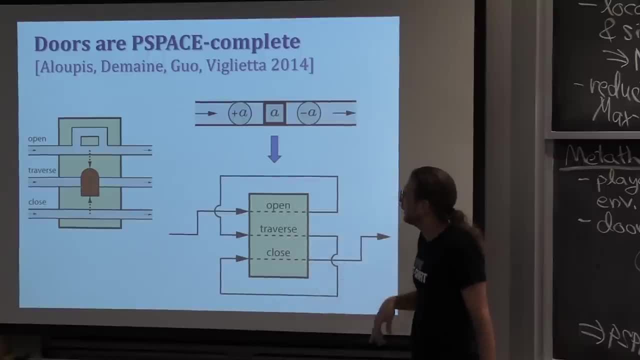 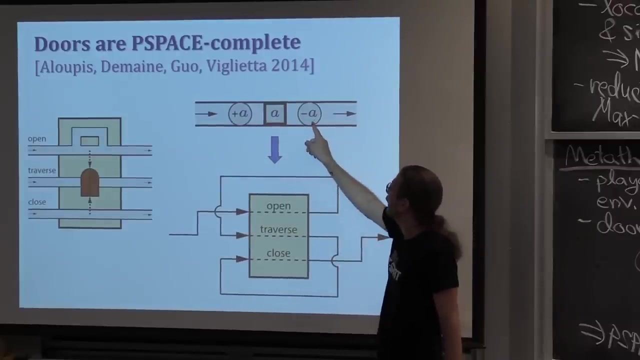 just sort of remapping that into this gadget, with when you go through the open traversal that's just visiting here And when you go through the traverse connection that's going through the door And when you go through the close connection that's visiting that pressure plate and vice versa. 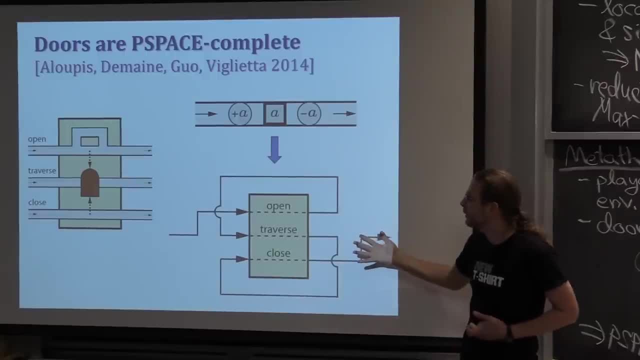 So you can take the previous reduction, translate it into this view. Of course you're going to end up with crossings and it will be kind of ugly, but you can do this. So as long as you have a crossover, gadget doors this. 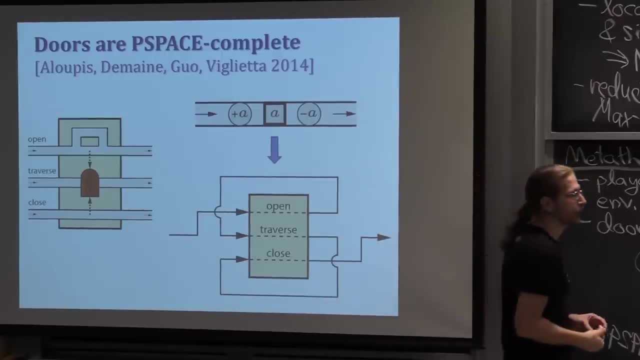 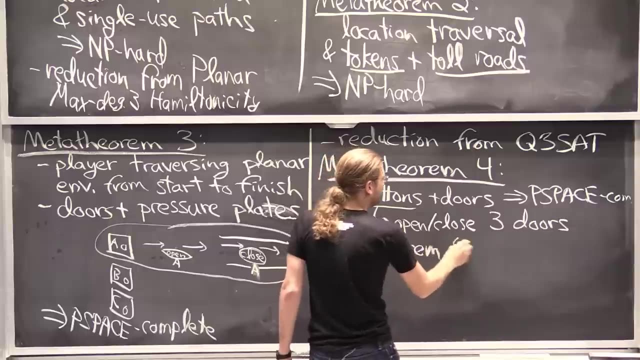 is called a door gadget by themselves are PSPACE-complete, So we'll call this Meta-Theorem 5.. I mean, this is very similar to Meta-Theorem 3, just like 2 and 1 were very similar, but just give it another name. 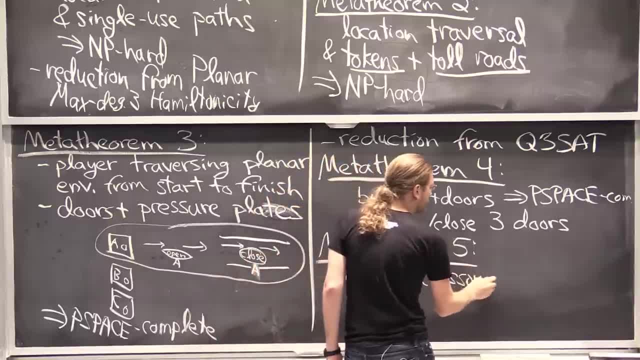 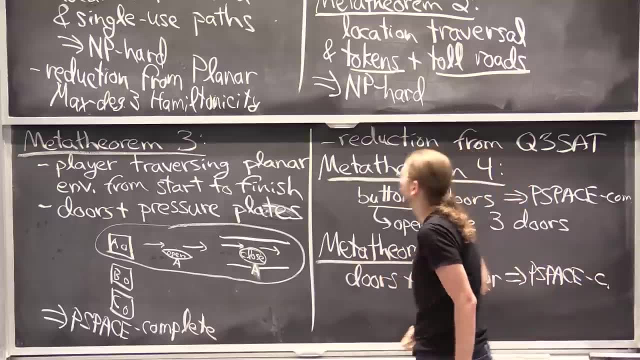 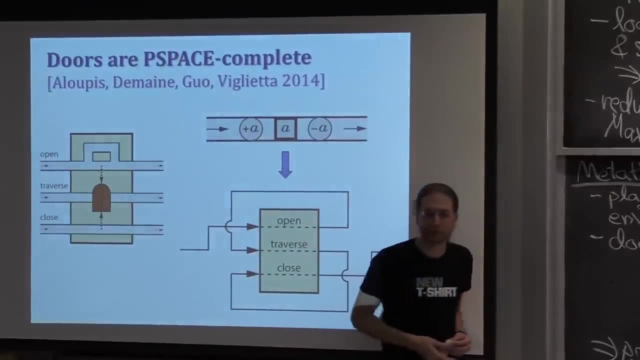 Doors plus crossover are PSPACE-complete- PSPACE-complete. So this is sort of a reinterpretation, if you will, of the original Viglietta paper. Viglietta is a co-author, but this is the Nintendo Games paper, So this is you can think of as a simplification. 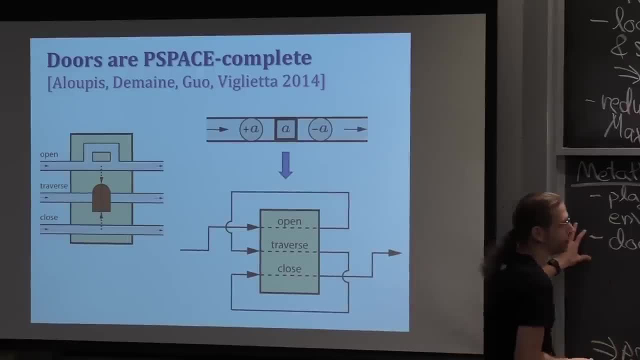 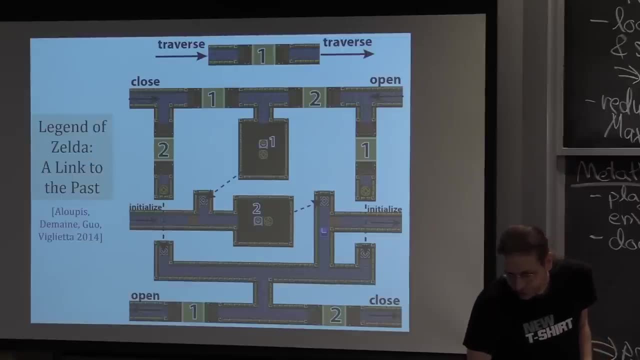 of that previous Meta-Theorem with pressure plates, And then that has been implemented in even more games than you've seen so far. So one of the first ones we did was Legend of Zelda, A Link to the Past. So a few things going on here. 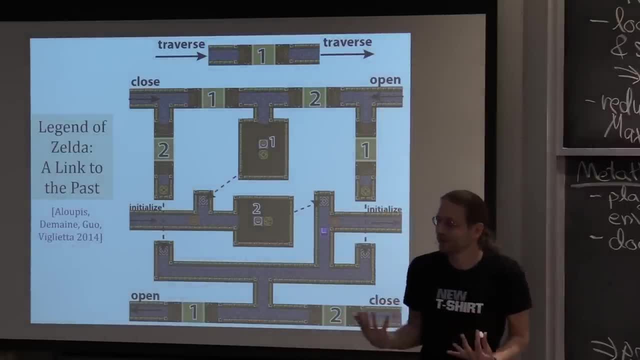 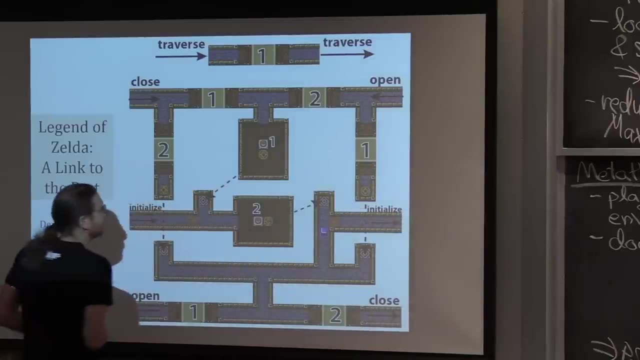 But this is basically the door gadget and then you're done. There are lots of ways to do crossovers in Zelda. That's not too hard. We showed a hookshot version some time ago, But anyway. so there are these notion of doors in Zelda. 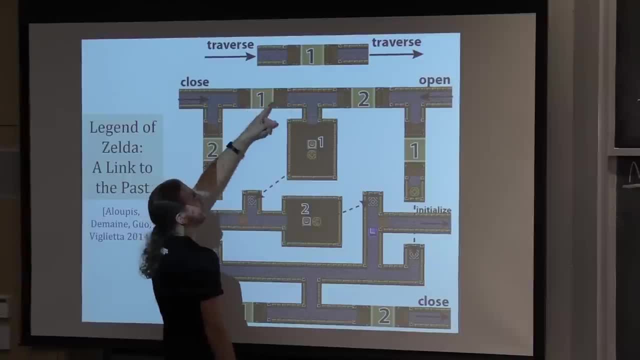 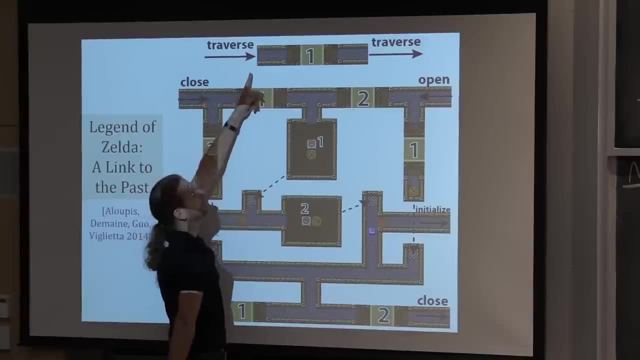 These are currently in the closed state. When you walk through this in the open state, you'd come out on the other side, And so, in particular, the traversal is going to be whether this door is currently open. Now getting back to the question in Zelda. 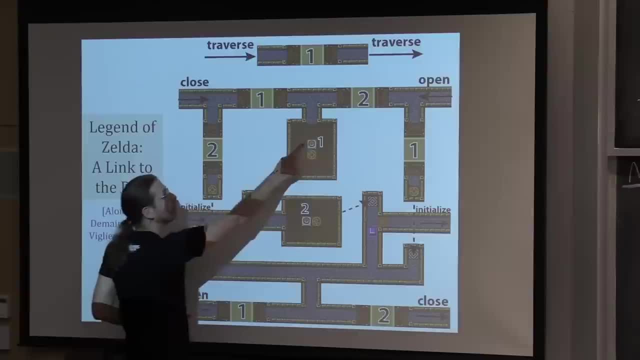 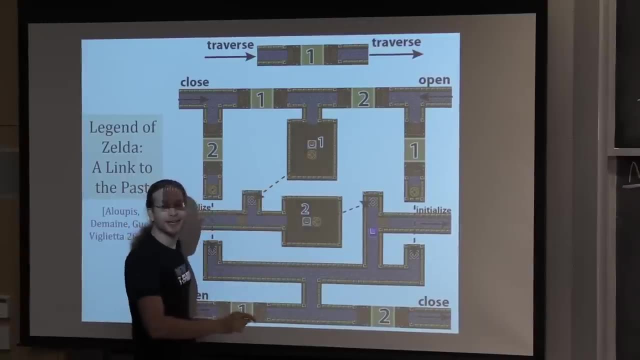 A Link to the Past. you only have toggles. If I press this button, all the doors labeled 1 switch state, But you can't jump and then land on the thing again. In this case you are falling down. The drawing isn't clear. 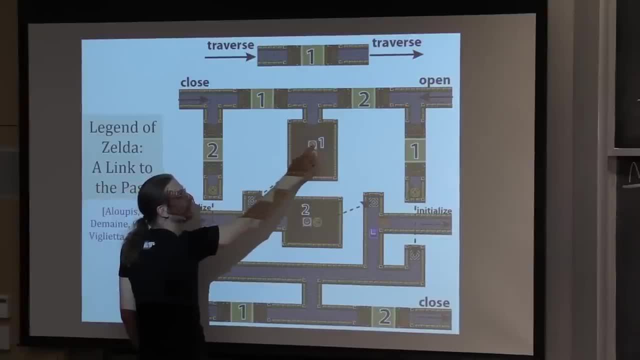 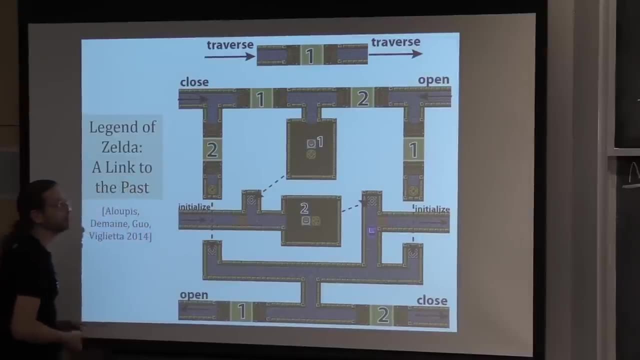 This is the 2D drawing of falling down a tunnel, And then the only thing you can do is walk down And then you hit a teleport and you immediately go Here. So this is one way to get traversals to work by preventing backtracking, getting toggles to work. 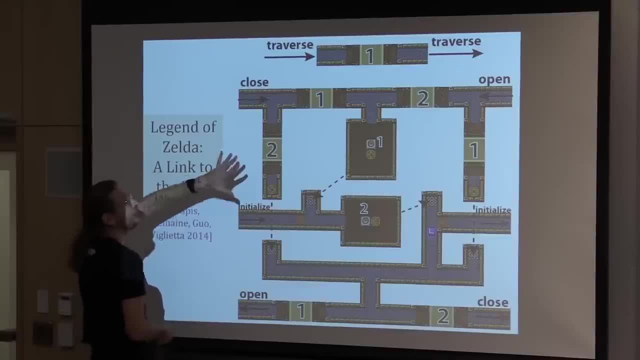 by preventing backtracking. So the intent of this gadget is: there are doors labeled 1 and 2. And it should always be exactly one of those is closed. Either the 1 is closed or the 2 is closed, but not both. 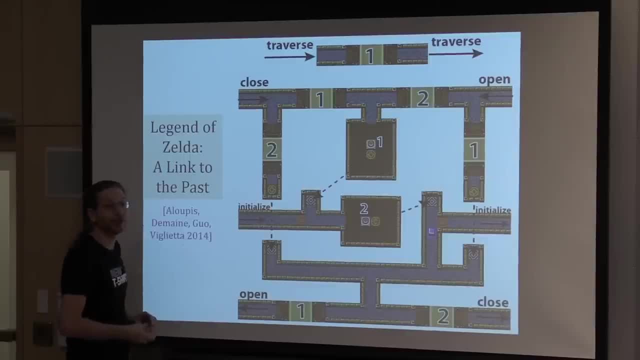 And in Zelda, all the games are initially closed, So this is annoying. So we have to build this. This is an initialized gadget through all of these doors. When you come in here, this is the end You can only go from. these are one-way teleporters. 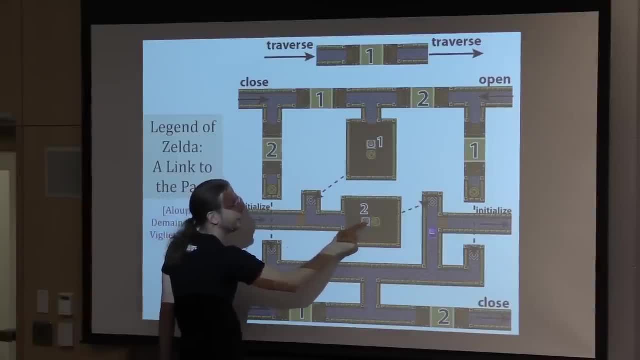 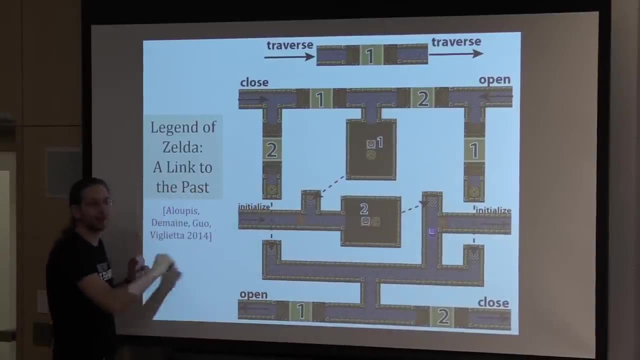 You can't go up here, So you have to go here, toggle 2, then go to this teleporter. go here. This is a block, so you have to go over. this way, We're going to chain all these gadgets together. 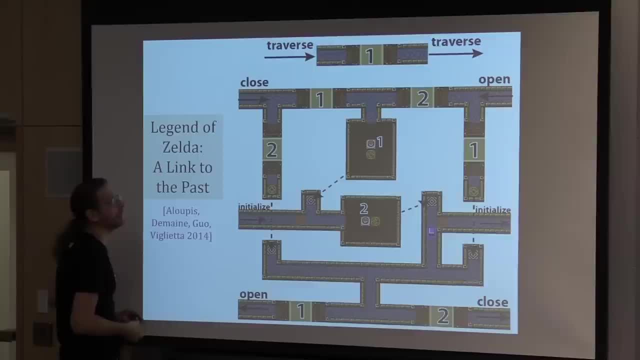 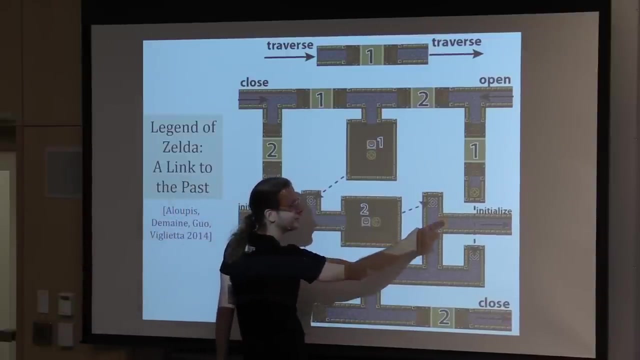 through these initialized paths so that all of the doors are initially in the closed state, with 1 closed and 2 open, And then there's a Crystal, something that you can break, And it flips. All of these blue blocks become these and all of these become blue blocks. 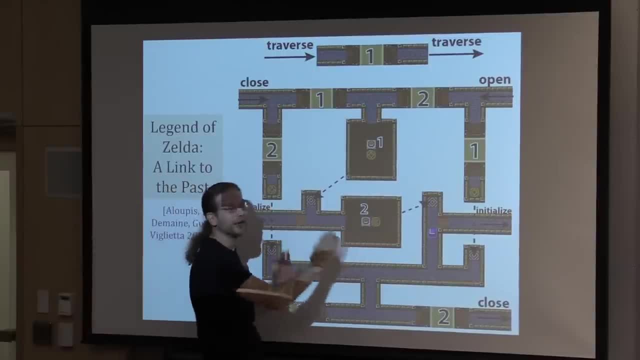 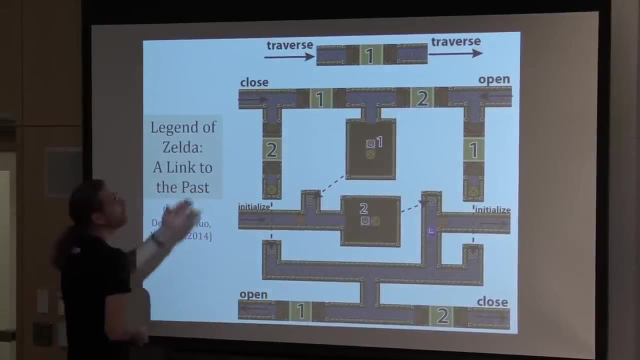 And that only happens once. So now, basically, the initialized paths are destroyed. So now, think of this as being untraversable and this is traversable. So now, if the door is open, door number 1 is open, then we can traverse it. 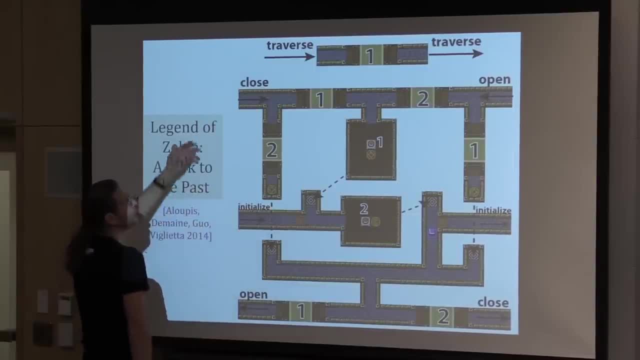 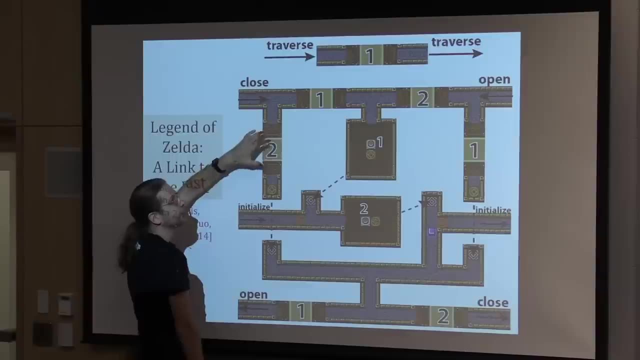 That's cool. Let's look at the closed paths. The closed path- exactly one of these- is going to be open. So if the door was already closed, that means 2 will be open. We go down here, We teleport to here. 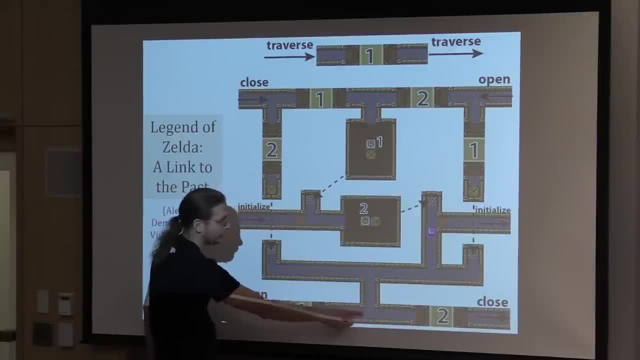 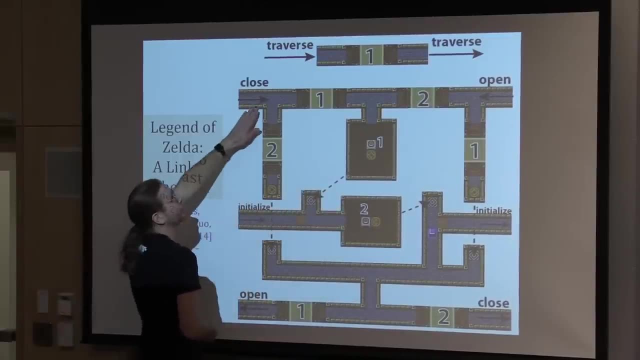 And then again, because 2 is the only thing open, we go out through the closed exit. On the other hand, if the door was open and we're trying to close it, we have to be forced to close it And indeed we'll go through door 1.. 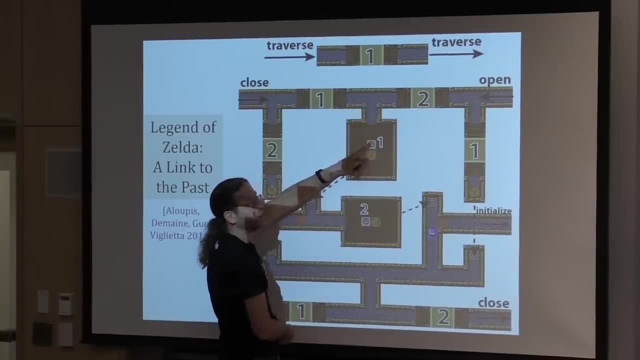 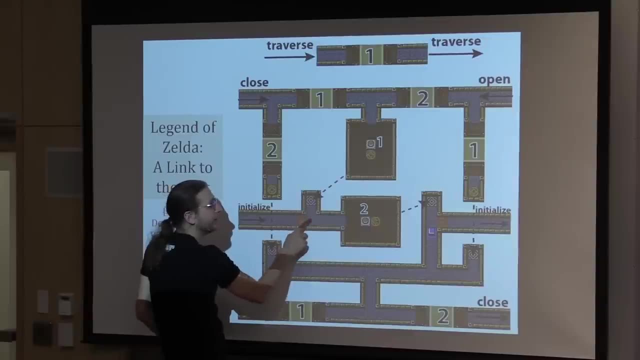 Can't go through door 2.. We'll go down here. We'll toggle door 1.. Now door 1 is closed and so is 2.. We'll teleport to here And now we are remember. this is blocked now. 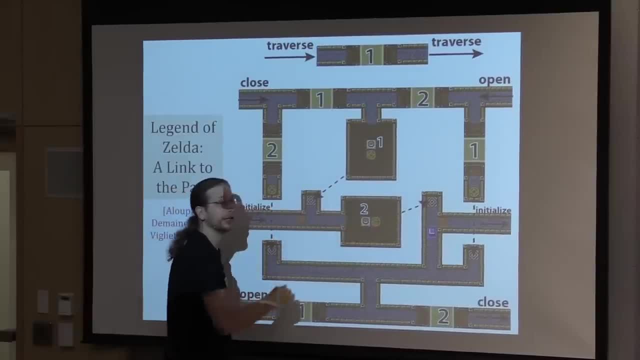 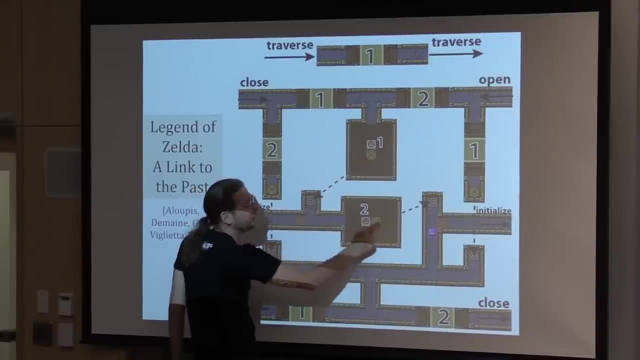 Now we're forced to switch 2 as well. So we're effectively simulating the effect of doing two doors with one choice of a thing. First we flip 1., Then we flip 2., Then we teleport here. Then 1 was open. 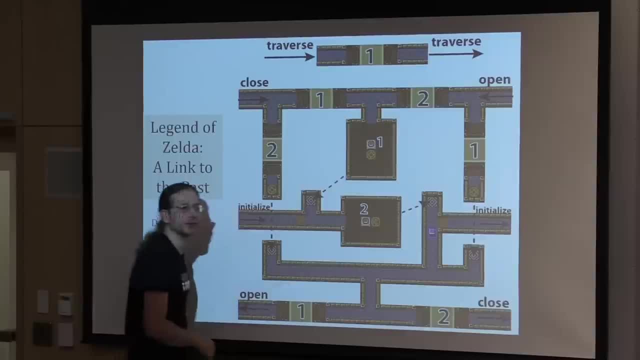 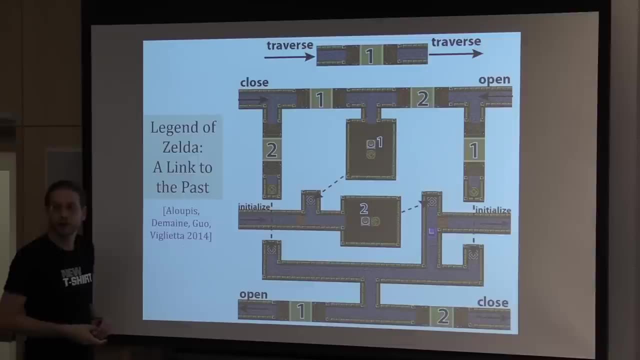 We flipped everything. Now 2 is open and we go out through the closed, So in both cases we exit through closed. Yeah, How do you ensure that the blocks only get flipped once, Because the crystals can be hit as many times as you want? 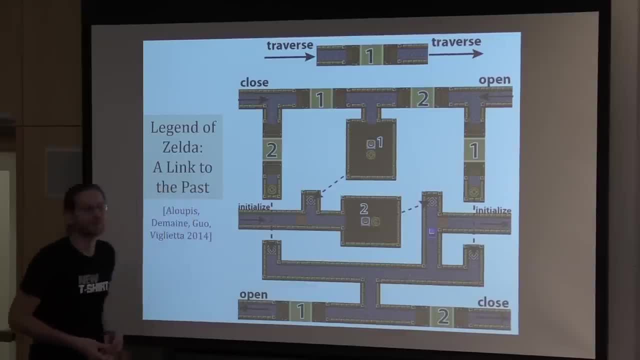 OK, So I had forgotten that detail. Essentially, we want to just put a one-way gadget. So when you hit the crystal, I mean either you hit it or you don't. But if you hit it, then we have a cliff. 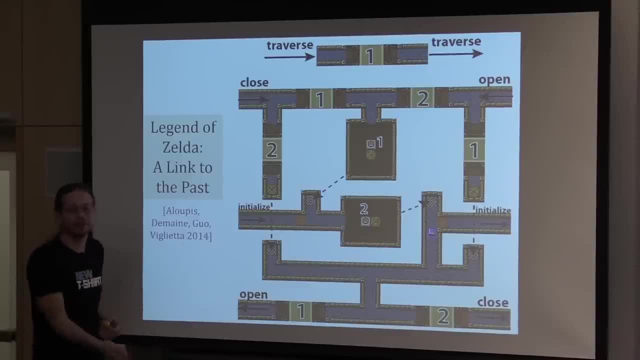 that you fall off of and visit the rest of the game. So you can't go back and flip the crystal. If you don't flip the crystal, then the gadget will break in other ways. If you didn't flip everything, you won't be able to traverse again. 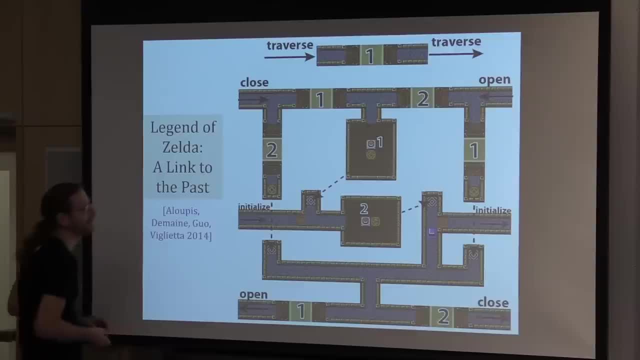 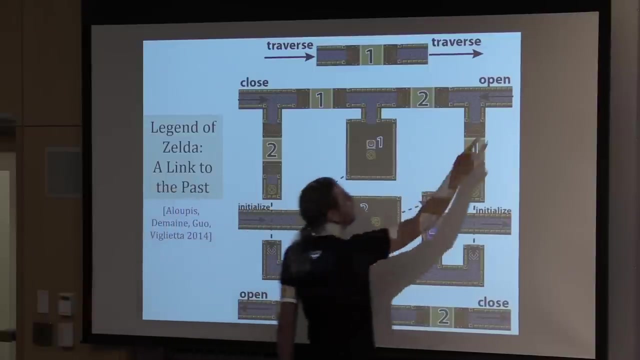 Yeah, I should have that drawn, But I don't. So there's just one crystal and it's hidden in between the initializer and the rest of the traversal. OK, So what haven't we done? The open case, So maybe we come in the open door. 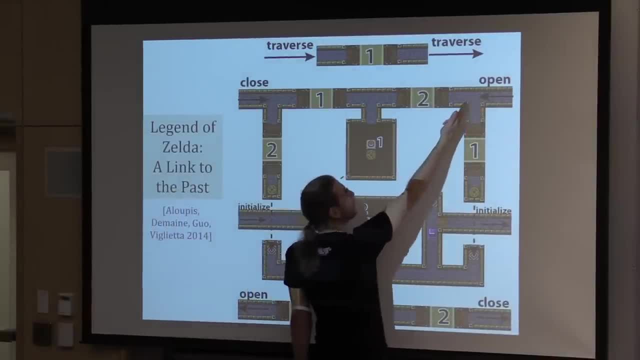 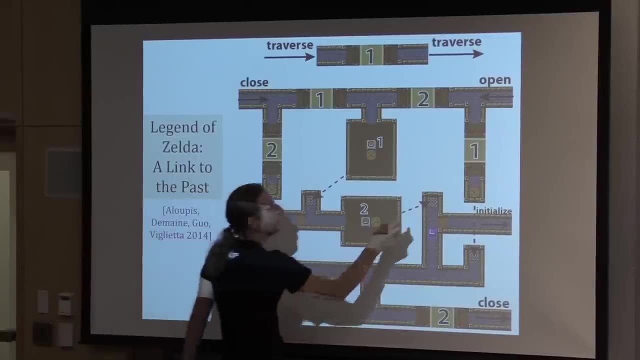 And here we have a. well, we're not going to have a choice. Either it's already open, then we'll go through here, teleport to here and we can go through the 1, and we're out, Or it's closed, in which case 2 is open. 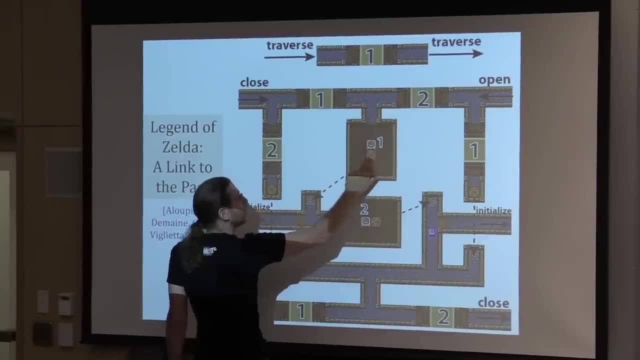 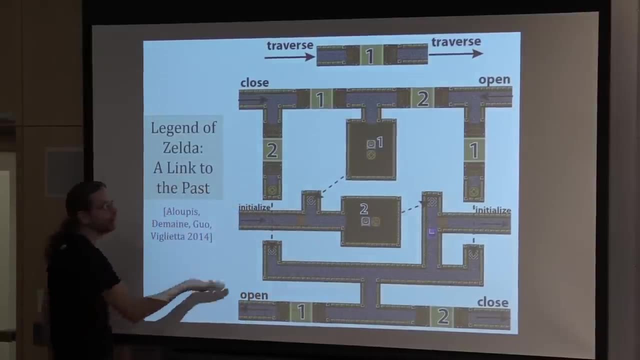 Then we can't go here. so we go down here, We toggle 1,, we toggle 2, and then we go out here And now 1 is open. So it's kind of cool When we're going through open. we. 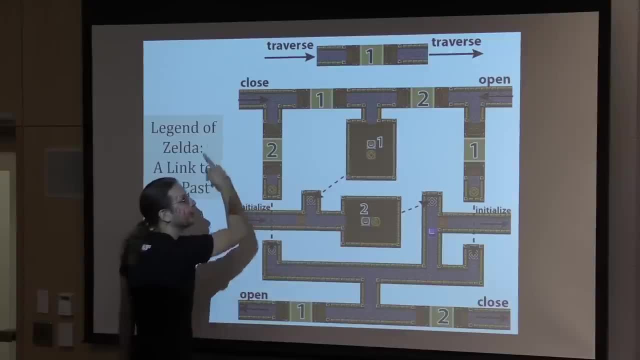 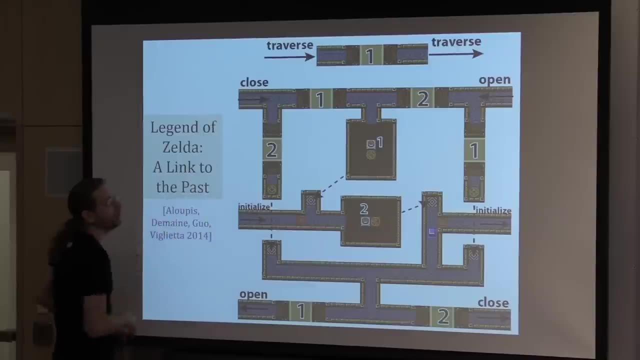 know that we'll end up opened, and so we'll go out the open And we go through the closed traversal. we know we will end up closed, And so we will always go out. the closed exit And traverse is just completely separate. 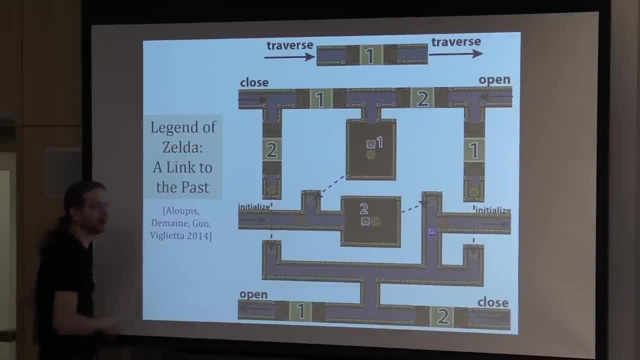 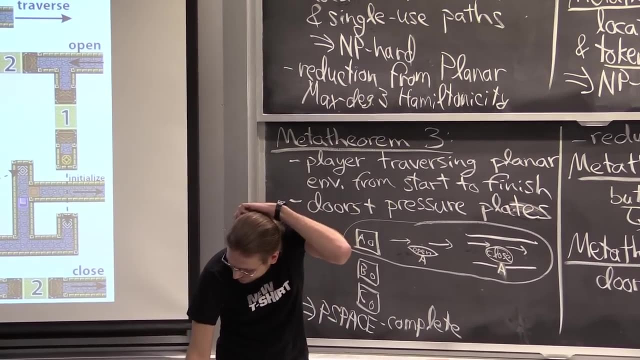 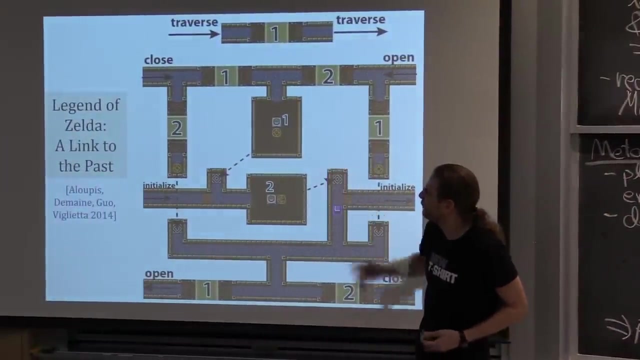 Cool, So this is a door in Link to the Past, Yeah, And so that's a good example of toggles And you can imagine setting, if you again have sufficient crossovers and so on, forced. I think you could argue this is more generally letting. 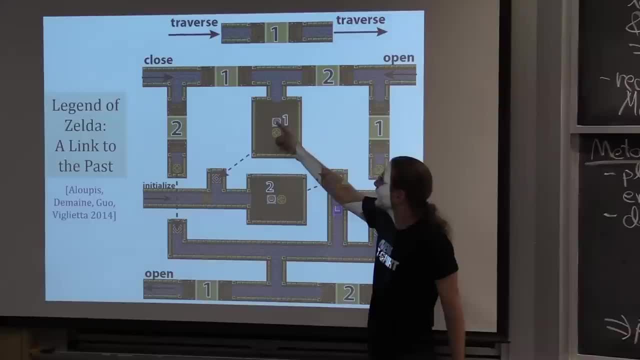 you deal with toggles. as long as you can, right next to a toggle, put a after traversing it, you essentially have, say you have a one-way gadget before and after it. in a certain sense, Here in Zelda there's only two levels. 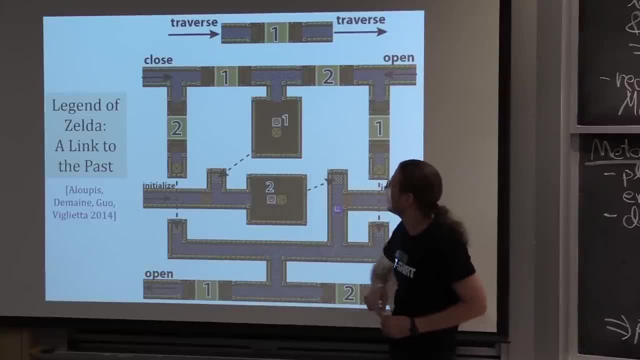 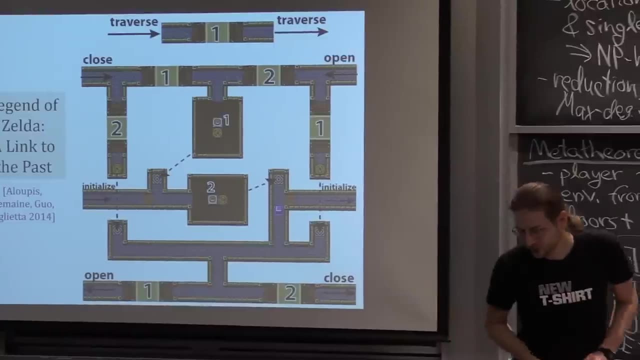 So we can't make you fall off another cliff. But it's the same thing with the teleporter: We have a one-way right before it, one-way right after it. You can only hit it once and you're essentially doing toggles. 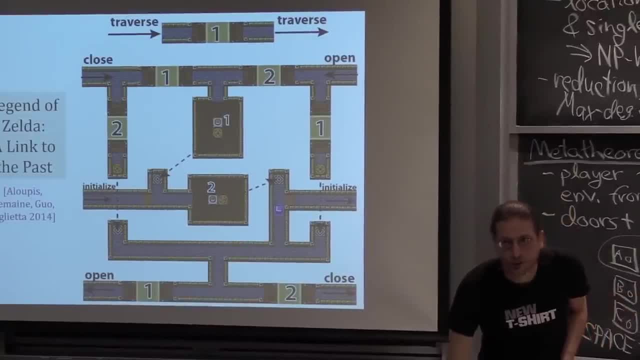 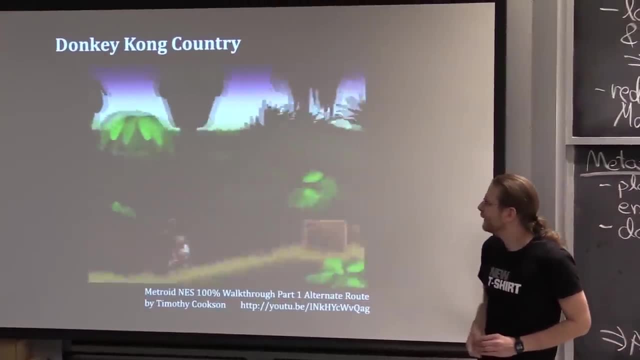 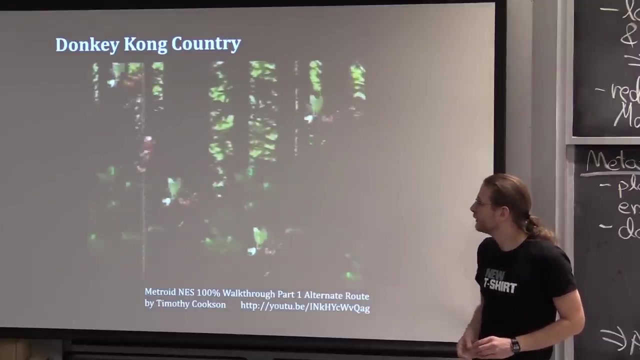 Cool, All right. Next one is Donkey Kong Country. This is a recall of the physics of Donkey Kong. You can jump around and kill enemies and stuff, But the main goal is to get to a destination Other than points. there are these bees. 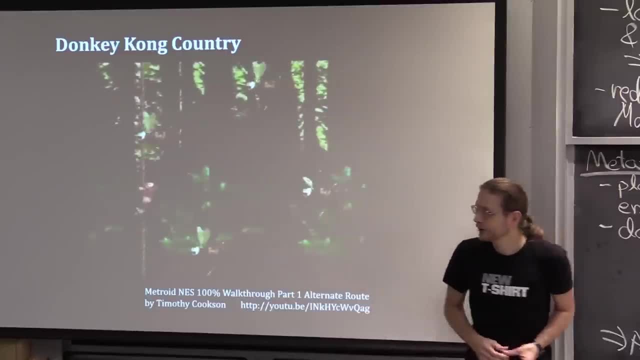 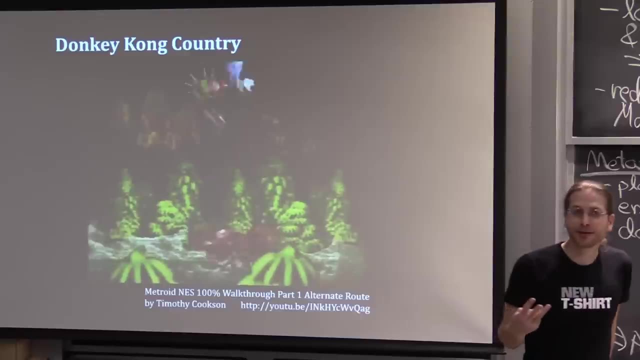 which kill you if you touch them. They're ropes and things you can climb And there are also barrels which you can throw at things. And there are three main Donkey Kong countries- one, two and three- And they each add an additional feature. 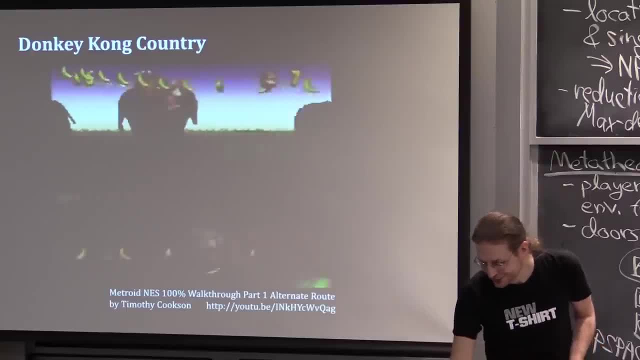 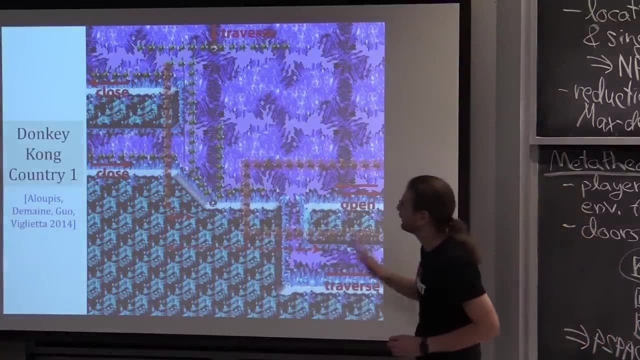 But none of them share that feature. So there are three different piece-based hardness proofs, each with an additional feature. So let me tell you, this is Donkey Kong Country. 1. Let me tell you the notation: We have these bees. 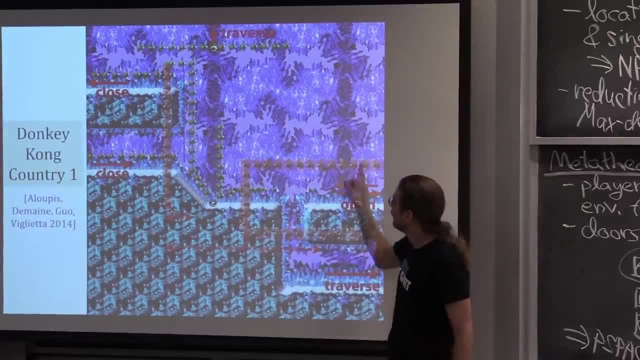 Which are stationary, So those serve as obstacles you can't touch. Then there are these bees highlighted in red. They're not red bees, That's different, But they are moving according to this arrow. So imagine this whole thing shifting over to here. 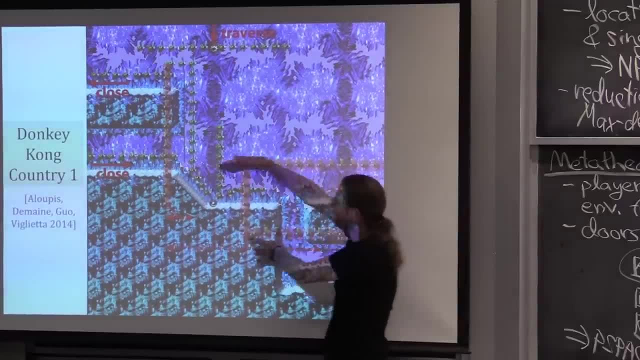 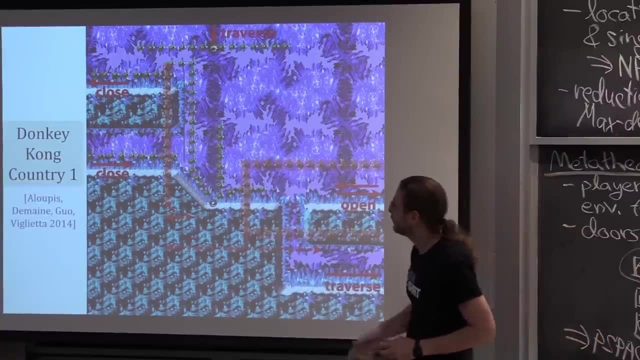 and then shifting all the way over to here and back and forth, And this is naturally occurring in Donkey Kong Country. You have bees which have some horizontal path that they traverse, But we're going to generalize a little bit and allow the bees to move different amounts. 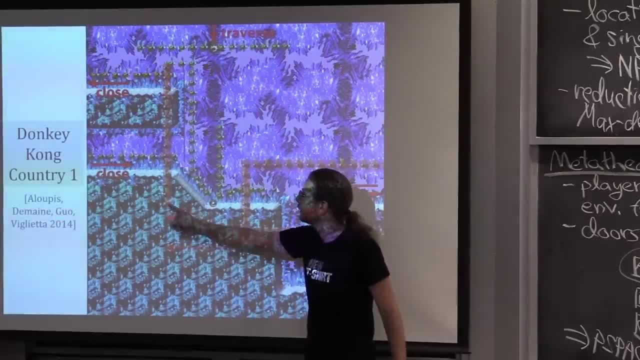 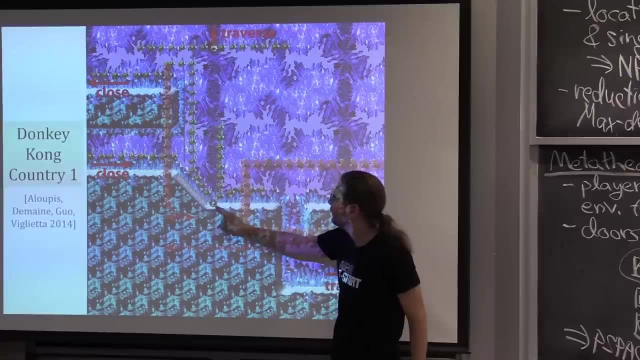 This one only moves a little bit back and forth. I guess it's between here and here. All right, So then there's this additional feature, which is this tire, And the tire, if you land on it, you basically bounce back up very high. 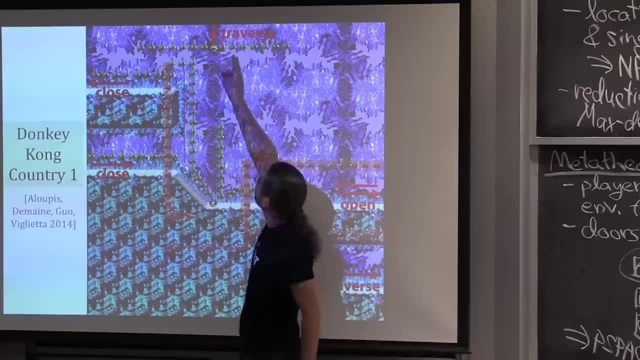 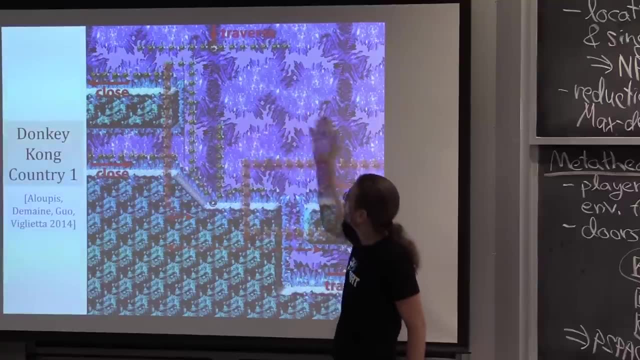 And that's going to be annoying From the traversal standpoint. we're going to be in this barrel. It's going to shoot us. We're forced to shoot straight down If we hit this thing. we are basically stuck in this connected component. 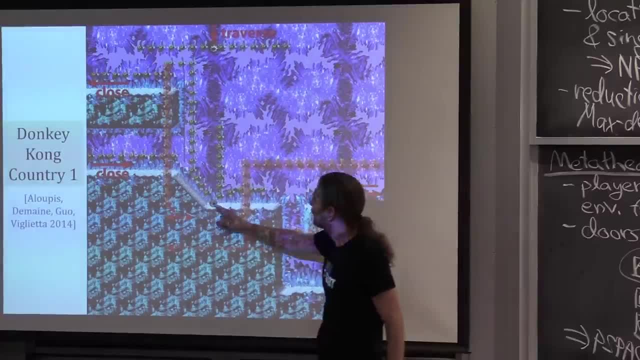 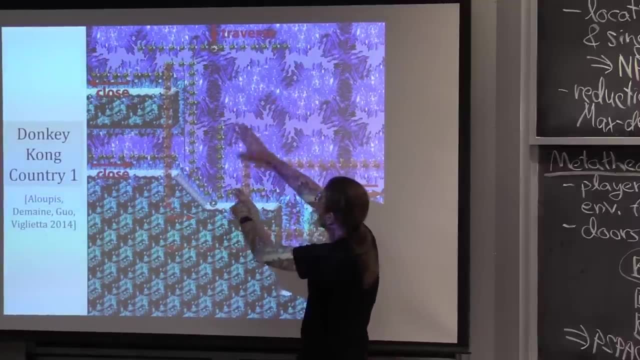 There's bees everywhere We can't get out. On the other hand, if the tire were up here, then if we shoot down, we can time it right, wait for the bees to be going to the right here And then we can run down here and fall down. 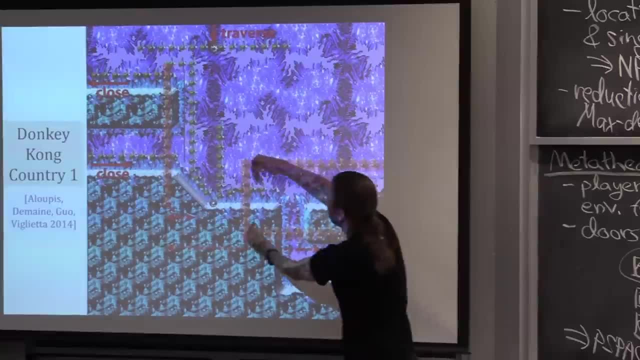 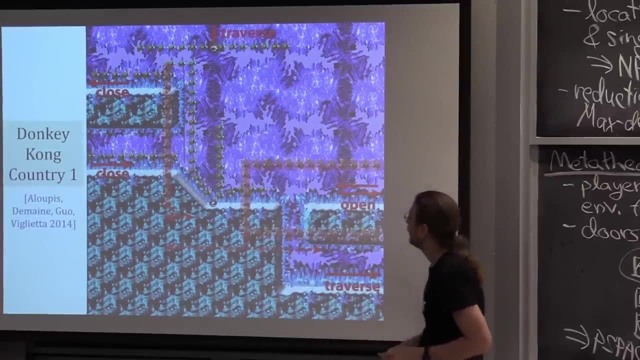 and go through the traverse out Because of these bees which are going to go most over to here. we can't go out through the open setting from traverse. But if we come from the open setting because these bees are going to go away over here, 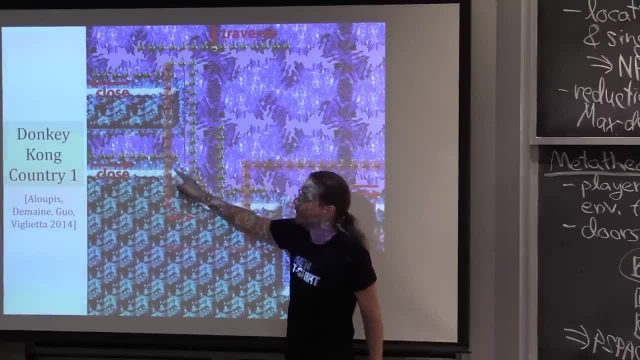 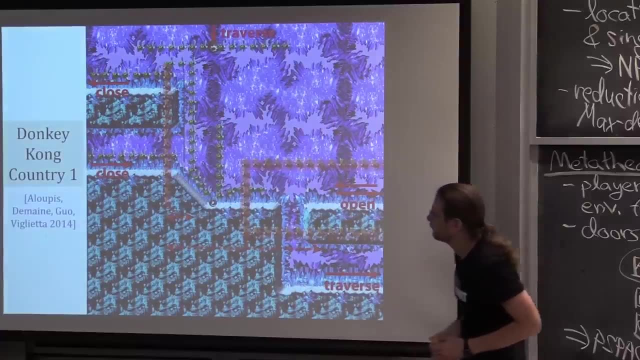 we can run over and push the tire up to this position. So if you land on it you bounce, But if you come from the side you can push the tire however much you want. So that will be pushing it into the open state. 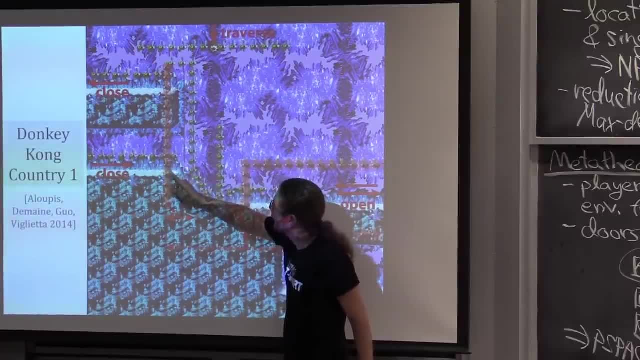 And these bees will go right up to here, And that's as far as we can push it right on that ledge, because you don't want it to fall down the ledge, which also happens in Donkey Kong physics. So that's open. 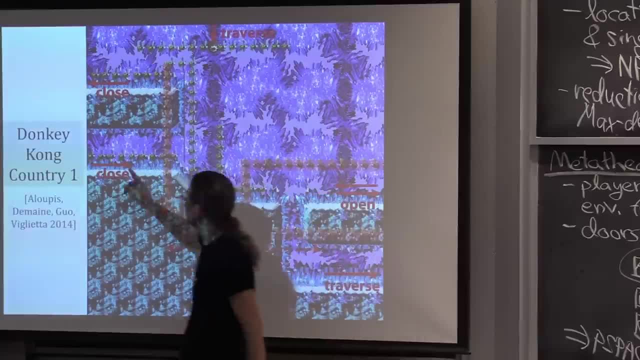 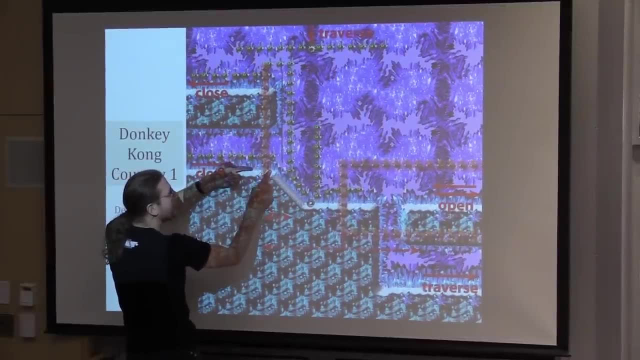 You don't have to open, but you can Now close. You have to close the door And this corresponds to coming through here. If there was a tire here, if we were in the open state, we have to push the tire off of the edge here. 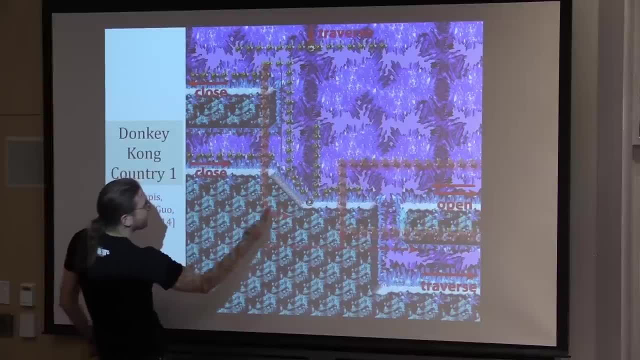 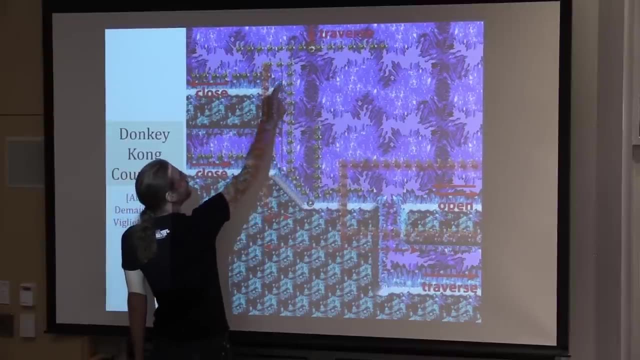 And then it will roll down to that position And if we time it right, the bees will be right over here And then we can jump around. You can climb the rope, And if you're really fast for climbing the rope- and these bees are really slow, rather then. 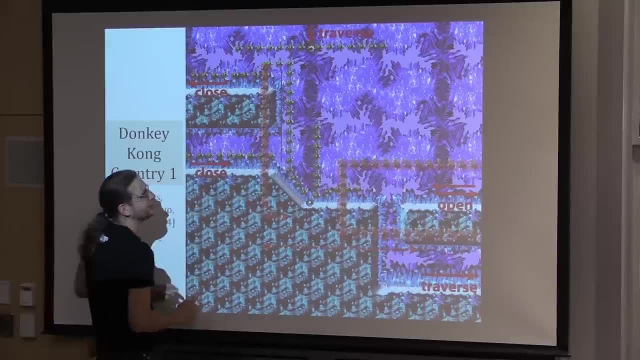 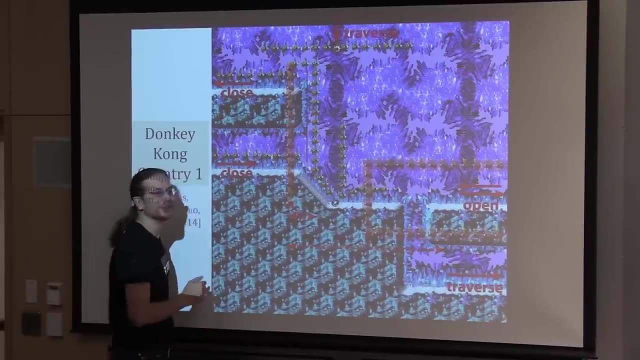 you can go over here. This might not be to scale. Maybe you want to widen the section here so that you have more time to climb the rope. That's just constant factors. Either you allow me to slow down bees or you stretch this diagram a little bit. 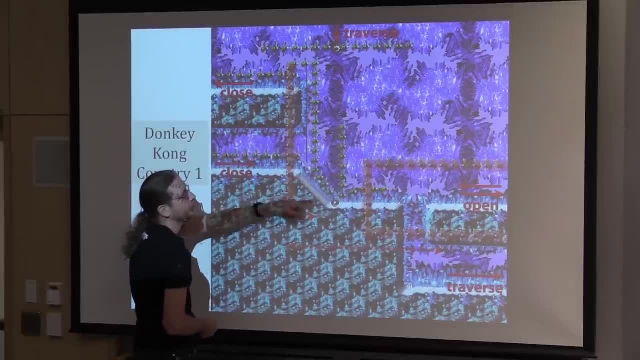 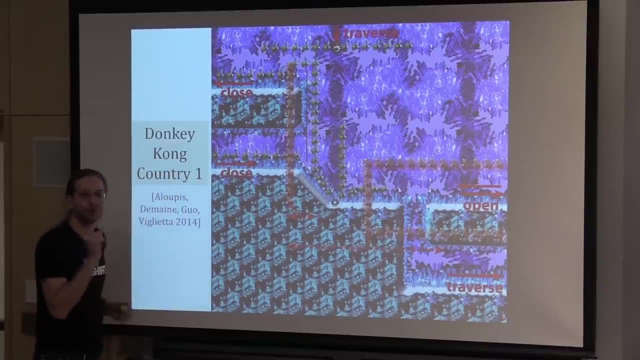 OK, so that's close. In order to get from here to here, you must push the tire off the edge And then it will roll to exactly there, preventing you from traversal. So that's a door. Donkey Kong Country 1 is PSPACE complete. 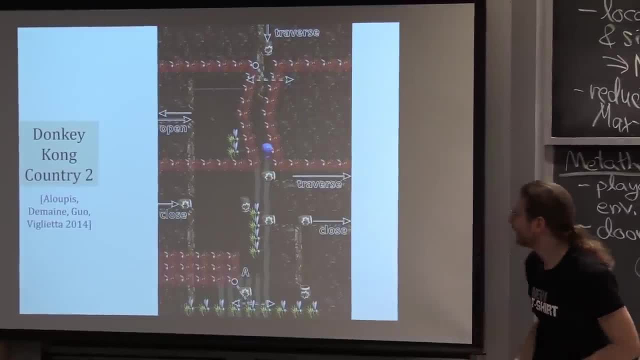 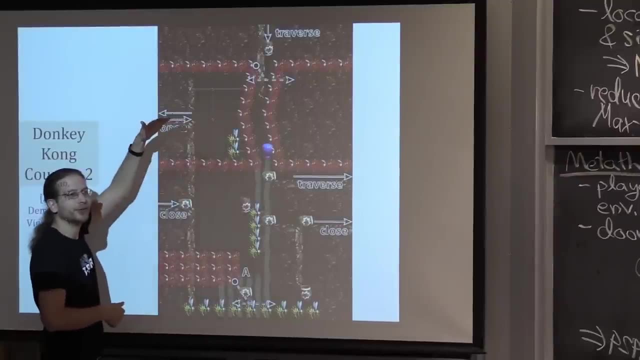 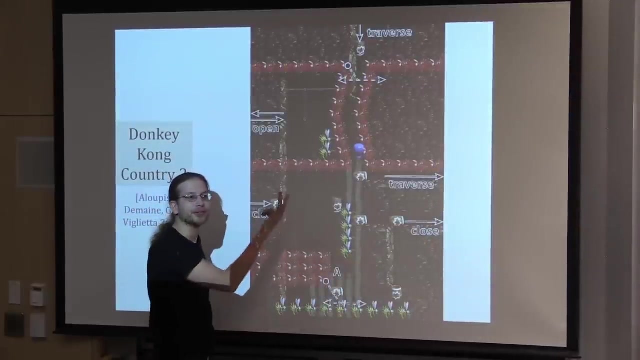 What about Donkey Kong Country 2?? It has no tires, but it has the balloon, The balloon, The balloon. If you're, Normally balloons go down, as you might know, from gravity, But if you have these air currents, the balloon will rise. 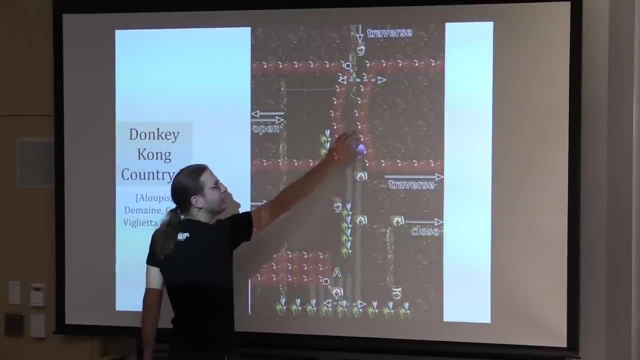 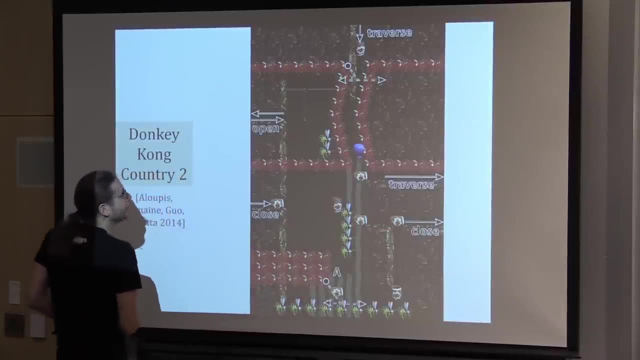 And when you're on the balloon you can use it as sort of a ledge. It may still go down, but you can control whether it falls to the left or to the right according to whether you press left or right on the controller. 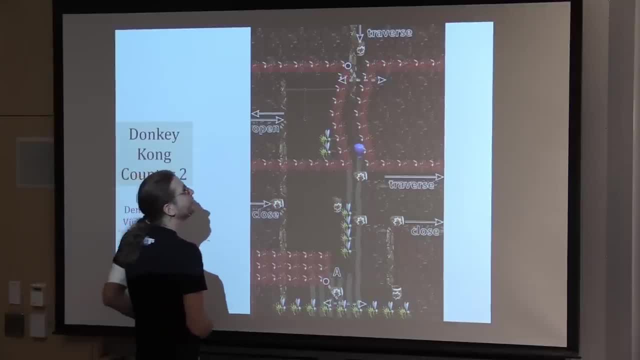 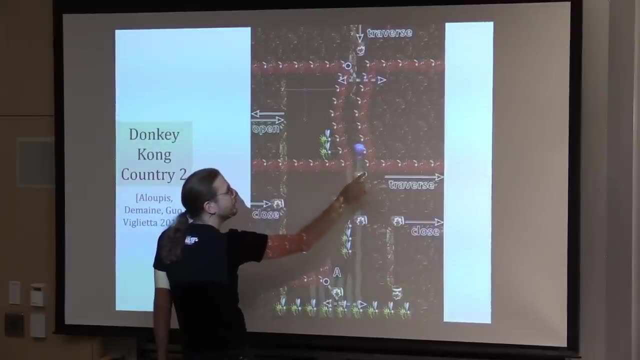 So this is actually the closed state. Again, there are these bees. They're moving a little bit, But if you time it right you can get down here. But if you land on the balloon, there's no way to get beyond this barrel, and so you're stuck. 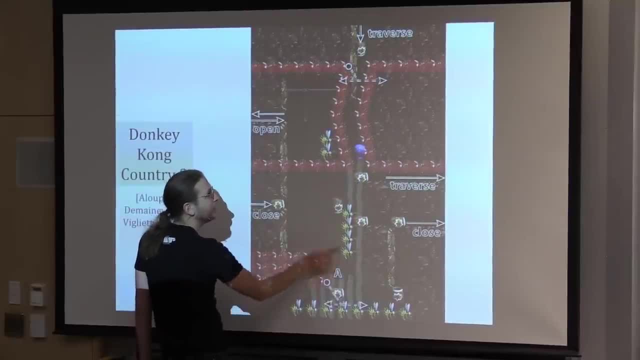 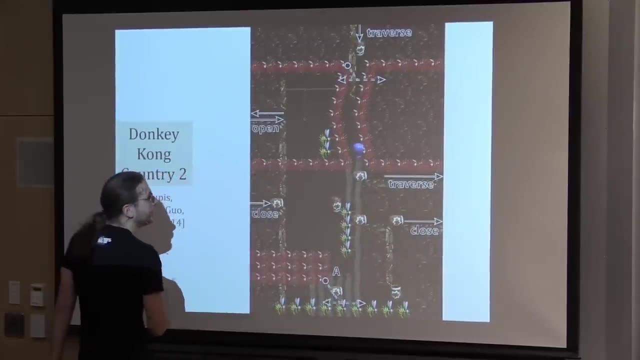 If the balloon is out of the way, it will end up being here at position A. Then when you shoot from this barrel, you end up in this barrel and you get to traverse out. So that's good. Again, these barrels is a forced shot. 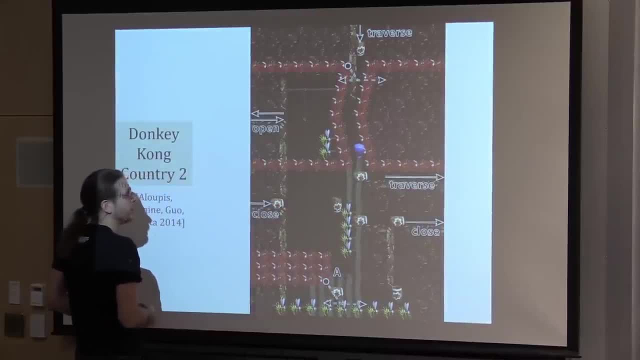 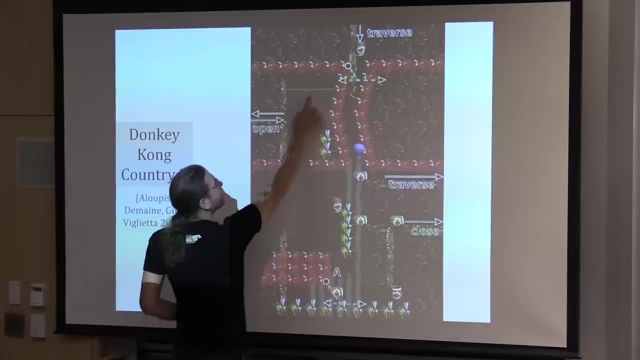 so you can't make any decision at those types of barrels. OK, Good. So the idea with the open clause is that you want to be able to get the balloon to this position. So you would. there's a little bit of rope here. 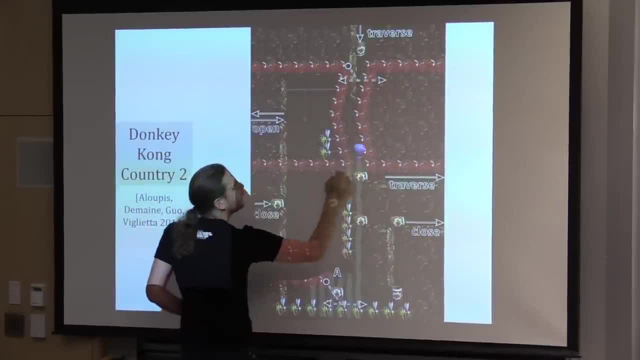 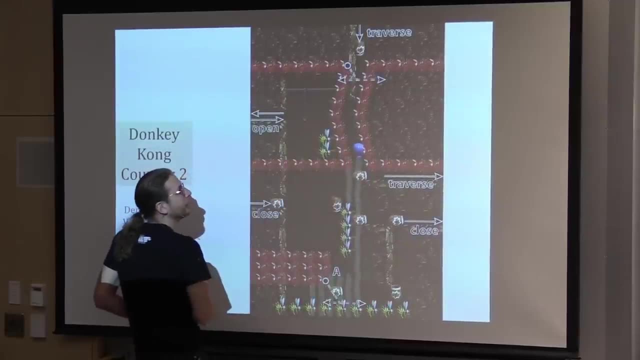 So you would climb this rope, jump When the bees are over to the right a little bit. they get over to here. Then go on this balloon, push it over to the left here and then jump back out and grab the rope and leaf. 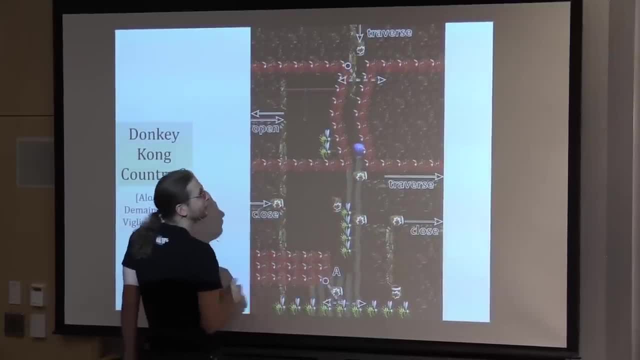 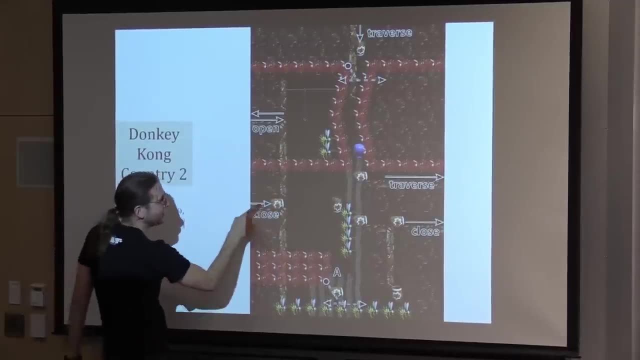 And if you get the balloon to here, it will settle to this position. So you've successfully opened the gadget even though you couldn't get here from there. The close is going to force you to reset that. So we get shot over this way, shot down here. 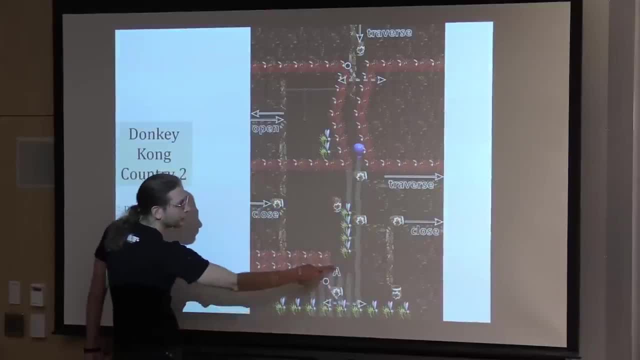 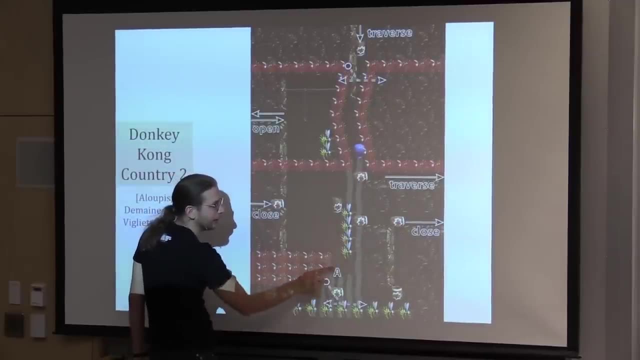 Now it could be, we just get shot, shot, shot and we're out. But if there was a balloon here, we will land on it. And then we have to. in order to get to this barrel or the next one, we have to push the balloon over. 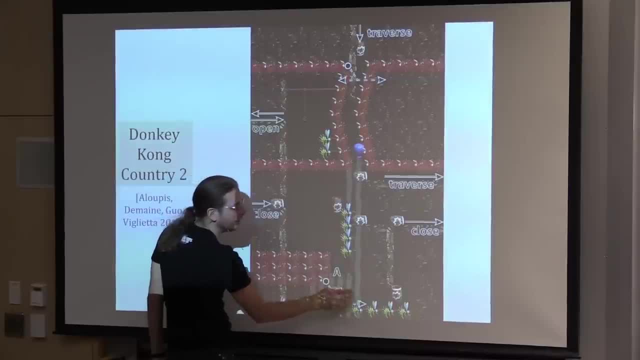 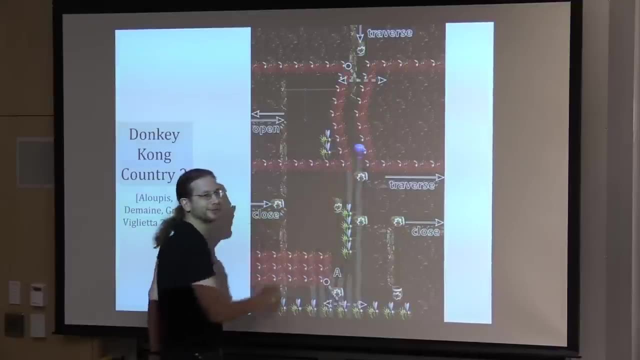 Then we can go here or go here, and we'll end up getting shot to this position and out. But because of these air currents, the balloon will go up to here- There In Donkey Kong physics, And so when you do close, you're forced. 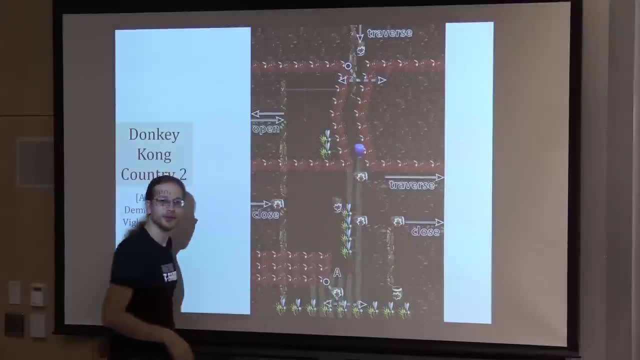 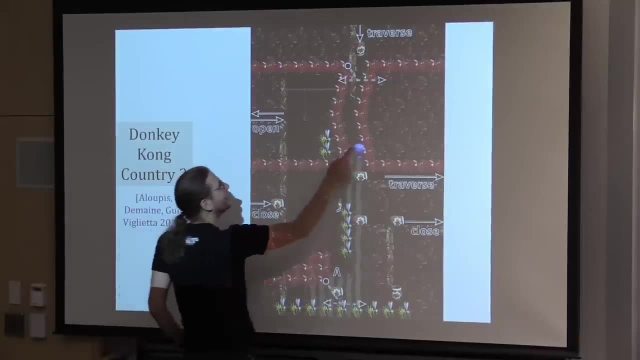 to put the balloon back here, which is annoying for traversal. So that's a door Question. Is there a reason we need a little zigzag in the piece at the top? Why do we need the zigzag? I don't remember. 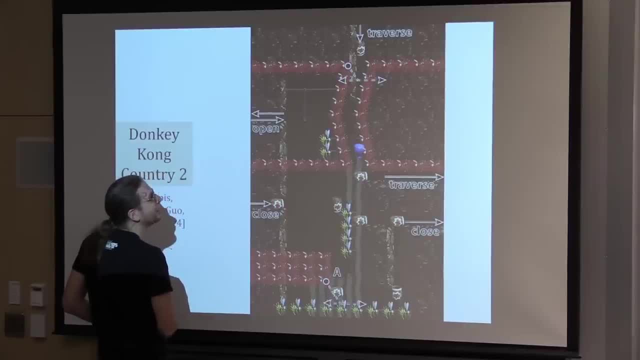 I was wondering that as well. Yeah, What it does do is force a particular sort of timing, maybe about whether it's to the left or to the right, But I don't know. Is there a reason? Not sure, I'll bet there's a reason. 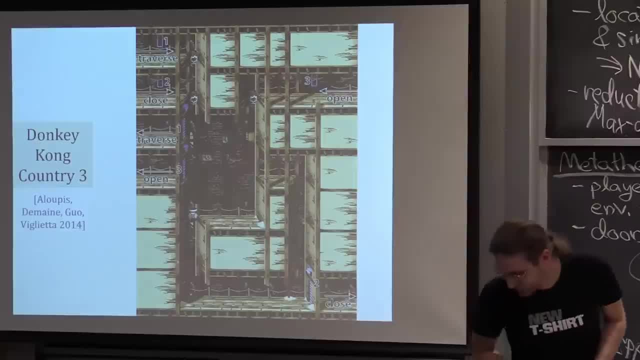 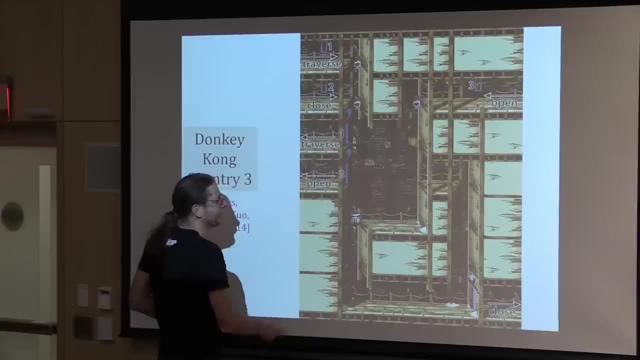 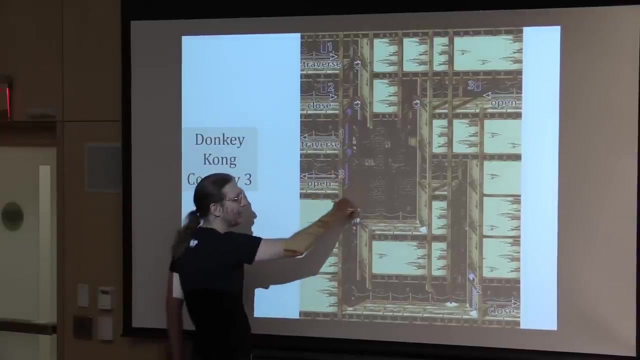 But this figure was drawn by Giovanni Cool. What about Donkey Kong Country 3?? Well, Donkey Kong Country 3 has neither balloons nor tires, but it has tracking barrels, the T on it, So tracking barrels if you land in one. 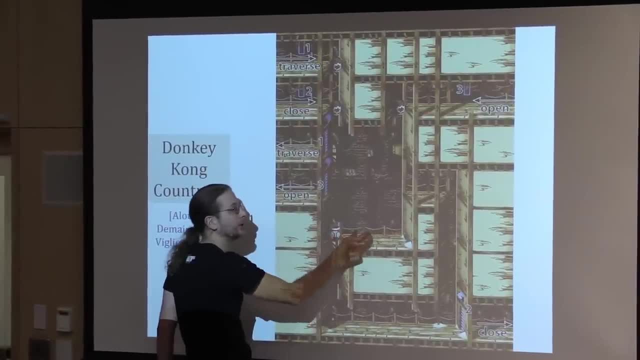 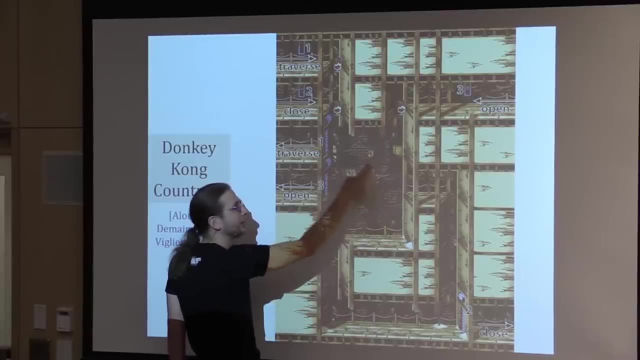 you can then slide it left or right, And when you leave it you always get shot up. And even if you jump out and then say: go over here and fall, the tracking barrel tracks you. So if you're coming from traversal. 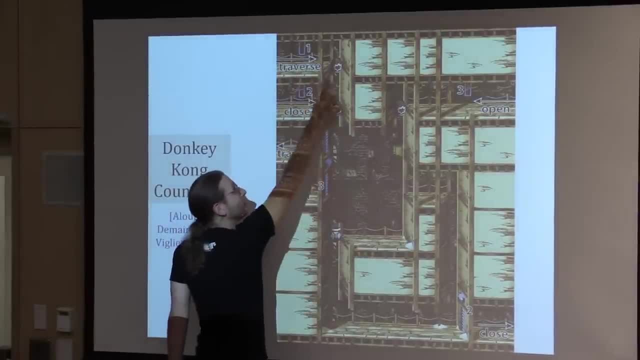 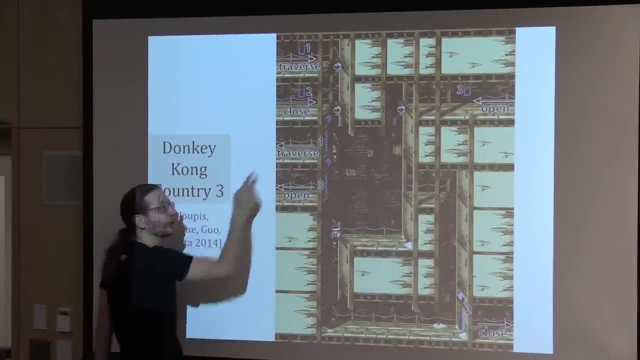 and you get shot down here. if the tracking barrel's out of the way, then I traverse, Then I'm forced to go down here and leave via the close exit, which is not what I want. I want to leave according to the traversal exit. 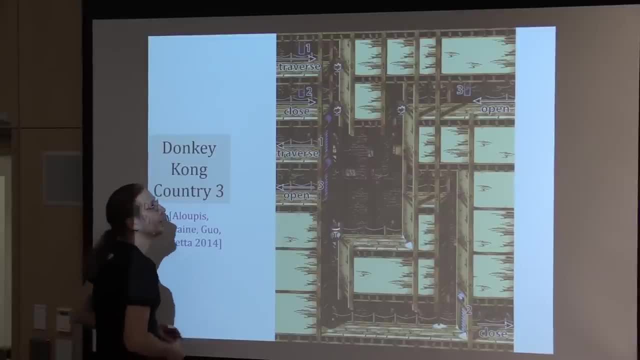 Now this has some leakage, but you can show this leakage is OK, You can go from traverse in to close out, but that won't end up helping you, because you were already closed, So you knew you could already get to close out. 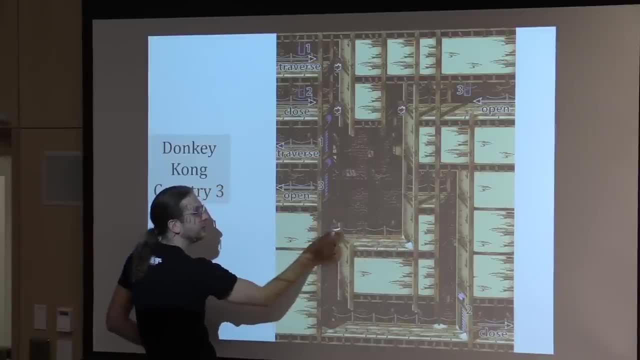 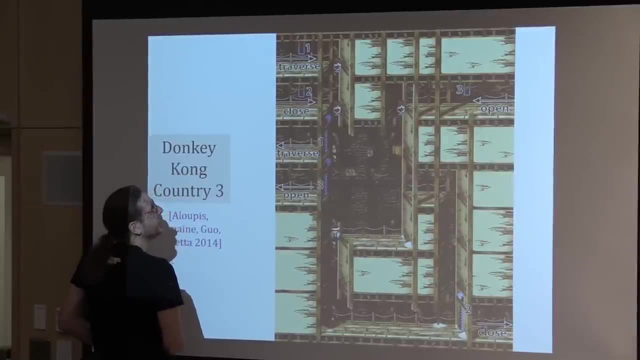 So this is the closed state. when the tracker barrel's over here, This is the open state. When we're in the open state, we come through traverse. we can jump out and leave here, So that's good. On the other hand, if we come via the open position, 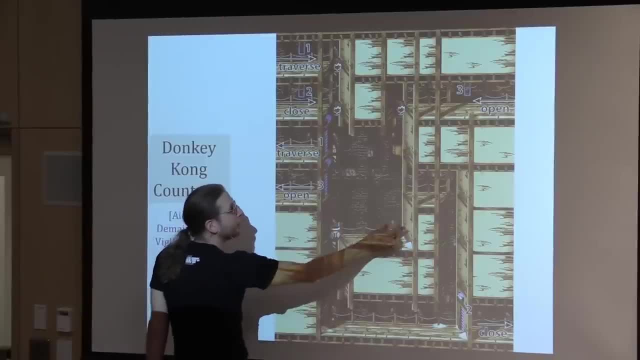 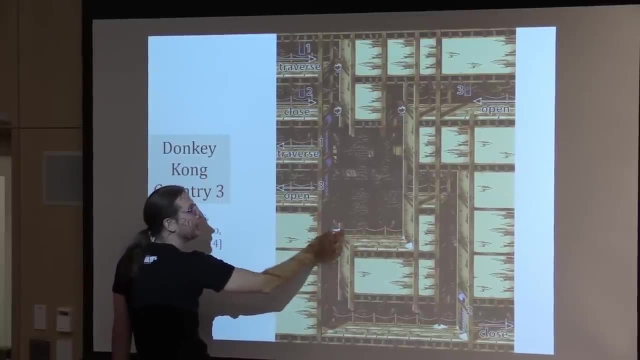 we can get shot down here, And if the barrel was there we're going to have to move it over to here. I guess we don't have to. We could leave it there. But we are able to bring the barrel over here and leave through open. 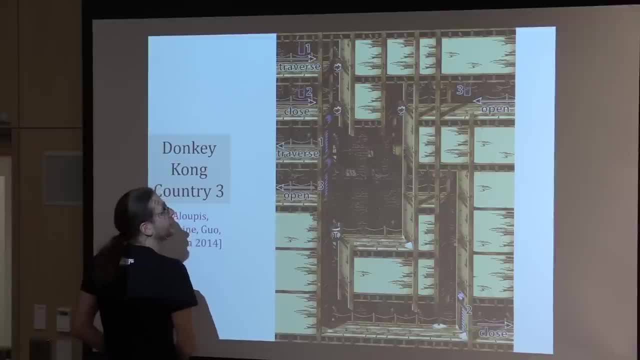 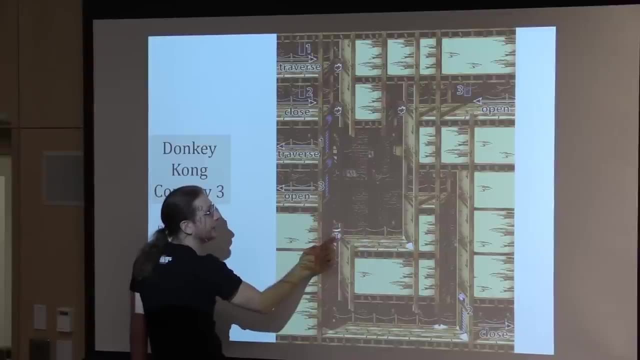 Now we're in the open state. That's good. On the other hand, if we come from close, if it's currently open, we will be shot into the barrel And then to get over here, we have to bring the barrel over here, putting it. 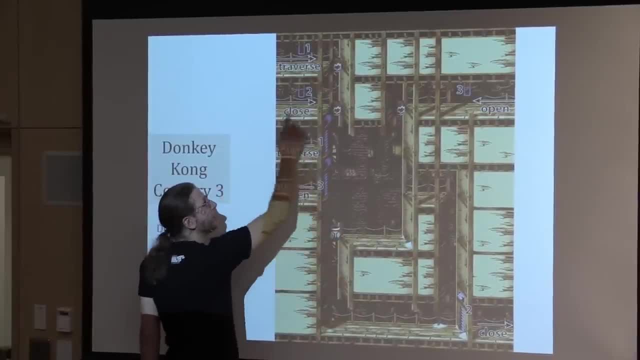 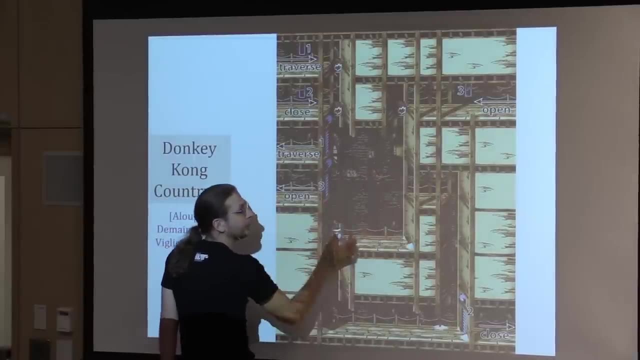 into the closed state. Now this is the relevant part where the tracking hurts you. You go in here. You'd like to just jump out and get out here, But because it's a tracking barrel, if you jump out here the barrel will come over anyway. 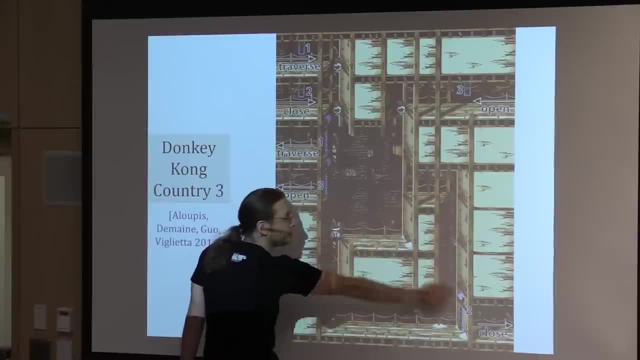 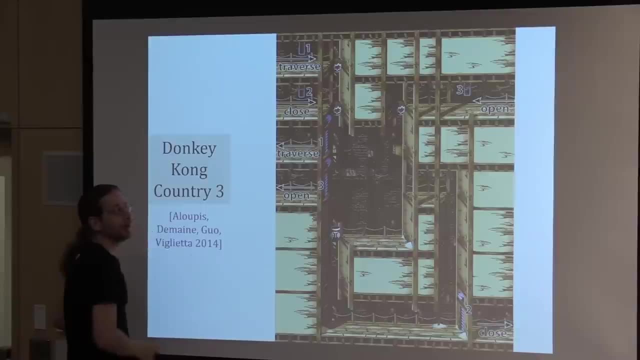 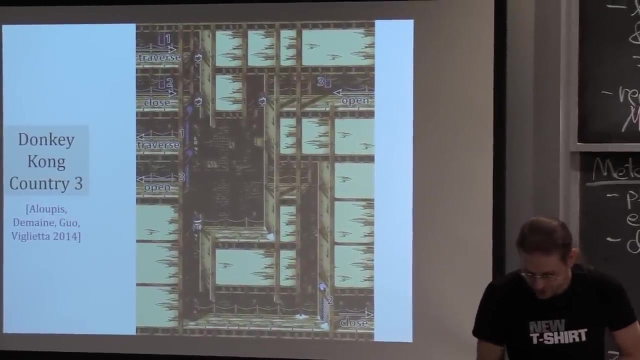 even though you don't go back into it. So if you leave through the closed exit you have to bring the barrel over to the right, So that forces the close preventing traversal. That's Donkey Kong Country 3.. But there's one Nintendo game that. 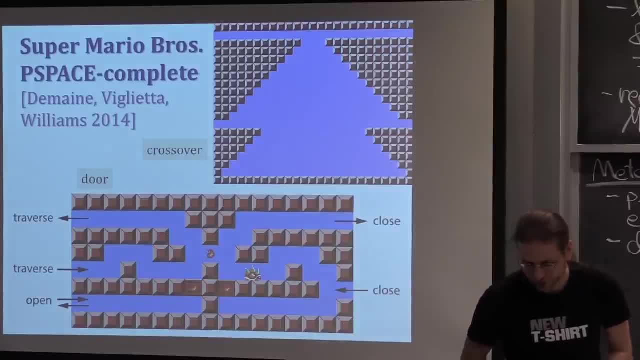 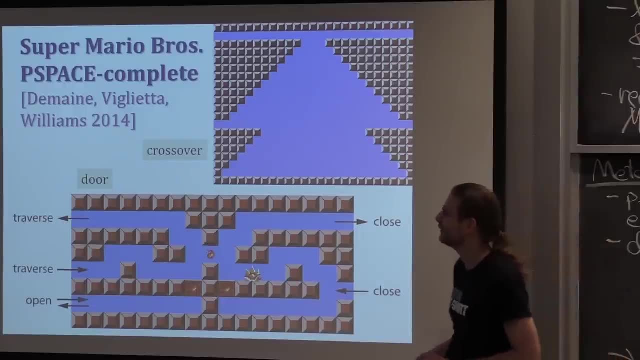 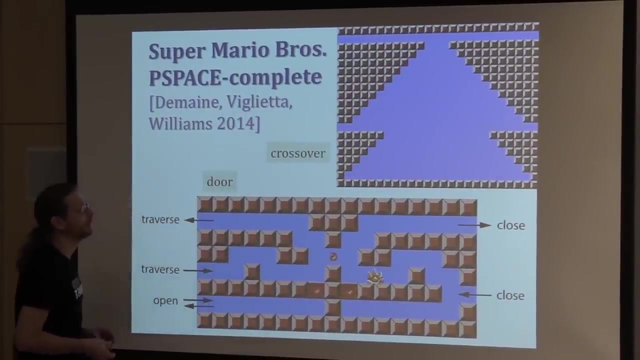 rules them all and that is Super Mario Brothers. And for the first time we are announcing a PSPACE completeness result for Super Mario Brothers. So the Nintendo paper and another paper by Giovanni, which I will talk about next, was prevented at Fun with Algorithms earlier this summer. 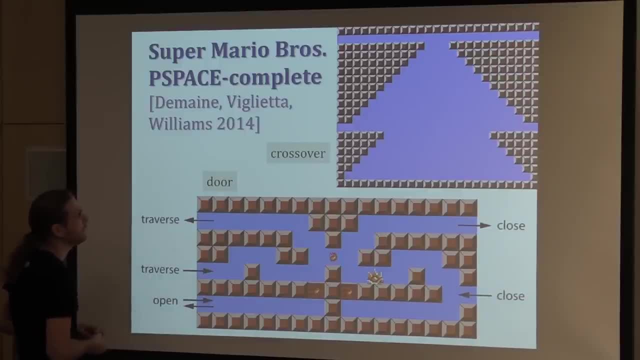 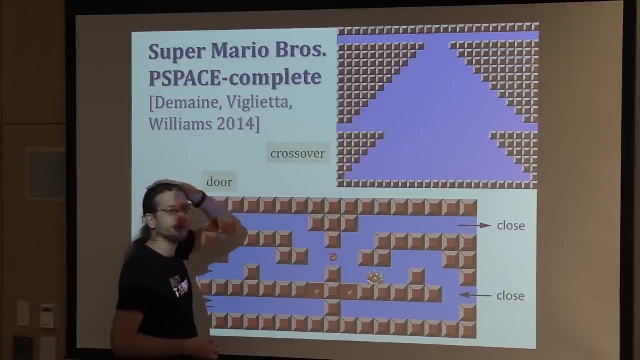 Two people were there And then we started talking: oh, we should really prove Mario Brothers also PSPACE complete. So this is our current reduction. You may recall another crossover gadget that involves invincibility: stars or mushrooms or something. Those are consumables. 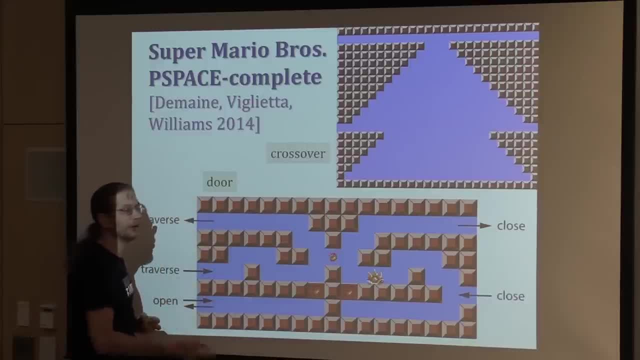 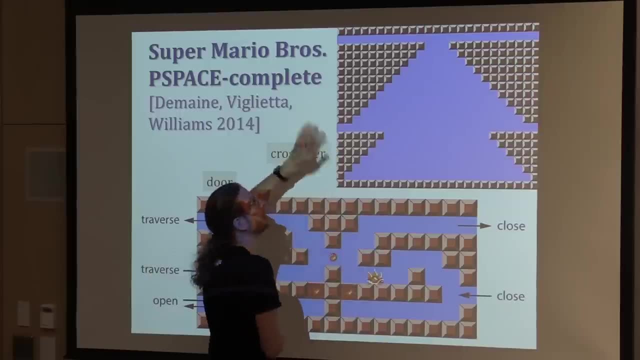 We can't afford consumables in a PSPACE reduction because we have to visit the same thing many times. But using Mario physics, we designed this crossover where you're going to be small Mario, throughout this reduction. If you come up here and you run, you will fall here. 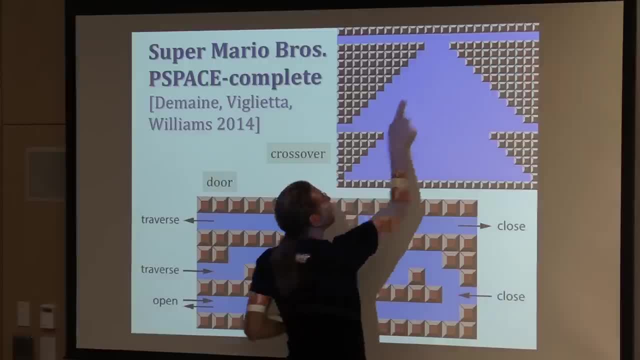 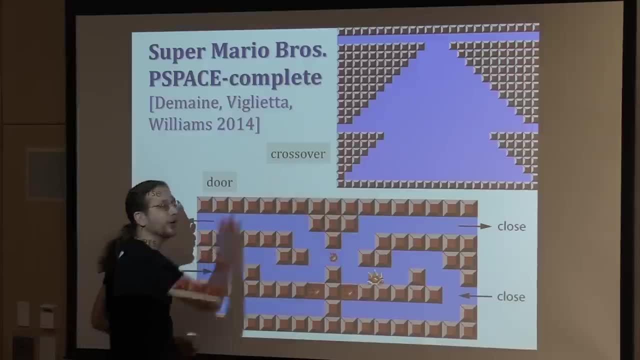 And if you come over there, you run And you fall here. But you can't jump around and land here. You'll end up down here And that's larger than your jump distance. So as long as you can't glitch through walls, 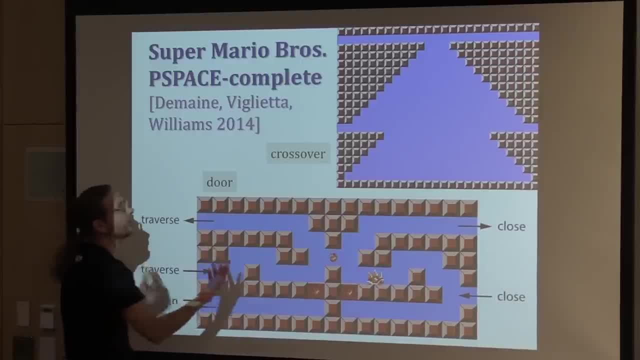 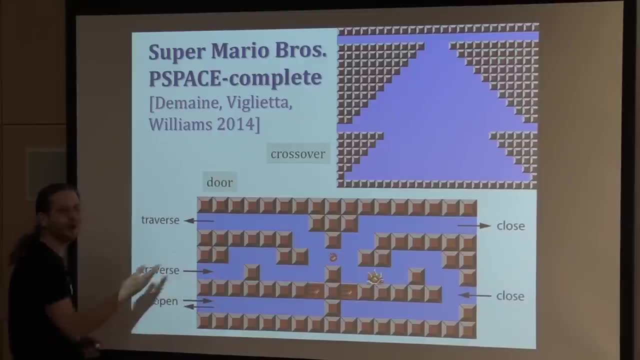 this is a valid crossover And it's reusable. It's a one-way crossover. You can only go from up to down. Now the door. The door is a little bit weird, But it has actually been built by modifying the Super Mario Brothers ROM. 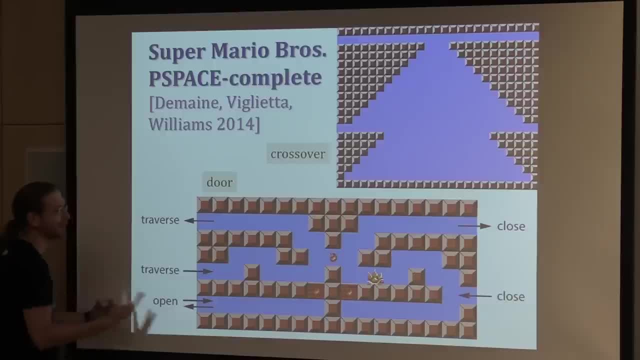 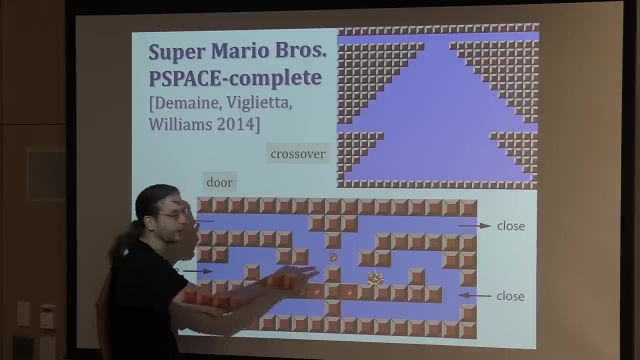 So it does exist, But it's not in the physics of the real Mario We're going to make. this doesn't have to be unit length, But this is a fire bar which is normally rotating, But if it has size one it doesn't really. 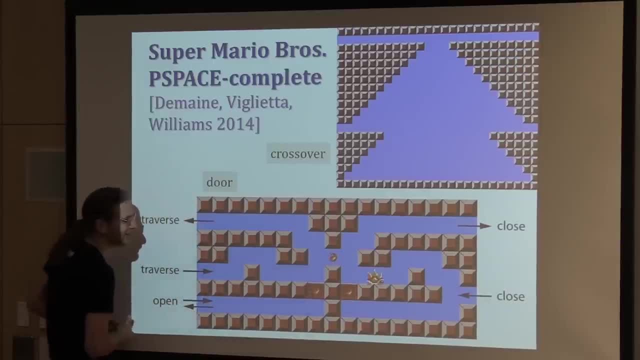 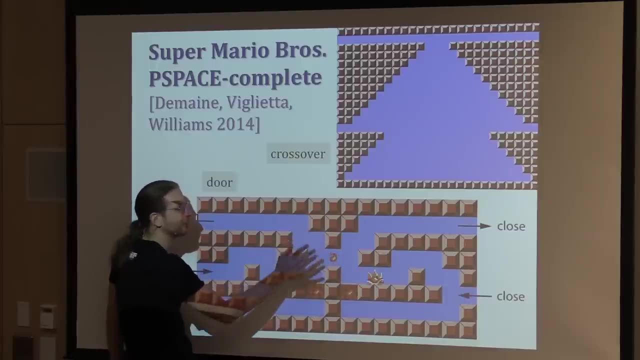 do much rotating. So these are things you're not allowed to touch, And the version we implemented has fire bars. Those do exist in the ROM, But even if you have fire bars that are much bigger, you can still do all the things you need to do in this gadget. 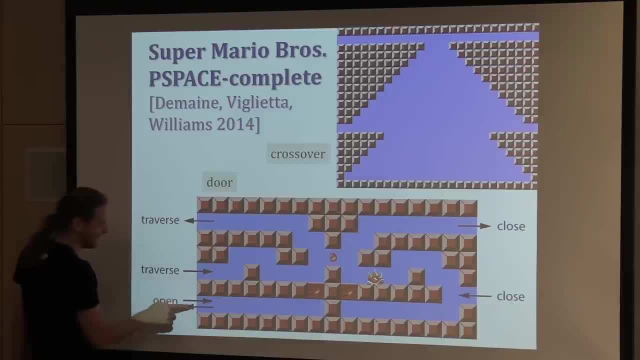 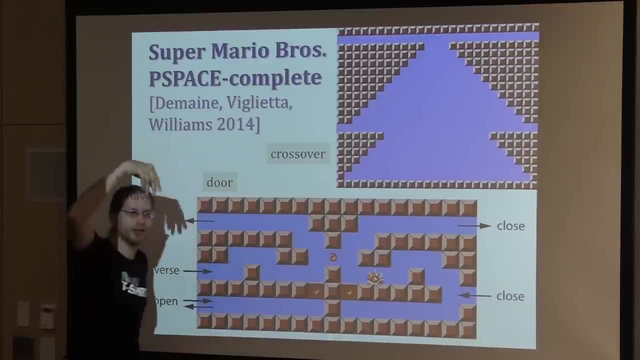 It's just a lot harder. It's a lot harder to do correctly. I was trying it earlier today And then we have this guy. I forget what they're called, But they're dropped by the cloud thing in the sky. You can also create them at the beginning of the level. 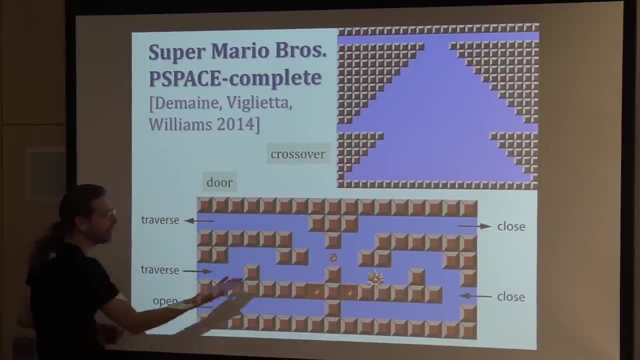 even though that doesn't appear in the true levels. You can make a new level that has these guys. initially It'll just be the case that there's also a cloud floating around at the top, But if you shield from that, you're OK. 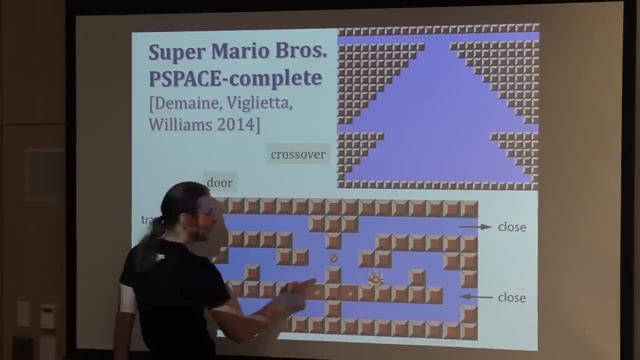 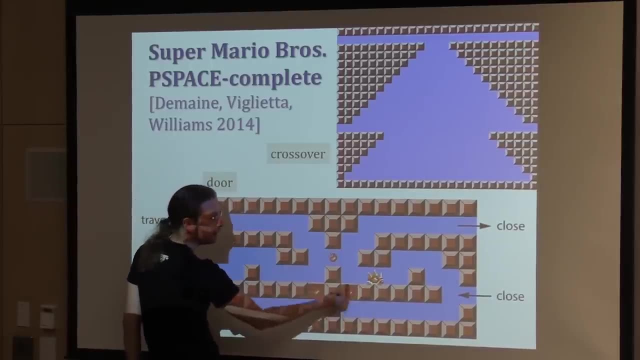 So there's one of these guys And he can basically be walking back. He can be walking back and forth here or over here And you can flip that, But if you hit this block with the right timing, this guy will end up bouncing and walking over here. 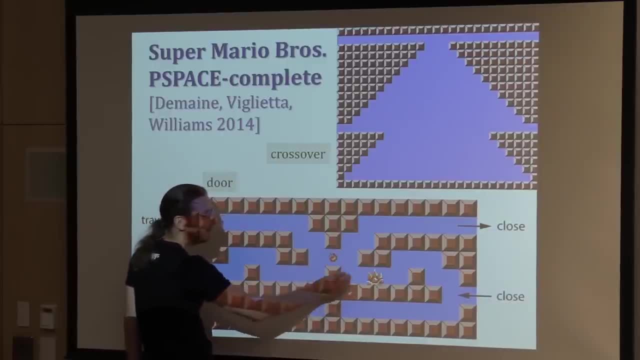 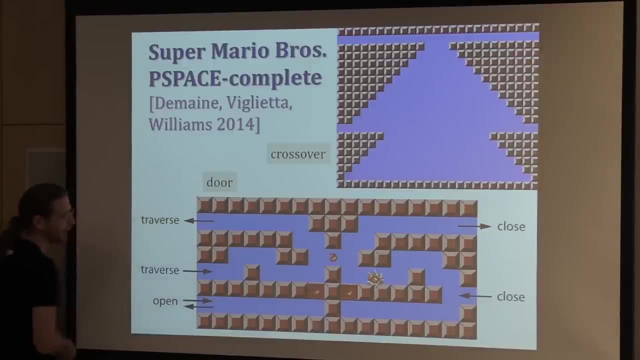 In practice you have to hit it a few times. Sometimes he'll walk back over. But if you get the direction that he's facing right, he'll jump up and then keep going And then he'll be over on the other side. 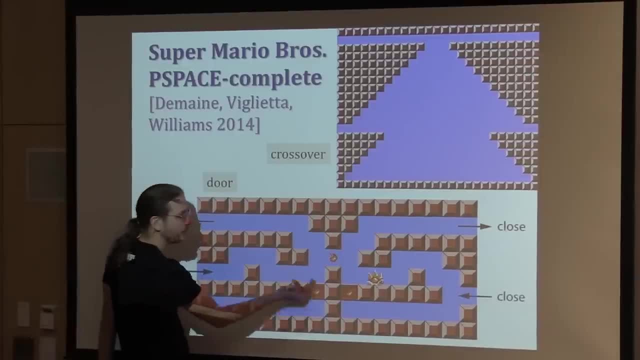 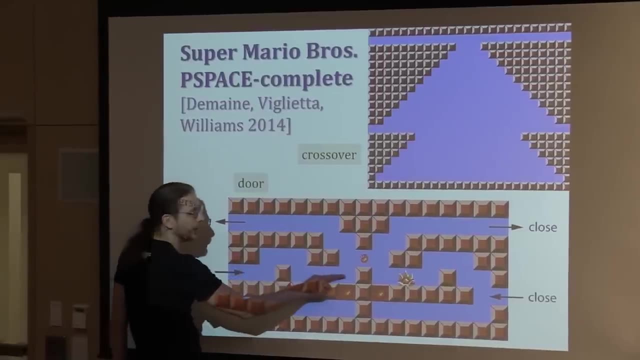 But you can't just reach everything here On the open side you can hit him if you want and put him over there. That's going to be the open setting. The traversal requires you to go through this way without the ability to hit this thing. 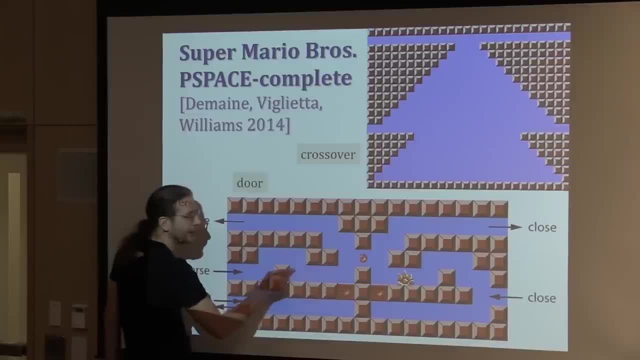 And so if the spiny guy is over on the left, you will die- Guaranteed, We checked- And otherwise you jump. If he's not there, if it's on the right side, then you can traverse. So this is the open state that's drawn. 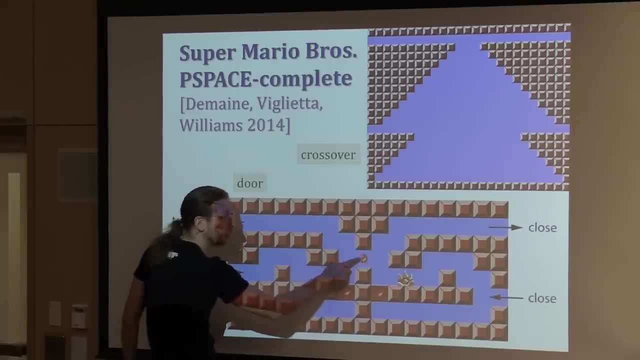 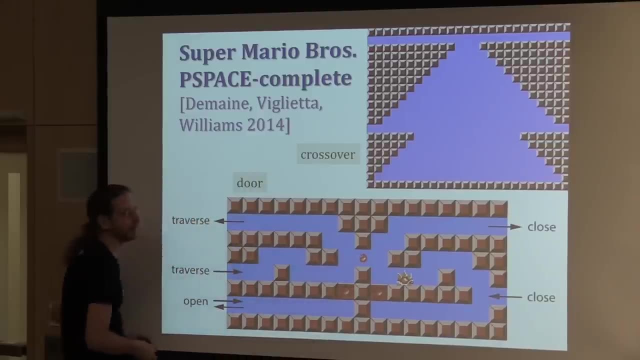 And so this is the tricky part. We need something that's untraversable by the player but traversable by the monster, And this could be a fire bar that's rotating. if you time it right, You can still rush by it And, of course, close. 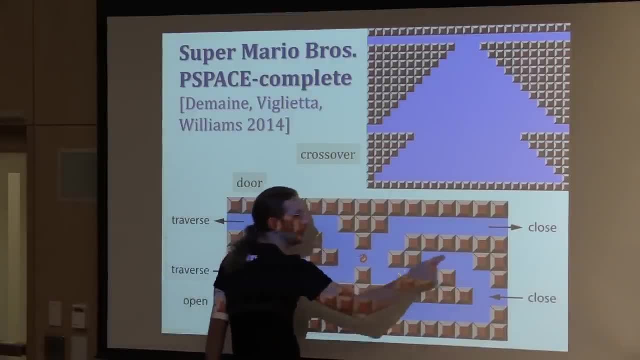 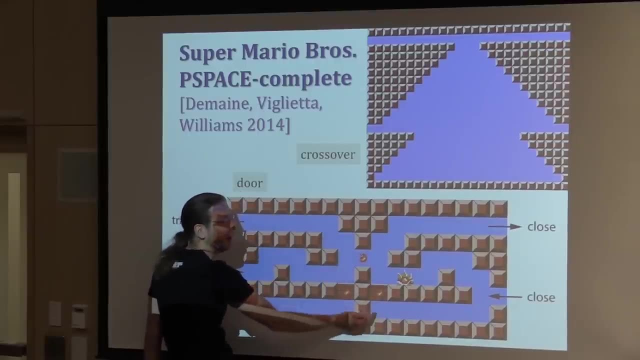 Close, we need to force this guy to be on the other side, And so we do the same thing that we did on the left: to go through to close. Just like on the left, this guy has to be on the other side. So first you can knock him over to the other side. 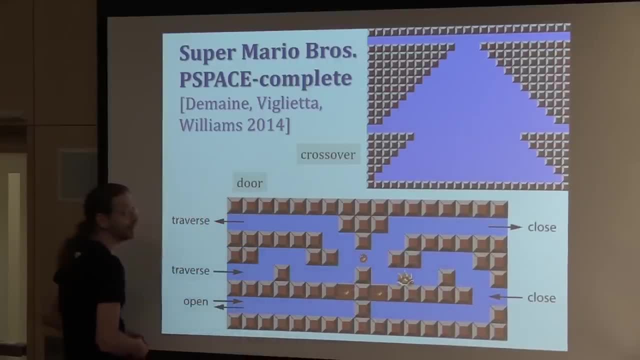 And then you can go back and jump through there. So Super Mario Brothers is PSPACE complete. Yeah, What was the advantage of the rotating fire bar? Oh, it's more naturally occurring In real Mario. there are rotating fire bars. There's never this single fire bar. 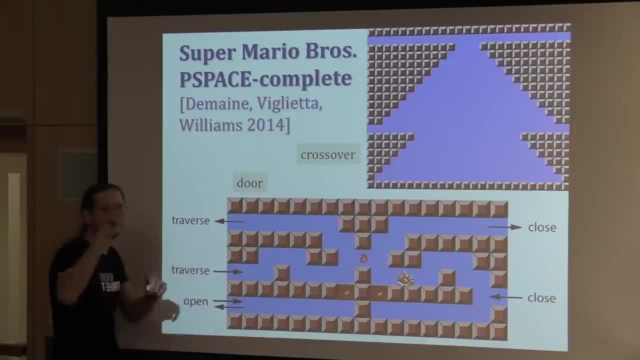 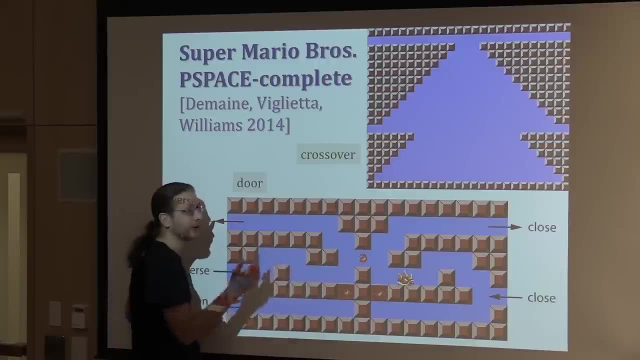 There's never a single fire just floating in midair. Fire bars can float in midair In reality, or in all the levels that exist in Super Mario Brothers. fire bars are a fixed length. There are six fire things or whatever, But in the ROM it has support for making. 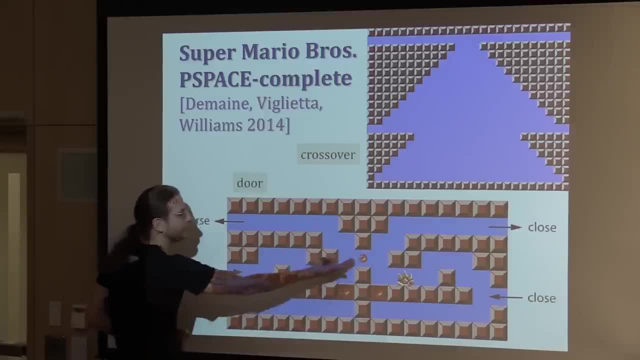 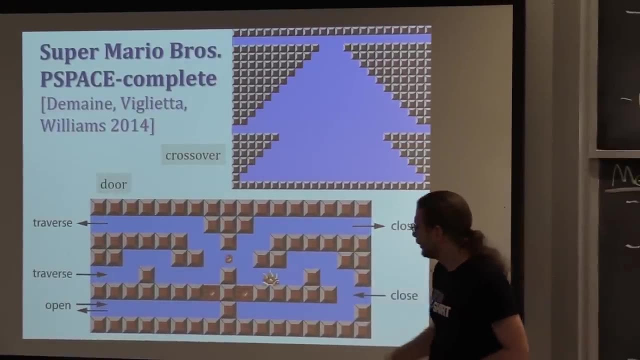 fire bars of arbitrary length or up to some size. So you can make this in the ROM or you can have it rotating, And then it's a more intense experience. Why aren't there fire bars in the little block that you're hitting? 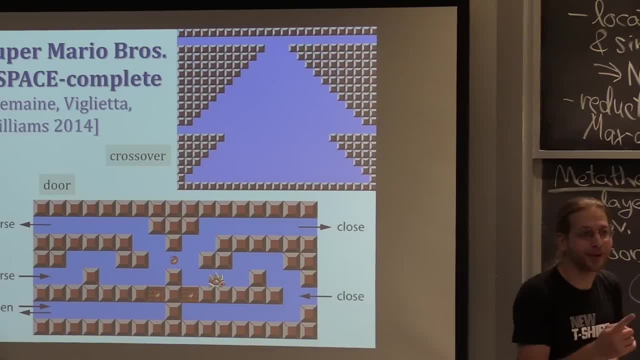 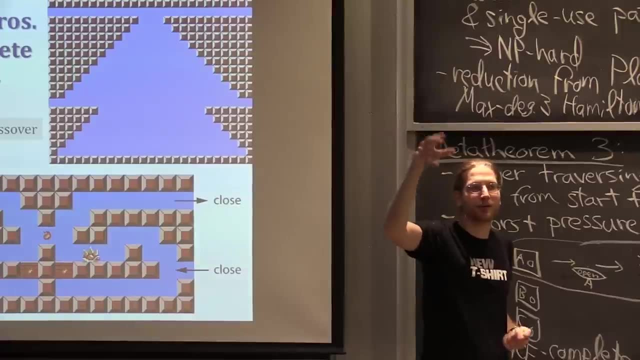 Yeah, It's dealing with glitches. Yeah, Where's the shell guy dropped by the cloud thing Or I don't know the game? Oh, in the game the cloud is up there And every few seconds he throws one And it falls in some kind of random spot. 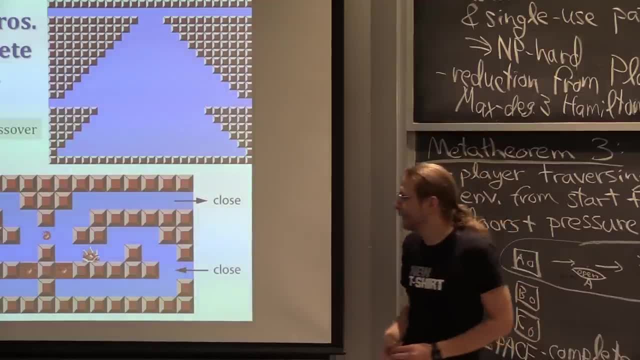 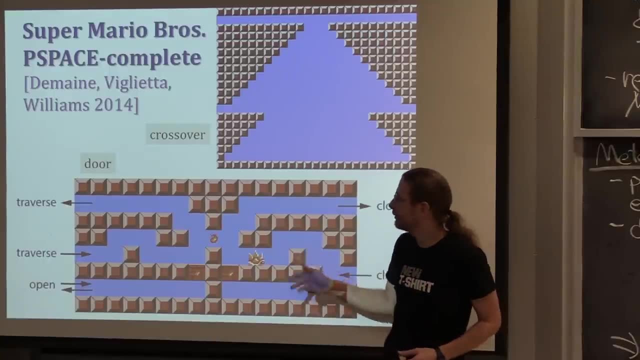 And then he traverses left and right like a regular turtle. But in this we're assuming that you can have him initially appear there, So he's not thrown by the cloud. There will also be a cloud throwing the spiny guys, But we don't know. 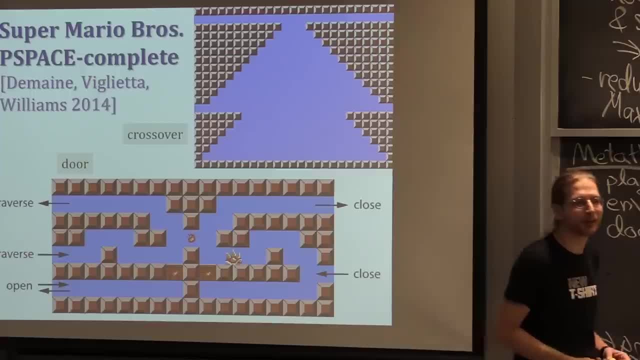 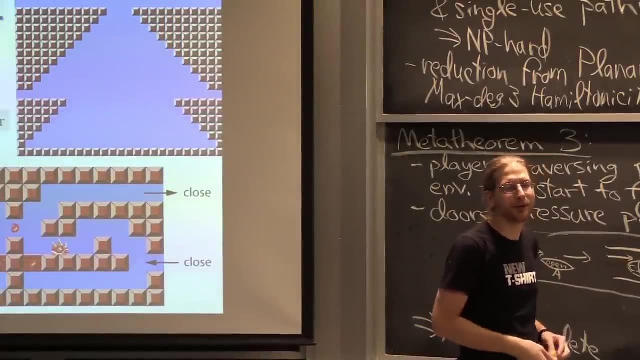 We're assuming that this guy can just be there from the beginning, So it drops more than one. Oh yeah, It drops one and then drops another, and drops another. I think it's unlimited. I mean there might be a practical limit. 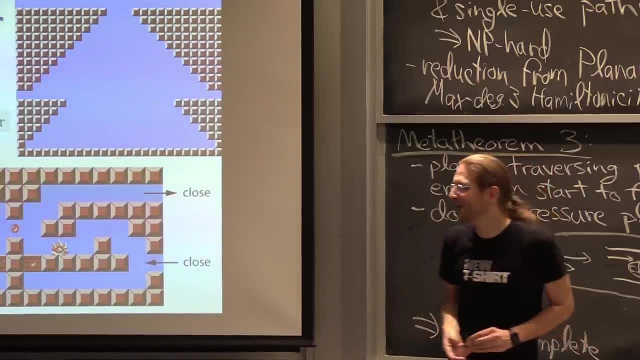 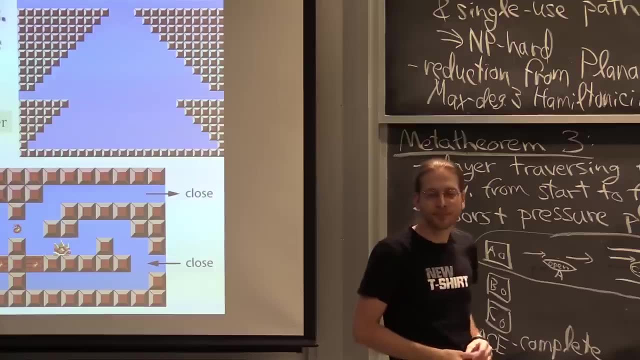 given by the memory of an NES, which is pretty small, But I think it limits to like eight creatures on screen at once or something. But we're generalizing that as well. Other questions: OK, I have one more proof I want to cover. 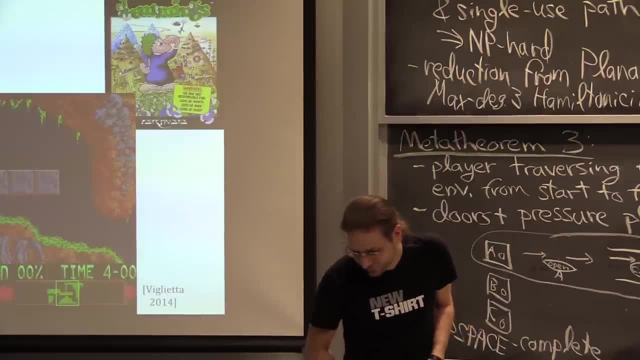 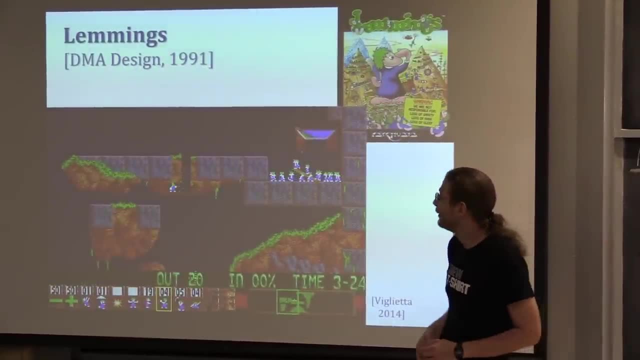 And this is the other Giovanni paper in Fun with Algorithms this year And it's about lemmings. If you haven't played lemmings, it's sort of the first real-time strategy game. So you have these characters which appear periodically. 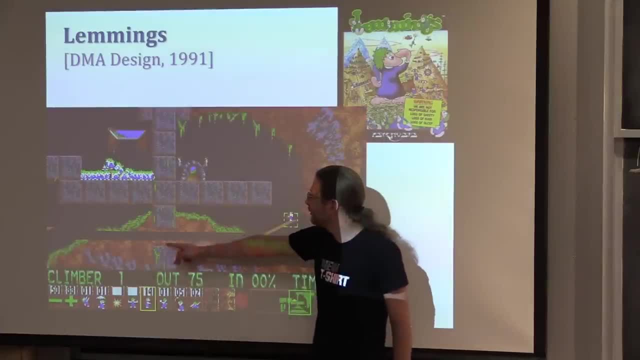 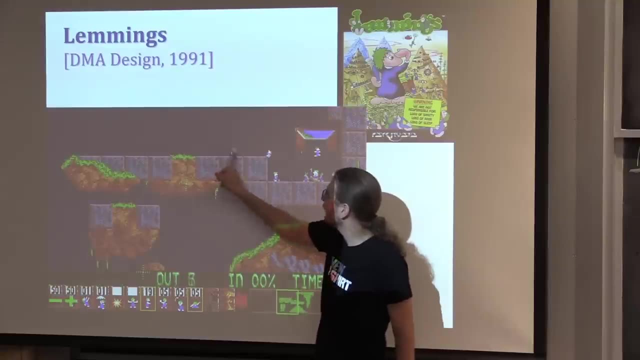 Then you can click on characters and make them do different things. You can make them build bridges, You can make them dig horizontally, You can make them dig vertically, And so going through that again, here we're making this guy climb and then digging down and then digging left. 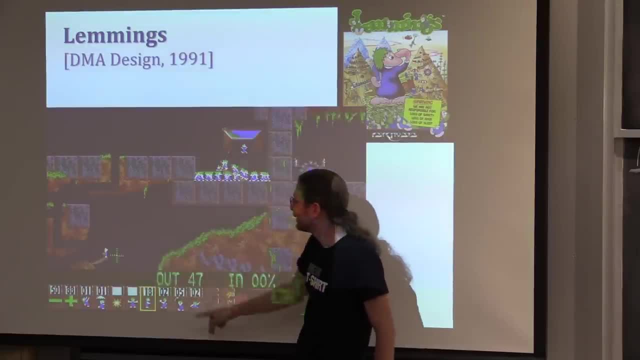 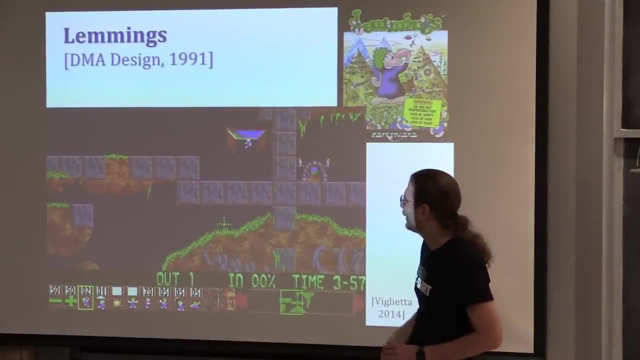 and then digging down and then make him dig left to switch directions, and then make him dig down again and then build bridge and dig through. This is, I think, level two or something. It's quite challenging And your goal is to get as many lemmings as possible. 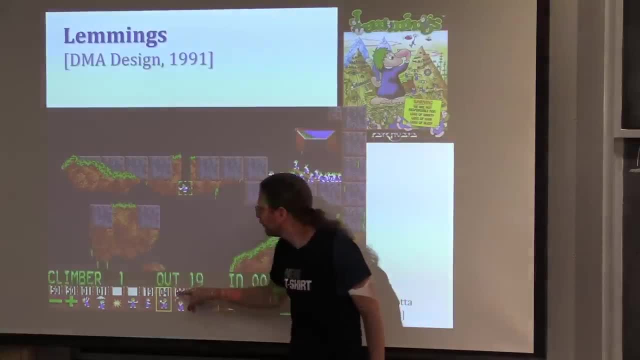 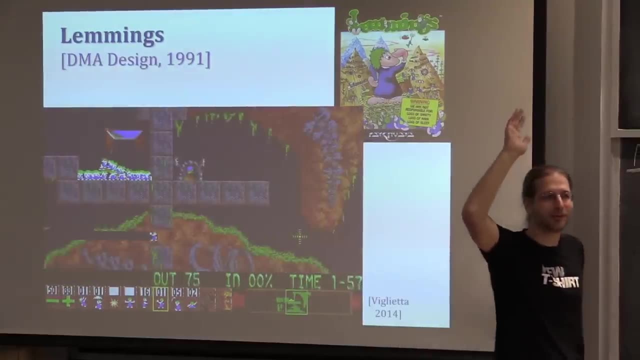 to the exit, And the way you do it is: you select the ability you want and then you click on the lemming that you want to do it on, And otherwise they are walking around. So how many people have played lemmings? 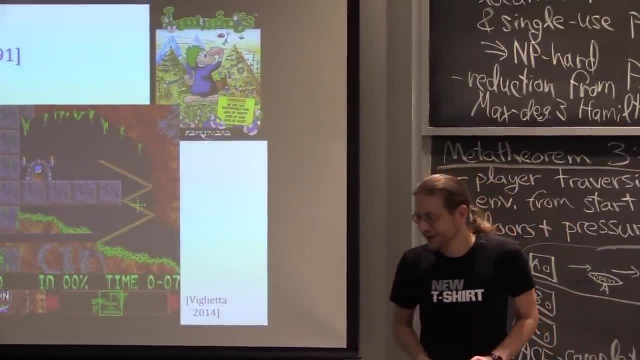 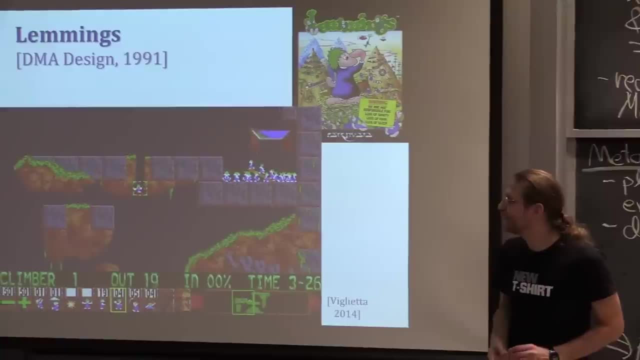 Yeah, this is a more popular one. If you haven't played, you should. It's really hard, though. I was reading Wikipedia, Sarah. one of your favorite authors, Terry Pratchett, was playing lemmings. He wrote a book that is clearly inspired by lemmings. 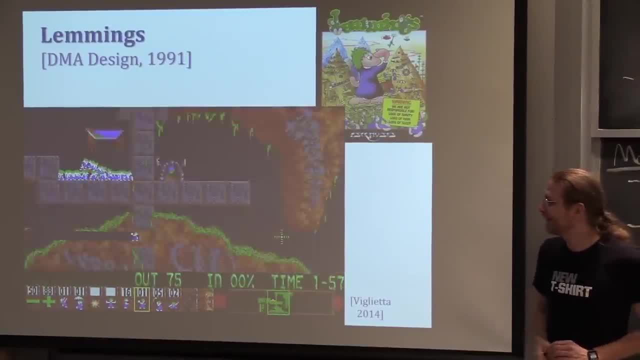 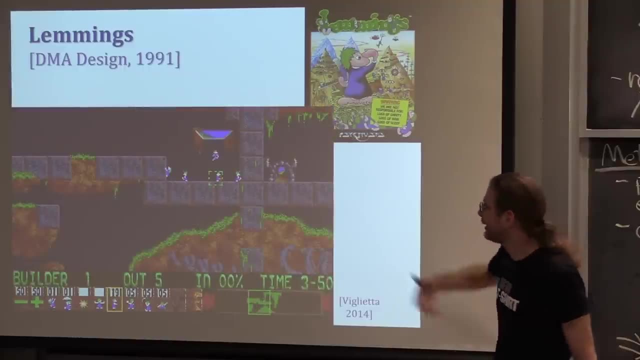 And then he said he had to delete lemmings from his computer and overwrite it in order to stop playing. It was so addictive. There are a bunch of levels, It's fun, And by now there are many free versions as well that have duplicated the lemmings, physics and so on. 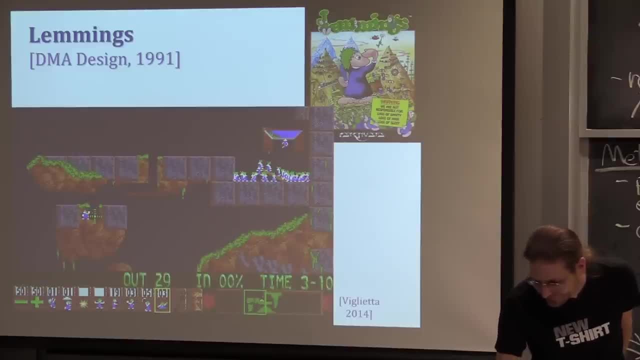 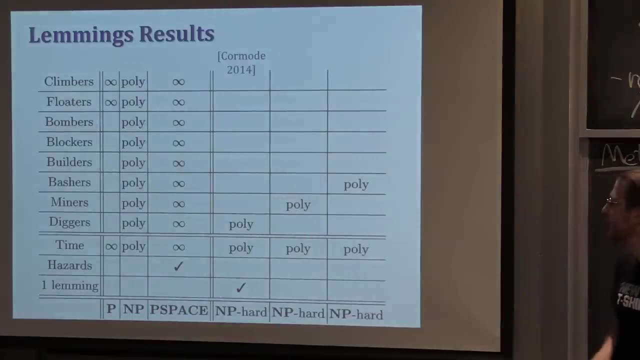 with new levels And there are level editors and all that good stuff. So you might expect this game is pretty hard. Here we're going to prove PSPACE hardness. There was the first paper by Graham Cormode which showed NP hardness and conjectured PSPACE hardness. 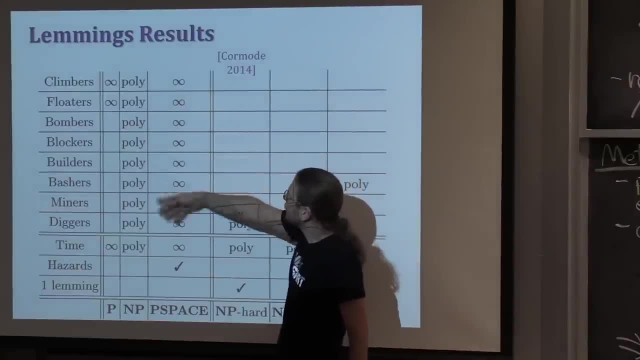 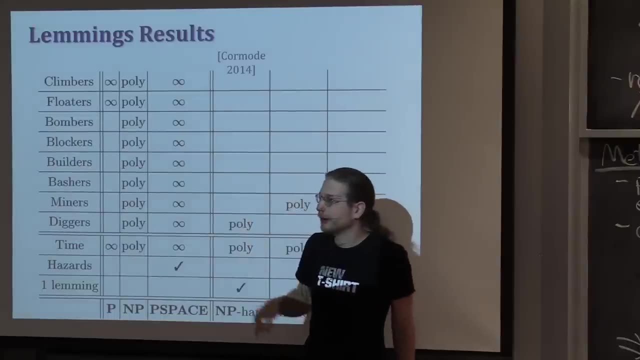 So this was the results before. But in particular, even if you assume there are all these abilities, I haven't defined all of them. I'll show you just a few of them. If they're unlimited, normally you're given a limit to how many you have. 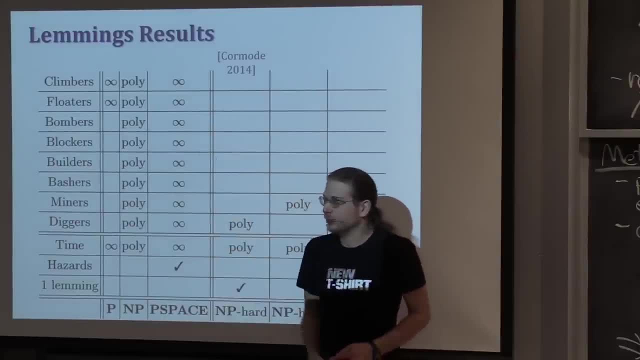 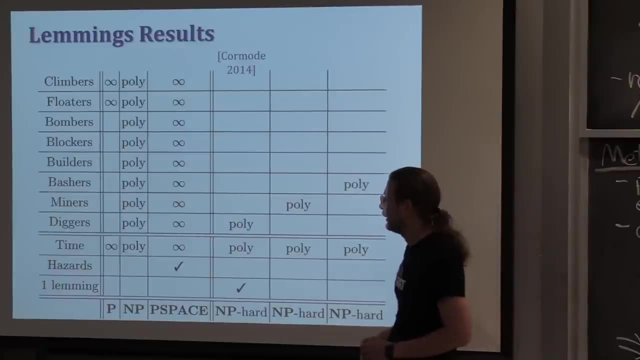 But even when they're unlimited and you have arbitrary time, the game is still in PSPACE because, again, the state is positive, It's a polynomial number of bits. There's another thing I didn't mention, which is hazards. These are traps. 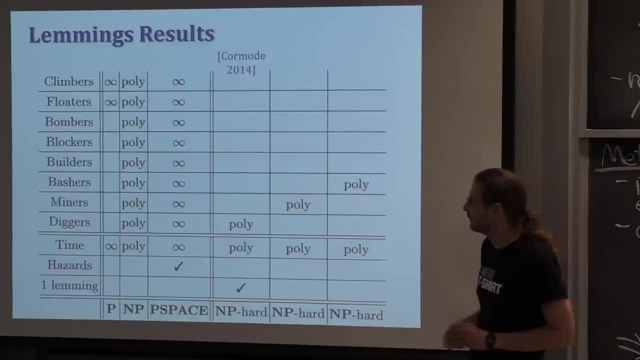 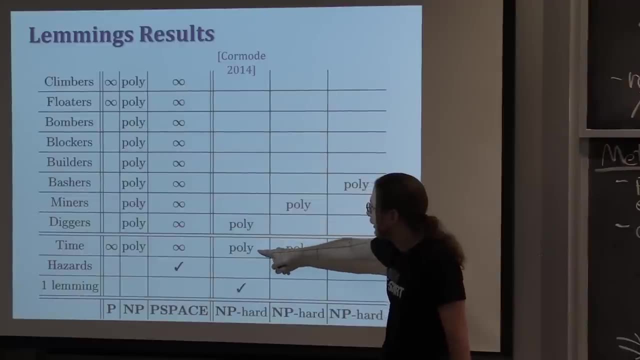 If your lemming goes there, you die. So those are also important for some of the proofs. And so Graham showed that if you have diggers and a time bound, then you get NP. With time bound, you actually get NP completeness. 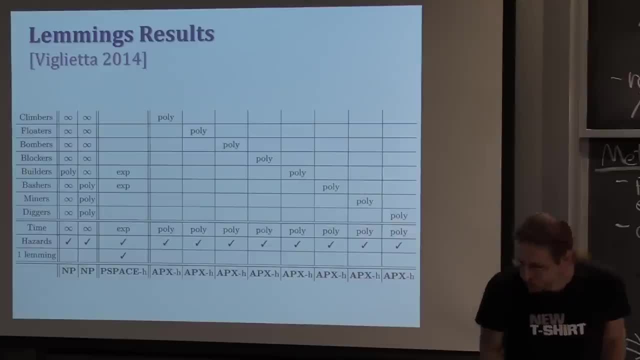 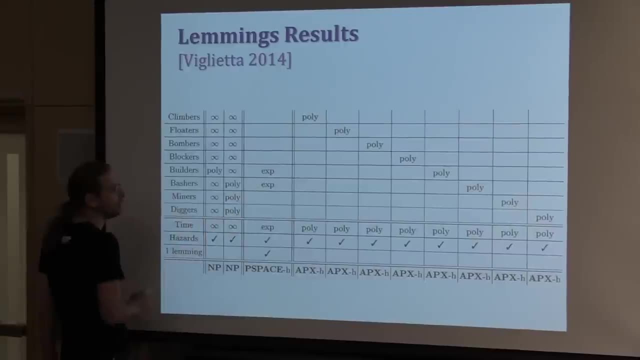 And you can convert that into other abilities. But the more interesting new results are this one We're going to focus on this column, which is given builders and bashers either unlimited or given an exponential number of them, because we need to run for exponential time and hazards. 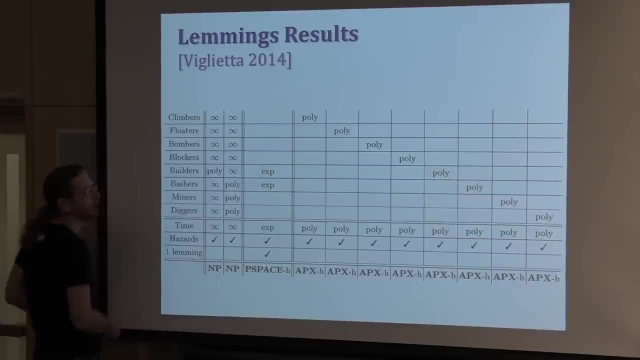 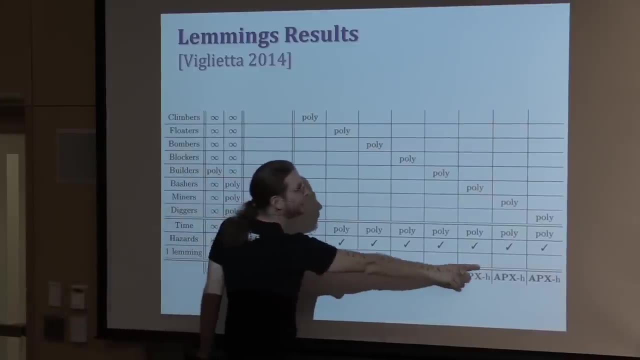 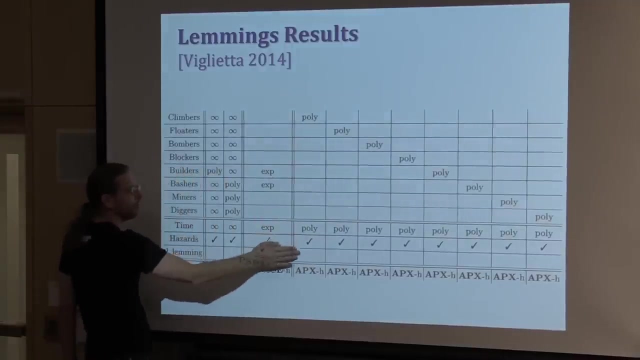 And just one lemming, the game is PSPACE complete. Another result in the same paper that might interest you, but we're no longer in the approximation section, is APX: hardness for any ability you want And a polynomial number, A polynomial number of lemmings and time and hazards. 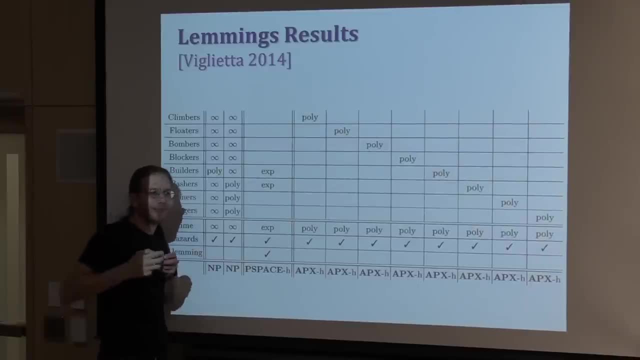 And it's based on this weird thing about hazards: If you have many lemmings go through a trap at once, then only one of them dies. The trap has to activate and it takes a certain amount of time. So if they're really bunched up, then most of them. 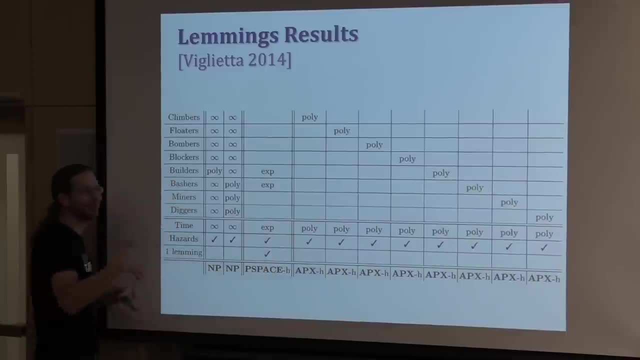 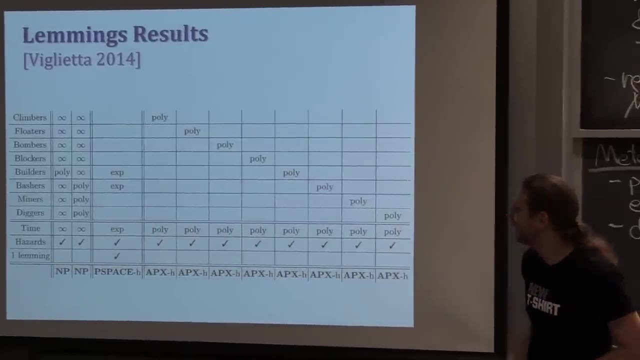 can get through. So you can use that to reduce the number of lemmings And you're trying to approximate how many lemmings get through. So that's fun. but I don't have those pictures here Because the PSPACE hardness is kind of the more impressive. 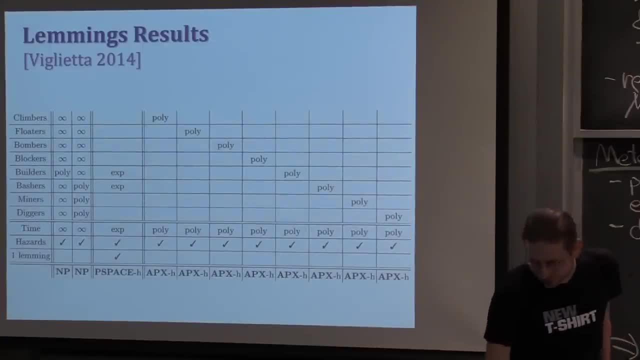 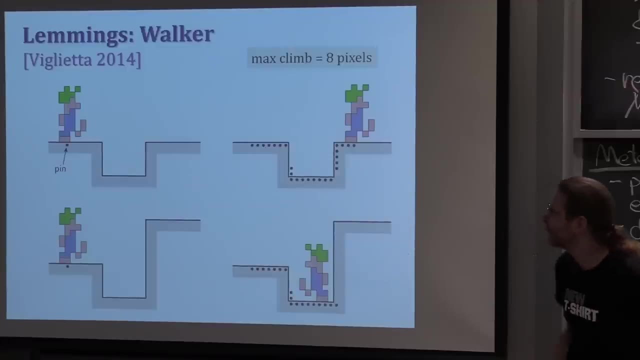 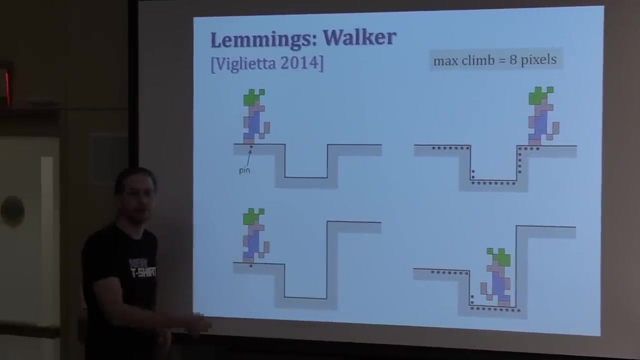 technical thing and it's already quite complicated. So in order to really get this proof right, Giovanni went through an incredible effort of documenting lemming physics at a pixel by pixel level, Because it is pretty weird, especially when you start using the bridge building. 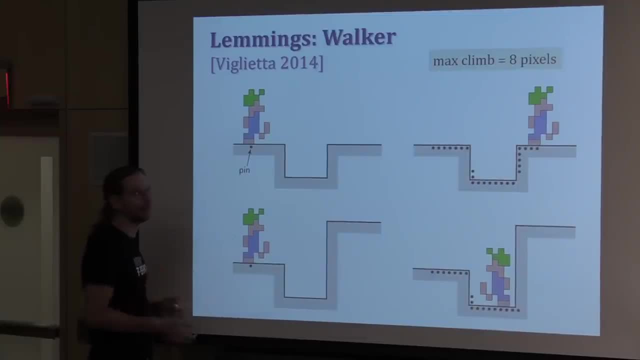 If you've ever played this game, it will stop at kind of weird moments. So here is the physics of what happens. In general, the lemming is represented by a pin right under its left foot. I don't know, Maybe that's the right foot. 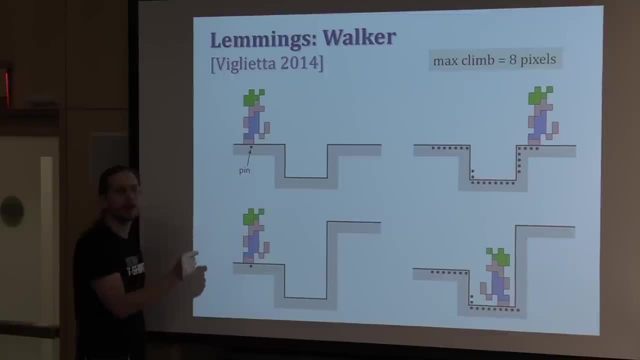 And that pin should always be on the ground. It's not on the ground, the lemming will fall. If it falls too far, it dies. but that's not relevant here. So the general walking: all lemmings start as walkers. 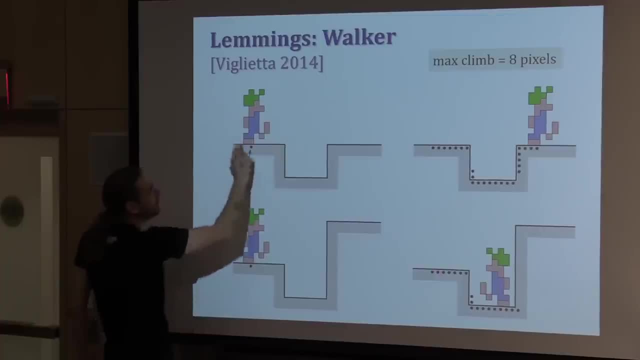 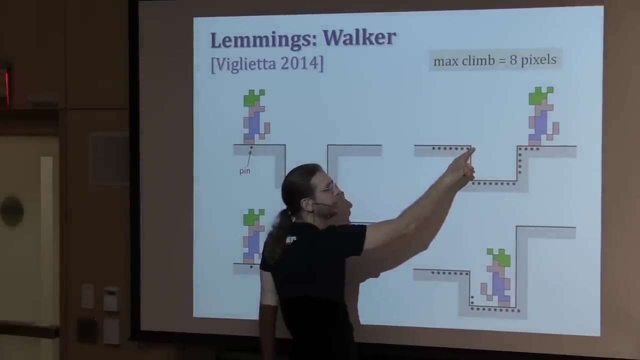 And what they do is basically move left to right. There's an animation, but mostly this pin is moving one pixel to the right at a time, And so it's visiting these things. Once it sees, oh, there's no longer an obstacle beneath me. 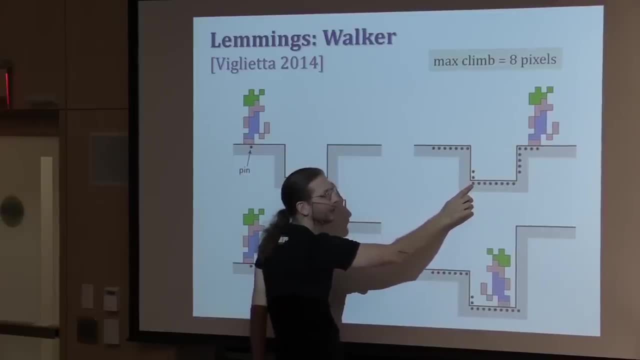 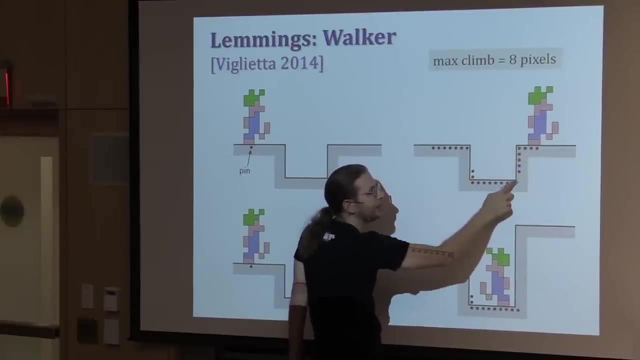 I'm going to fall this amount and then I will fall one pixel at a time until I hit the ground. So there's a gap here. That won't be important here, but these are the real physics. If I hit a step- and this is at most eight pixels up- 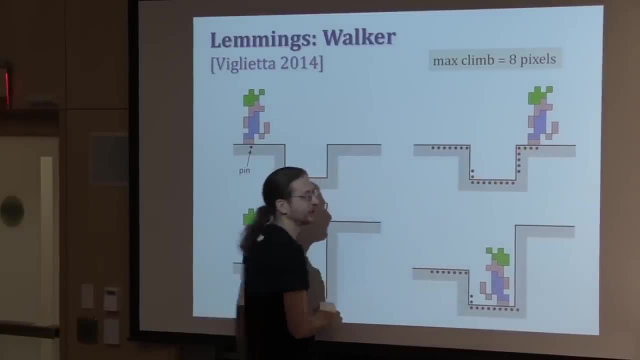 then I will rise up and go over. But if I have too big a step- more than eight pixels- then when I hit the wall I will switch directions. So in this case it will hit here and then climb back up. That is the regular walker physics. 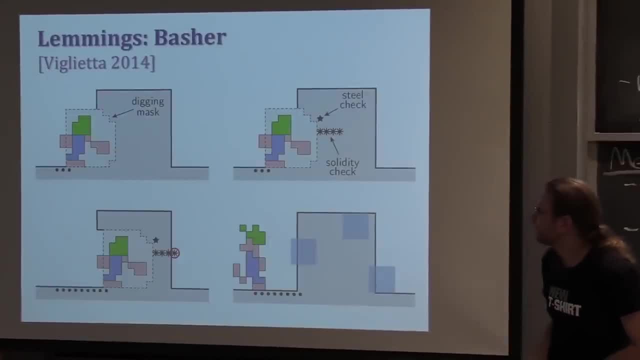 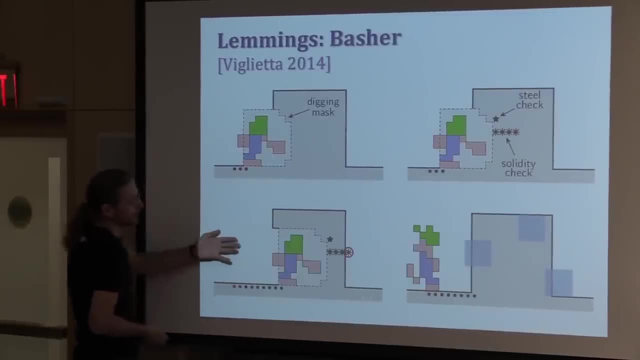 Now We're going to use two abilities. One is called basher And there's some animations here of what happens with bashers. In general it's horizontal digging, But it's kind of weird horizontal digging. There's this particular pattern that you dig. 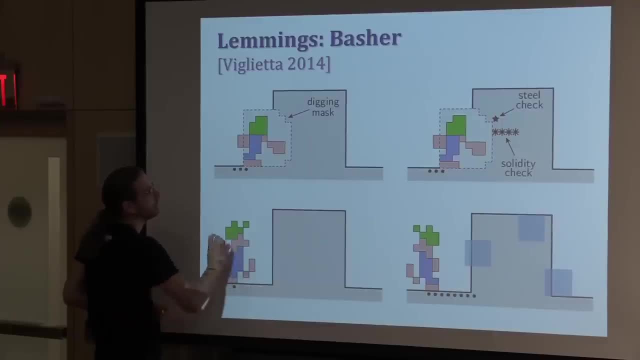 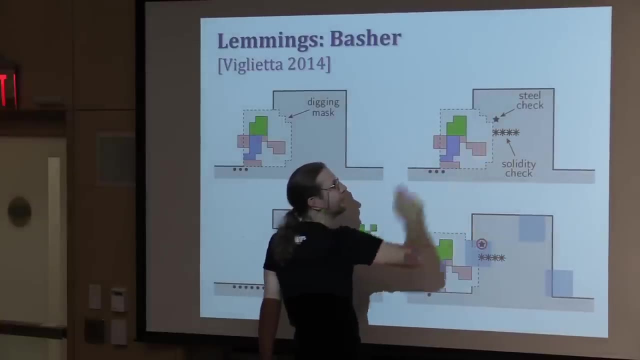 which ends up tunneling a big horizontal rectangle, more or less. But the way it tells whether it's finished is it looks at these four positions right in front of the dig mask, And if at least one of them is solid, you will keep digging. 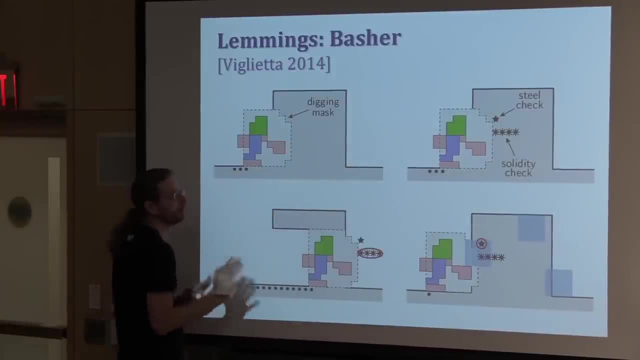 If they're all empty, you will stop digging. That's important because we need to see exactly when these things stop happening. Then you return to being a walker. So if everything is normal, you just dig through Here. that position was when all four were empty. 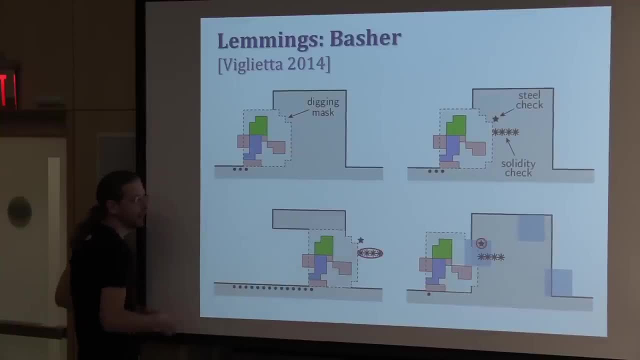 One was empty, but then all four were empty, And so then you stop digging, keep walking. But there's also this notion of steel. Any pixel can be marked as steel. It's a separate, independent bit. Usually there's some graphics to indicate. 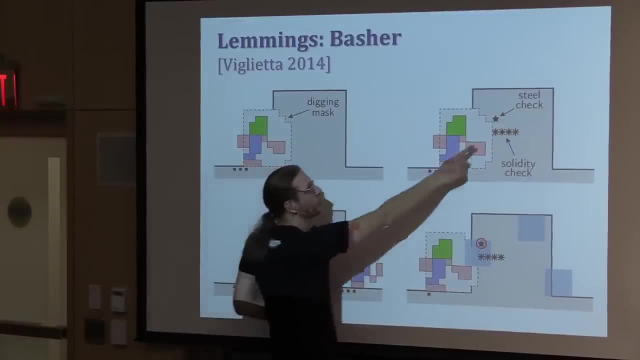 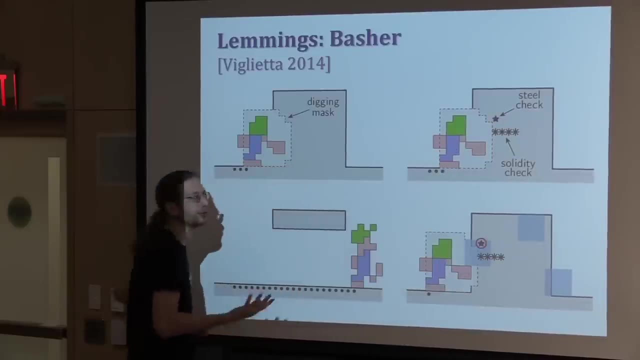 You're steel. but here we're going to use blue And there's this one steel check And if that position is steel, you'll immediately stop digging, Or you will stop digging when that star position hits the steel pixel. So we're going to use that in the proof. 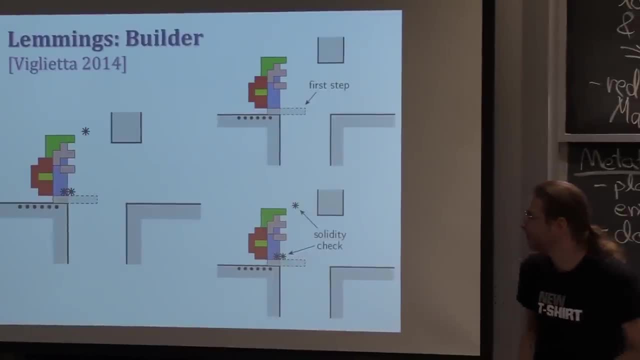 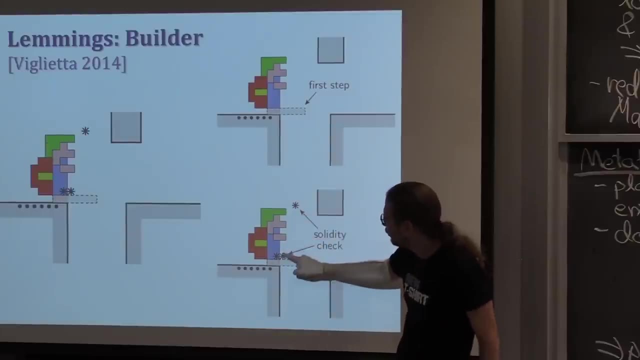 But that's how bashers work. Next, we have builders. These are building the staircases, And there's this subtlety that the solidity check are these three points. If any of them is solid, it will stop digging, And if this one's solid, you'll also switch directions. 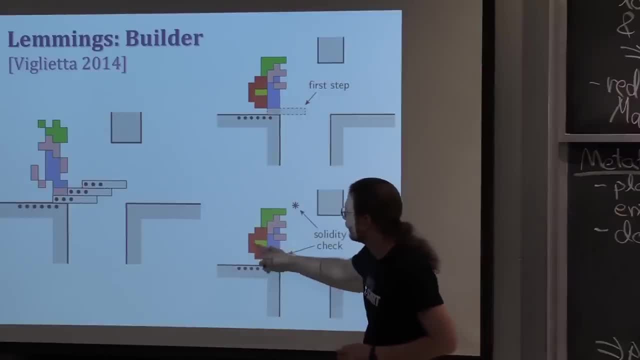 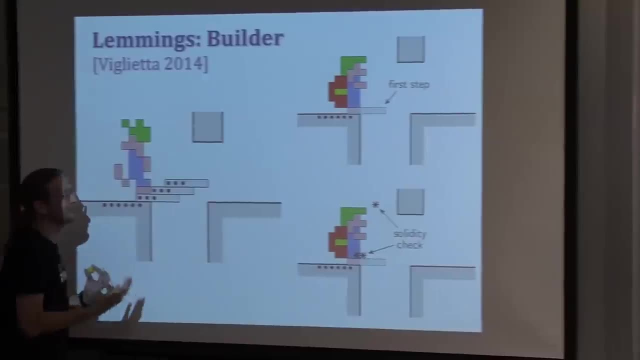 There's also a limited number of stairs, because you can only fit so many in this little bag. That won't matter for the proof. We're always going to stop before we hit the 15 stairs or so 10 stairs, something like that. 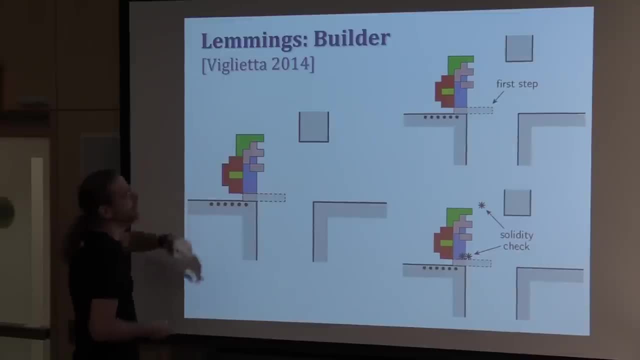 So you can see in action: here you place the step, It's right, You actually the initial step overlaps your feet, It's a step by two pixels, And then you do this offset of two to the right one up until you hit something like that: 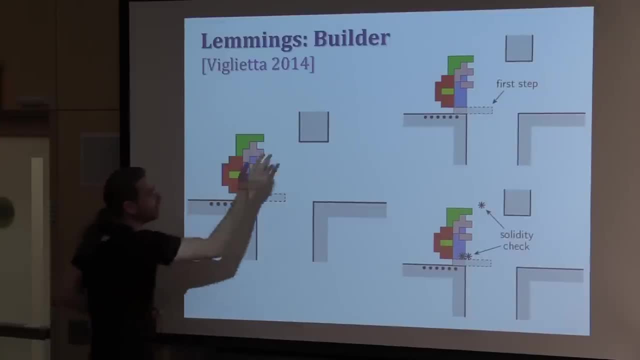 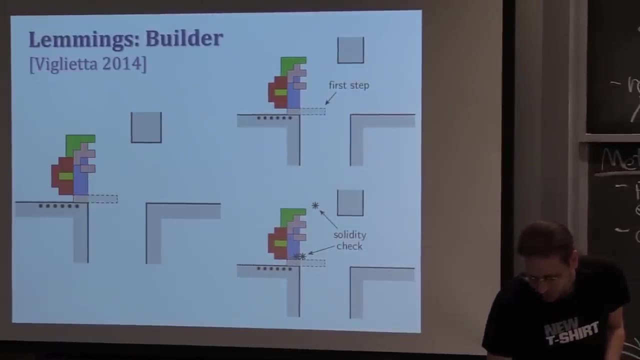 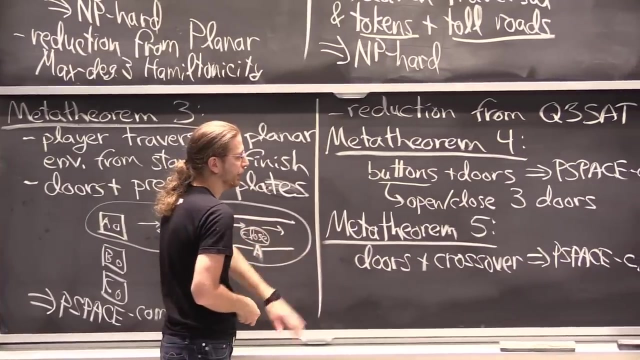 And then in that case, you turn around because you hit the wall, so to speak, But notice, there's this big gap here. OK, So now we want to use Meta Theorem 5. We want to build the door and crossover, I guess. 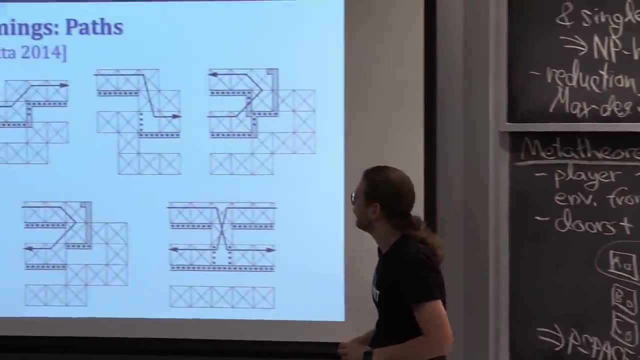 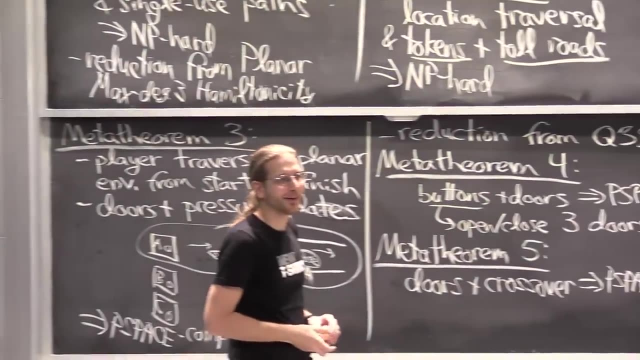 I don't know if I have the. I do have the crossover here. It's not so hard. First, we just need to be able to move lemmings around, And they move in a very simple way. Yeah, How did he check all these pixel things? 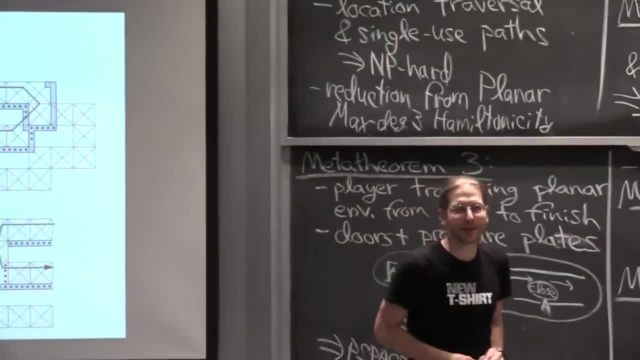 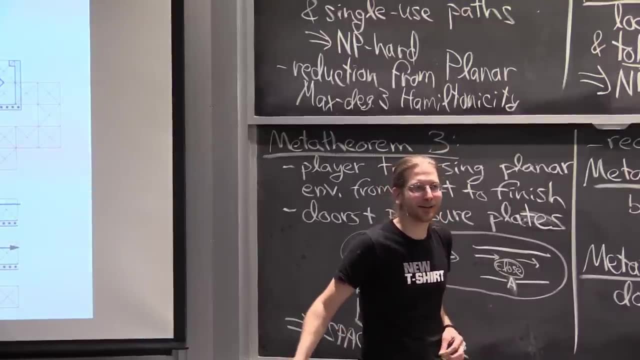 It's a good question, I think definitely. one thing he did is look at one of the clones of lemmings and read the source code How that clone was done to mimic exactly the original lemmings. I'm not sure, So I don't know whether this has been compared. 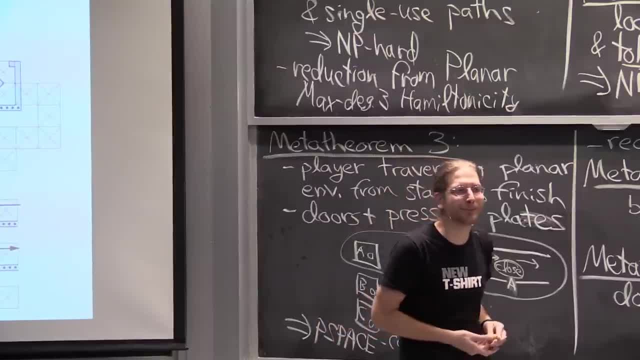 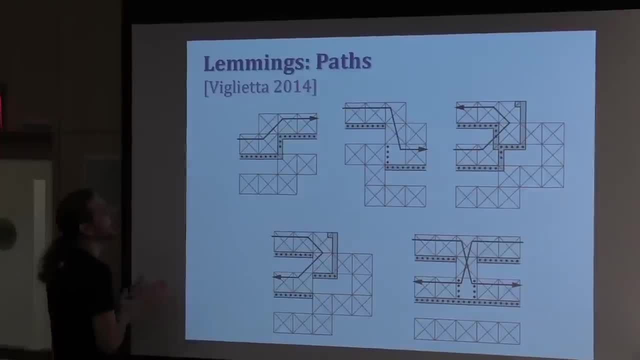 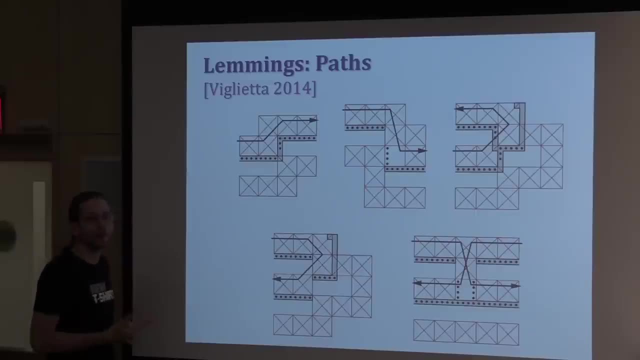 against disassembled original lemmings code or what. But I'll follow up with him. I was talking to him earlier today. OK, So we are only going to give the player the ability to do builders or bashers And we want to prevent the player from doing builders. 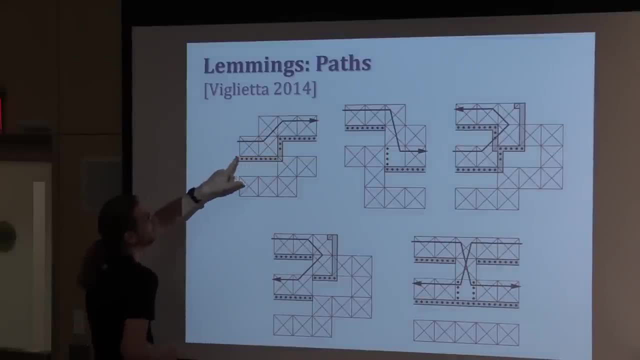 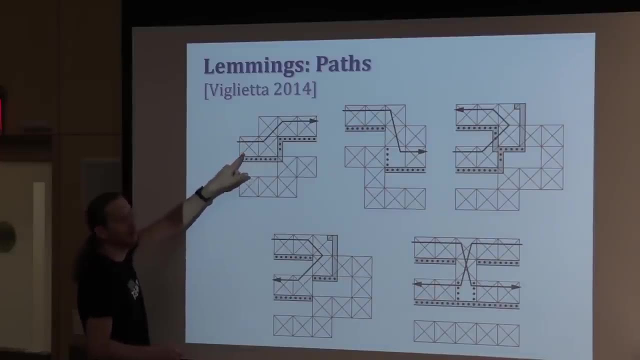 in random places. So these red things are traps. If you ever at any point decide to become a builder, you will elevate, Your dot will not be here, Your dot will be above And then it will be touching the trap and then you die. 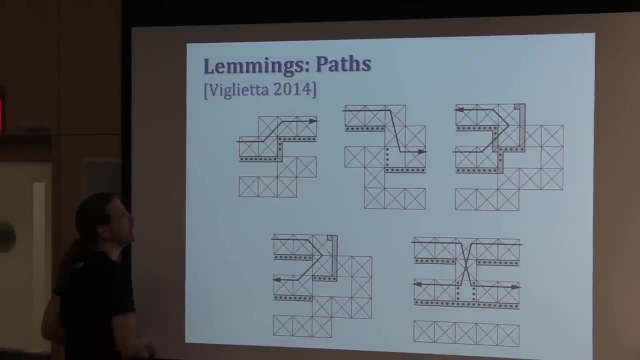 So these red things are to prevent you from building anywhere. You also can't bash anywhere because let's say this is all steel, OK, Or actually I think the whole background here is steel, except in specific places in the gadget. 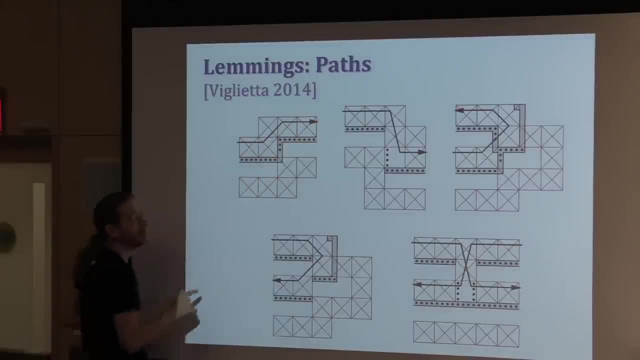 So this is a small thing. This basically lets us ascend slightly, Because lemmings only like to go left and right and there's no jump ability. we want to be able to make our wires go. We want to be able to build a graph. 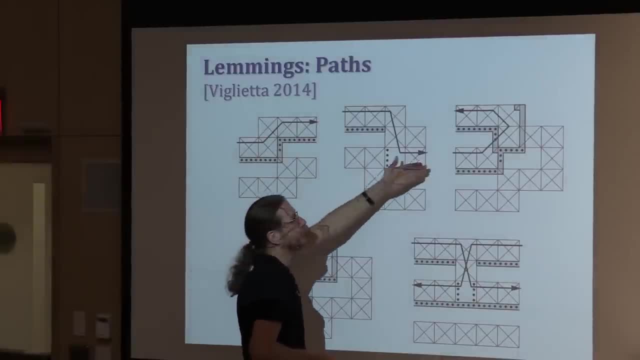 So this will let us go up a little bit. This will let us go down a little bit. This will let us change directions And going up, change directions and going down. This is a crossover, because lemmings will just proceed to the right. 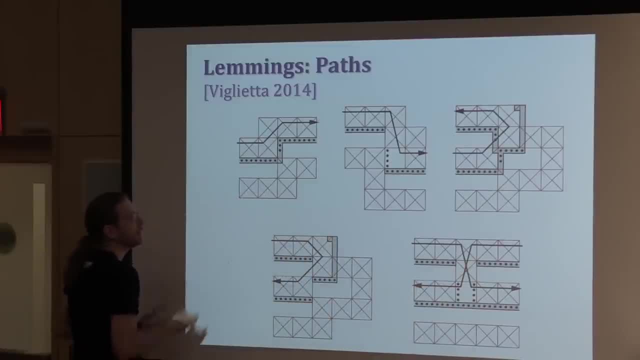 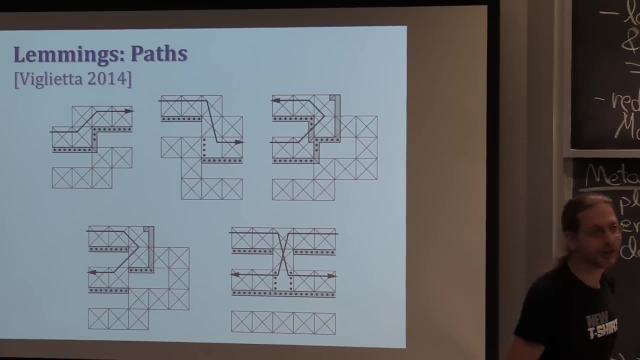 There's no way to make them change direction unless they hit something. So that's basic lemming driving We also need. these are not explicitly stated in the meta-theorem. You see here the weakness or the vagueness of the meta-theorem. 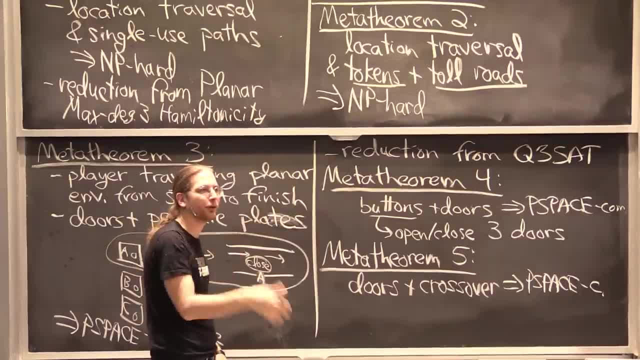 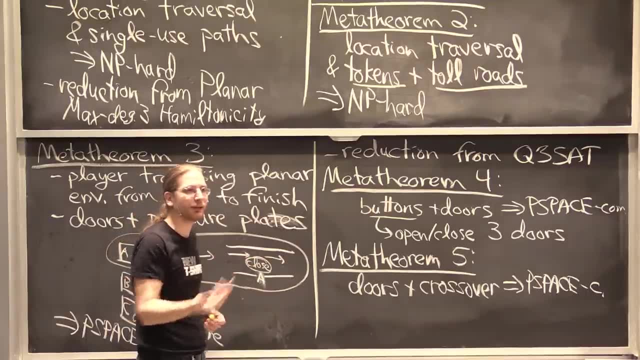 We need the ability for the player to choose whether lemmings go one way or another way. We need that, for example, in the existential quantifier. But in general we were kind of assuming that the player has this kind of agency to choose directions of lemmings. 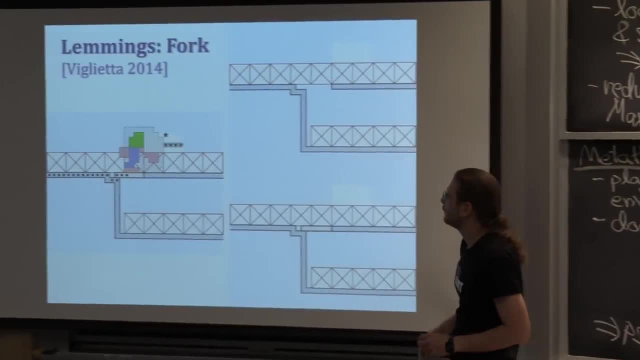 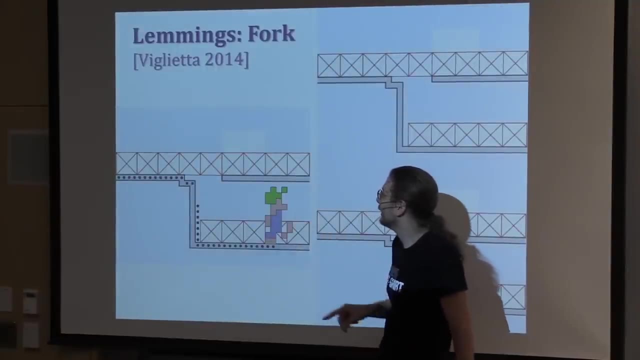 So for that we need a kind of fork gadget And you can either do a build immediately followed by a bash, or you can do a bash in order to get down. So if I do a build and then a bash, I will stop building. 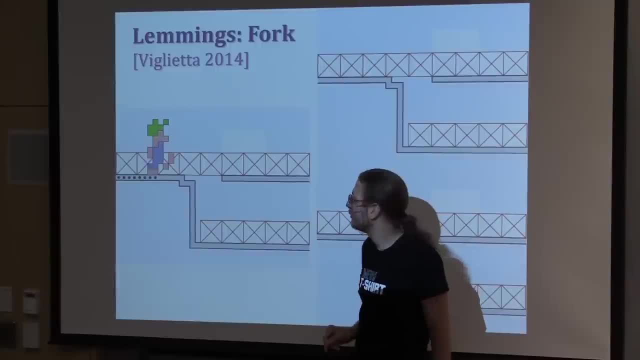 And then just make one step, Because if I made a second step, I would die from the traps That will let me choose to go to the top path, Or even if this is already there, I could bash it away. Or if it isn't there, just wait. 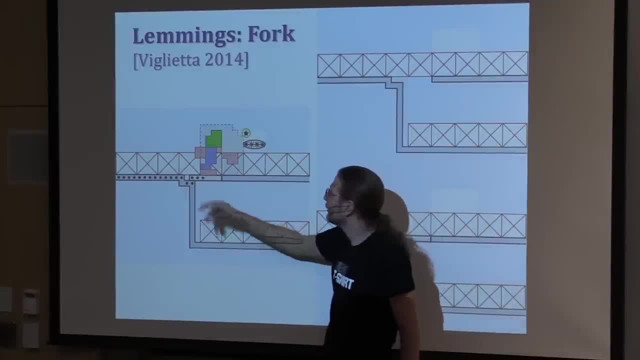 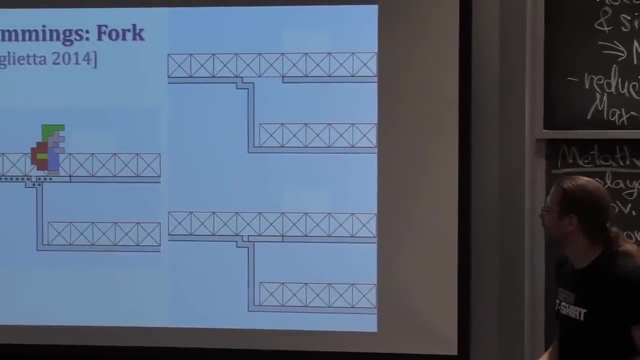 And then I will go down here. So, no matter what the state of this gadget is, I can either take the top path or go down to the bottom path, Because here I have unlimited bashes and builds. So those are the two states. 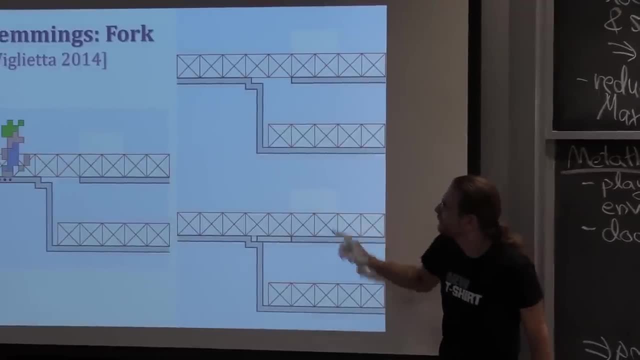 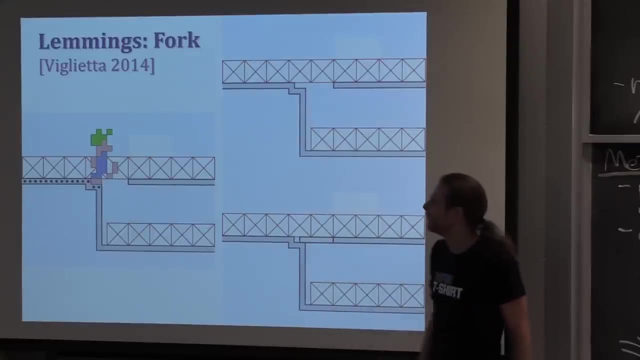 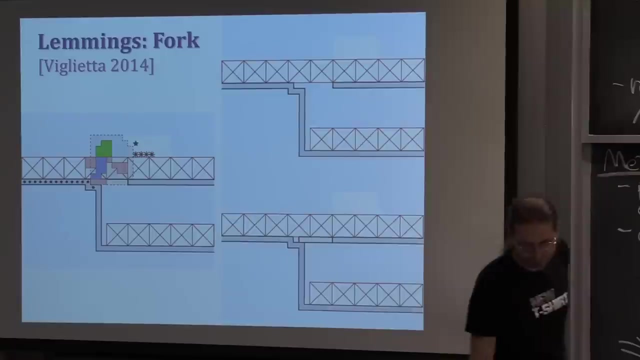 This is the non-steal part. We need that for the bash to succeed. So it ends up bashing, But because it's all empty here, you immediately stop bashing. OK, that's the fork, And finally the door. 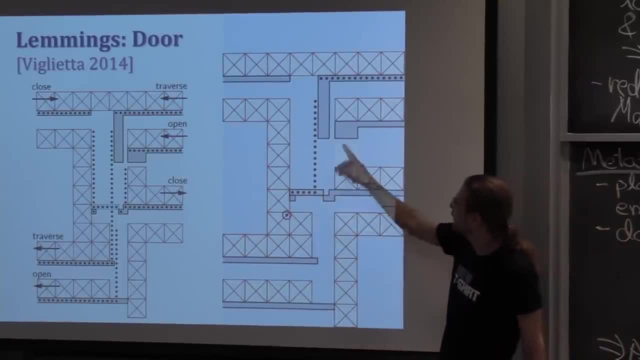 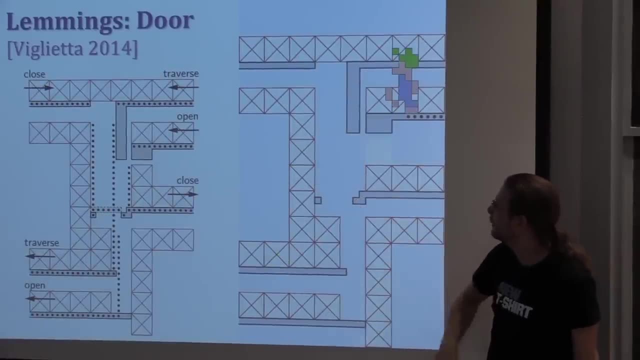 So if the door was open, you go through it. If it's closed, you die, even if you try to build a bridge. If I go this way, I can either fall down or I could bash it away and then open the door. 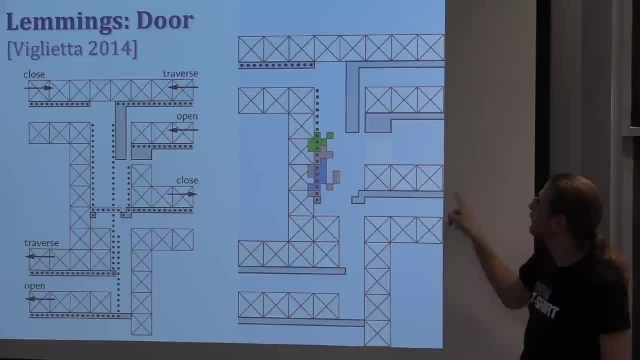 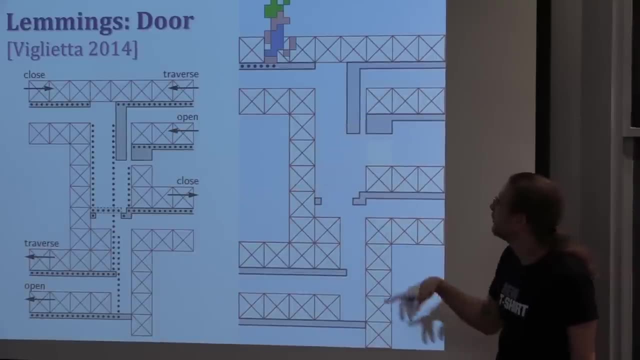 But I still fall to the bottom. If I come from here with a closed door, fine, I can exit. If it's an open door, I better build this thing. If I build too far, I'm in trouble. But if I build just once and then immediately bash,